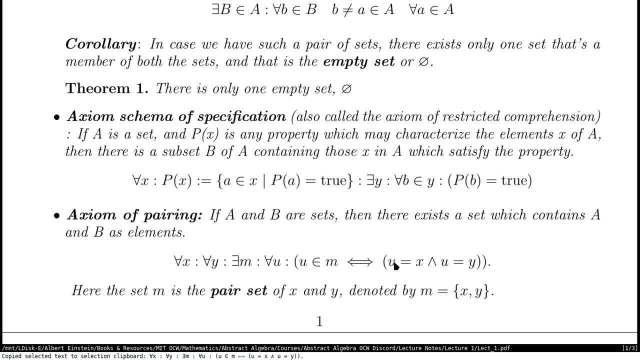 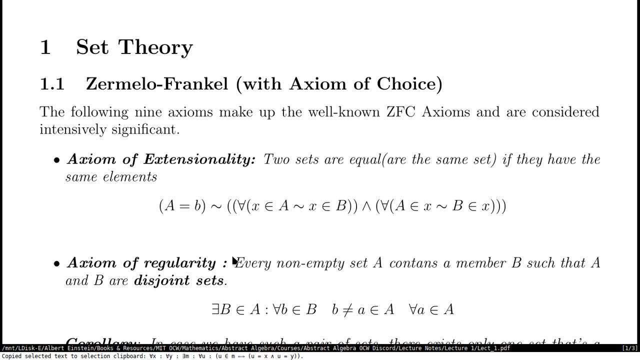 write it using logical operators and symbols. There are a few typos, but that will make it fixed. So the goal is, you know you should like develop the kind of thinking which results in like when you see this kind of like sentence, normal sentence. you should 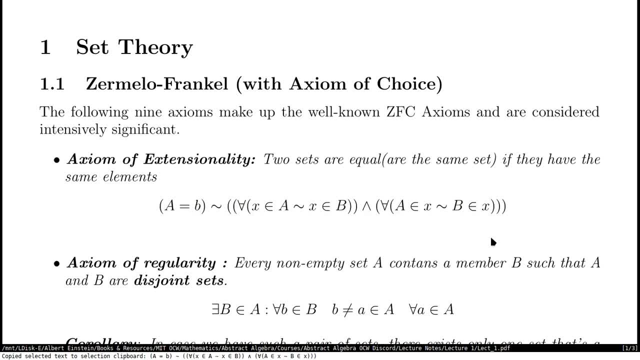 think of the mathematical format of it and symbols, And this will be very useful when you go to writing groups, which is THE most important thing in an algebra course. So the axiom of extantiality says that if your set, A is equal to B. so this actually 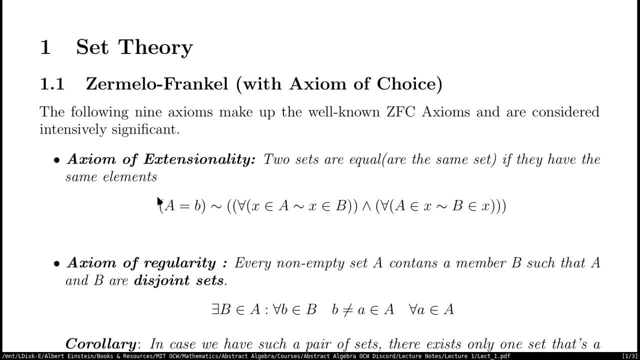 should be uppercase: B. A is equal to B. so when you say this, this is actually saying that talk is about the same as the word experiment, because A is equal to B in algebra. is equal to b is a statement that is true. So this is what the 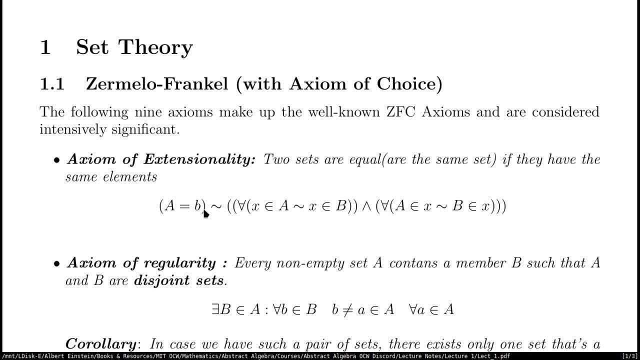 current is using, So it's a statement that is true, Then that statement being true is equivalent to saying that for all x in a, it's equivalent to all the elements x in b, And so this is the symbol for, and such that for all the 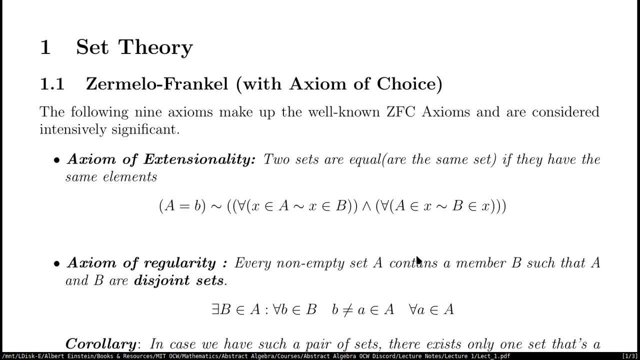 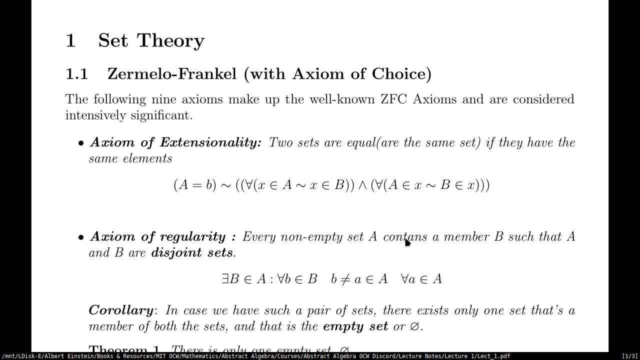 sets a in x. you can equivalently write down b, all the sets b in x. So this lets you use the epsilon relation, the member's relation with sets. So yeah, that was the first axiom. It doesn't really have any kind of. 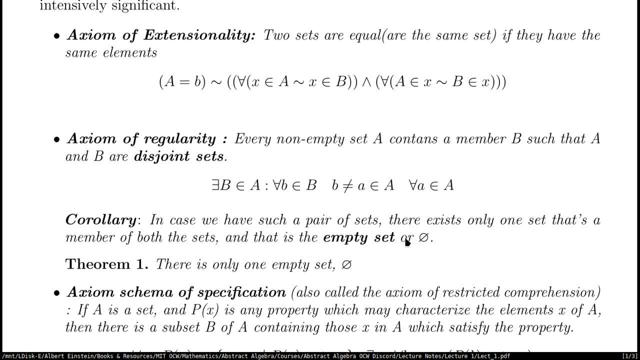 meaning Like anything else, to say that's just limited. And also I forgot to say: but when I'm talking, this is not really a lecture student kind of format. You can actually speak whenever you'd like to. You can just. 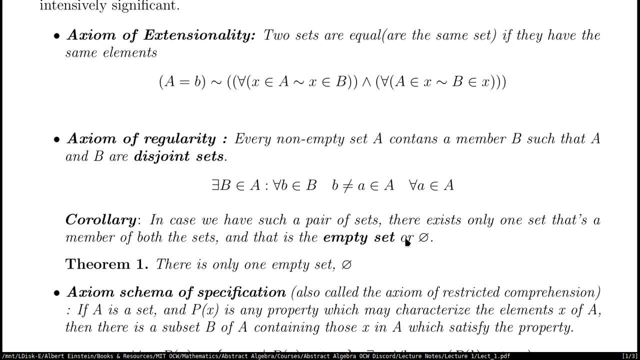 either interrupt or you can say anything in the text chat. But yeah, this is supposed to be interactive and a discussion kind of thing. Okay, So we have the second axiom. The second axiom is about regularity. So this makes it clear that every set that is 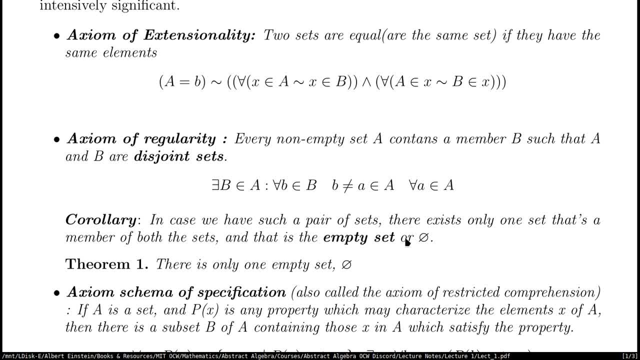 non-empty must contain a member right, So it must contain another set within itself, such that the parent set and this set, the other set b, are actually disjoint right. So they don't have any elements involved. They're just in common between them. 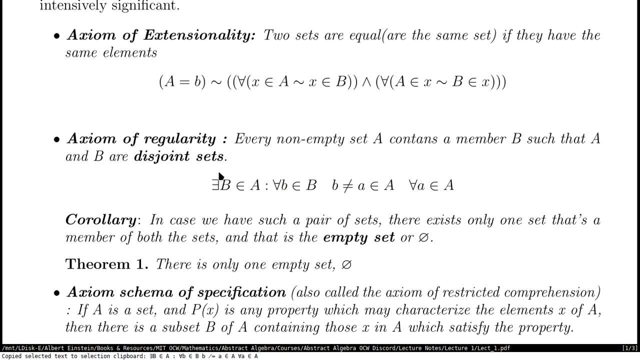 So the axiom can be written down in this manner. So there exists a b in a, such that for all the lowercase b, the elements in capital B, it is never equal to any of the elements lowercase a in this set a. So that's the disjoint property right. 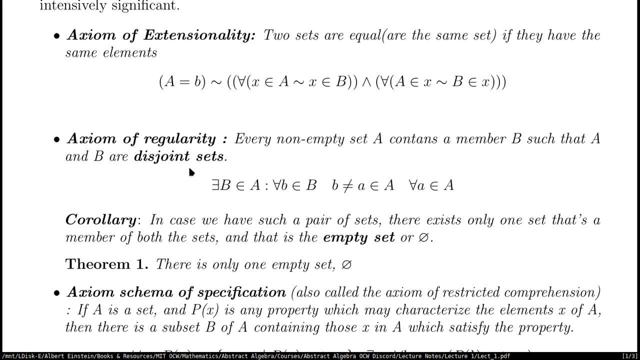 One of the interesting corollaries of this axiom is that one of the interesting corollaries of this axiom is that one of the interesting corollaries of this axiom is that if you have such a pair of sets, you can say that the only set that is actually a member of both 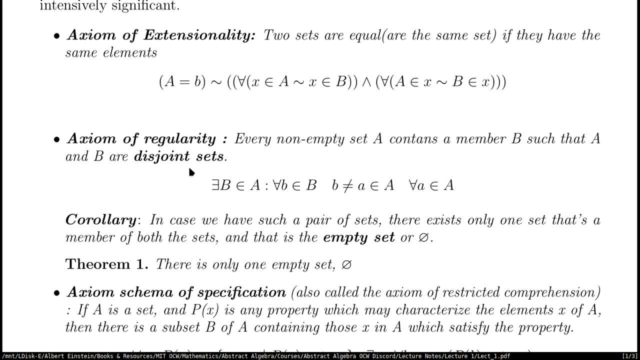 of those sets is actually the null set, the empty set. all right, So that's 5.. And indeed you can't really state this without actually having this as an axiom. so this is the axiom. Then we have the corollary. 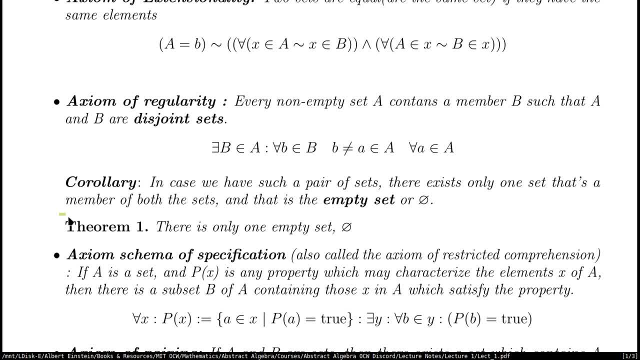 And then from the corollary, you can actually give it what you can enter for the set, have the theorem that there is actually only one empty set, and this is a theorem you can try. this is: this would be a good exercise, actually, of like dealing the. 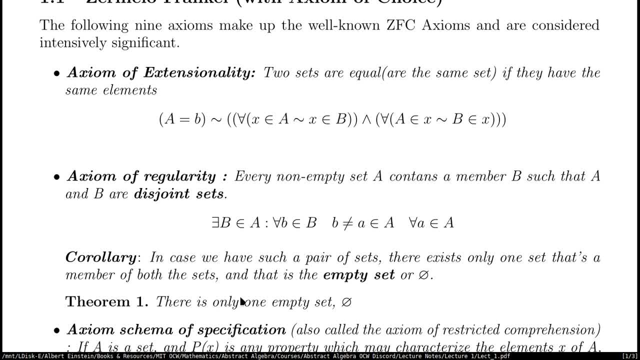 axioms, you can try to prove that actually there is only one empty set possible. the way is that you assume by counter, assume with the intention of contradiction- that there are two empty sets and then you try to follow from the axiom of extensionality and then you reach a contradiction that I know two. 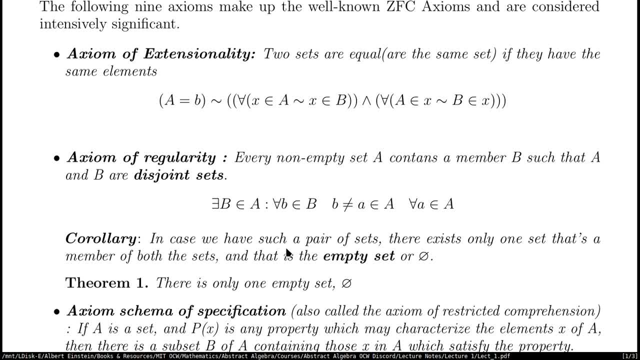 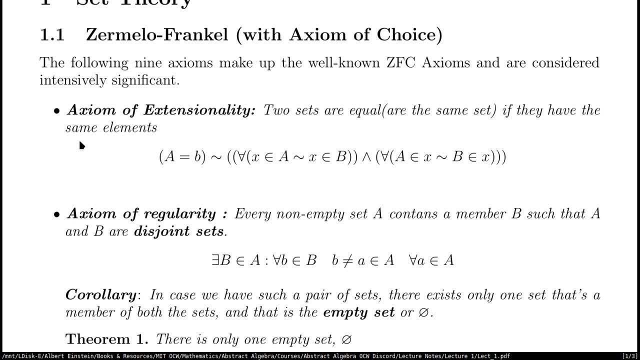 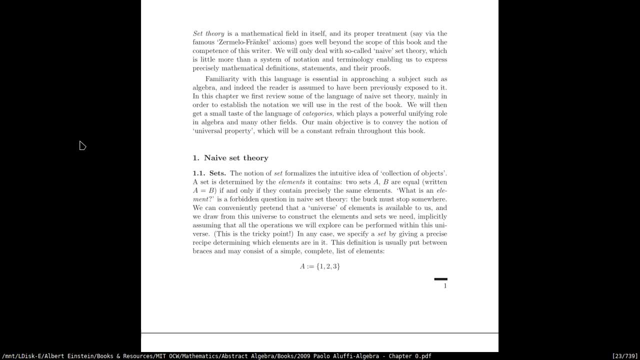 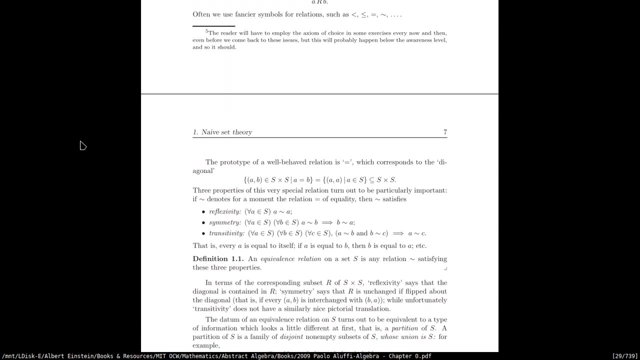 sets cannot be the empty set. okay. and there's the other interesting thing about these two axioms is that the Russell's paradox- this is actually mentioned in the Luffy mentioned- I don't think in these sections, but it's in the exercises. it's not on the key set, certainly, but it's in one of the exercises that you 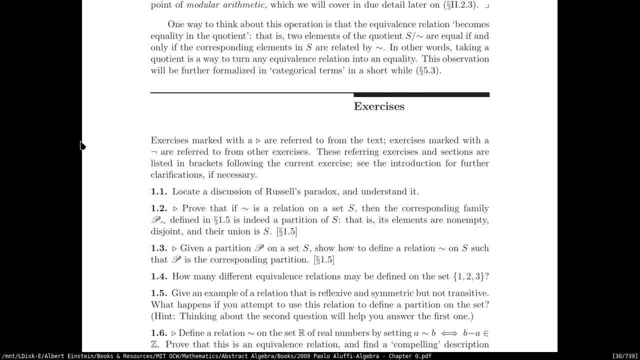 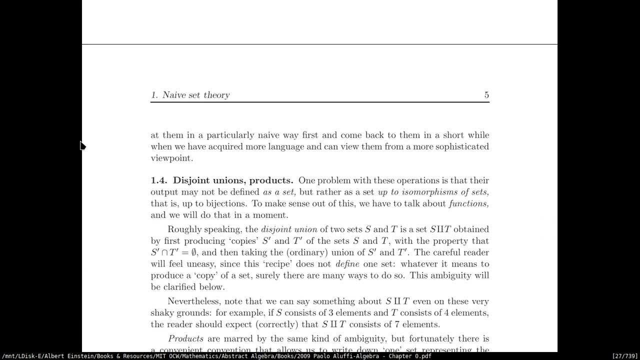 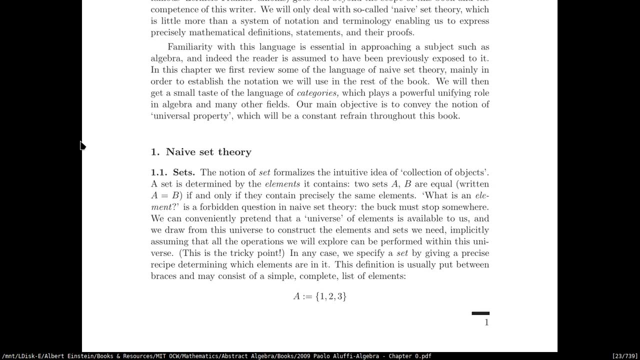 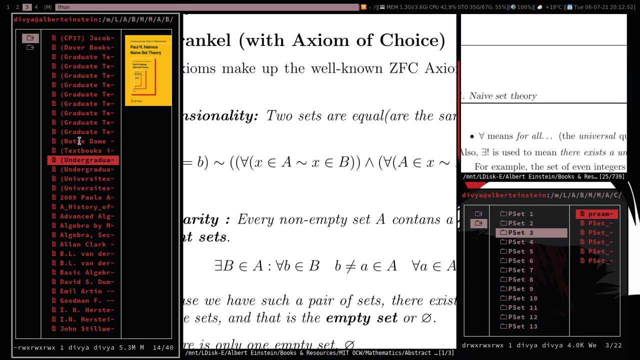 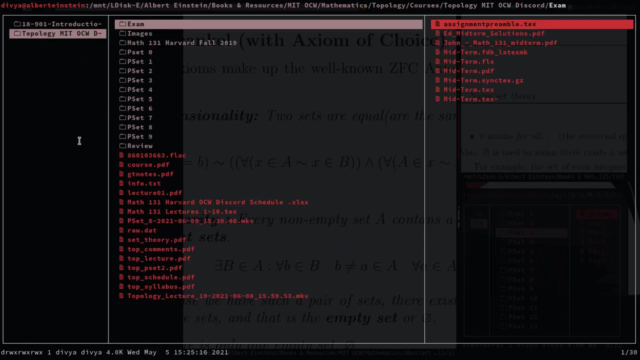 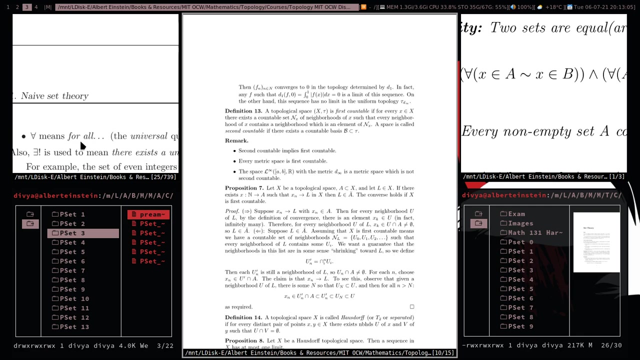 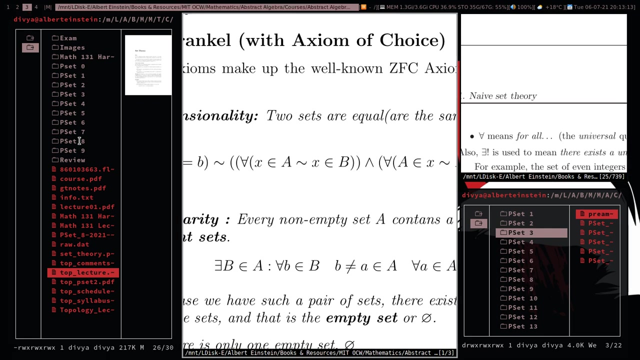 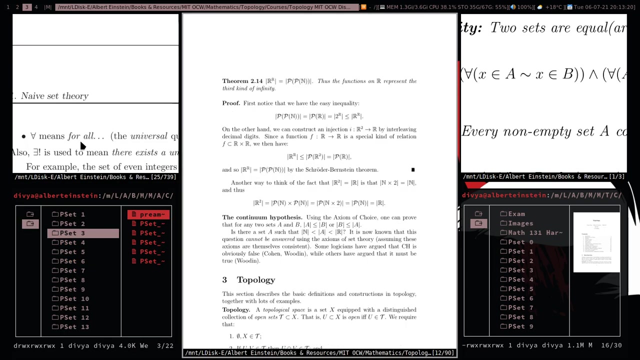 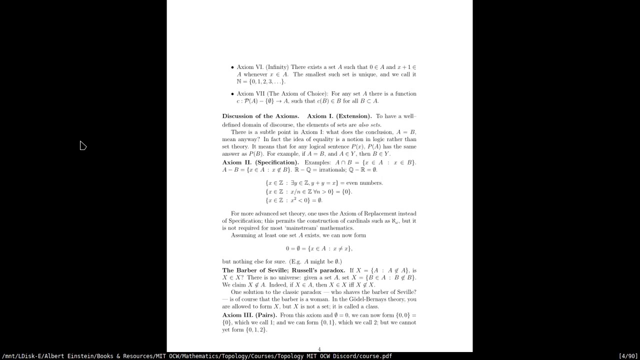 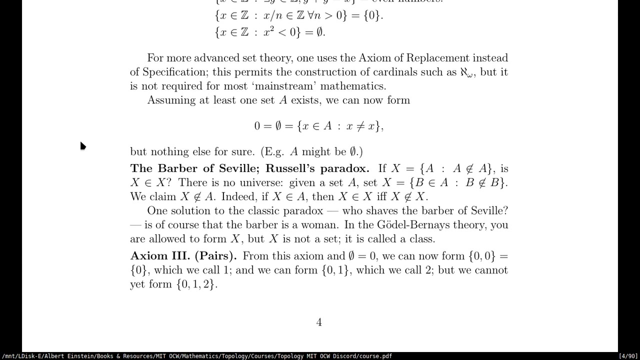 have to understand what the Russell's paradox is. so if we go back a bit, I can, you can find it. I know I thought it would be here. yeah, I'll get back to my sectarian notes. yeah, so this no random. yes, obviously versus paradox, and just forgot which file it was also. 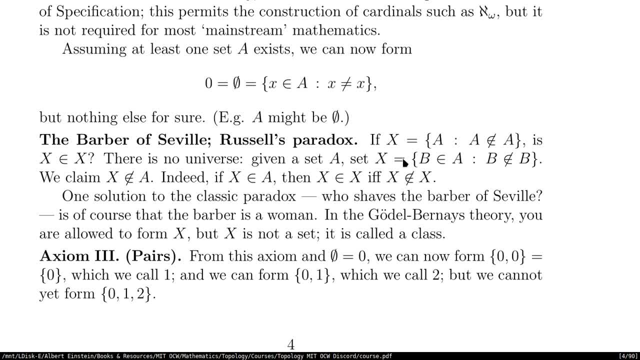 Russell's paradox is that if you have a cent a, if you have a set X which contains a and a is not an element of A, and then is X an element of X. so is the union of such A's? is it going to be X? 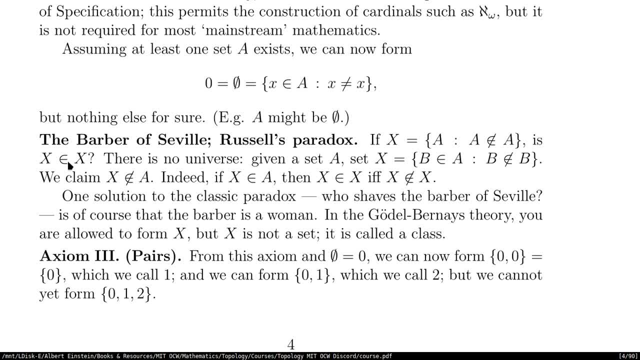 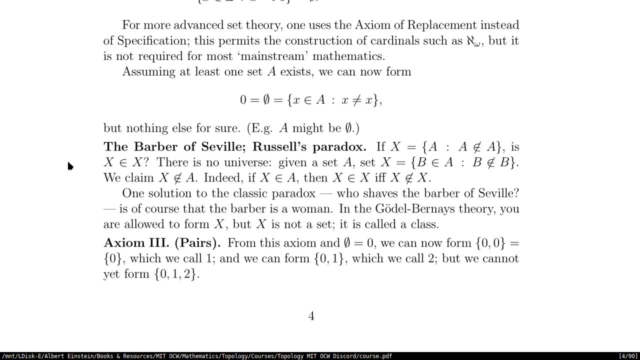 And the answer is no, And there is actually a proof for this, which is interesting. What's more interesting than the proof itself is how to think about it, And it's kind of paradoxical, but this is actually pretty straightforward from the axiom of extensionality. 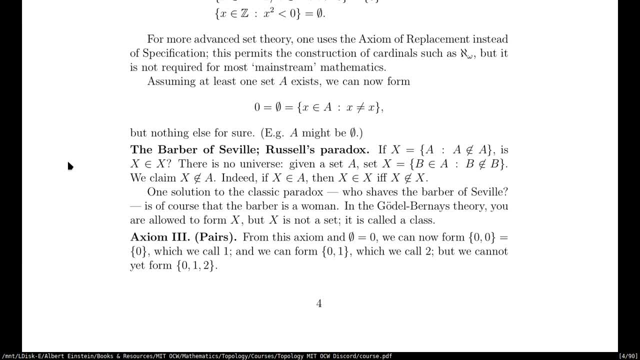 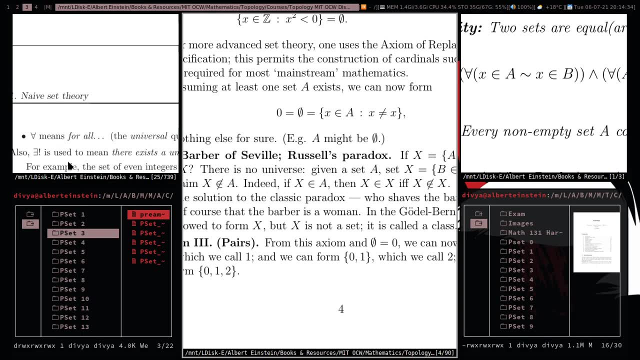 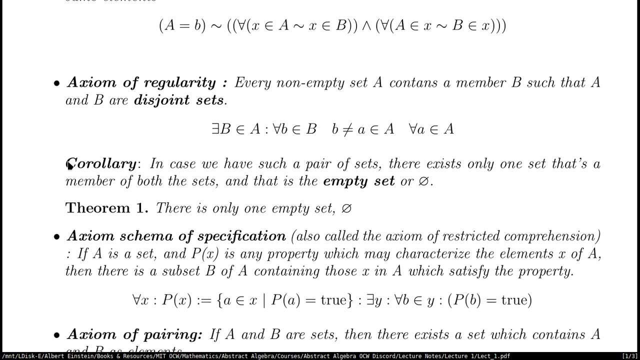 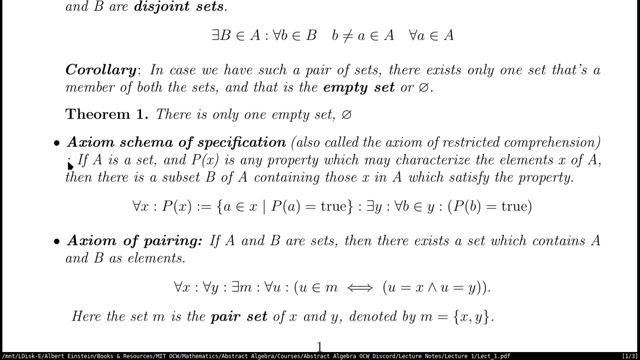 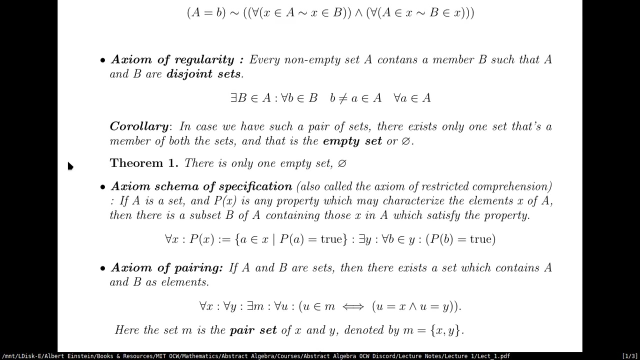 and the other one about the disjoint sets. Using those two, you can approve it. So yeah, that was the axiom for regularity. OK, so now we have the third axiom, which is for the schema of specification, But it's more generally known as the axiom. 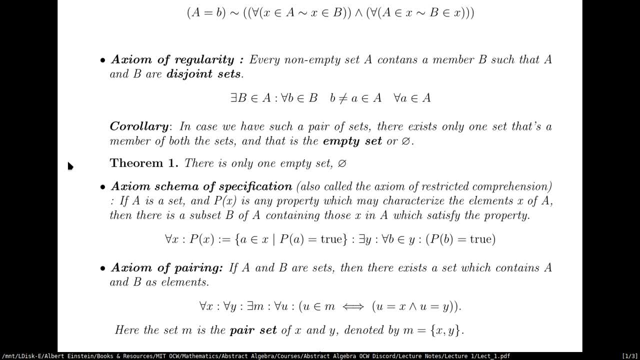 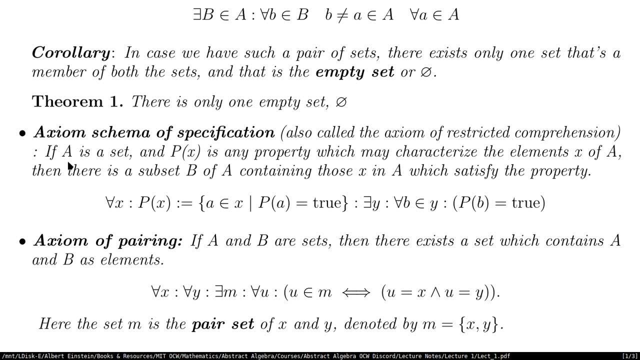 of restricted comprehension And this can kind of sound daunting, but it's kind of a very straightforward. So you have a set A And on this set A P of X is a property, any property which characterizes the elements X. So if you have that, then there is 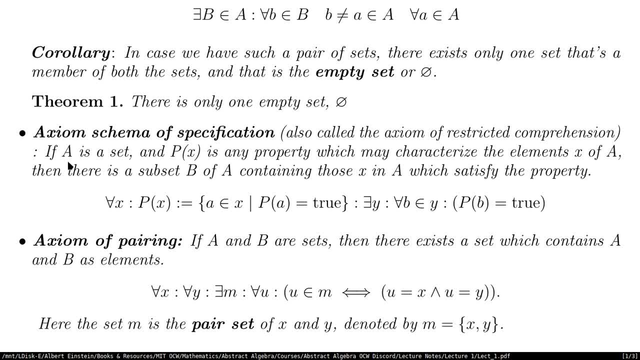 a subset B of A, which contains the elements of A that satisfy the properties here. Mathematically, what you can do is write that for all X. so here X is a set. for all the sets X, you have this property P of X, which is defined as picking out. 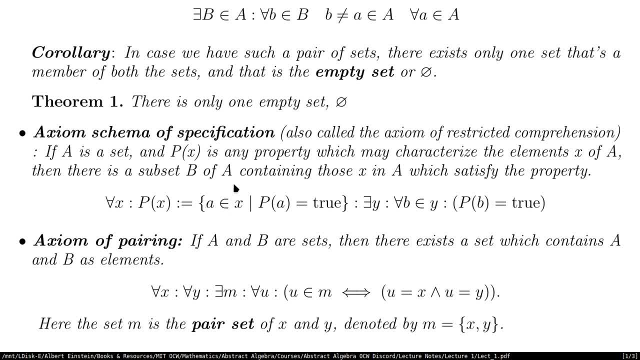 all these A's From the X, such that P of A is true. So P of A being true means that this property holds for this element right. So this element has the characteristic that the property is trying to look for. So if you have that, if you have such a property, P of X defined on X. 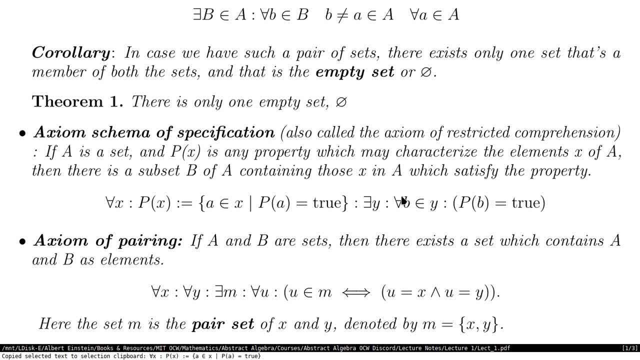 then there exists a set Y, such that all the elements in Y for all the elements in Y. this holds right. So P of B is true for all the elements B. So what that means is that all the elements of Y satisfy the property right. 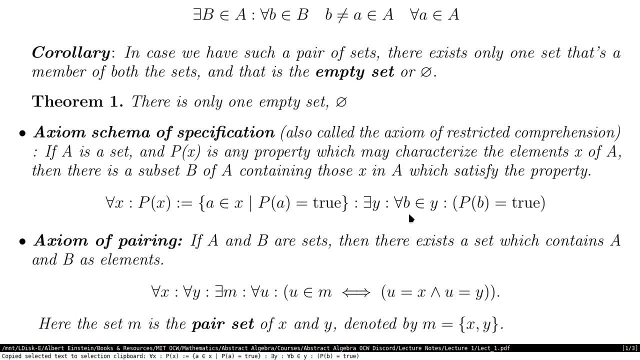 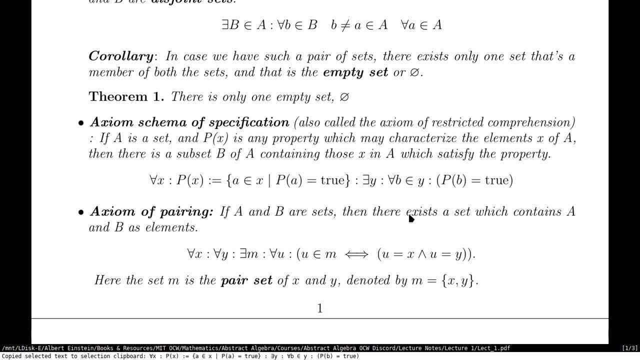 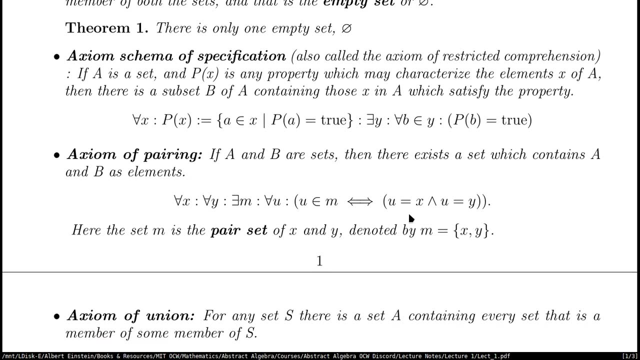 And thus you get Y as a subset of X, right? Okay, so that was the restricted comprehension X. Then we have the axiom for pairing, right. So this is important. especially the direct result is the Cartesian product, if you know. 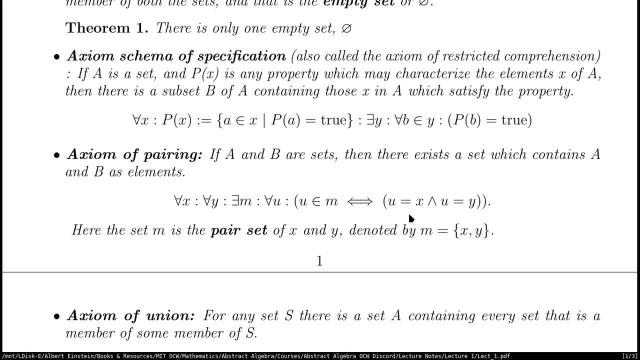 about it, Except that's a very special case. you have an ordered pair, but this is just an arbitrary pair. So if you have two sets- A and B- then there exists a set which contains A and B as its elements, right? 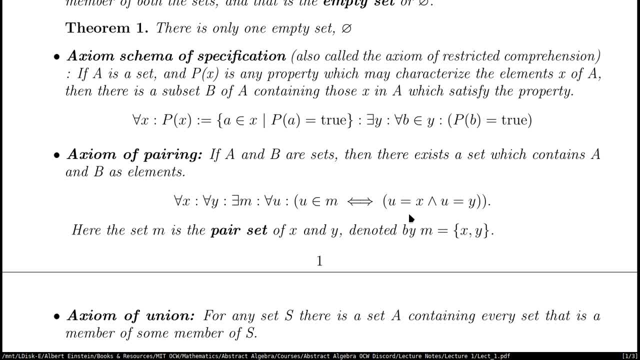 If you have A and B as sets, then you can have another set in which A and B are elements, right? So you have the set X and set Y. then you can say that there exists some set M, such that for all U in M, it is equivalent to saying that U is equal to X and Y. 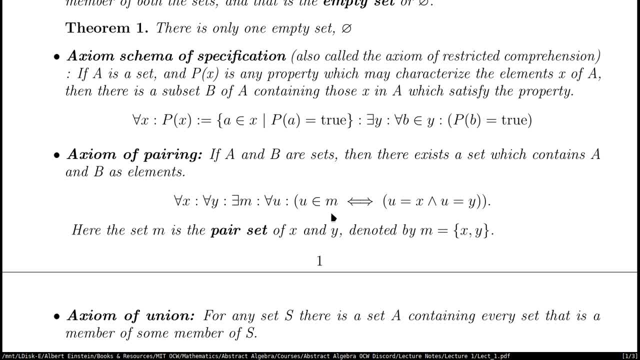 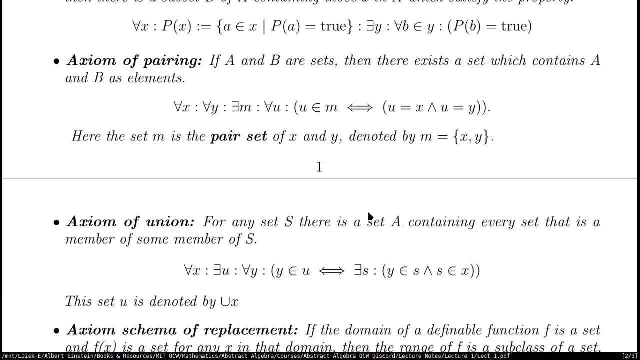 So So the thing is, every element U of M is either going to be X or is going to be Y. okay, So what that leads to is having a pair: X and Y and M is the pair set, which includes them as a set. 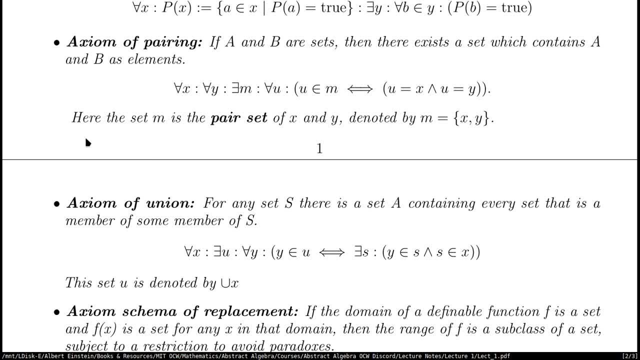 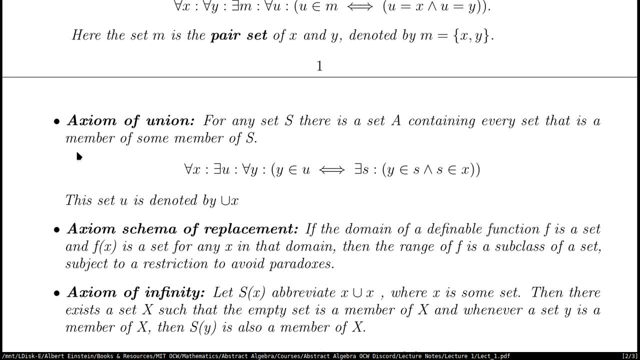 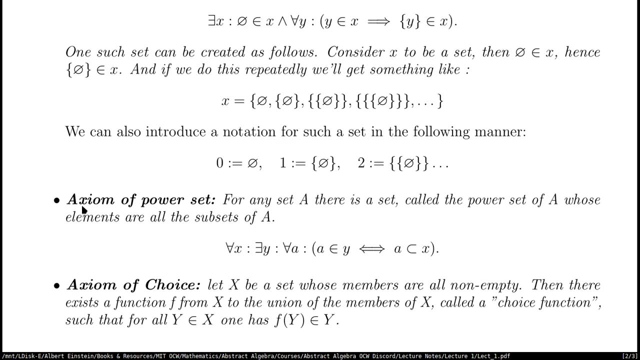 So yeah, this is the axiom of pairing, which lets you pair stuff, And this is important. when you have a lot of subsets, essentially you can. there is also the axiom: if we go down for power set, and the power set axiom actually depends on: 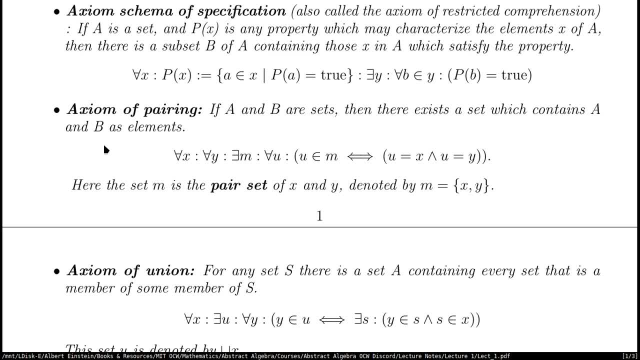 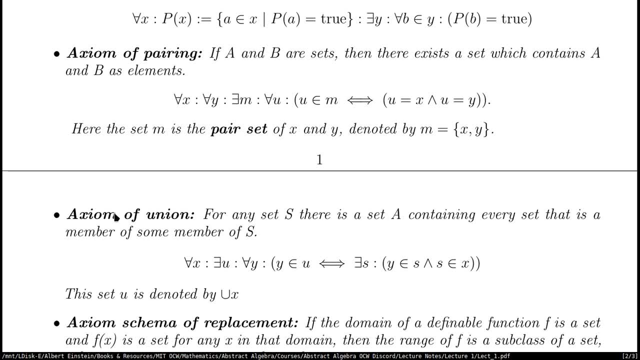 the axiom of pairing. without the axiom of pairing, you can't have the power set, So okay. so the next axiom is the axiom of union. So if you have any set S, then there is the set A, which contains every set, that is a. 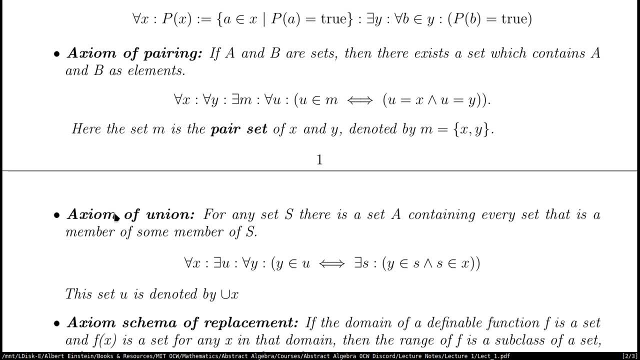 member of some. member of S. That sounds confusing, but all it's saying is that if you have a set S, then you can have a set S that is a member of a subset of S. So yeah, there is a set A which contains every set that is a member of a subset of. 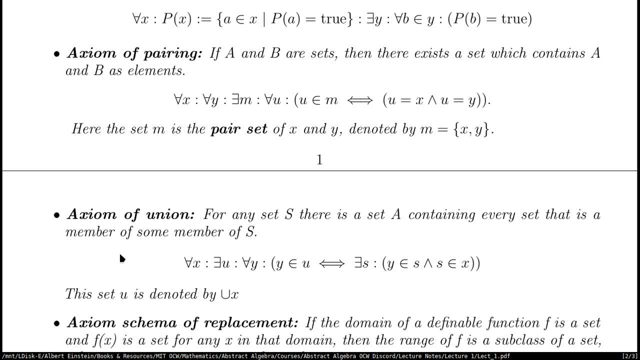 S. So essentially, S has a lot of sets, some of them like they're subsets- And then there is a set A which is containing, which contains every set that is a member of the subset of S. So let's see this logically. 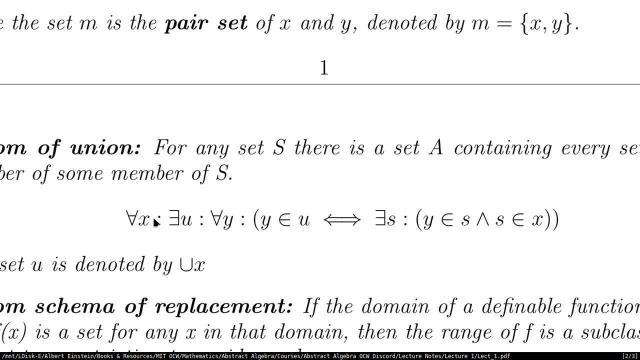 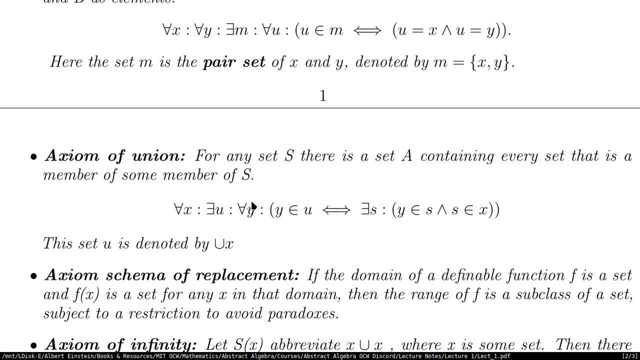 So logically it's saying you have a set S, Yeah X. then there exists a set U, such that for all the sets Y being right, so the set Y is contained within U. and that's equivalent to saying there exists a set S such that Y is in S and S is in X, so Y is in the set S and S itself is a subset. 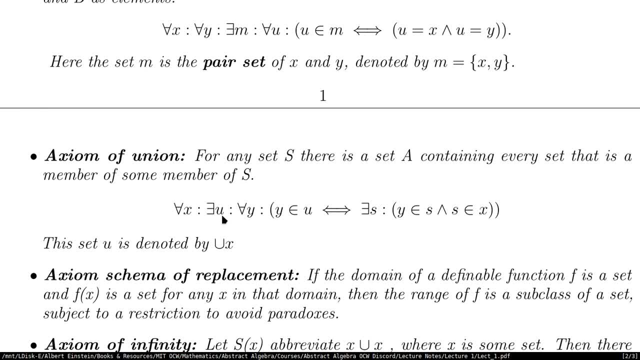 of X right. so this leads you to forming a chain of subsets, and what that means is that you are actually getting a set of set whose elements are subsets of some other sets, other set. so this set U is actually the union of all the X's right, and so that's the chain you're creating. 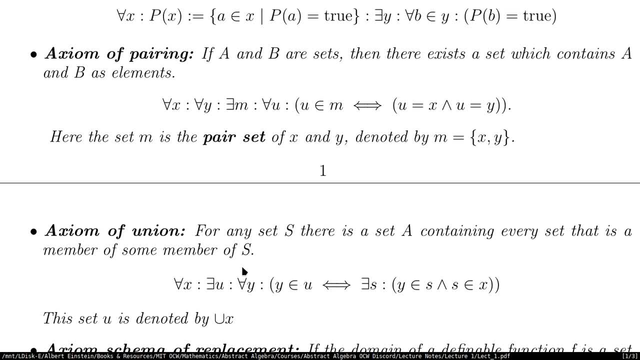 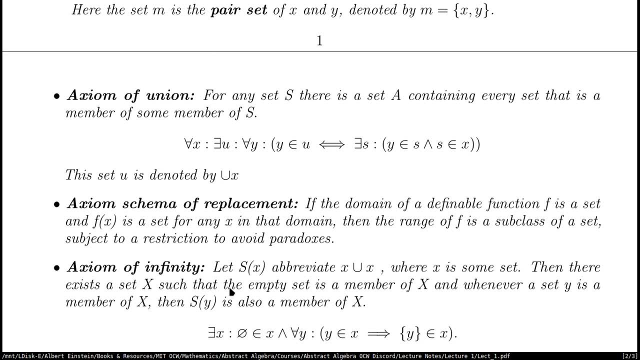 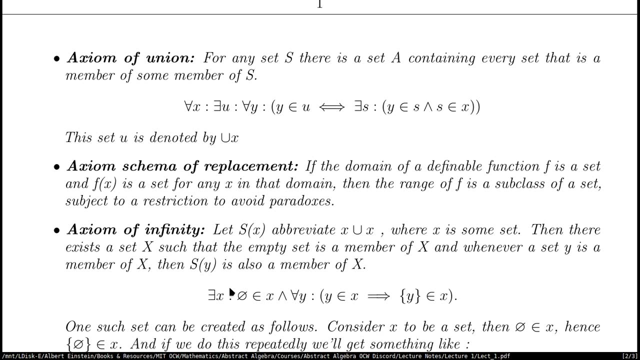 so I hope you've seen like this kind of notation before the cup and the inverted cup for intersection and everything. so you can see thateneralspl. Então vocêvіт essa. according examination, you have the axiom schema of you to change the absence of a subsection. 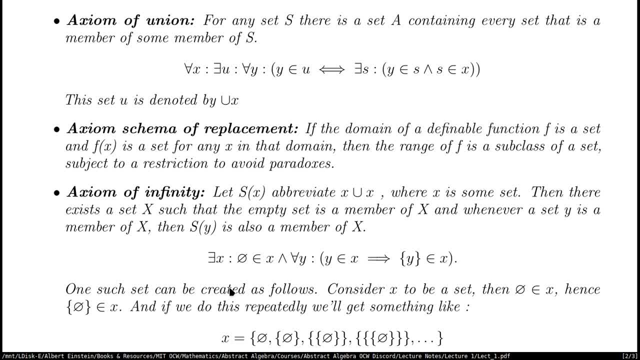 of the set that you got, actually going to you to say we got class, that the g affected had more value to the skills you had given each plot because you were basically不同 of F. you could say that. so this one says that if the domain of a definable function F is a set and F has to be set for any X in that, 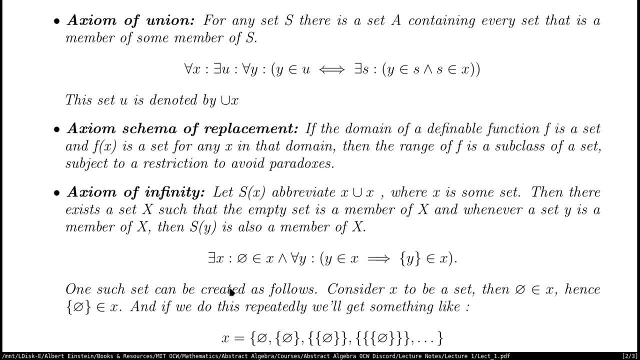 domain, then thisituated these chima, idAll, these92, which is subject to restriction. so this is kind of tricky because we haven't yet got to function, so we don't know what, how to actually like. think about functions, right, but, but the but the thing. 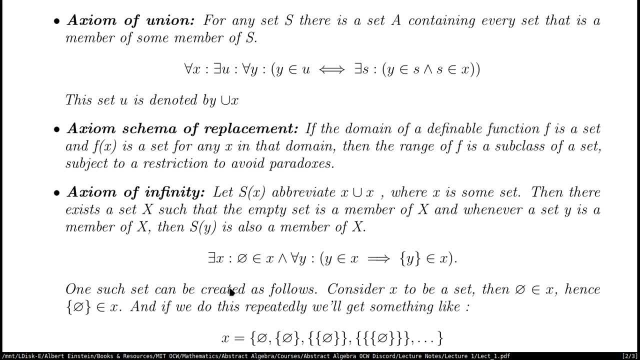 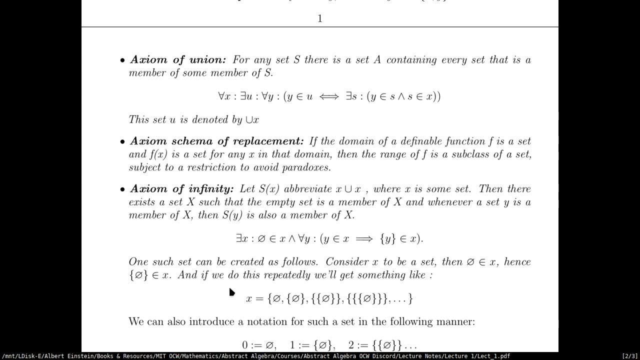 is, you don't really have to have a function. you can actually try to think about it in terms of relations, if you think, if you know relations, so yeah, we have to let this go as of now and we'll come back to this when we have gone to functions. but but the the idea of this. if you know what a 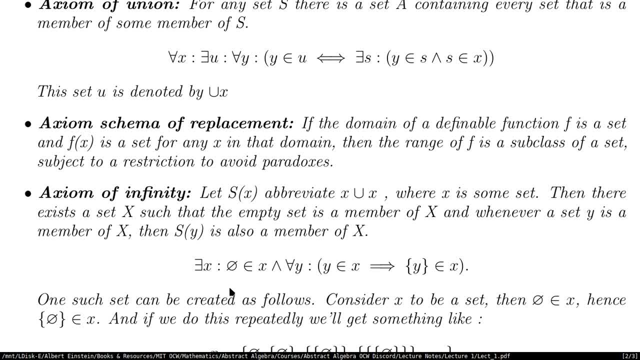 function is is that if you have a function which is definable, definable on a specific domain, then the image of that function is going to be a subset right of the codomain and when it's restricted it's perfectly definable. so so when you restrict, for example, if you have a function f going from a to b, f restricted. 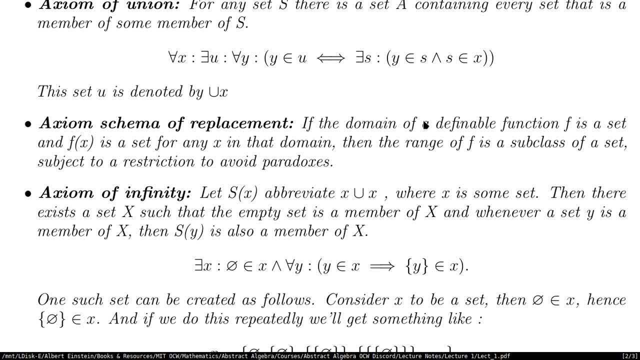 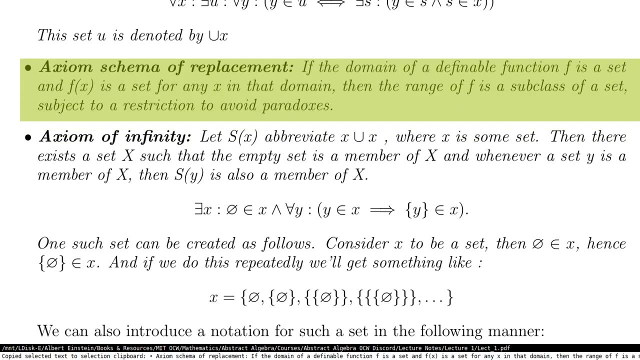 to a is going to be, is going to give you the image of a, and that's the schema of replacement. so f is the function of the kernel, so f is the function of the whole thing and f is going to be a part of the whole thing, right, so? so let me just go back to that and i'll leave this one here, because i'm a little. 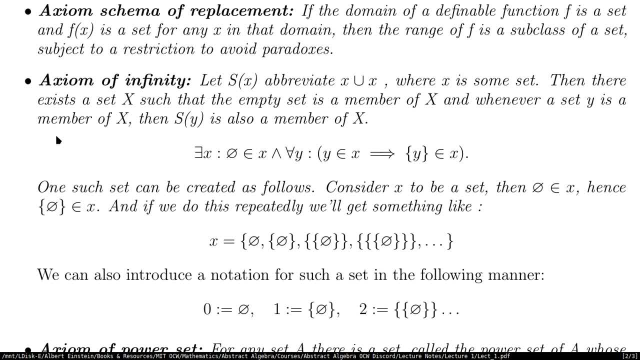 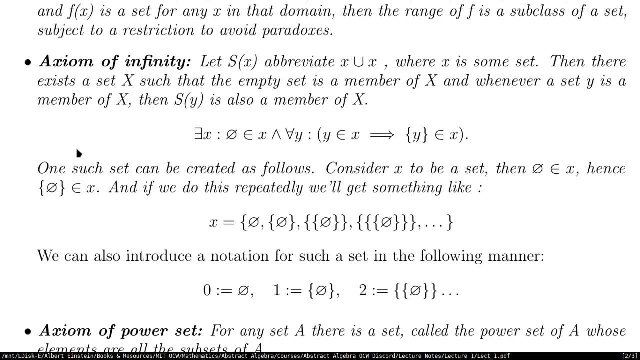 bit confused, right? so? so we have such a function that you can use in a very simple fashion, so let's just go ahead and just sort of go ahead and just go over this one- and we'll get into that later on- so so let's just sort of go ahead and check out some of the other functions that are in here. 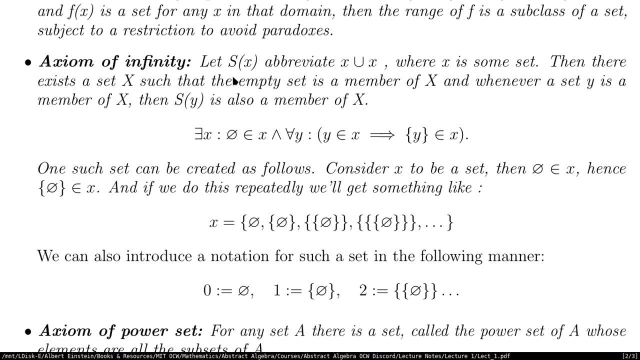 um, it's used a lot, but mostly you don't really use this act as an axiom, because it kind of comes along when you deal with functions. um, okay, so we have the axiom of infinity, which is kind of an important one. X, right. so S of X is a set which contains union of a set, X, with itself. so 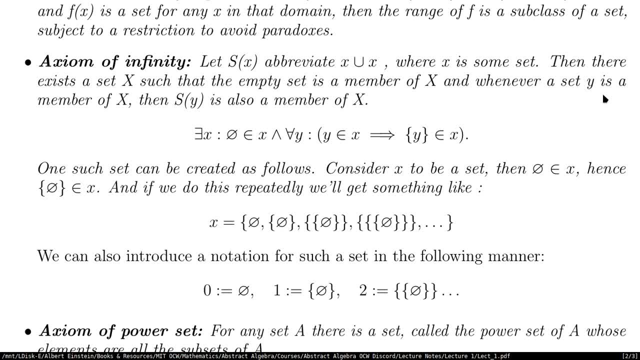 you're essentially making chains of the same sets. so there exists a set X, capital X, such that the empty set is a member of X and whenever a set Y is a member of X. so whenever you have another member of X, then S of Y is also member of X. so this: 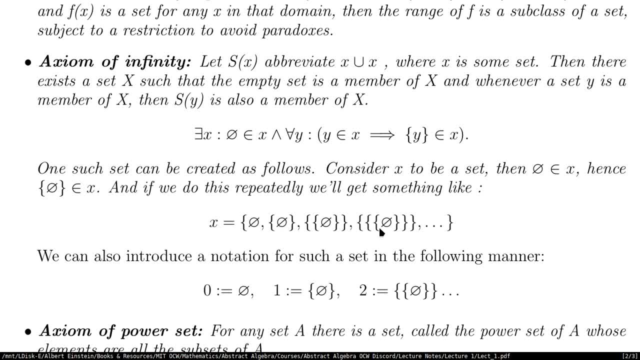 is just a tricky way of saying that you have a set X and empty set is included in that set, and so now we define this property. so this property says that whenever you have another member of X, S of Y, remember what is S of Y. S of Y is just Y, union, Y, so the chain of the same elements with the union. then 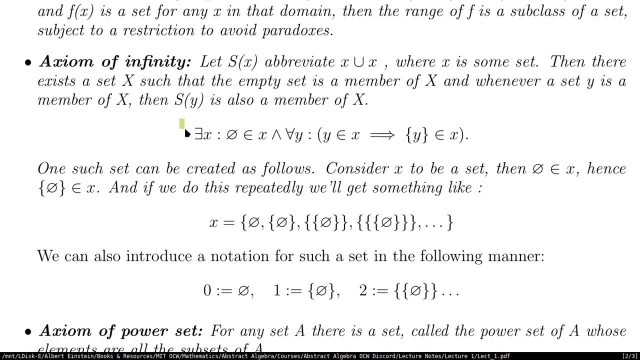 that is also included in the set. so this is what it says. there is such an X, such that that you have the null set in X and for all Y. if Y is an X, then that implies this is not how it's supposed to be. this is supposed to be S of Y actually, but yeah, S of Y is also an X or Y, union Y. so 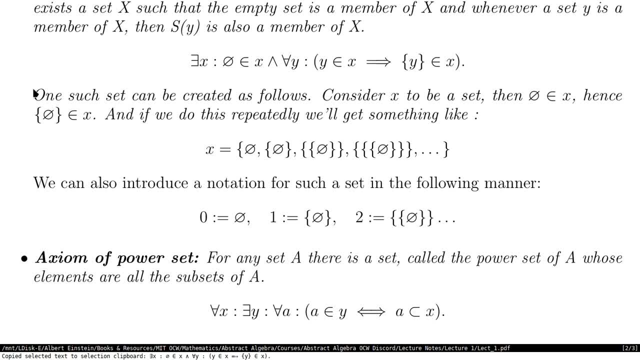 a very interesting example is how you do. this is if you have a set X and then you take again the null set to be in it, then this null set is an X, but this singleton right, so this set, including the null set, is also in X one. so what do you do, is you? 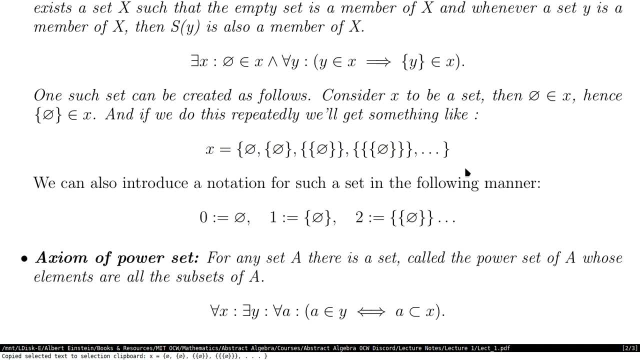 repeat this process. you repeat this process until eternity. you have the null set, then the set including the null set, then the set including the set including the null set, and you do this repeatedly and you have this chain and you have a new set and you can actually like a denote each of the the sets such that 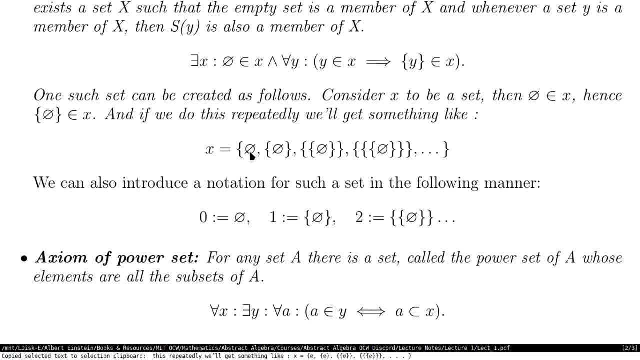 like this null set which, like, isn't included in it in any other sets it can be 0, then 1 is the singleton, then 2 is this set within itself. so like this, you can have the entire whole numbers actually. so yeah, that was the axiom of. 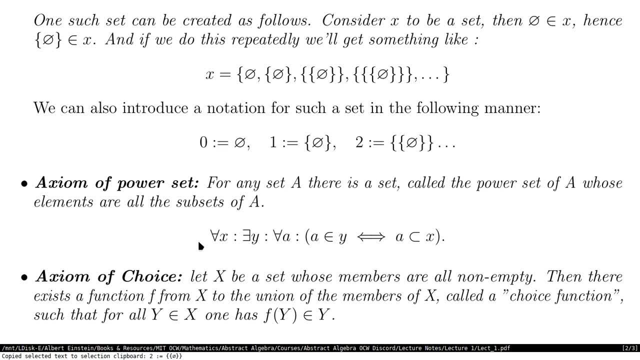 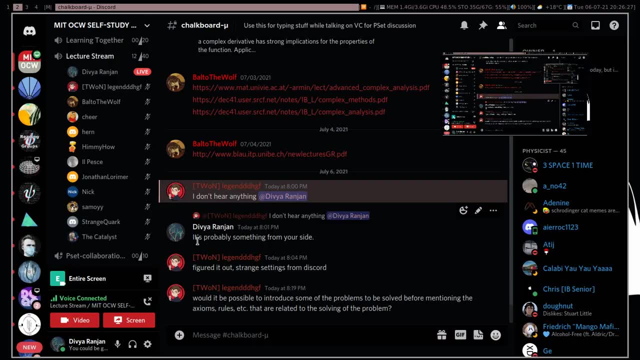 infinity. sorry, I think I someone just asked a question in the chat it. would it be possible to do some of the problems to be solved before mentioning the axiom is solving the problem? I'm not sure, but like are you asking? like, like some kind of problems that we should solve? 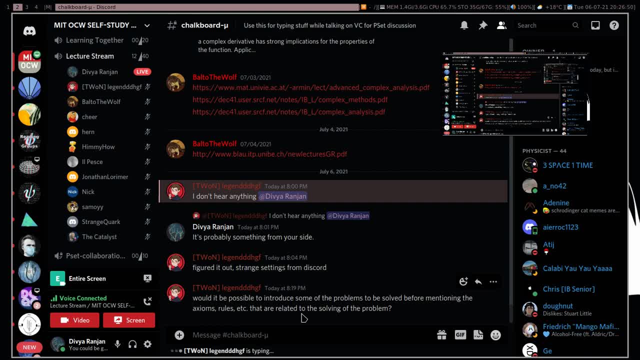 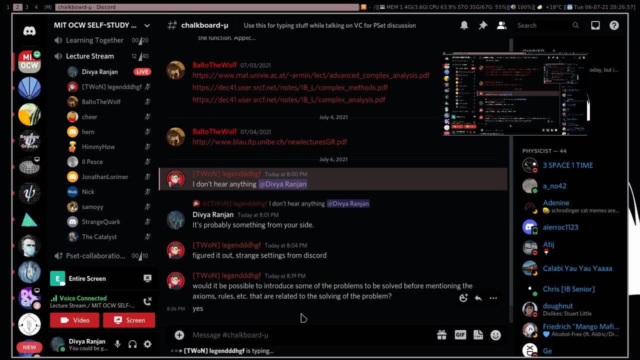 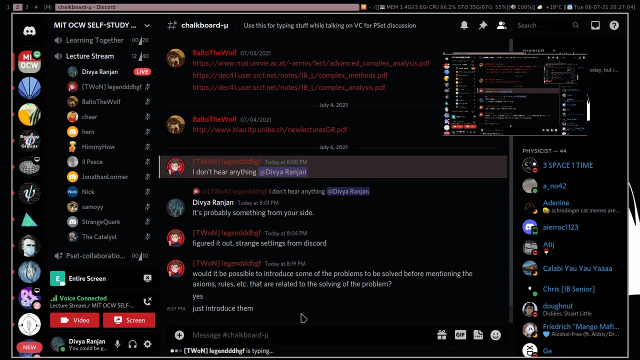 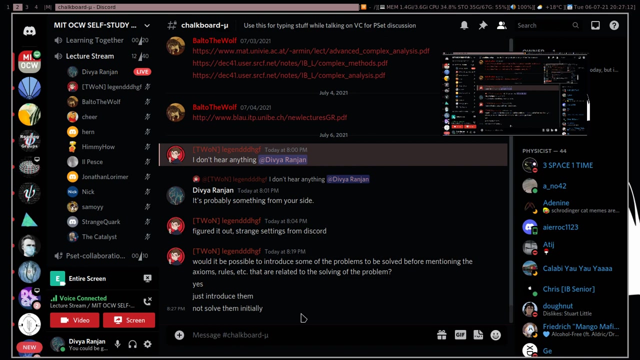 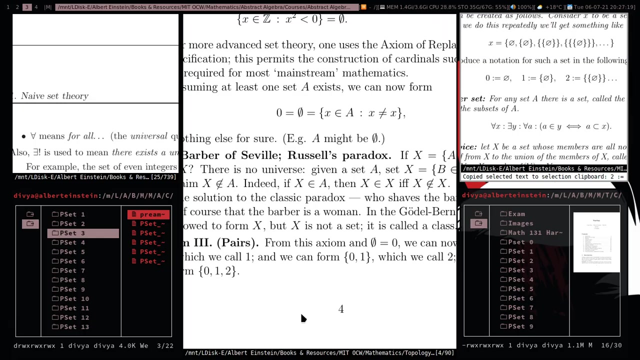 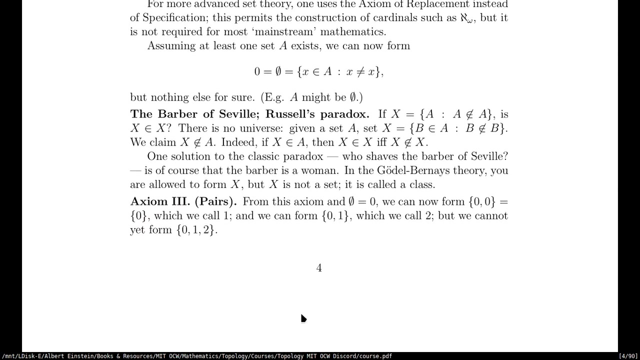 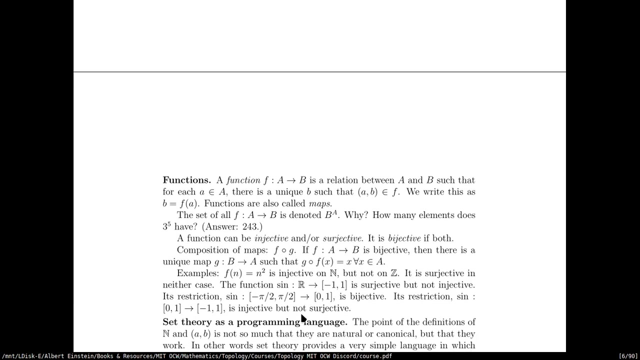 using the axioms. okay, that would be, that would be good, but the thing is, the thing is, when you try to prove things- okay, so essentially, examples now right, okay, okay, so that's a good idea, because are these axioms are pretty abstract, yeah, um, okay, I think I have a set of 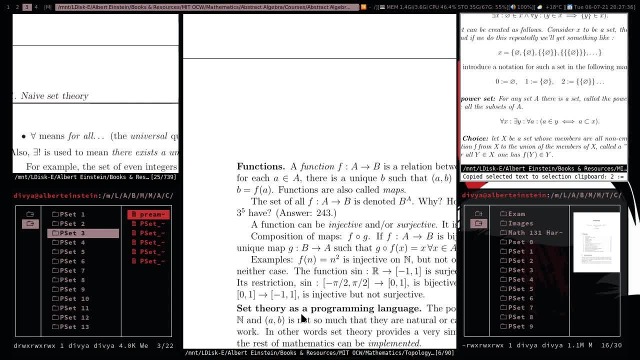 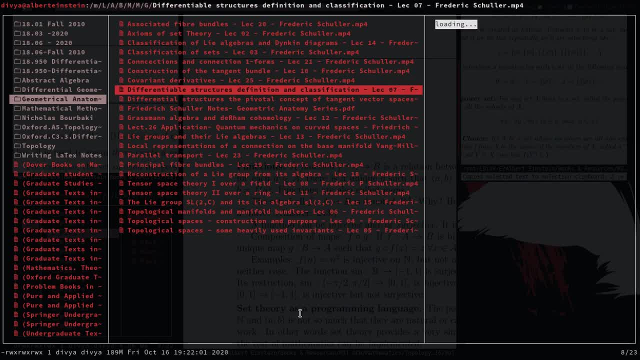 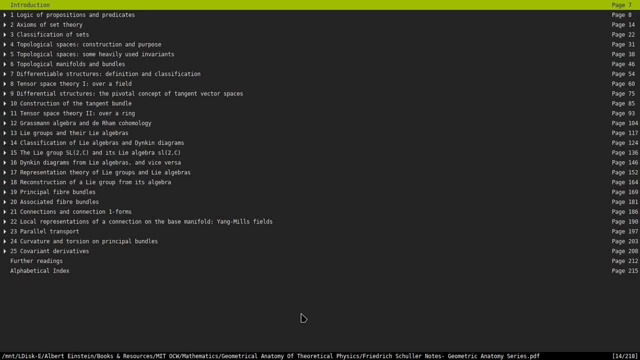 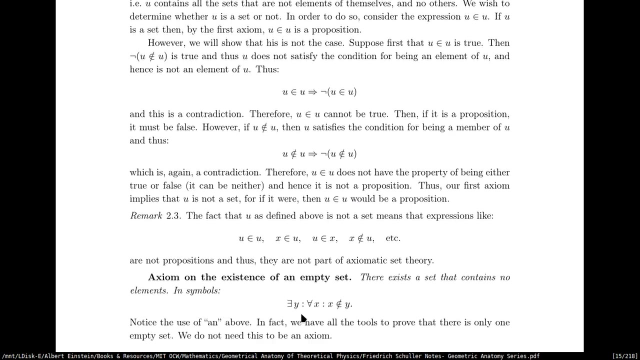 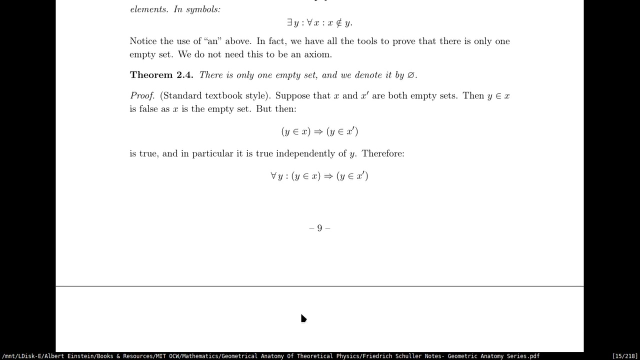 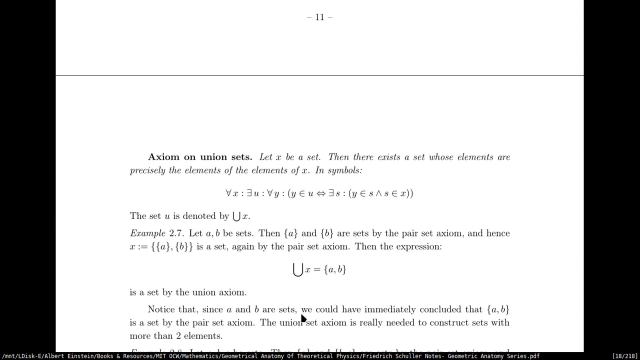 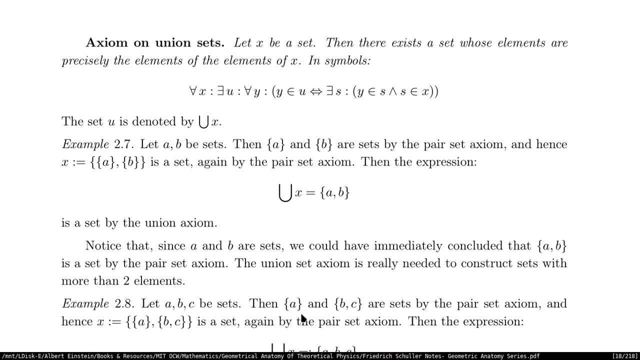 notes. which does that? let me get to- and I guess that's a good idea, we can do that right. so I believe this set of notes actually goes through each example. okay. so, for example, this: this is the axiom of union life. so here is an example: if you have A and B as sets, then these singletons containing just A and 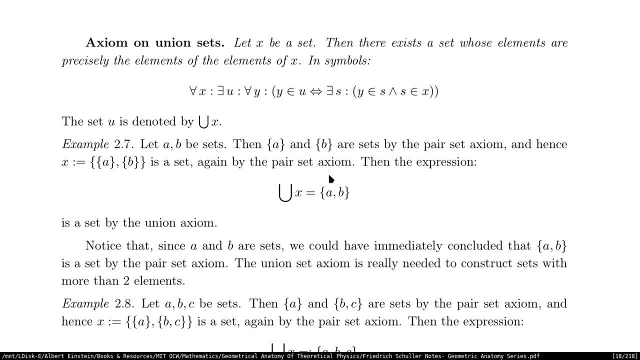 just B, are sets by the pair set axiom. yeah, and hence you can like have X which contains these singletons as elements for it, so that again is a, set again by the pair set axiom, you know, apply again. so then the expression, you know, this union of X, is going to be a. 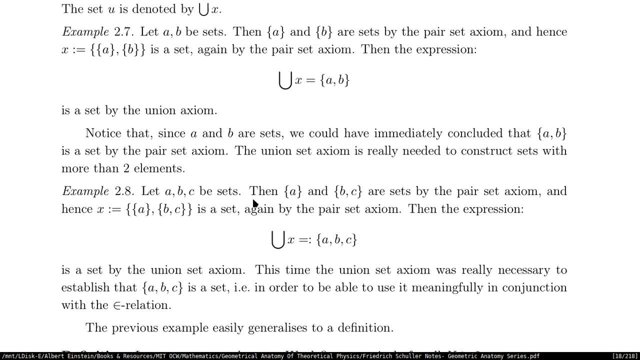 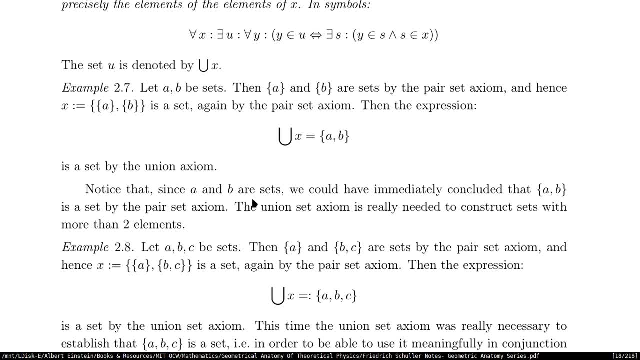 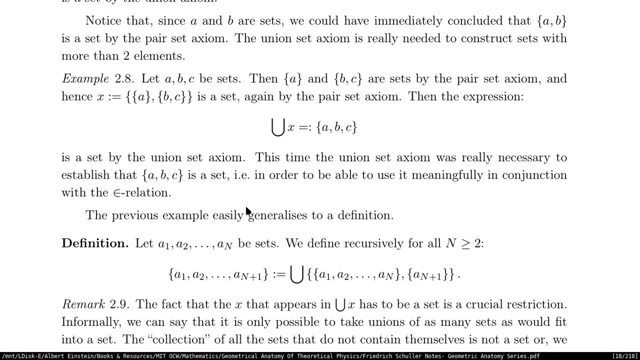 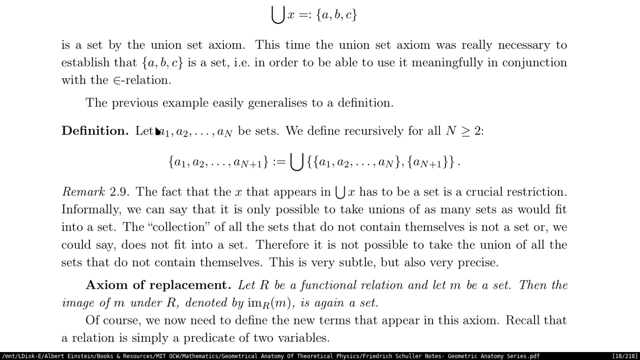 set again. so this is essentially. I mean, the examples are pretty much straightforward, or they're either straightforward or they need like a lot of axioms to conclude them, but you kind of try to repeatedly apply the axiom. this one is an interesting one, right? so if you have this, this n number of sets a1 to an, you can define. 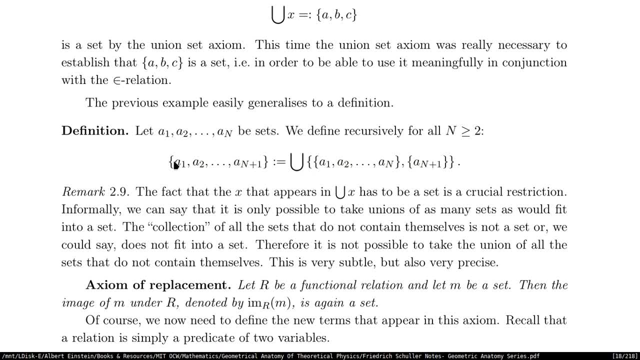 recursively and this kind of relation, so on. so we have this set containing all the n sets with n plus 1 as well. so this set can be defined as the union of this set with this set right? so this is how the union rules. you take two sets and then you can like pair them to make. 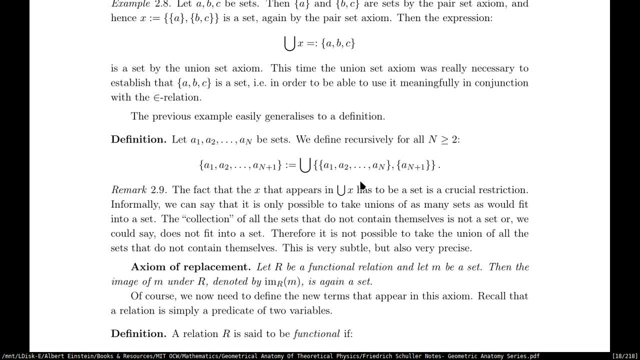 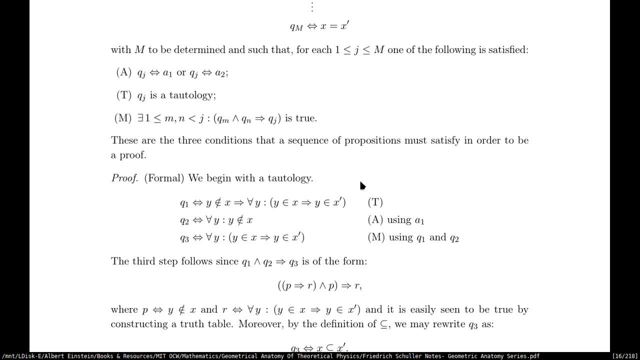 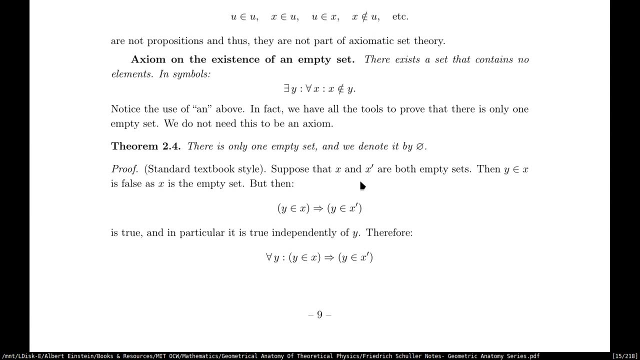 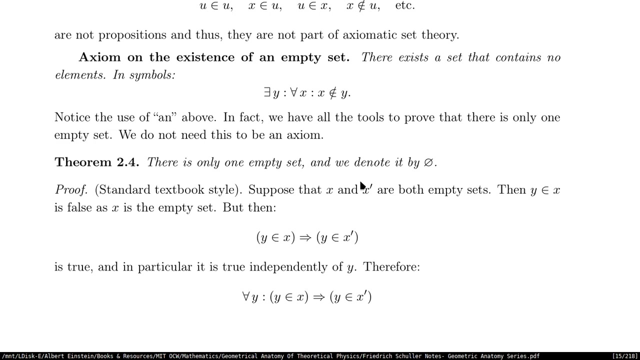 a bigger set. ok, that was for the union axiom, but if you look, look through these, you can't have examples for the most part, because using the examples needs further more axioms. right? for example, this theorem that I just told you, you know to practice. kind of think about that. there is only one empty set. this looks simple. 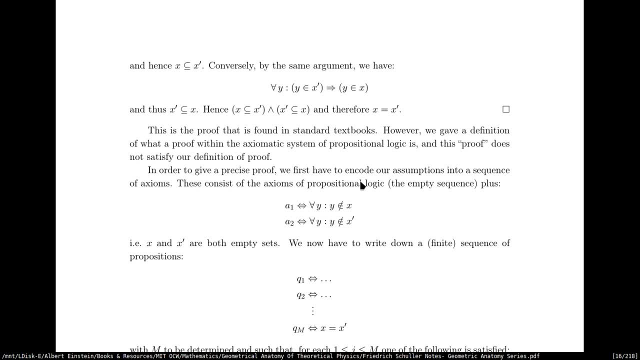 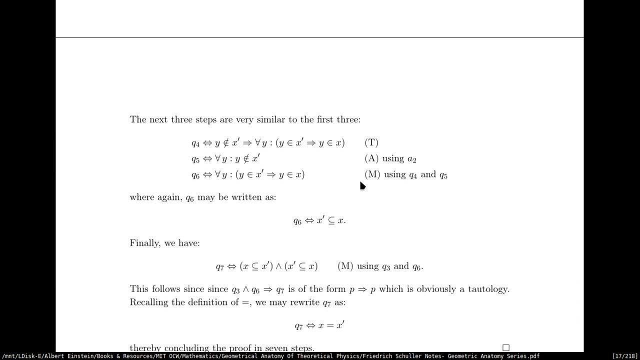 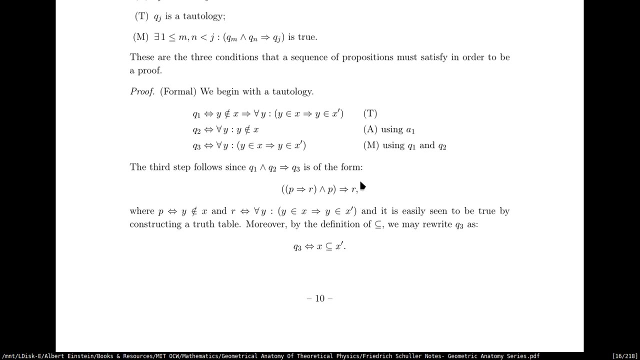 enough. but if you actually deductively go through each proposition and each following each axiom, it takes a long time. formally it's pretty long if you're trying to follow using the axiom. so that's why giving examples of axioms is kind of hard, because they are abstract, but yeah, 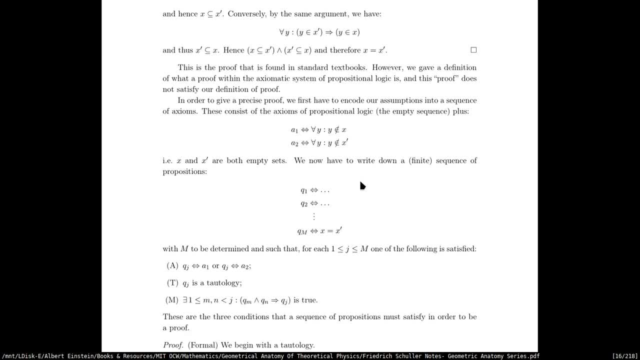 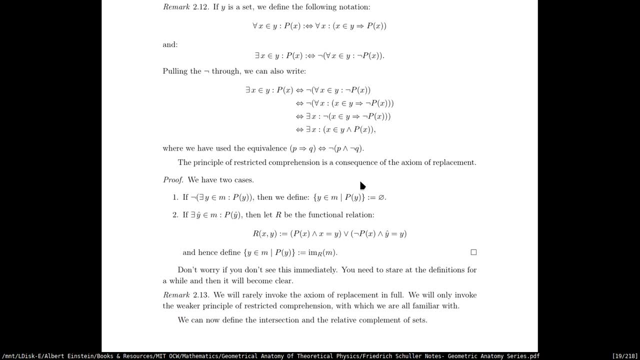 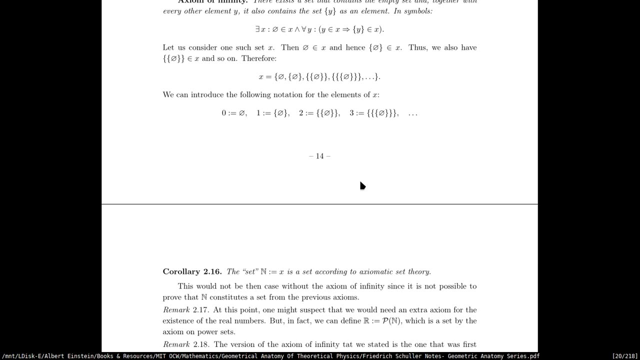 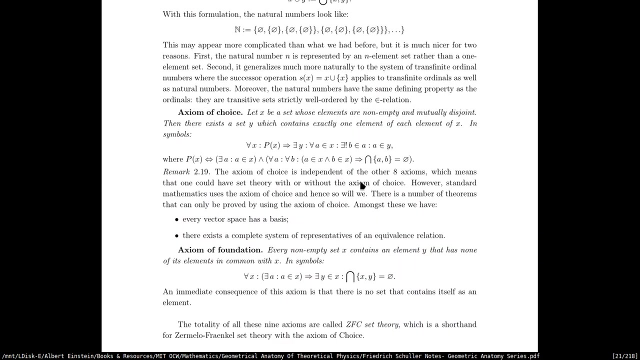 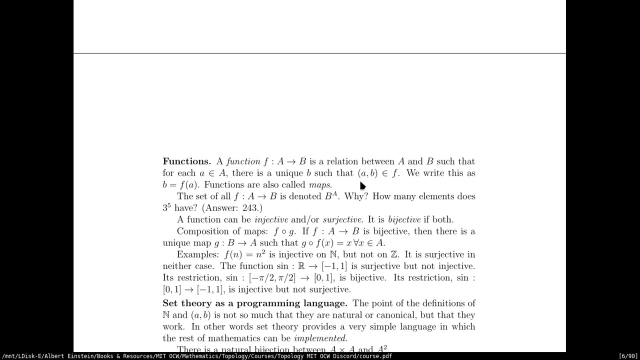 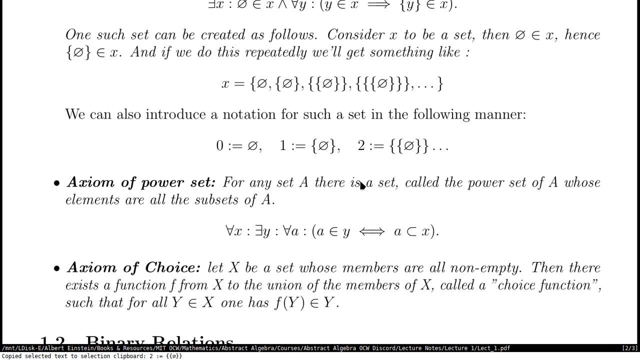 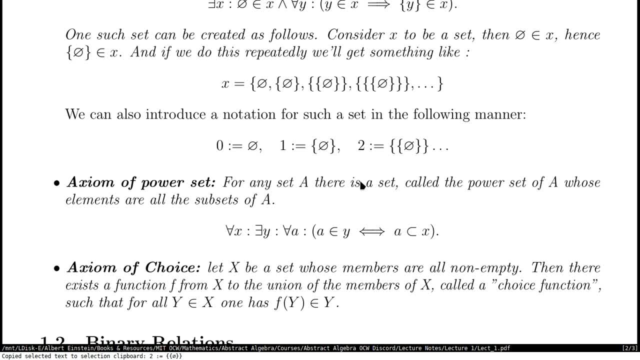 so we have the axiom of power set. so we have the axiom of power set, which says that for any set A, you have a set which is called the power set, whose elements are all the subsets of A. so this is directly from the axiom of pairing. if you have a set A, you have its subsets and you can pair each of those. 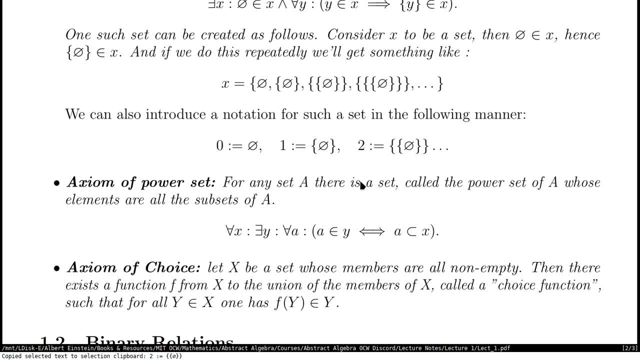 subsets with an each you know, you know each other, and then you can create bigger and bigger sets until you reach the biggest possible set, which is the power set. and if you have seen set theory before, for any set of n elements, the power set contains 2 to the n elements. 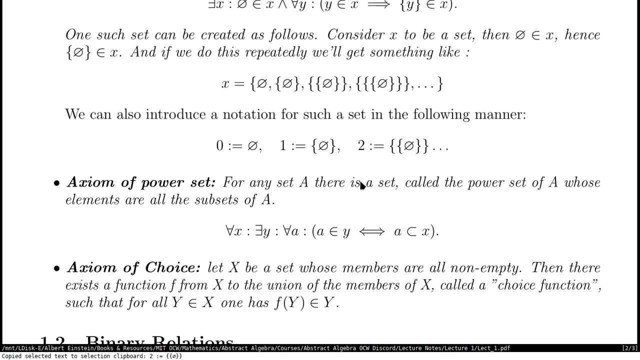 yeah, and that was the. the power set contains 2 to the n elements and that was the axiom of power set and it's it's almost always important because you're going to use power sets for everything. then the last one is the most controversial of axioms, the axiom of choice. some people like to include it, some people don't. 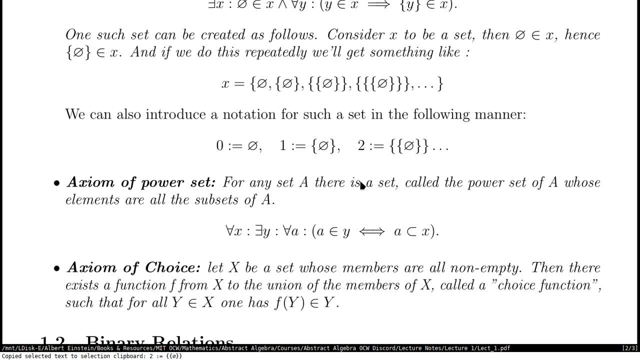 there's still a controversy. I don't want to get into the controversy, but the axiom of choice is this one. the other kind of incarnation of axiom of choice is the zones lemma. that's kind of complicated. we might meet it some. yeah, I think we'll meet it at. 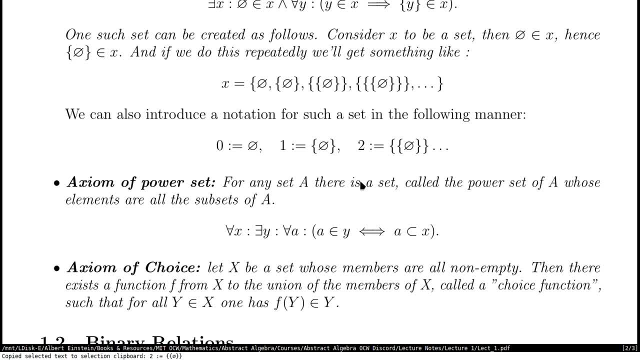 some point. but as of now, we can just go to the axiom of choice, which is that you have a set and all of its members are non-empty. right then, there exists a function, F, from X to the union of the members of X. so let's think about this. I'm going to show you an example of this. 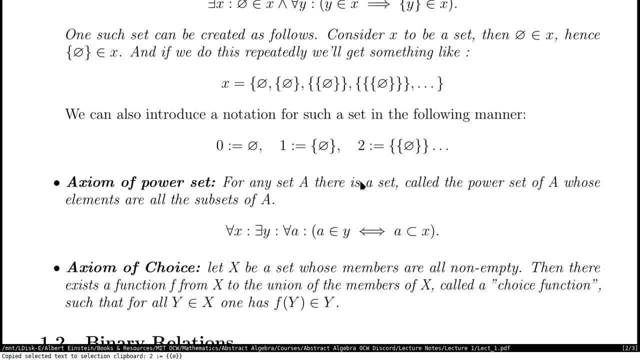 function F from X to the union of the members of X. so let's think about this. I'm going to show you an example of this. you have X and you have a function which takes you from X onto the, onto another set, where you have the union of the members of X and they're not the 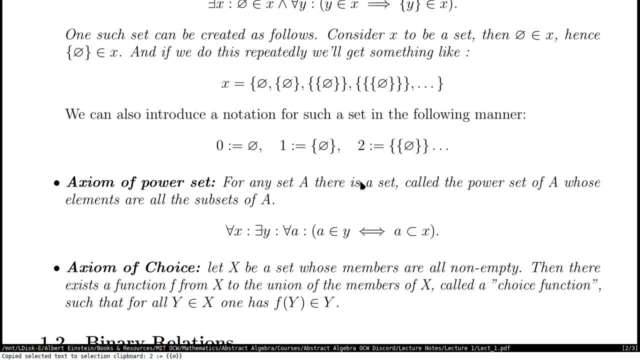 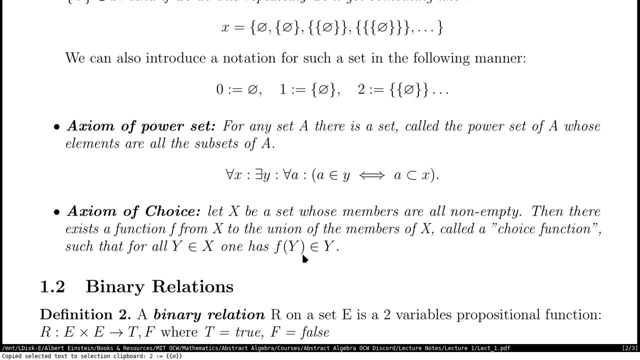 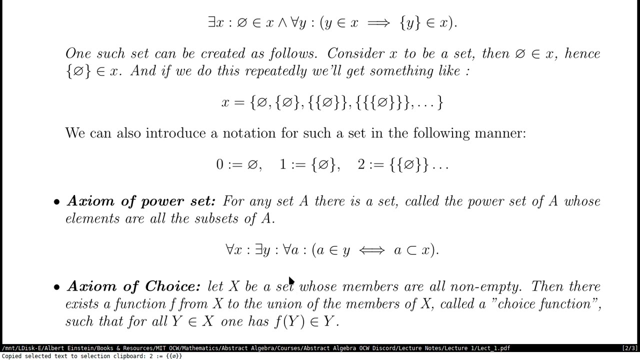 same thing, right? so this function is called the choice function. so what it lets you have is that for every member, Y in X, F of Y is also going to be in Y, right, and this sounds kind of like both trivial and paradoxical. but this is just like you have a set and you have another set. 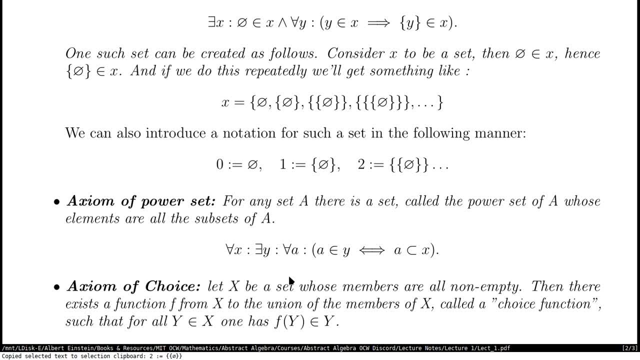 which contains the union of this elements, right? so if you have, let's say, the set X contain the elements A, B and C, then the other set which you're taking the function to is the union of set A with set B, with set C, so it's the union of the elements. so, with this function that lets you have is: 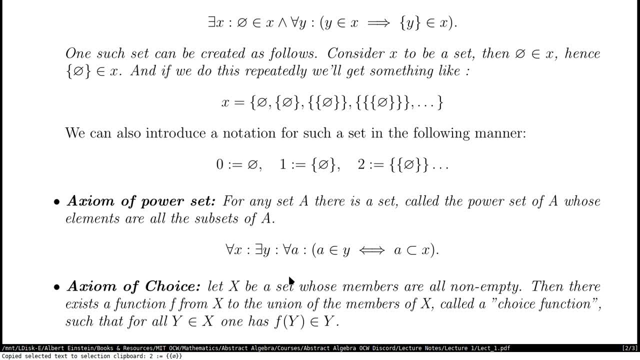 that if you're going from, let's say you pick one set in X, so let's say the set A containing the singleton A, so then F of A is going to be within A because again F goes from here to the union of elements. so you're actually going to 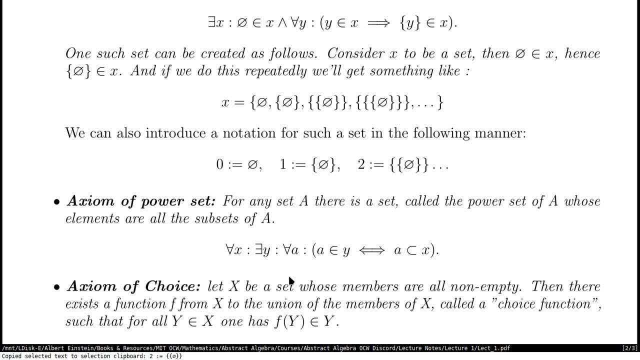 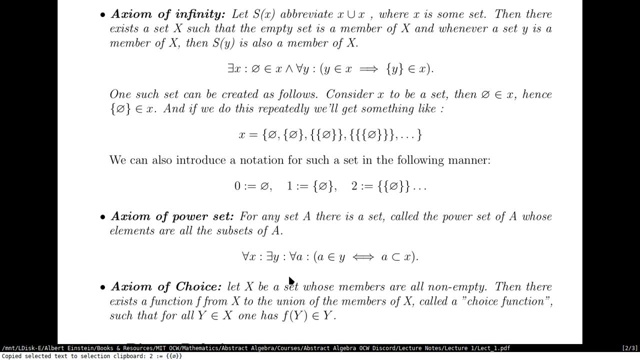 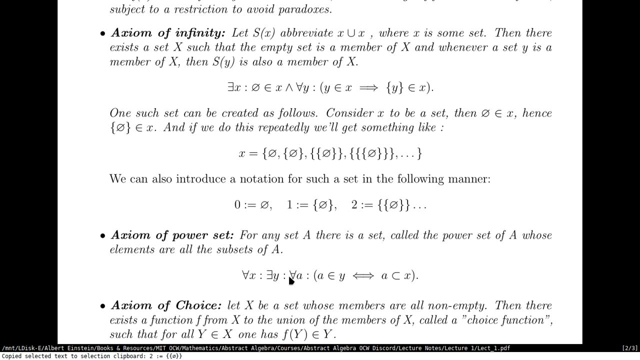 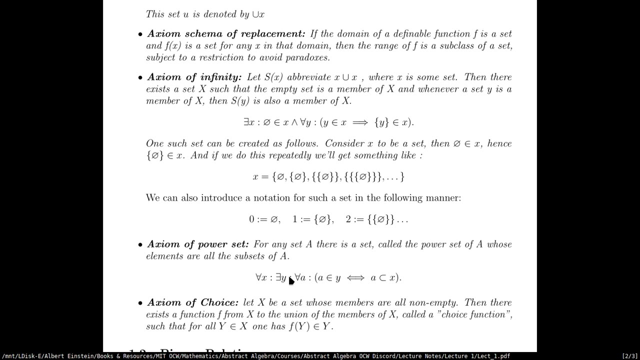 have a set of elements inside the set again, and so this kind of like, let's see, like give a choice in some manner to do this. we're not. we probably won't need much of it. we might- I'm not too sure, because we're like going to a lot of. 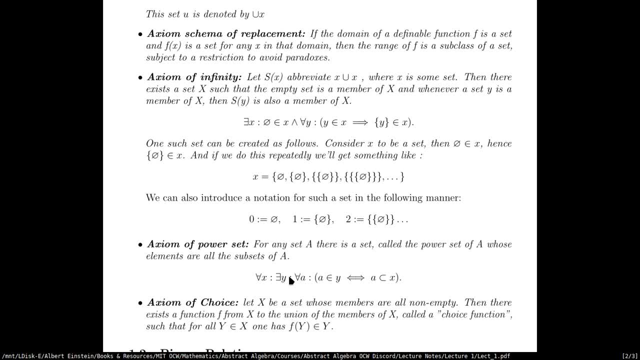 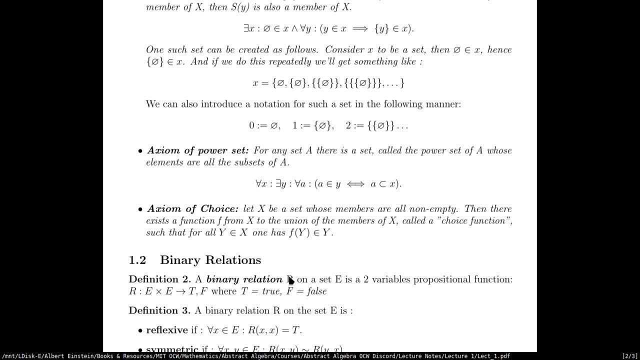 books. so some books don't like to be like no choice at all, but most people do, though. yeah, on chapter three of turns, Taos analysis, one for the axioms, and it was his paradox, yeah, I was talking to Balto the other day and he was saying: 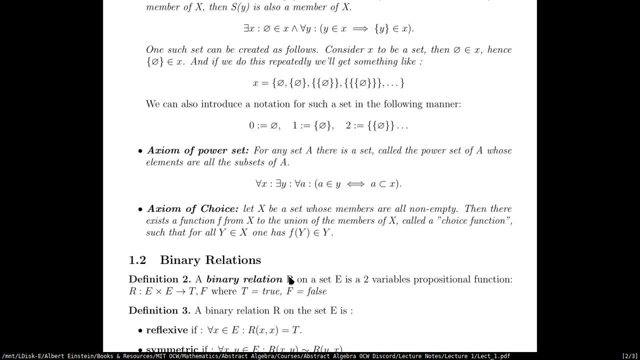 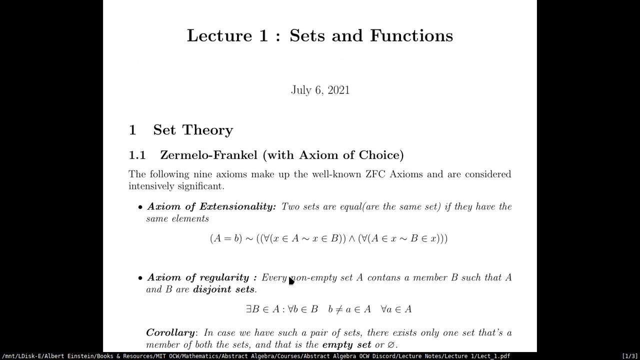 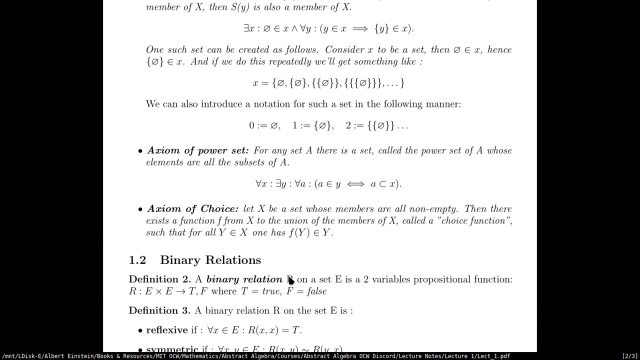 how the analysis by Tao is actually very, both like it starts from very basic and like does a good job at it. okay, so that was for the axioms. we covered it. the book doesn't cover it and the presets are not going to be using these, but these are actually very. 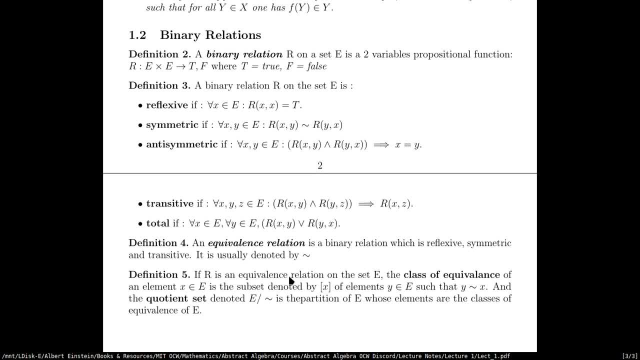 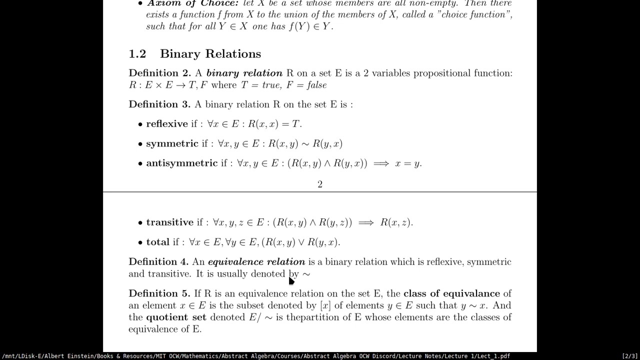 important. yeah, okay, so now we have this brief section on binary relations. the book also doesn't cover binary relations, I believe, but we're going to need that for defining what an equivalent solution is. so a binary relation on a set is a two variable propositional function. so what this does is it takes two elements, an. 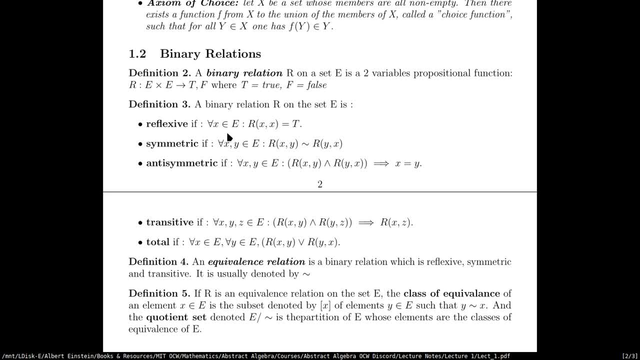 ordered pair of those elements and then it gives some propositional value about it. so either it's going to be true or it's going to be false, the relation between the elements that it pegs. so more precisely, if you have a binary relation R on the set E, then it has. 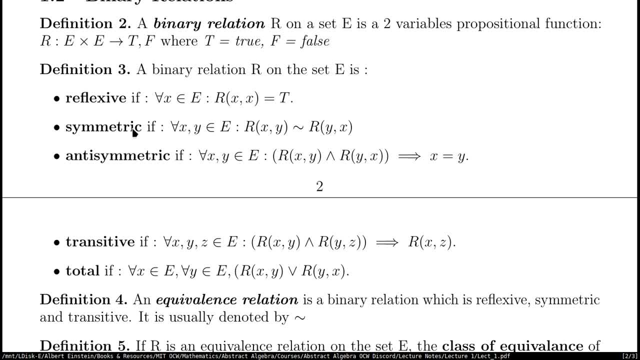 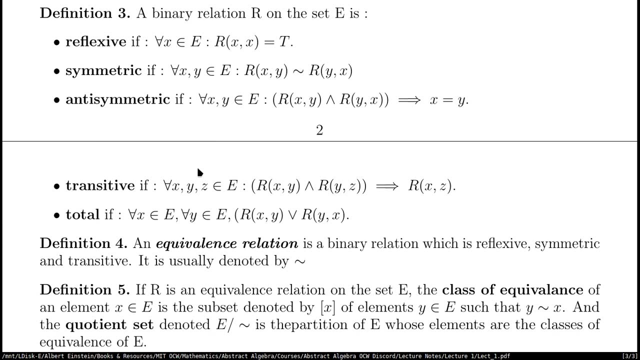 a bunch of properties, right? so if the binary relation satisfies this condition, then it's reflexive. so, okay, so we're going to go through these conditions. mostly, you would not need more than the first, second and the fourth one, because that's those are the ones that we need for. 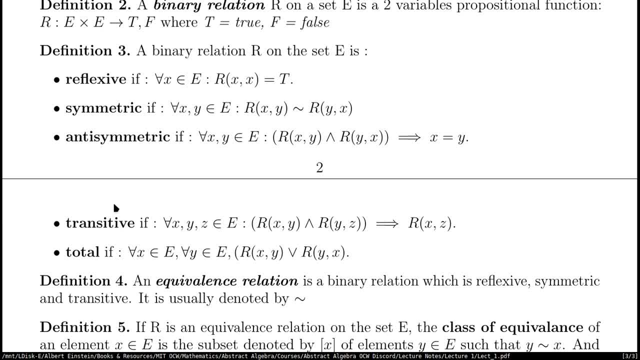 equation, but it's good to know the other ones as well. so, for reflexive properties, every element in E, when you apply the relation to it and then you use the pointer, you would do something similar to that. we were going to ask, but first we are going to go through. 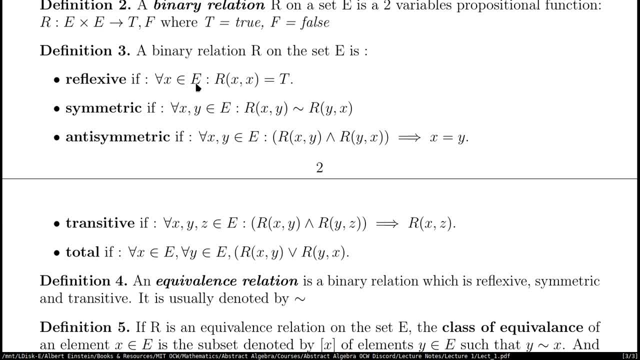 itself is true, the relation is true. so it gives you the true value. so r of x, comma x. so this is read as our relation of x with x, right? if you had y, it would be relation of x with y, and that's true. so that's when it's reflexive, right. so the symmetric 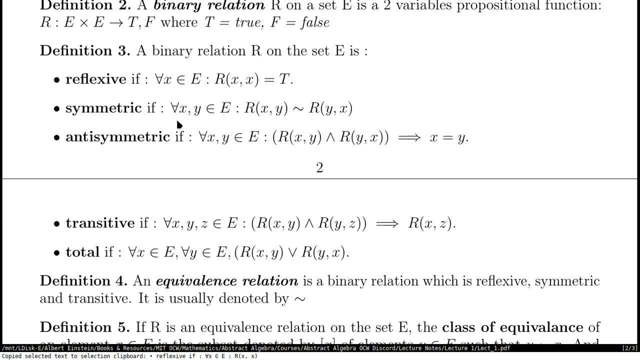 so the binary relation is symmetric if you take two elements of the set e and then you apply the relation to those two elements and then you reverse the order and the relation stays the same. so this says that r of x- y is equivalent to r of y- x, so the relation doesn't. 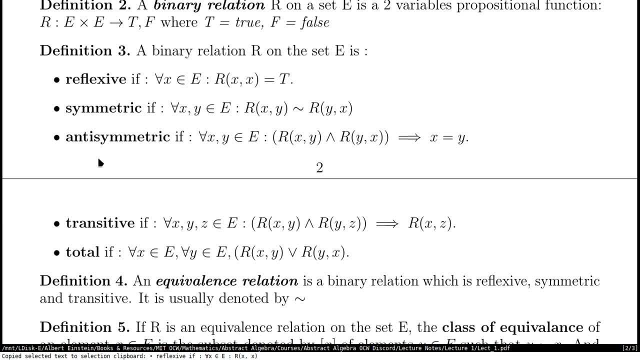 change when you change the order of the elements. so that's when it's symmetric, when it's anti-symmetric, it's symmetric, when it's anti-symmetric, exactly the opposite. right, you take the two elements. so if you have like r of x, y is like: 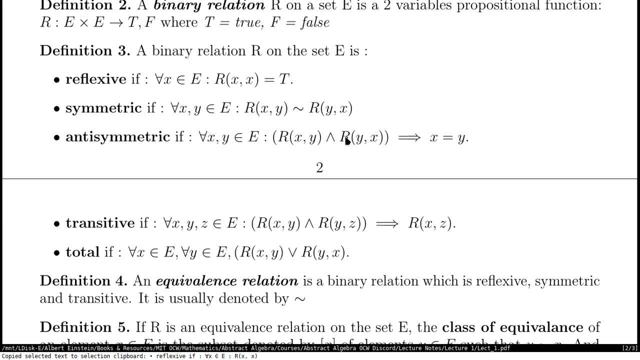 and r of y, x, if you like. if you take those two statements essentially- i mean, yeah, these are statements that, like the relationship is true, like if you have like both of them to be true, then that must imply that, like these elements are equivalent, like they're the same, um, uh, if that's like anti-symmetric. 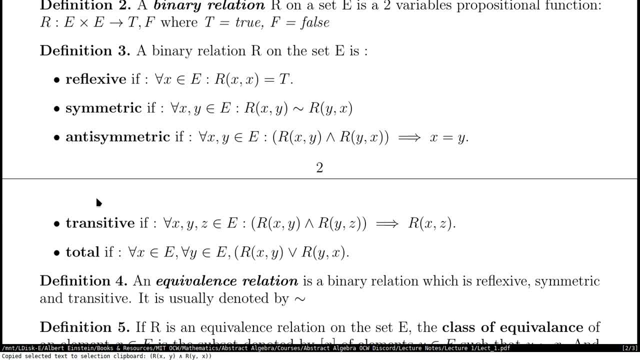 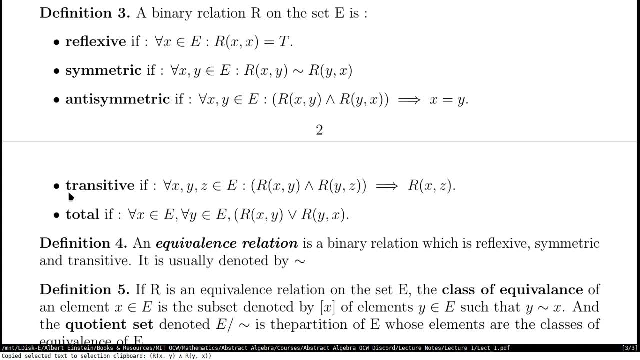 right. so that's uh, that's anti-symmetricity. so then you have um transitivity, so it's transitive. when you have like two, three elements, x, y and z, and uh, r x y with r y z implies that r x z holds right. so if you, if the relationship between x and y is like that, then you have: 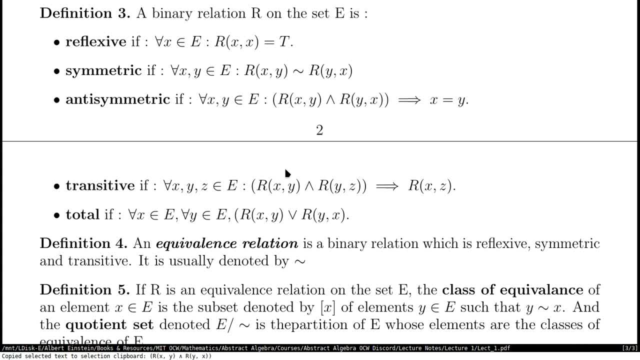 x and y holds and the relationship between y and z holds, then that implies that transitivity, that uh, the relationship between x and z holds right. so, yeah, that's transitivity and uh, binary relation is total. if, um, you have again x and y um, but for all x and y um, either r of x, y is true. 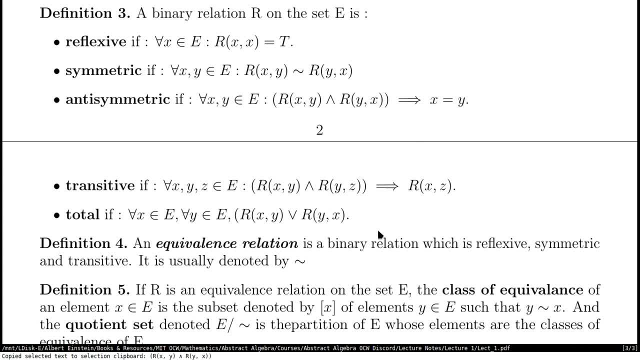 or r of y, x is true. so that's the answer to that question. so that's the answer to that question, is true? so they, both of them, cannot be true at the same time, right? so, um, um, it's kind of um like the anti-symmetric, that like if both of them are, uh like, true at the same. 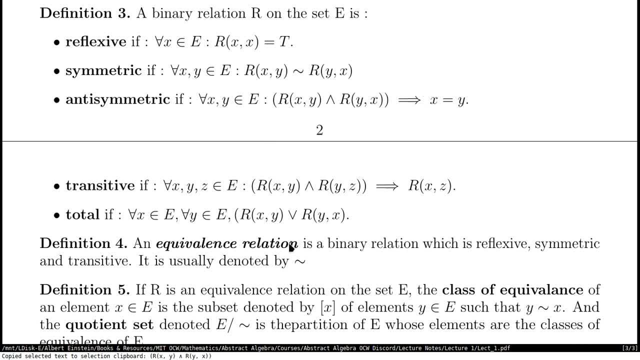 time, then that implies x is equal to y. but here you don't really have anything about x, y being equal. you just can't have uh, the relationship between uh- two elements in both the directions at the same time, right? so that is what a binary relation is. it gives you a relation between two elements. 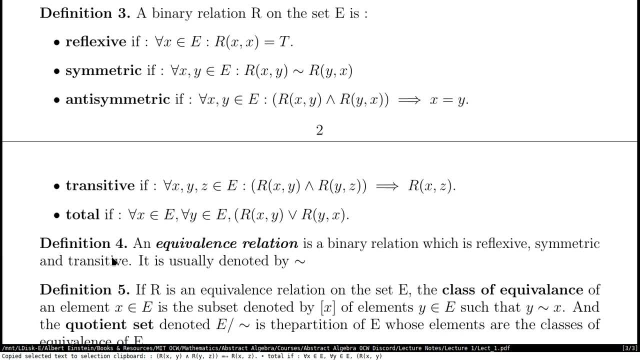 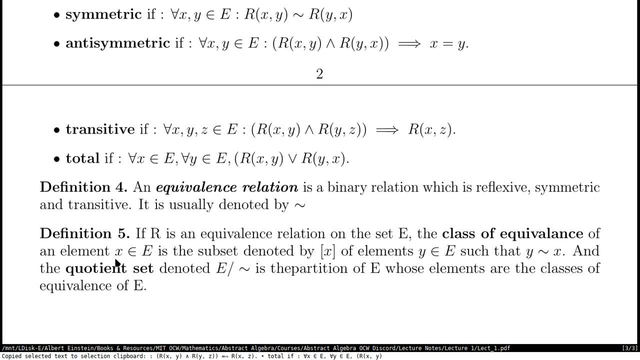 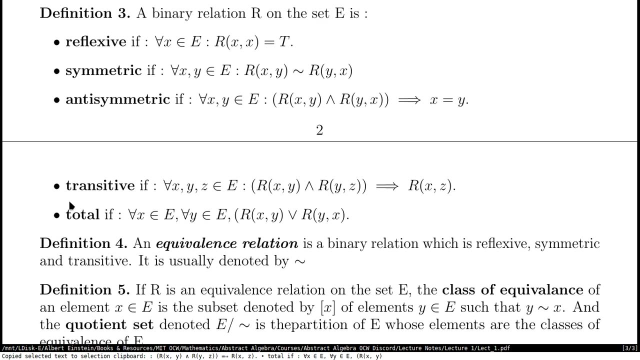 of a set, roughly speaking. so, uh, one of the special cases of, uh, what a binary relation is is, uh, this thing called the equivalence relation. so an equivalence relation is a binary relation which satisfies these three properties: it is reflexive, it is semantical and it is. 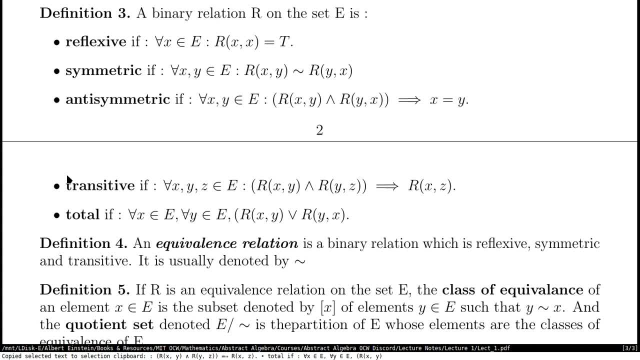 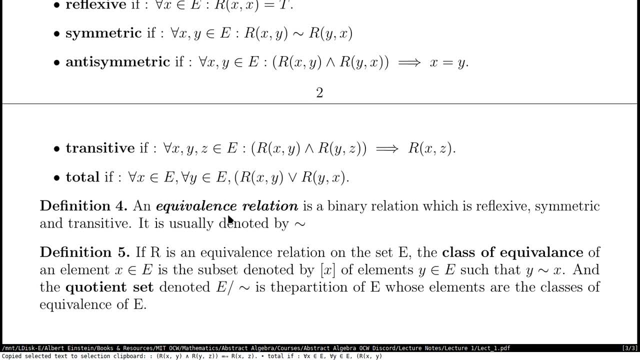 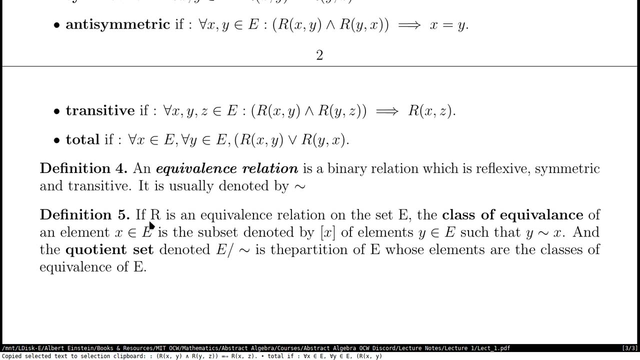 and it is transitive. so if you have these two properties, your binary relation is an equivalence relation and most often we're going to denote it with the tilde. so that's the equivalence relation. now, if R is an equivalence relation on the set E, then what you get is: is you get okay. so this is the from. 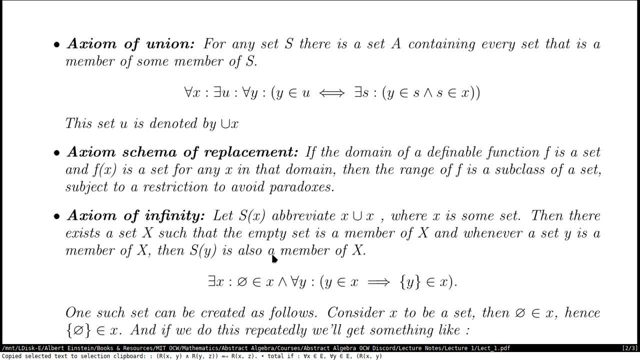 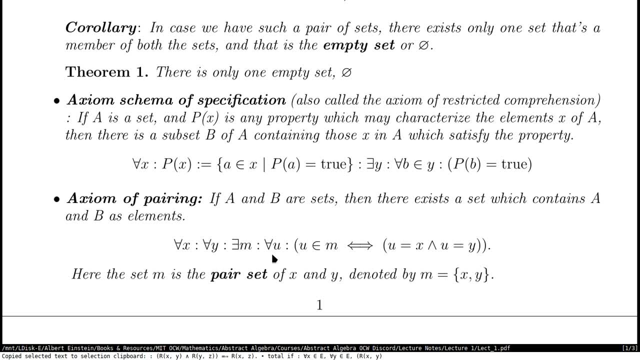 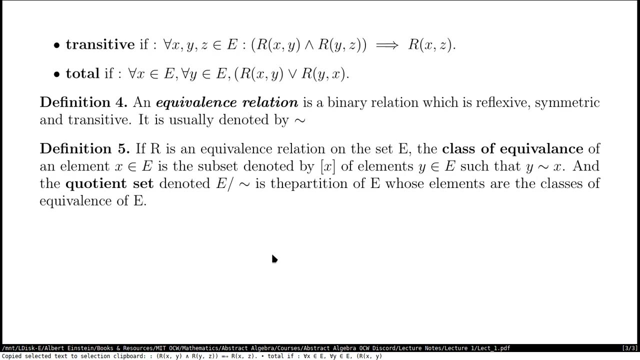 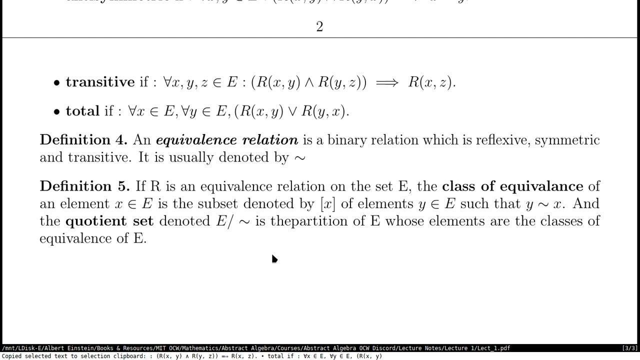 the axiom of it was the axiom of the property. one way specification, axiom, scheme of specification. yeah, restricted comprehension. so you have the equivalence relation. and now what the equivalence relation does is that it picks elements from the set E that satisfy the equivalence relation so they can be related using 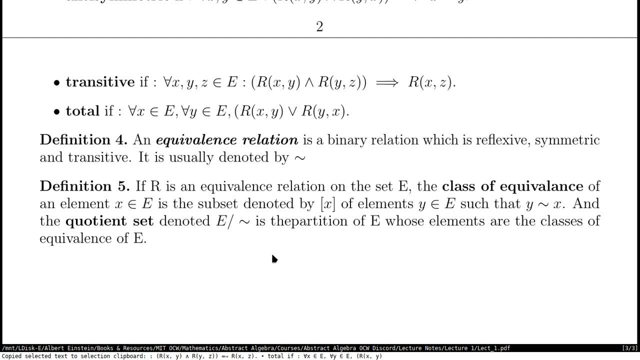 equivalence relation and then you create a subset of the set E which includes all the sets that satisfy the equivalence relation, and that is called a partition. we don't really talk about it here. we don't really talk about it here here. we don't really talk about it here. 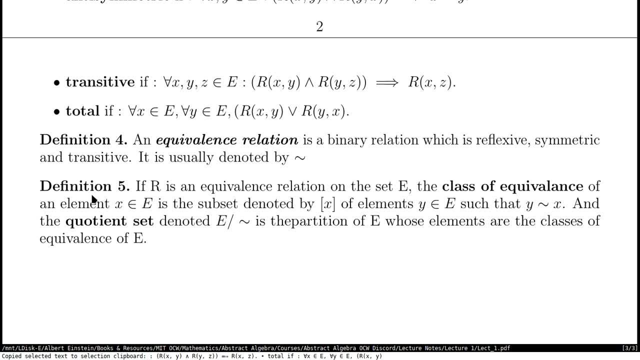 Yeah, but we're going to go back to all of these where I talk more about it. So if R is an equivalence solution on the set, the cost of equivalence of an element X is the subset denoted by X of elements Y in law E, such that Y and X have this equivalence solution. So they satisfy the equivalence solution. 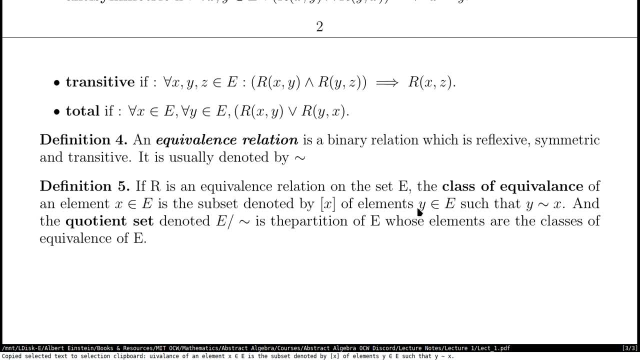 So for every element in the set you have an equivalence class. So the equivalence class is like all the elements. So, for example, if you have A, the equivalence class of A is like all the elements in the set with which you can pair up, with which you can have the equivalence solution. 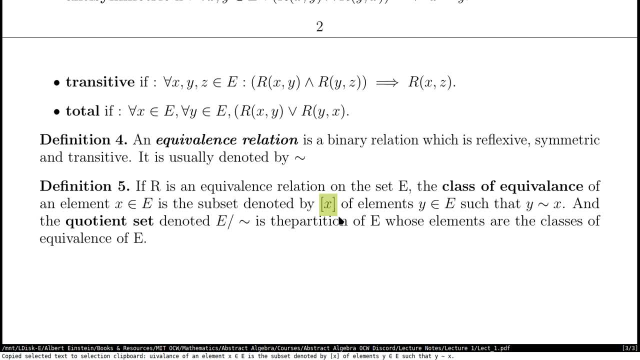 Right, So that is equivalence, And this is denoted by this symbol X within close brackets. And yeah, So that's the equivalence class, And this is very useful in pretty much every area, but one of the areas where it is something that I've seen a lot recently is in algebraic topology. 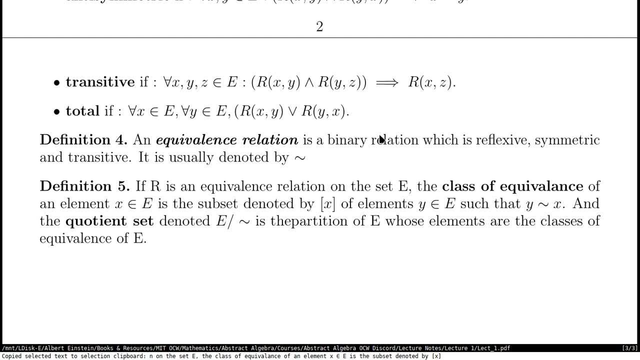 If you've seen anything in algebraic topology, we're always using equivalence classes, Right? But yeah, that's it. That's another story. So, apart from this, we also get a quotient set. So the quotient set is actually the partition I was talking about, Right? 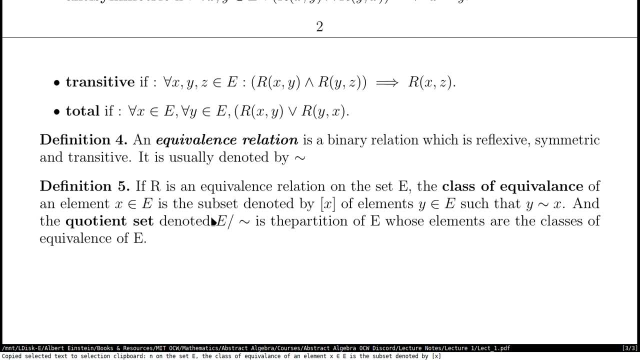 So the quotient set is the set E and slash this tilde, So this notation kind of you can think about it kind of like division. If you've done modular arithmetic before, you know about modulus Mod, But if you haven't, then this is like you have the set E and then on the set E you impose this specific relation on the entire set. 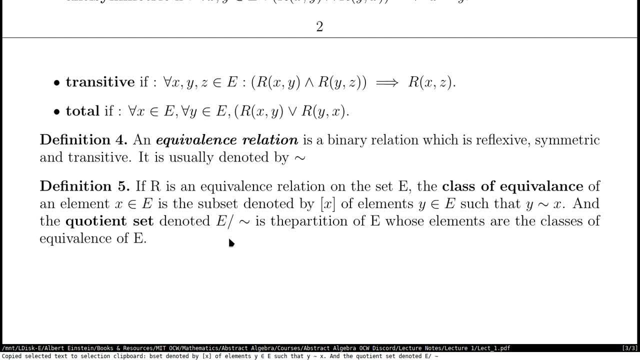 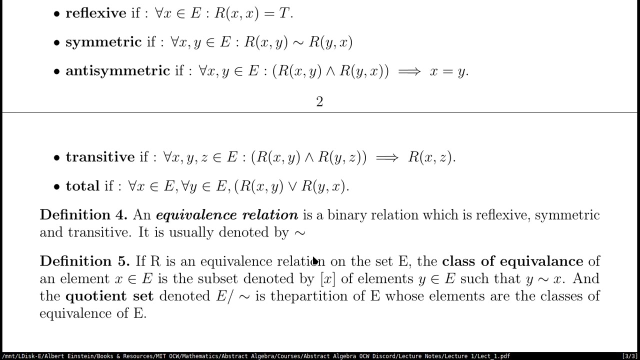 And when you do it you get a subset of it which is the partition, and then that is actually the quotient set. So this is E slash tilde. We're going to use this extensively Because this is kind of like one of the fundamental things with which we can do a lot of things. 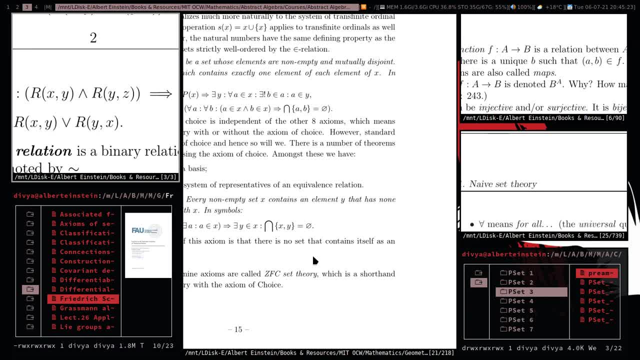 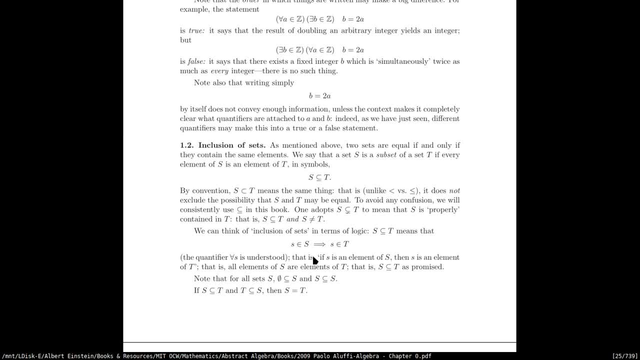 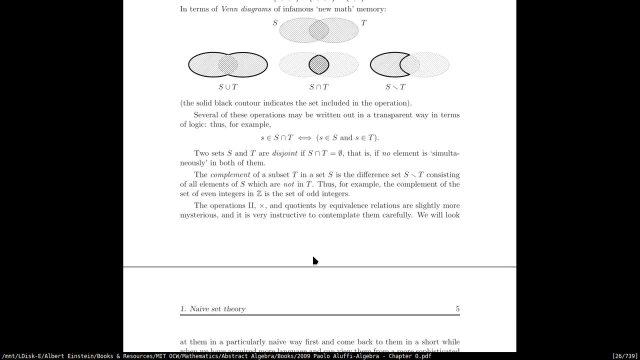 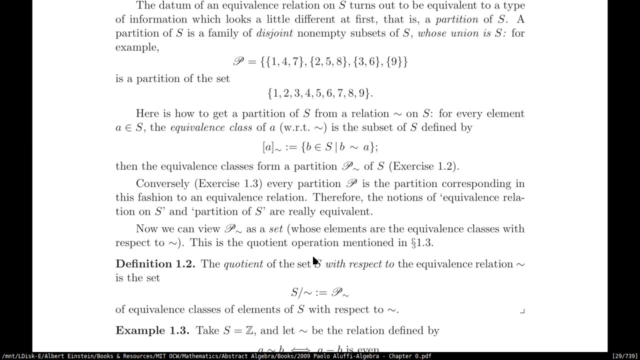 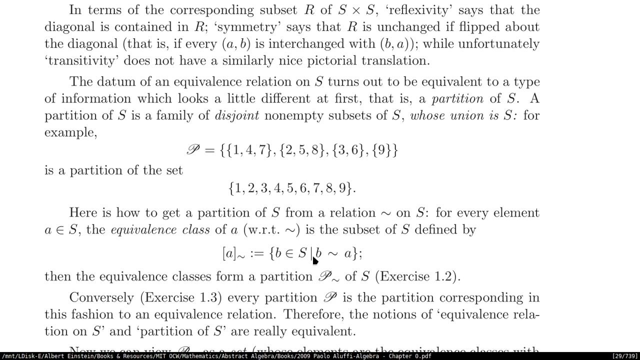 So that was about equivalence relations. So now let's get back to the book. Okay, So yeah, The book contains a few examples. We should go through these examples to get the idea of equivalence relations clear, Right, So yeah. 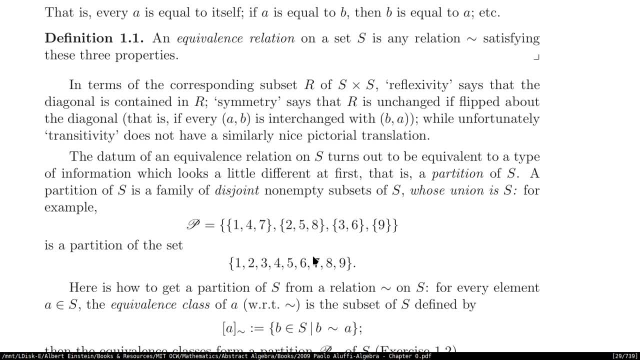 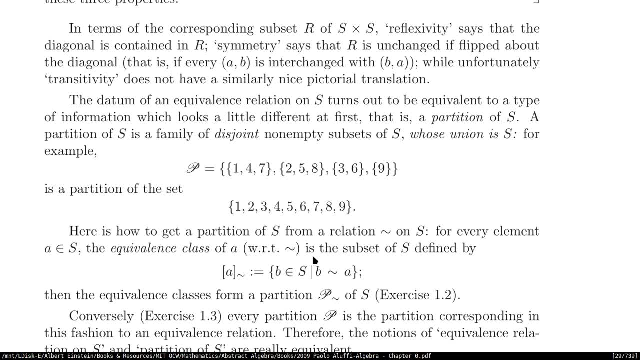 And the idea about partitions in general. Okay, So, yeah, So here we have a more descriptive definition of partition. So partition of S is the family of disjoints, Non-empty subsets of S whose union is S Right. 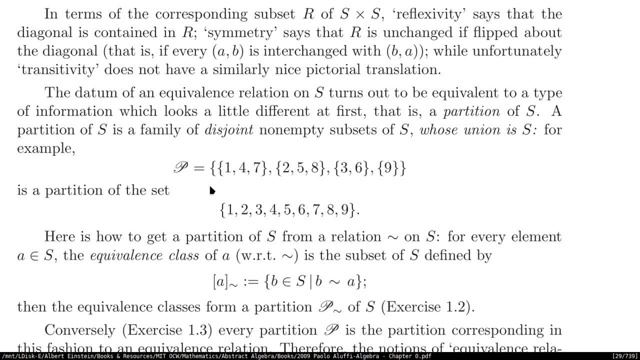 So a partition, as I said, is like the set you get after applying the equivalence relation, So it kind of like divides the set into partitions according to the rule that the equivalence relation follows. So let's see, You have the curly P here, which is a partition. 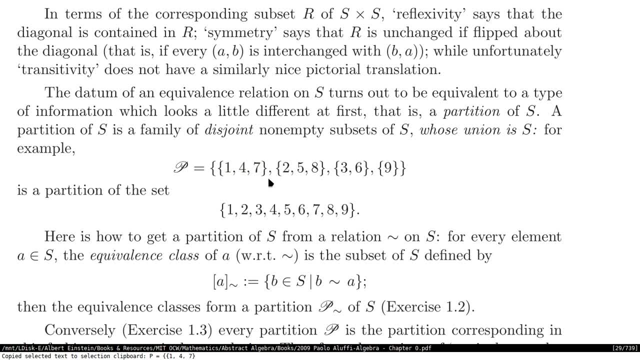 So it contains this set of 1,, 4,, 7,, 2,, 5,, 8,, 3,, 6, and 9.. So it is a set containing four sets Right, So it's a partition. 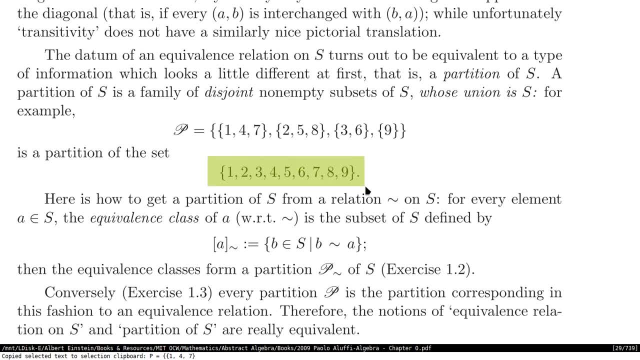 So it's a partition of this set which contains nine elements, the nine numbers. So how you get from this set to this is by By applying an equivalence relation which picks these numbers Right, These numbers, and partitions them into each set. 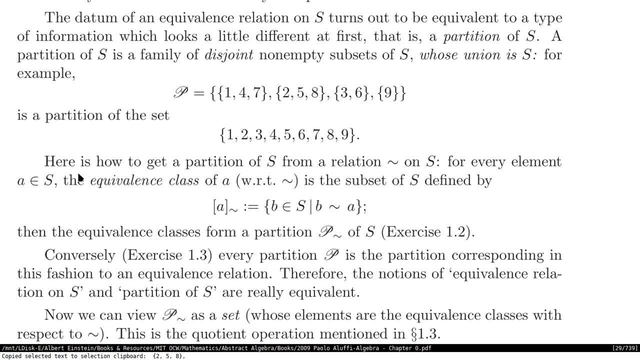 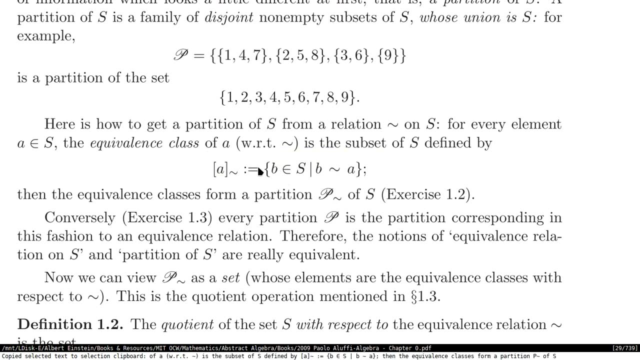 So here's how you actually get it. So, for every element A- yeah, we just talked about it- The equivalence class of A with respect to this relation. If the subset So, is that like The subset containing all the Bs which are definable under the equivalence relation with A? 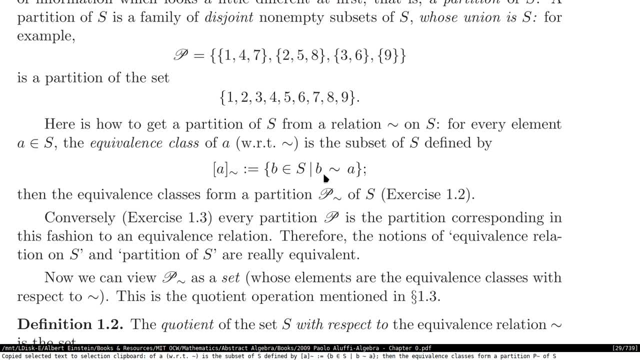 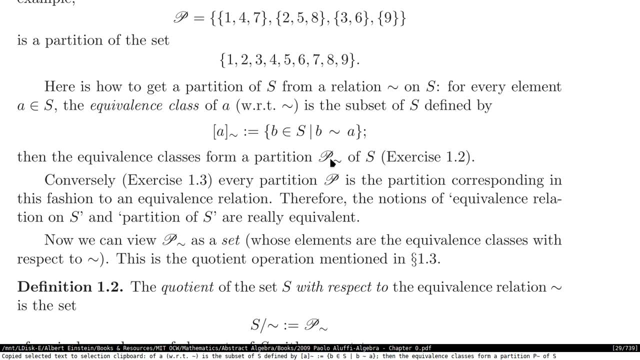 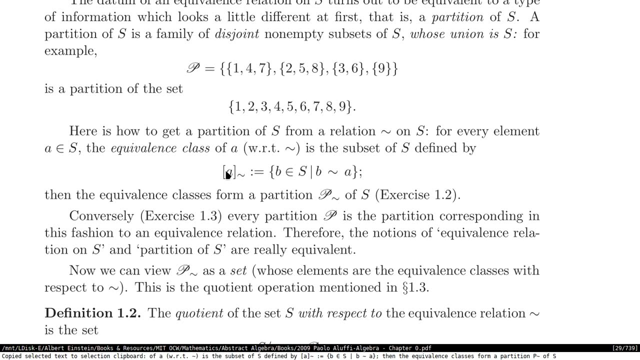 So all the partners of A, in a sense, for this relation. So then the equivalence classes form a partition of P, total of S. So what you have is that these equivalence classes are defined for each element Right. So for each element you can get these kind of sets. 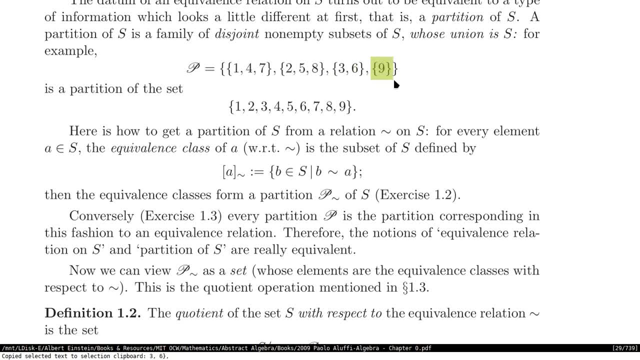 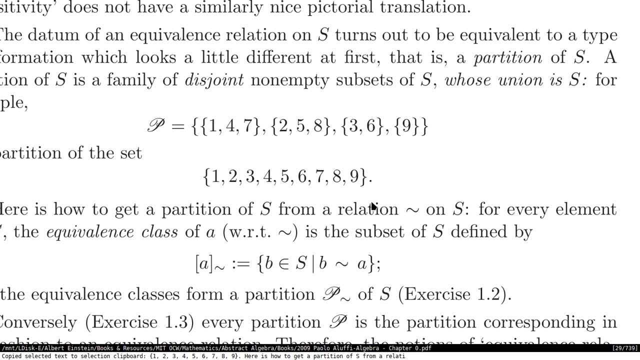 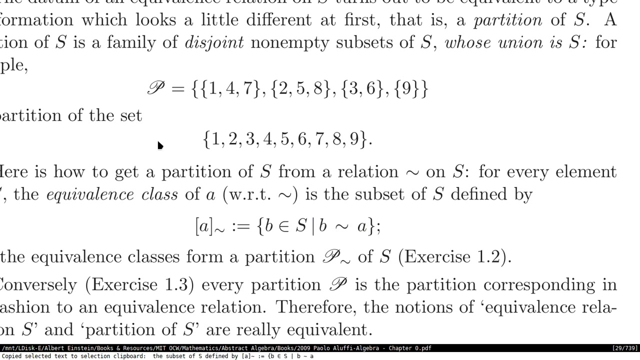 Right. So you get these kind of sets. For example, let's see here On this set we define some kind of equivalence relation tilde Such that we identify. So this is also set as identify. So this can be read as B tilde. A is read as B identified with A. 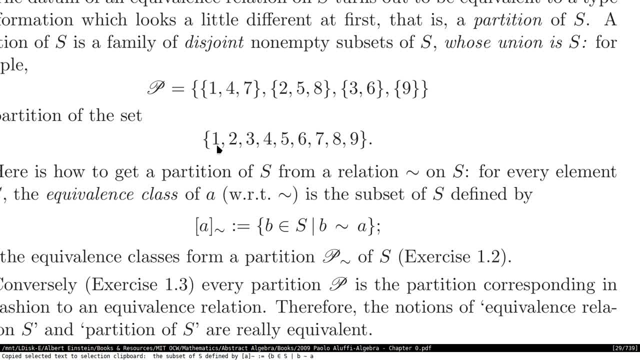 So we can identify 1 with 1.. Then 1 with 4. And then 1 with 7.. Right, So we. That's how we define the tilde to be. So again, what is the equivalence class of 1 in here? 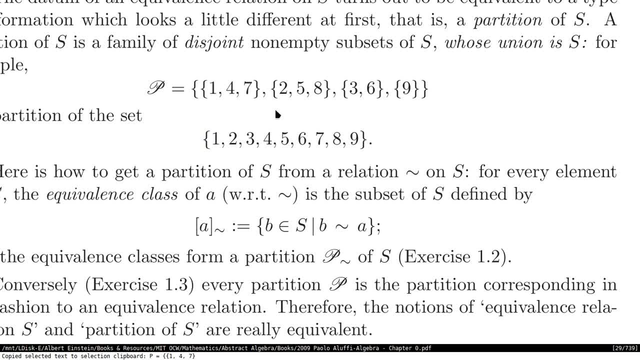 The equivalence class of 1 is precisely this, because that's how we define the relation to B. It identifies with these three elements, Right? Then we do the same for each of the elements, Then you're going to get these sets And then you have the partition of the whole set. 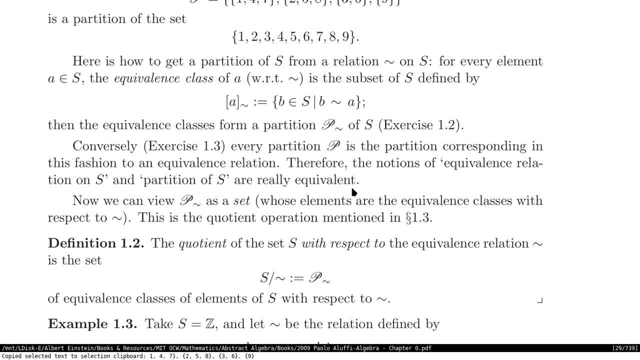 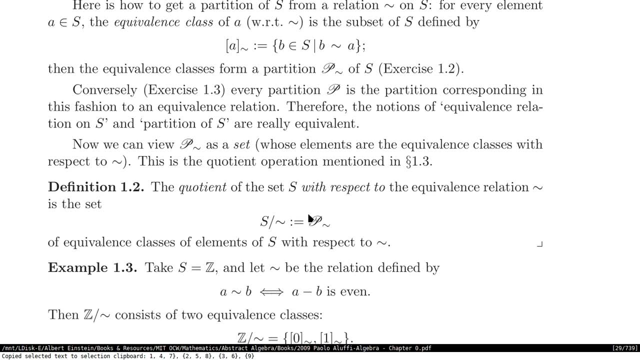 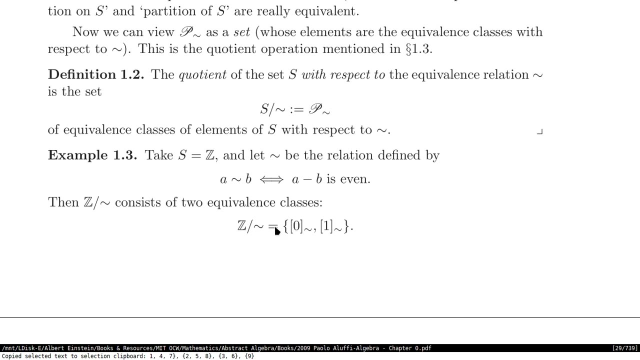 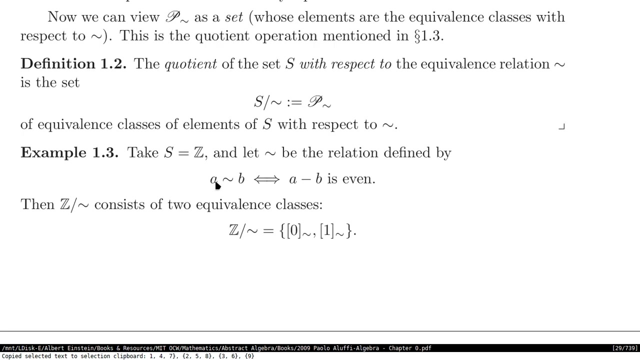 Right, So that's how the equivalence relation works. Yeah, So we have this example using the integers. So if you have the set of integers and the relation that you have is that you identify A with B, if, and only if. 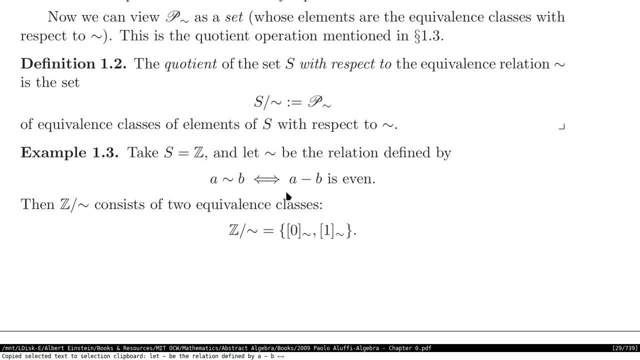 So this Symbol is just of if and only if. So A is identified with B, if and only if the difference between them is even, So A minus B is even Right. So you know, you can have, You can think about, like what it would look like. 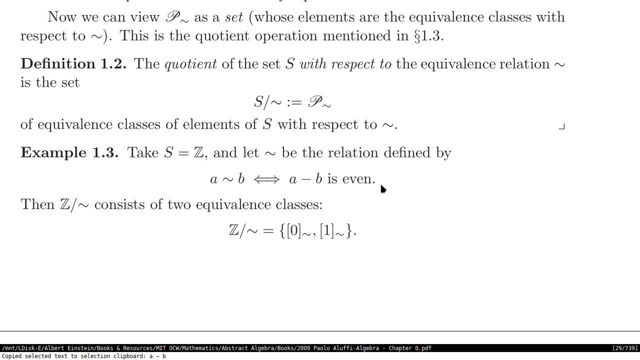 Right. So B is the set of integers You can have minus 1, minus 2,, 1, 2, whatever. So Let's see 3 can be identified with 1.. Right, Because 3 minus 1 is 2,, which is even. 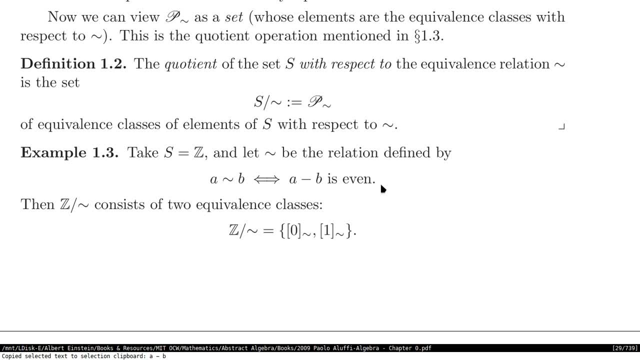 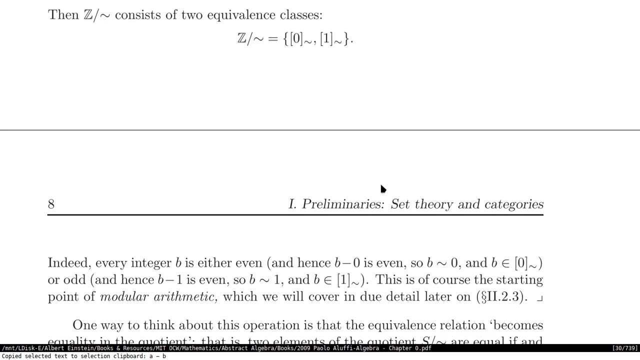 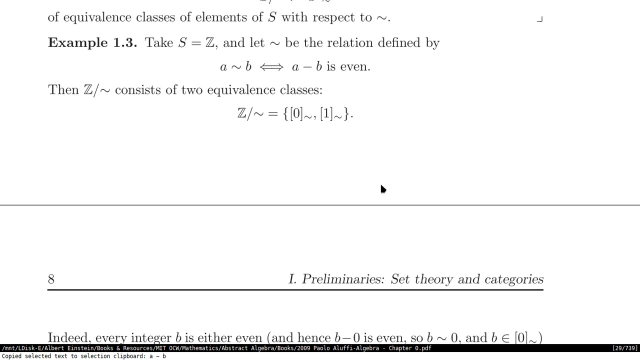 Then Let's see: 4 can be identified with 2. Because 4 minus 2 is even, And in this manner you can like think about the number of relations Identifications you can create with each Element. But the thing is, if you go with this, you're going to actually have just two equivalence classes. 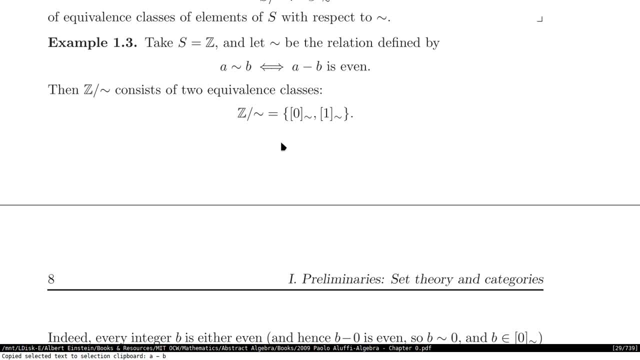 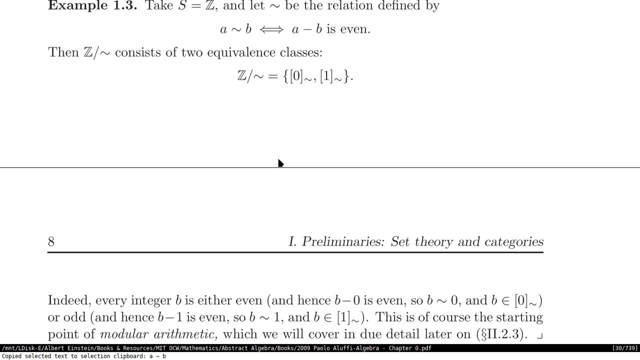 That is, of 0 and of 1.. So this is how it is. So This is the equivalence class of 0.. So the equivalence class of 0 is all the elements in the integers, all the integers which, when subtracted with 0, gives you even. 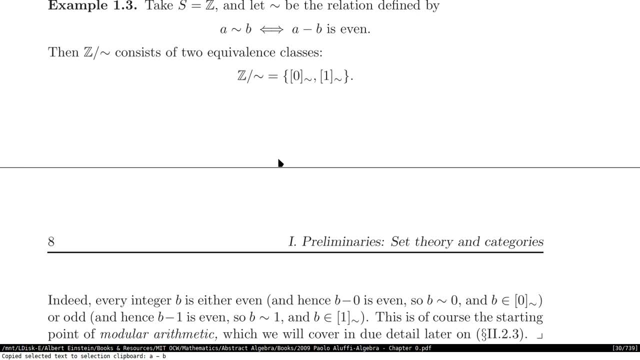 So that would be the set of all even numbers, Right, If you're considering the positives. So that would be 2,, 4,, 6,, 8,, dot dot dot, So that would be 1.. 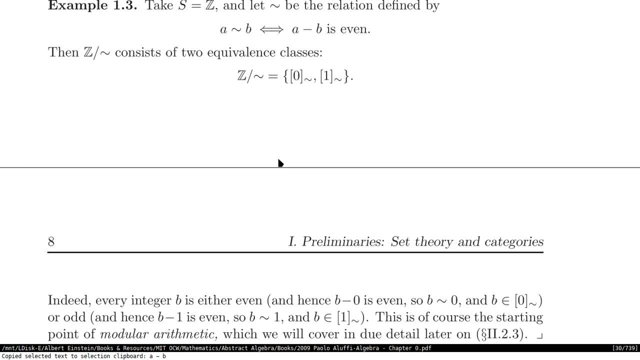 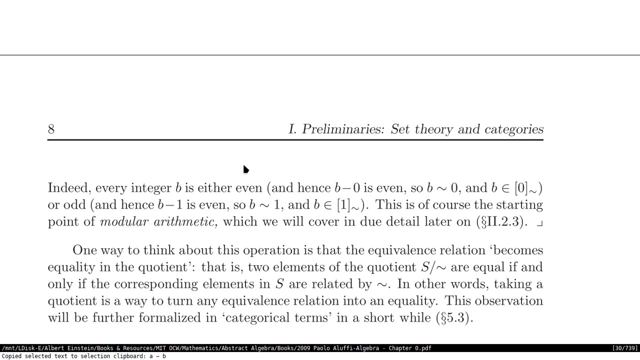 And then you would also have. Let's see, Then the equivalence relation for 1 is going to be all the odd numbers, Right, All the odd numbers. when you take the difference with 1, you're going to get even difference. 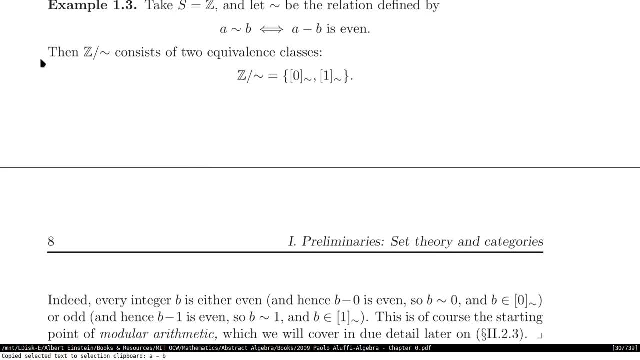 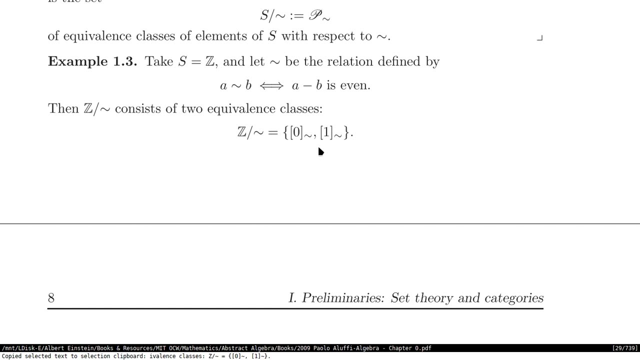 Right. So that's how the quotient space of the integers with this relation is just this, Right, And this is how it is helpful, Right, Because you don't really have to worry about each element of the quotient space or each element satisfying the relation. 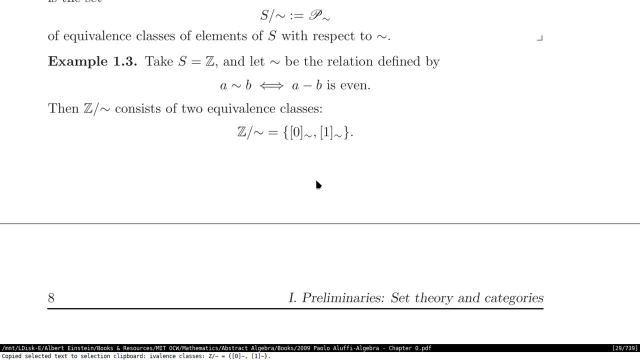 If you can find a relation and apply it to the whole set, it should just work, And then you can get the quotient space which lets you do a lot of things with it, which we're going to see later. But the direct consequence of this is: 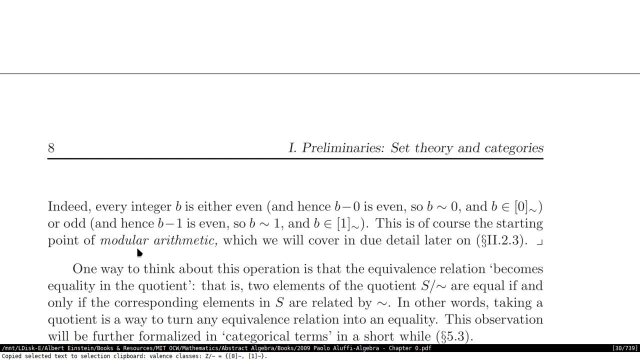 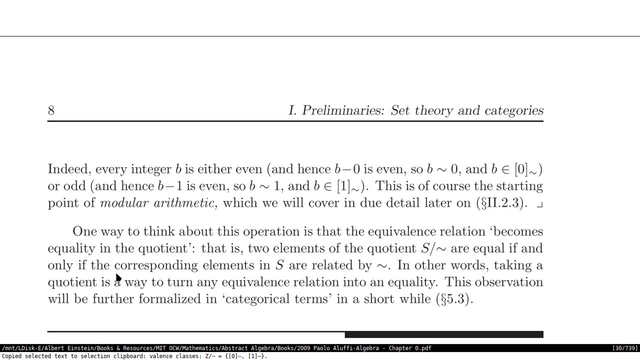 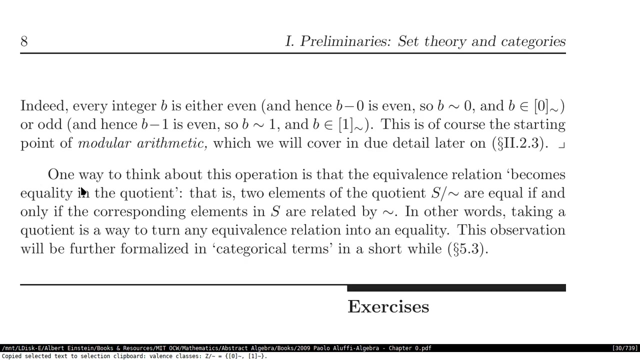 The direct consequence of this is modular arithmetic, which we're going to see when we do groups next week. Yeah, does it in the second chapter of groups, Okay, Yeah. So this is a very helpful explanation, One way to think about this operation of the equivalence relation. 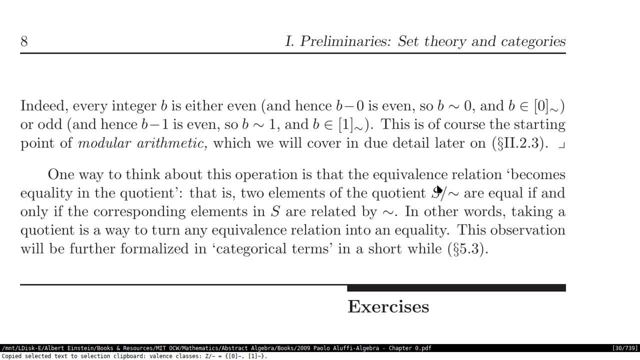 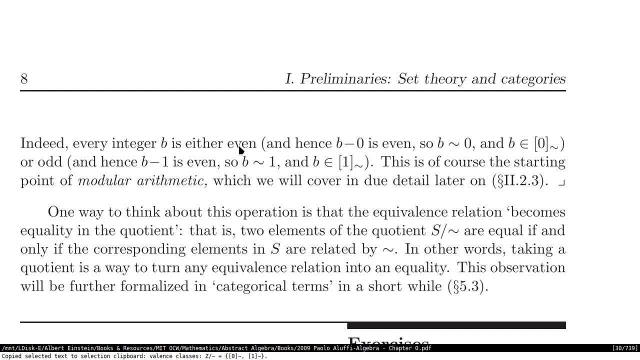 Is that, once you have the quotient space, these elements A and B are equal, considered to be the same elements, Right? So they become equal under this equivalence relation, And that's why it's important you can make things equal using this relation. 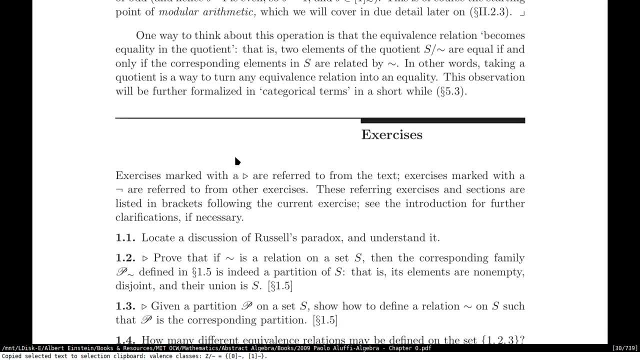 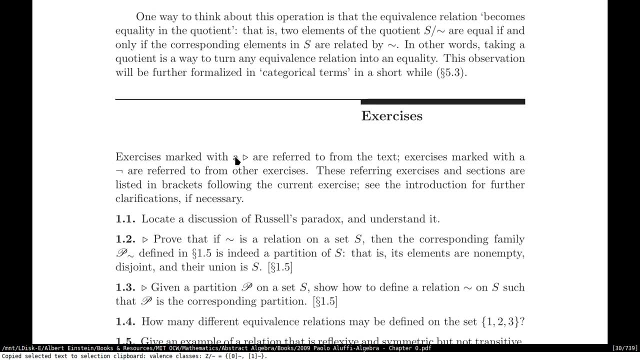 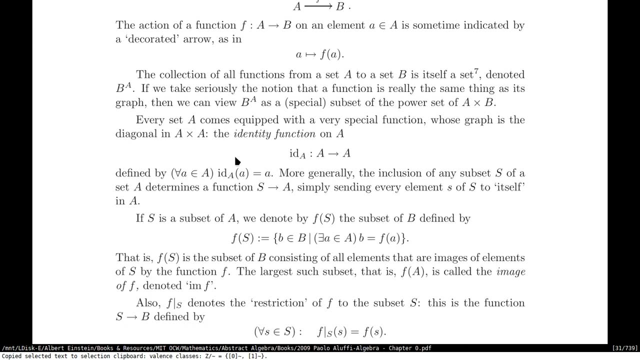 So that was about set theory, about equivalence classes, And we completed a section of the theory And we're going to give another hour to functions. Any questions on set theory as of now? I had a question? Sure, So I don't really understand the Zanello principle. 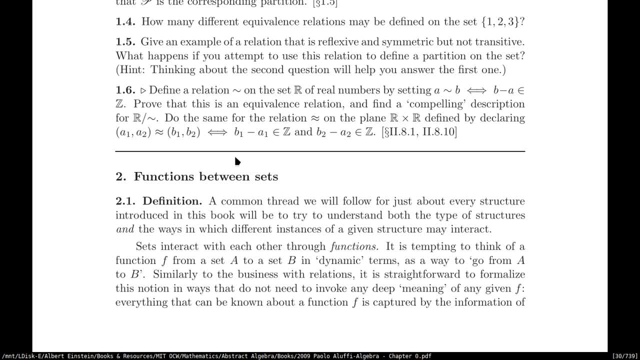 Sorry if I'm saying that wrong. Mm-hmm, The original axon, the first one, Mm-hmm. Isn't that part of the well-ordering theorem? Yeah, it is, Except you can't have the well-ordering theorem without the axon. 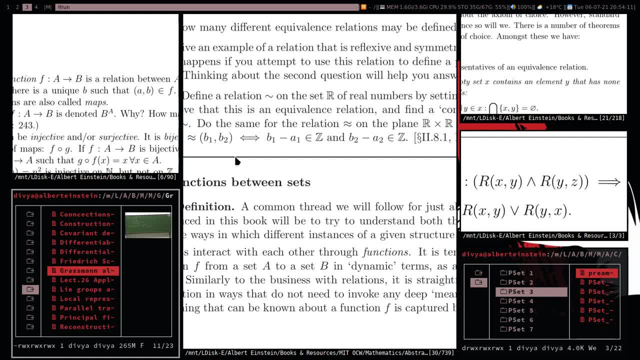 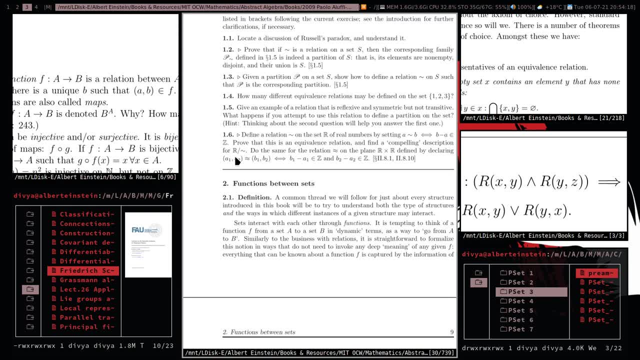 Okay, Yeah, So say I wanted to create a system capable of rendering infinite sets. Mm-hmm, If we chose a starting point like an origin, then there would exist an element within an infinite set that requires infinite space to render. 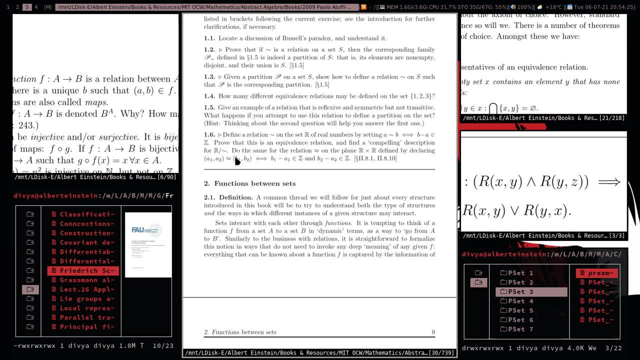 So we really wouldn't be able to choose an origin. So I don't really understand how you could represent infinite anything in this system. Okay, So if I understand you correctly, so you're saying, if you have an infinite set and you start from the origin, you're saying, like, the infinite subsets are not going to include the origin. 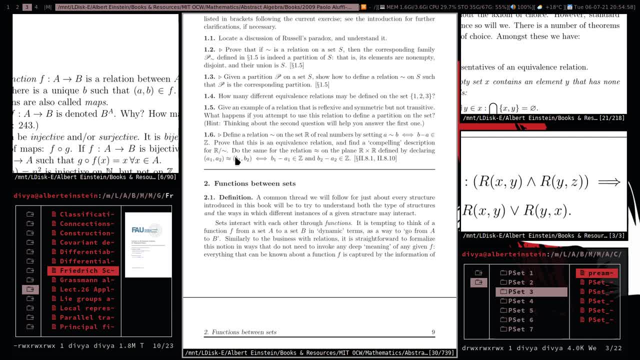 I can use an example of an origin. Okay, So say we define an origin and we just wanted to represent a single particle. Let's just assume that that particle is so far away that it would be impossible to ever represent that particle, because we don't have infinite space to even represent that vector. 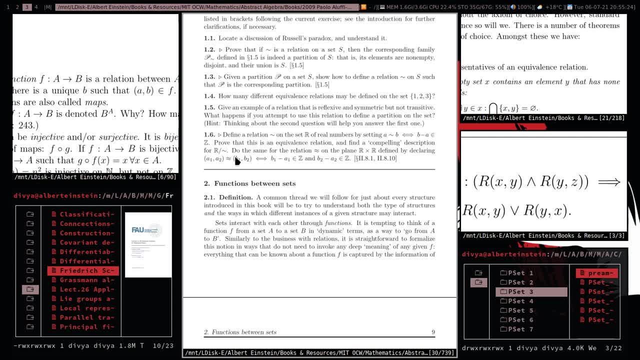 Mm-hmm. Wouldn't it mean that you would have to apply the same rules to every location in space in that particle system? Follow the logic. You don't really care if you can. The thing is the logic. the axioms allow you to have infinite sets, right. But whether you can actually have infinite sets, like a set which actually somehow represents infinity, that's a question the axioms don't have to answer. 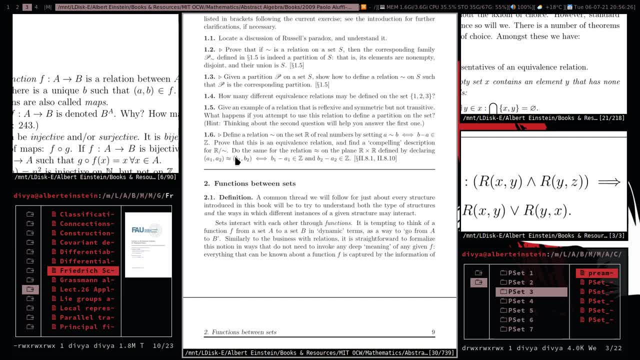 And this is again. this is like a typical of the things that set theory, foundations, logic even analytic philosophy deals with. It's kind of like. again, the example that you gave is about the physical world, right, That we can't represent a point that is like so far away and we don't have the. we can't formulate it using vectors, right, The position vector. we can't precisely write it down. 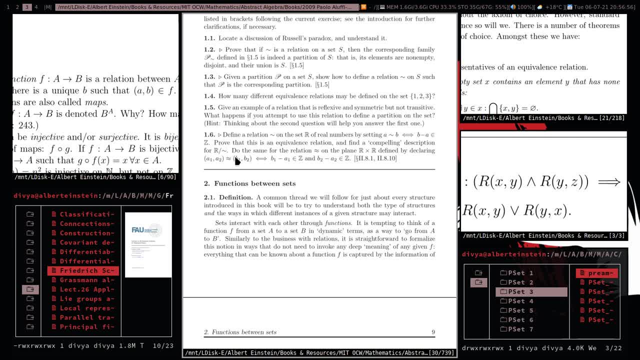 But in theory, the set theory axioms are going to say to you that you can actually formulate the distance using the subsets. Like the thing is, you can like have a vector until some point, right. So if you can have that, you can like repeat the process and use the chain to get there. 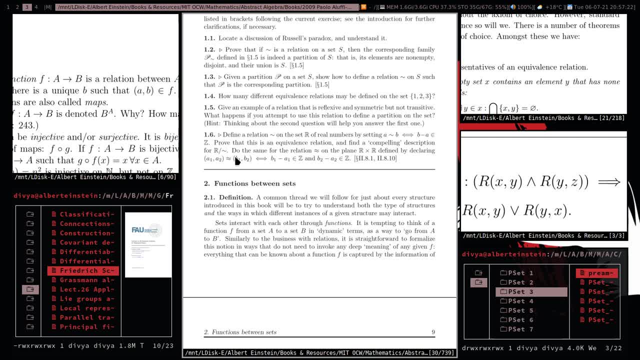 But if you're actually going to get there, it's not something that's Can be said using the axioms I guess I'm saying. if that position is not, is actually truly infinitely far away, You can say it. There's no frame of reference that you could take to where it stops. 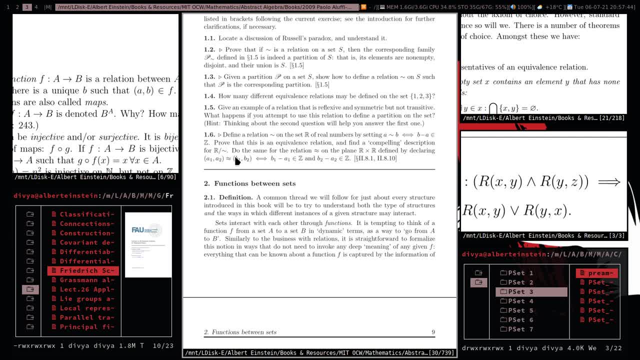 The thing is: how do you know whether it actually stops? Well, that's what I'm saying. If you do, you wouldn't even be able to tell if it stopped. Yeah, Yeah, the thing is, if it stopped, it would not be finite. 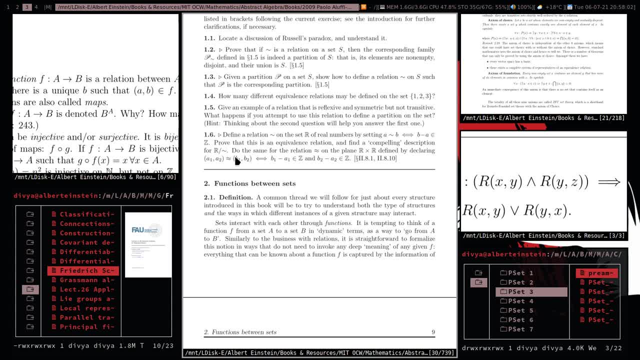 Sorry, it would not be infinite, right? Exactly Yeah, So that's totally logical. It's kind of circular logic, right? The definition of infinity depends on itself. That's precisely because we can't yet formulate anything precisely as infinite. 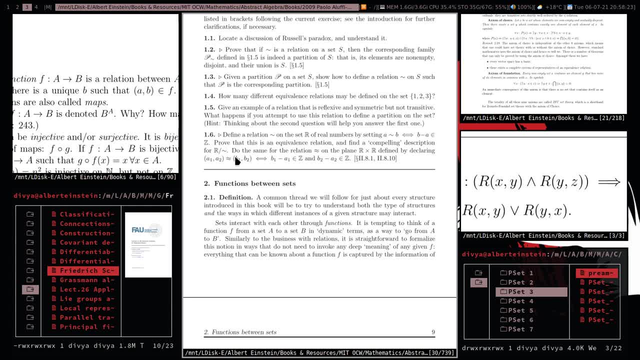 Because again, What does it mean to formulate infinity if formulation itself is dependent upon finite things? So yeah, I just don't see how you could choose a single origin and hold precedence over any other origin in an infinite system. Because I mean, the thing is: 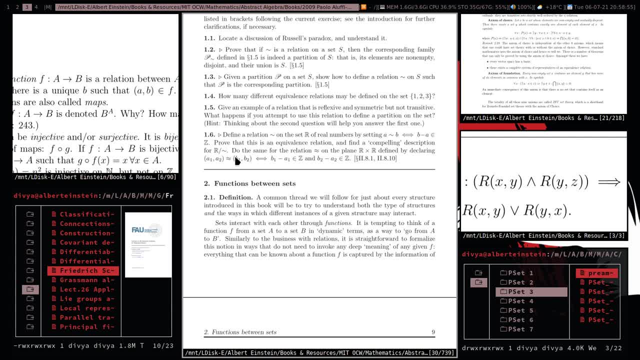 Okay, if you have the origin and you have the infinite system, the promise isn't that you'll be able to go as far as you can and still have a connection with the origin, Or like be able to get from the origin to there. 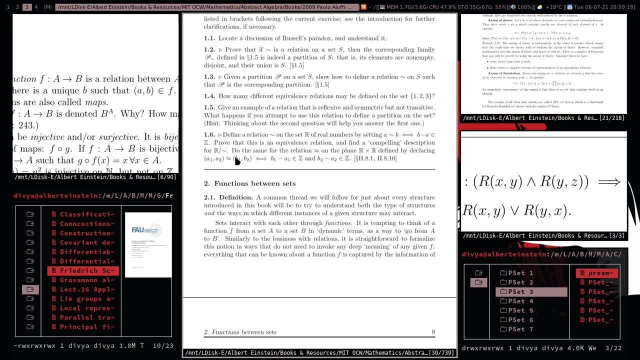 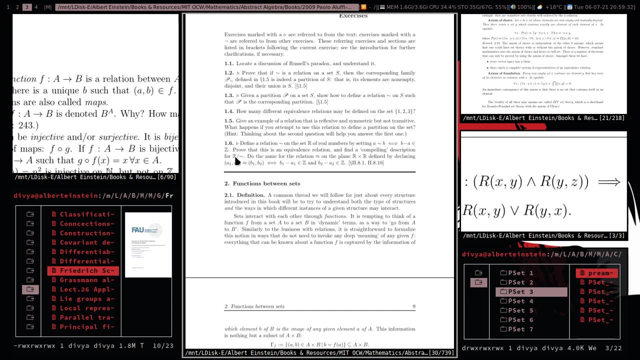 The promise is that the infinite point itself is possible, like exists, because of the subsets, as I said. But yeah, I'm not sure if what you're saying has something to do with the axioms themselves, but more like how they're applied. 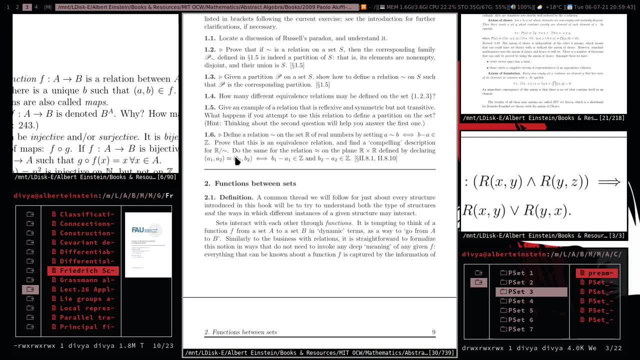 I think it's just more my. I have like an issue with the well-ordering theorem in describing the infinite systems. Okay, so we didn't see the well-ordering theorem, Let's see that. Well, I figured the well-ordering theorem is part of the axiom of the choice, right? 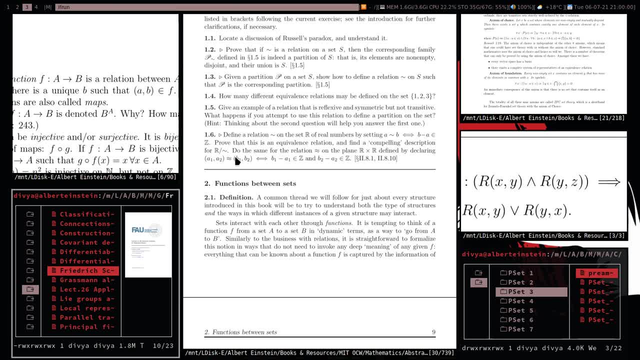 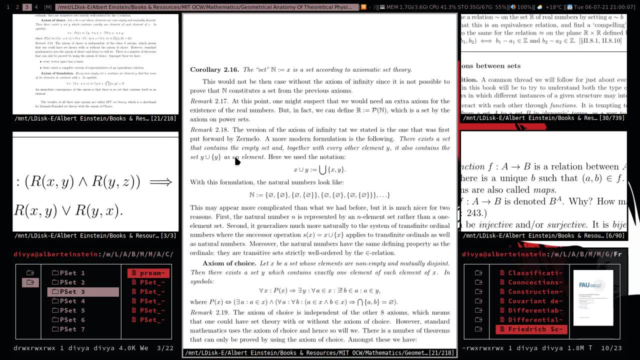 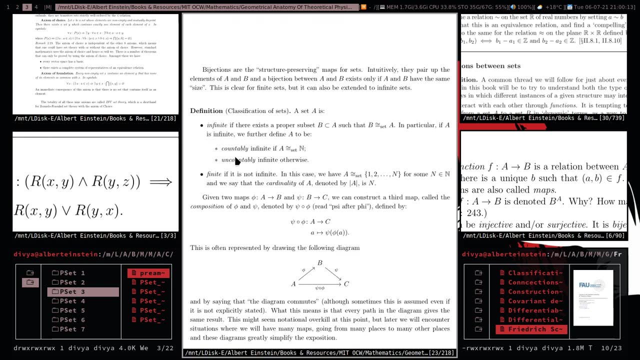 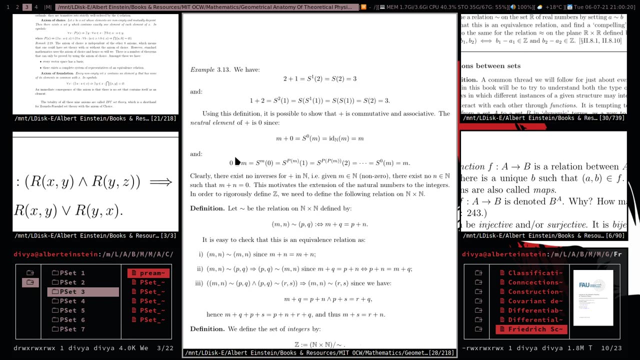 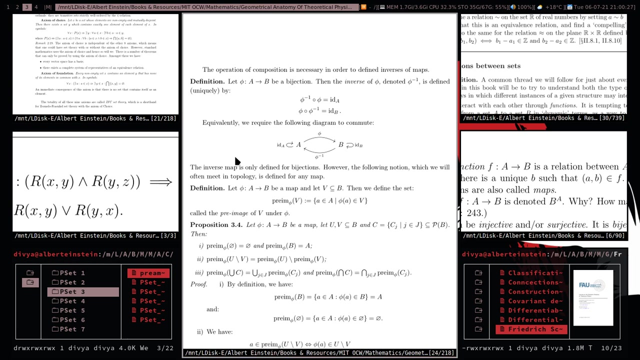 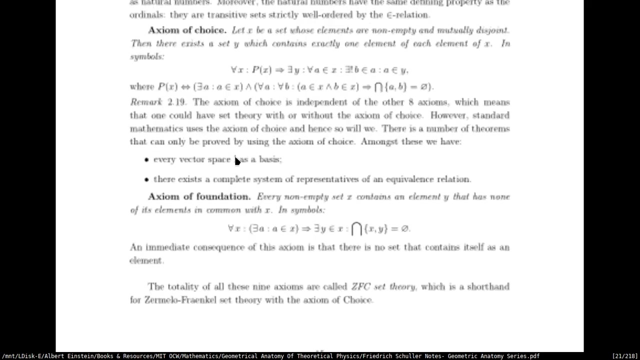 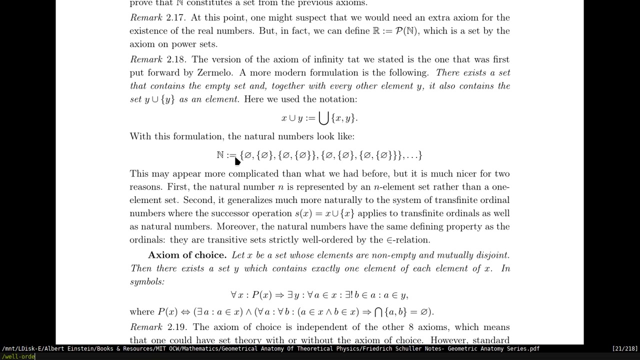 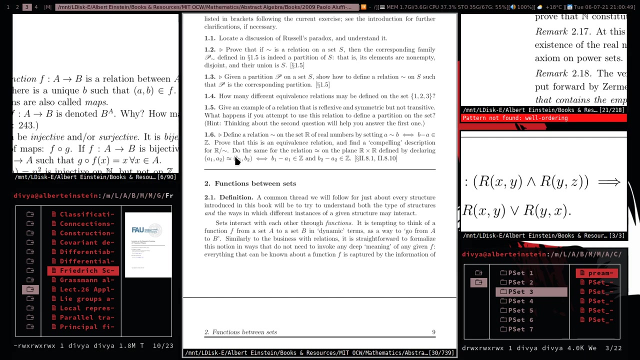 Or do you think, Yeah, you have the axiom of the choice from the well-ordering theorem. Indeed, I'm not entirely certain, Okay, Okay, so we should continue with the functions, I guess, And we'll see. 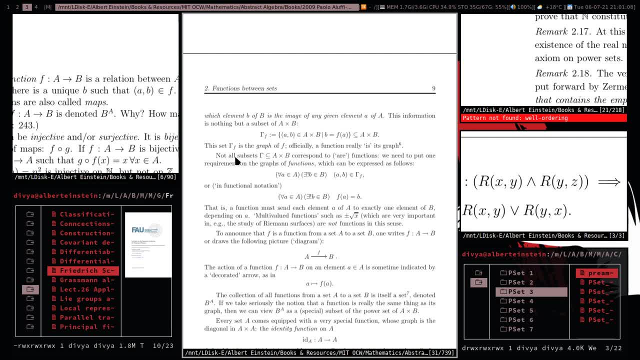 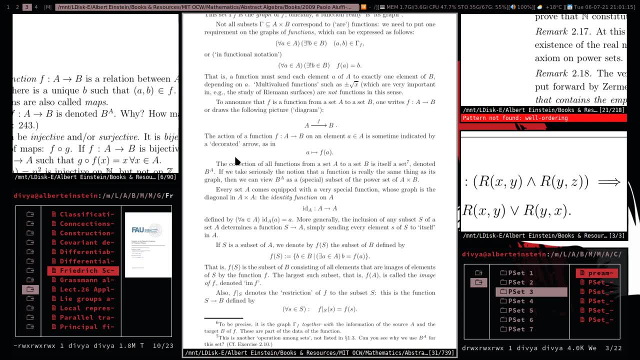 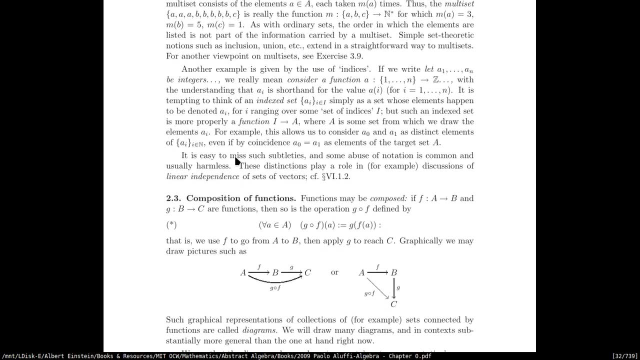 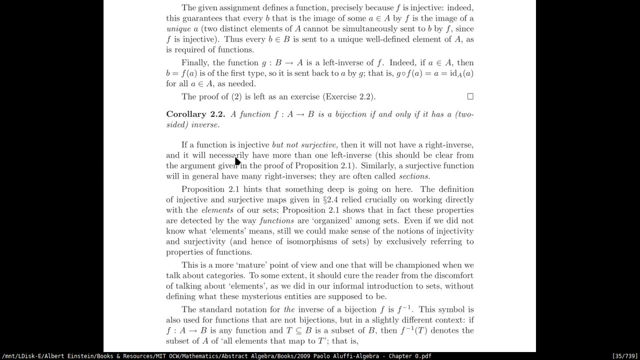 Yeah, Balto is right, Physically you don't have infinity per se. Okay, so we have actually a bunch of things to go through for functions, And they're all important, And the injectivity surjectivity. there are two different ways they approach it and some 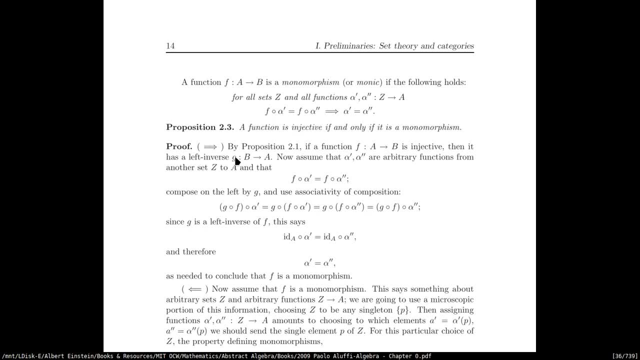 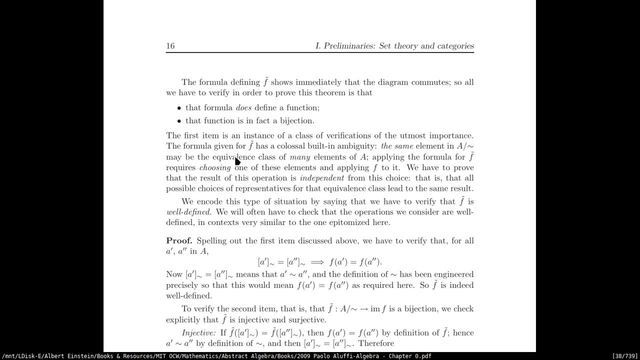 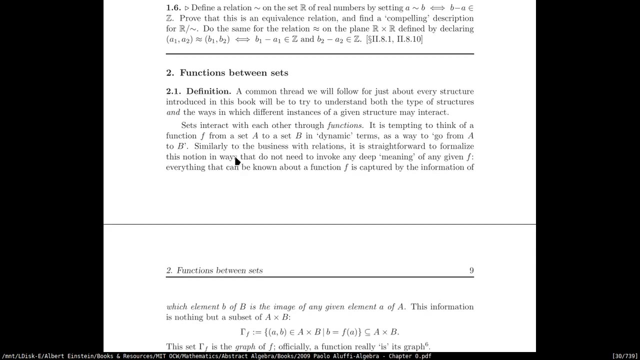 of the ways they prove it. so, yeah, let's see how much we can go through. I'm not going to go through like each of the proofs because that would be too long, But we'll try and discuss. Okay, so what is a function? 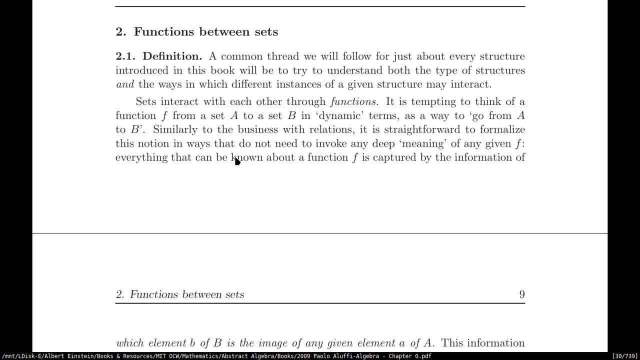 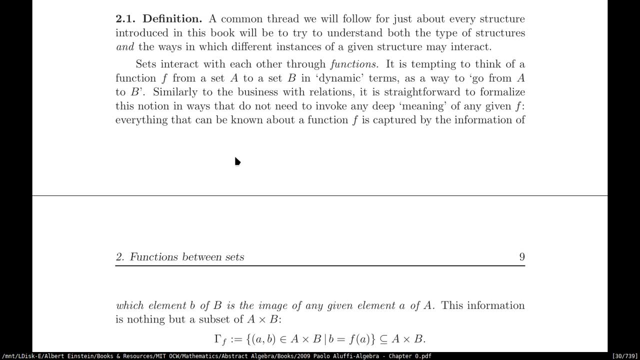 Okay, so the function is. well, they don't actually define it here, but a function is such that you have a relation between two sets such that, for any given element of a set, you have precisely a unique element, which is this image. 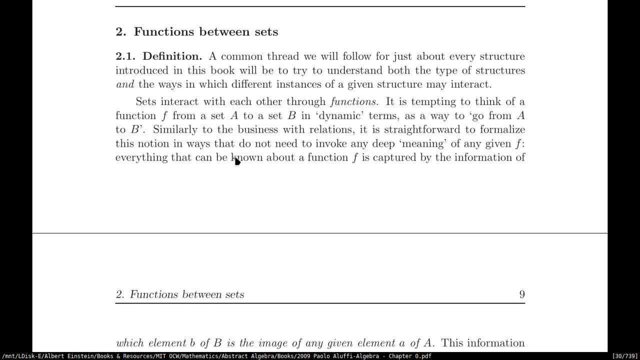 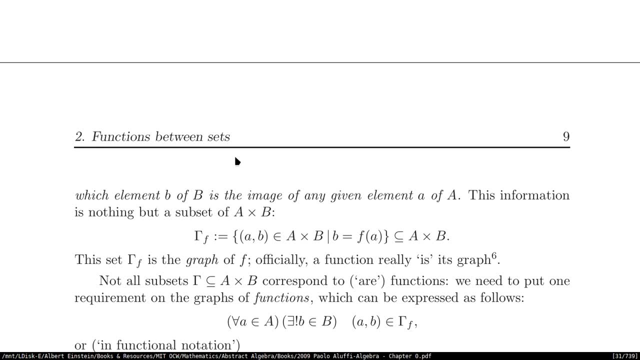 So this is actually the graph of a function. So, the graph of a function, they denote it with the gamma sub f. so it's the graph of f. It's a subset of all the other pairs, a, b, from a cross b, such that b is the order of a, b and a- b. So this is a subset of all the other pairs, a, b from a cross b, such that b is the order of a, b and a- b. So this is a subset of all the other pairs, a, b from a cross b, such that b is the image of a under that. 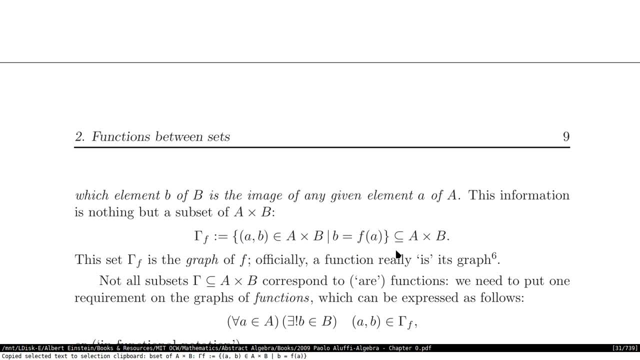 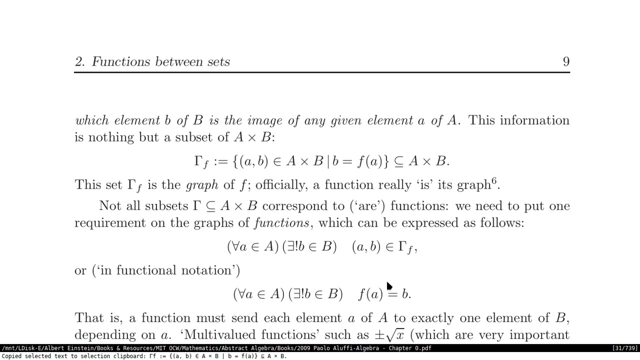 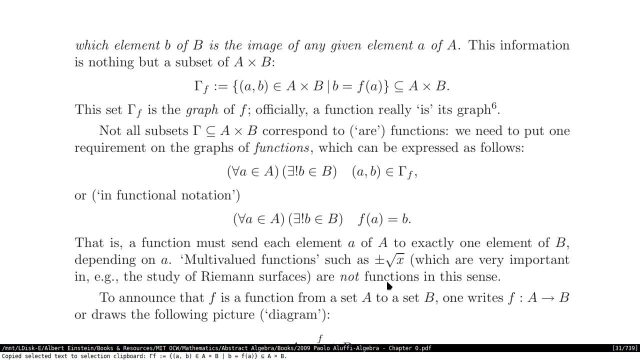 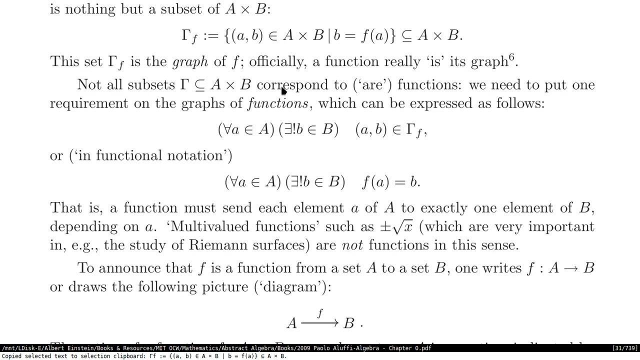 So this is going to be, yeah, all the pairs a, b, such that the latter is the image of the former, And this graph is going to be a subset of the Cartesian product of the two sets. Okay, so Yeah, not all the subsets of gamma correspond to functions, Not necessarily, but for a function. what we need is this condition actually: that for every element a in the set a, there exists a unique b, such that f of a is b. 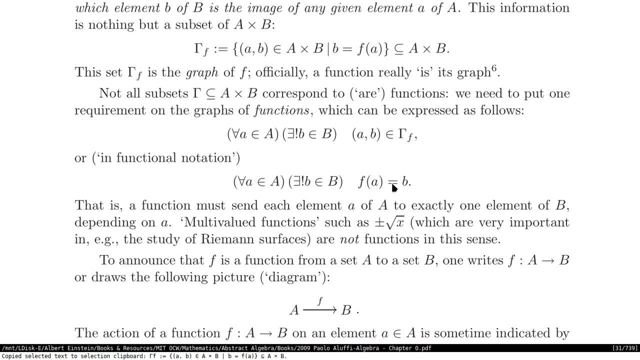 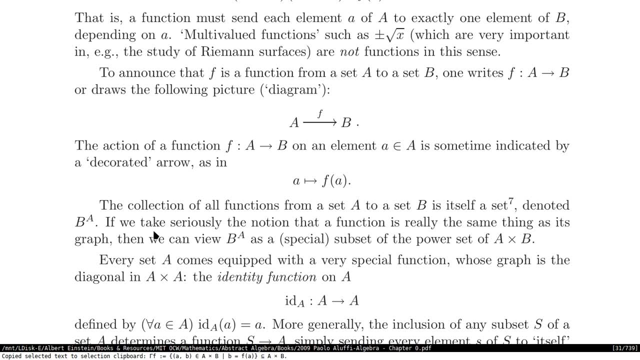 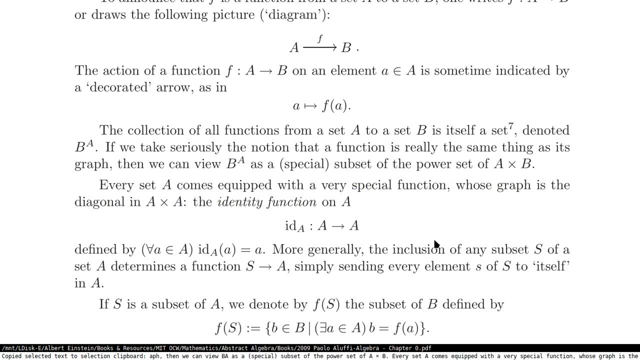 So that must be the case for it to be a function. And then you have the notation f from a to b in a typical way. So this is one of the special functions. So this is the identity function. So the identity function takes you from an element in the set through the set. 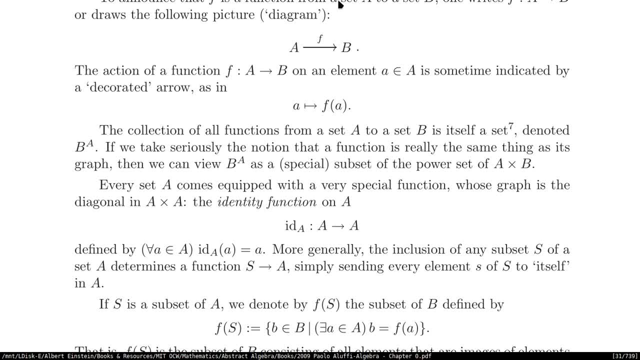 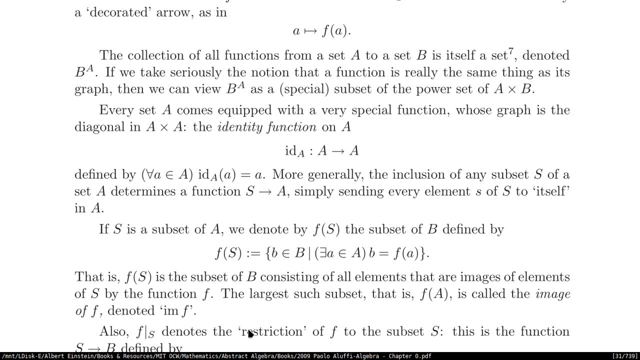 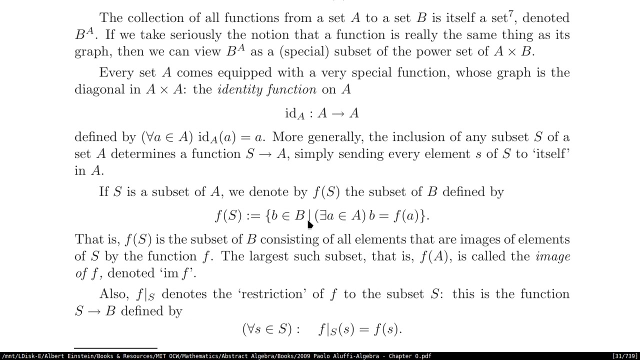 From the same element in the same set. It's essentially just going from the same set, from the same element, to the same element in the same set. Okay, And then you define what is the image of a. I already told you that if you have s as a subset of a, 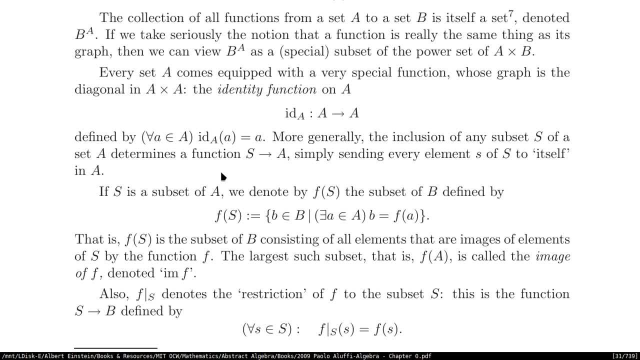 then f of s is going to be a subset of. we denote by f of s the subset of b defined by yeah. so f goes from a to b. So f of s is a subset of b, which is like the set of all the images of f. 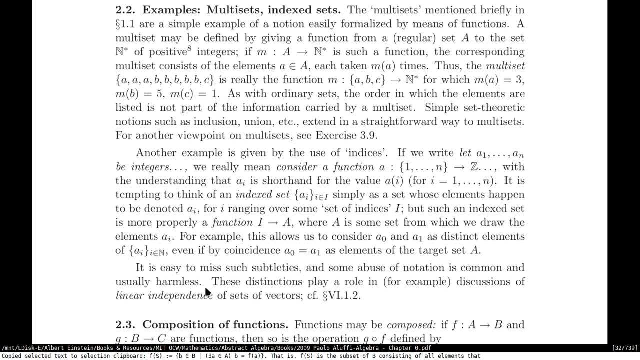 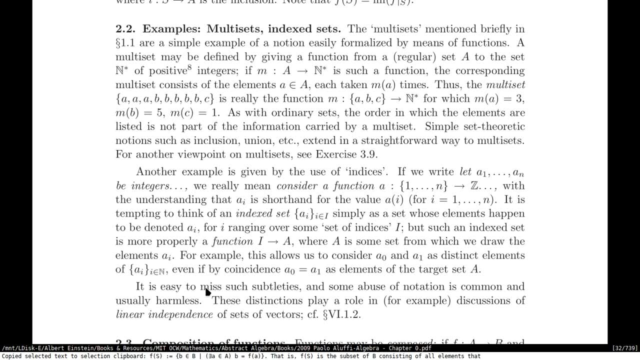 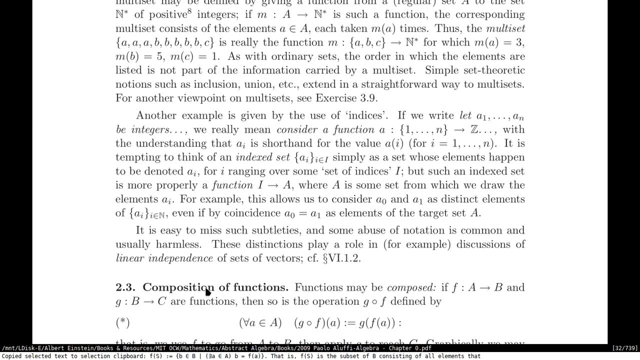 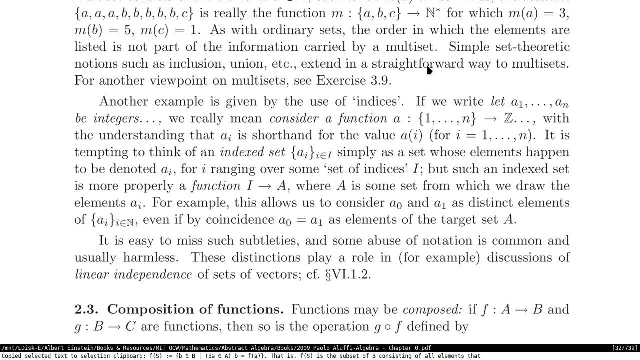 Mm-hmm. Okay. So yeah, this is kind of important because the notation can be confusing sometimes when you have indices and functions. So if you have a1 to a2.. So if you have a1 to a2.. So if you have a1 to a2.. 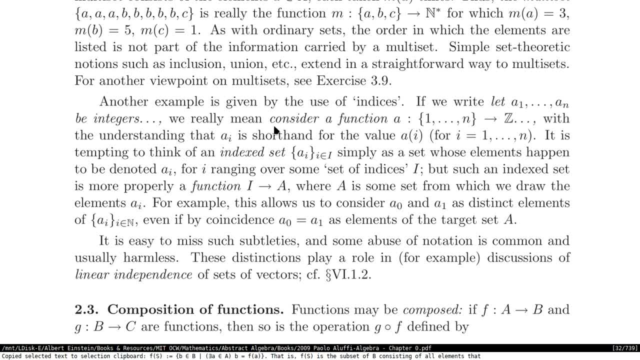 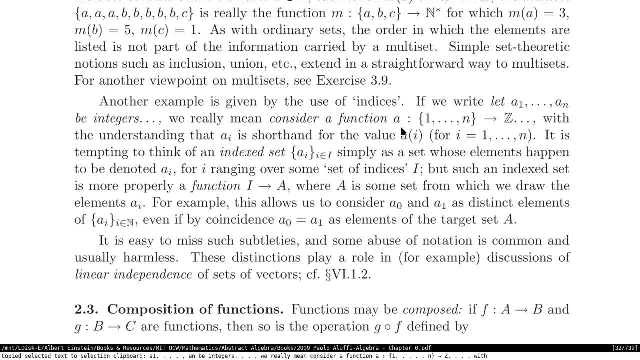 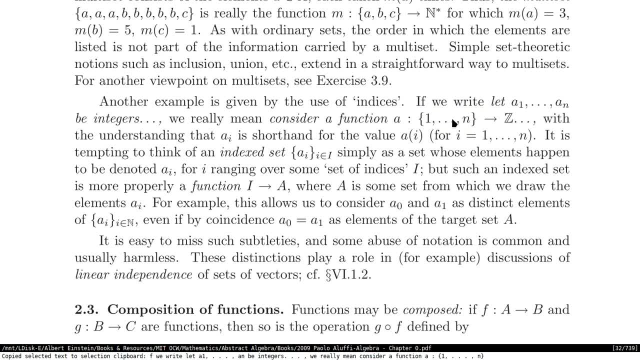 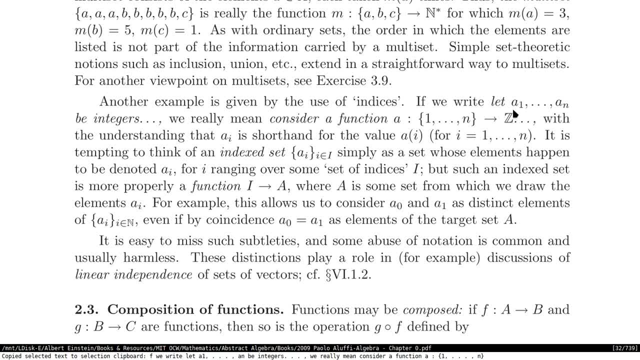 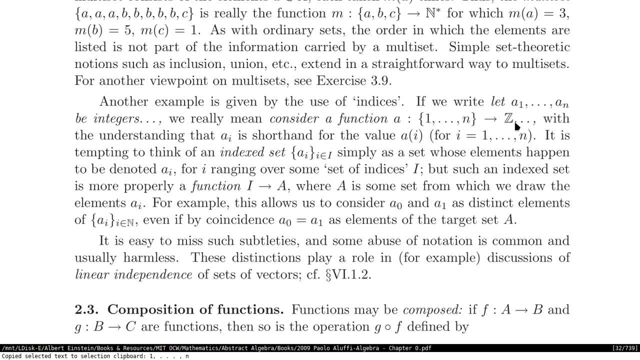 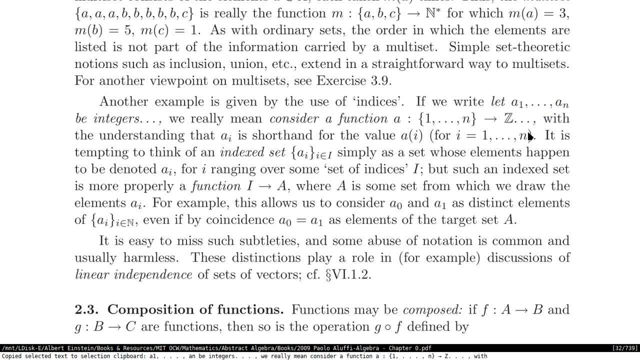 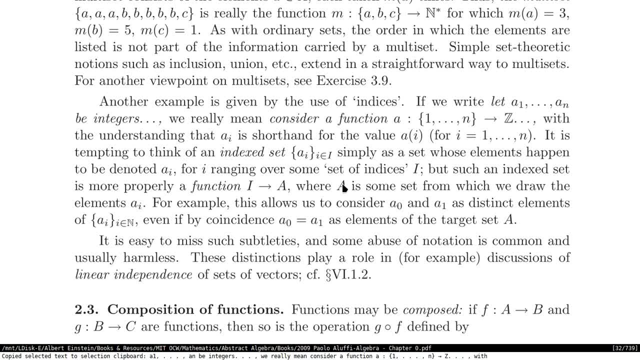 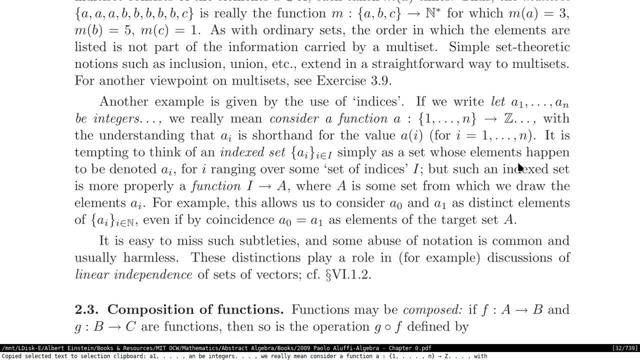 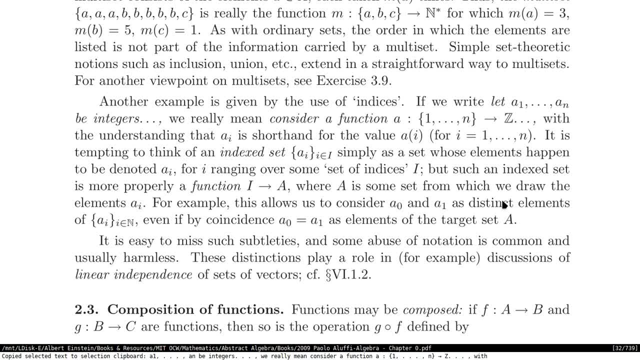 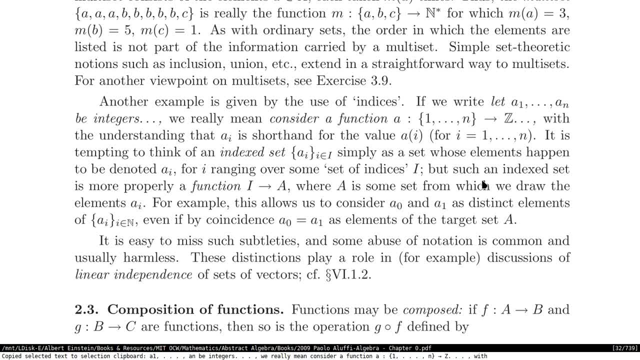 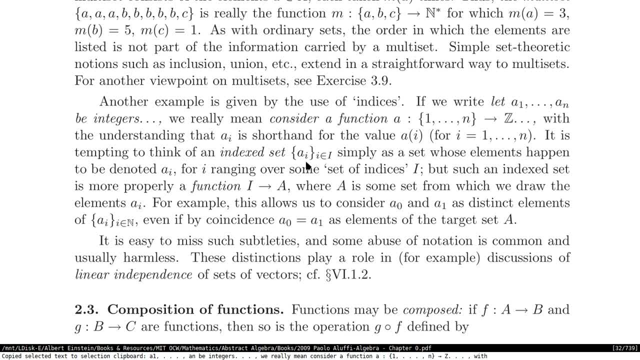 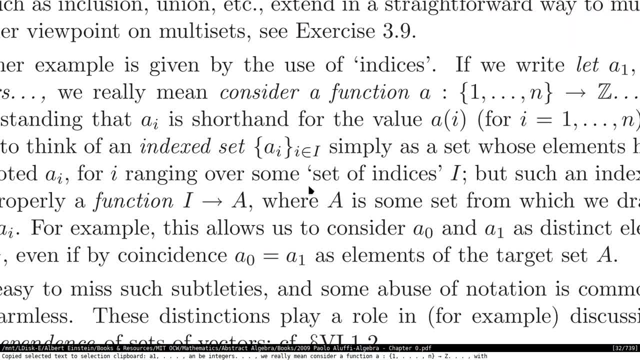 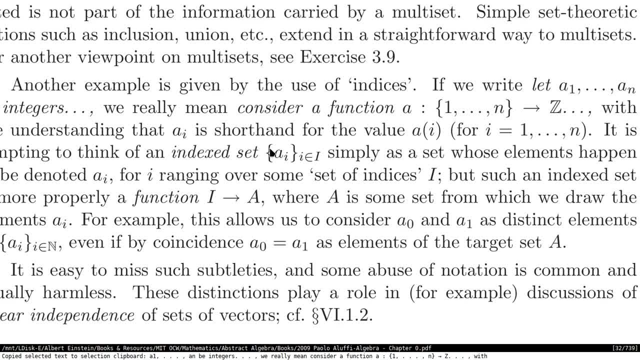 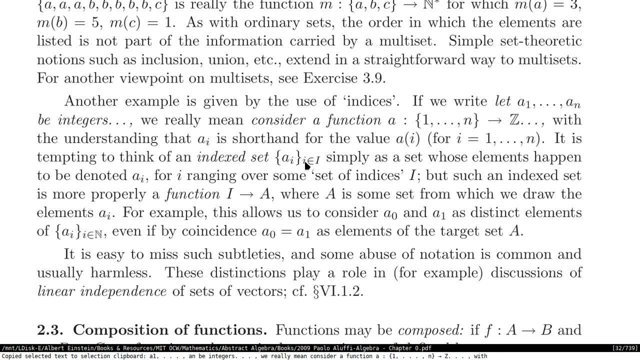 this index set is like the set of ai's, where i is like: belongs to this index, i capital, i right. so so this index set simply is a set whose elements happen to be denoted by ai, for i ranging over some set of indices i. so this is like how normally we want to think about it. 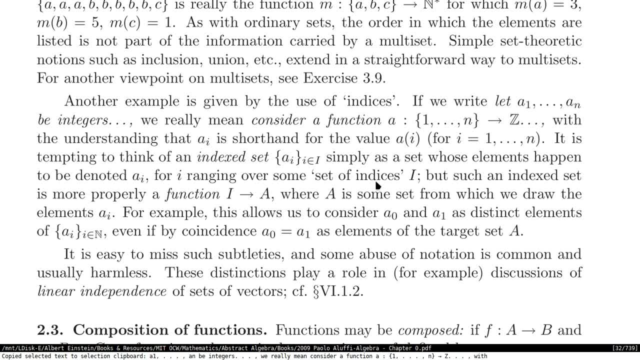 but that's not really what it is. um, it's actually you have to think about it as a function, right? so, more properly, it's a function from this index that we have, i onto a who has, which has elements, these ai, right, and that's how you get this indexed set, and we're going to use the indices a lot. so 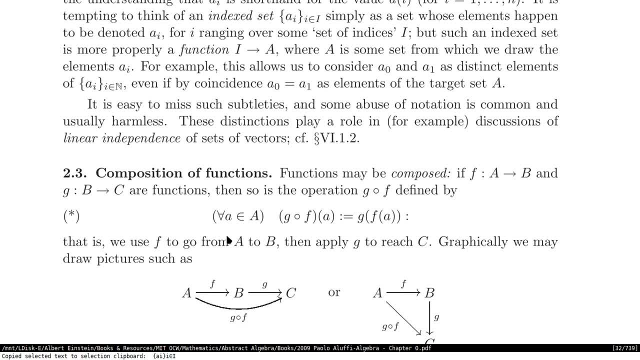 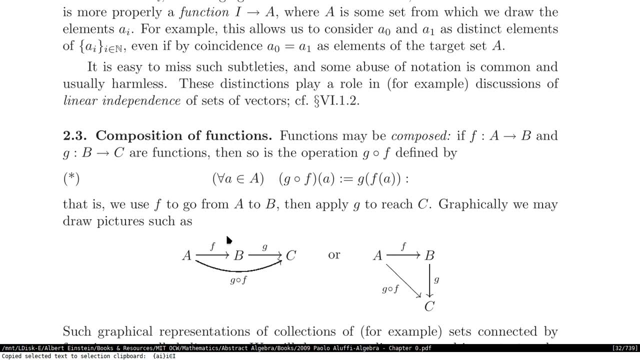 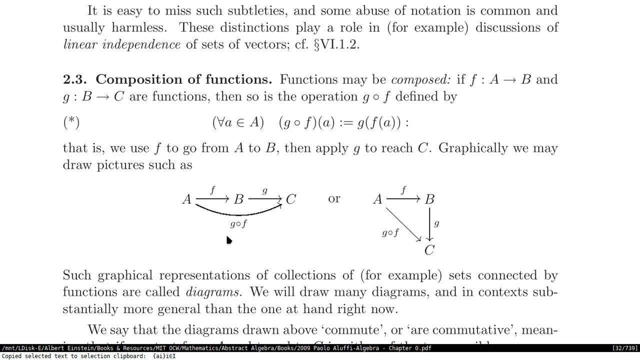 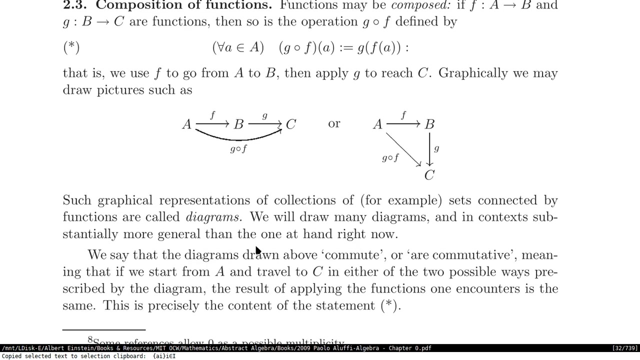 yeah, that's important. and then you have the typical way you define the composition of functions. so if you have functions f and b going from a to b, then b to c, then you can have g circ f which goes from a to c. so, yeah, you probably have seen this before. 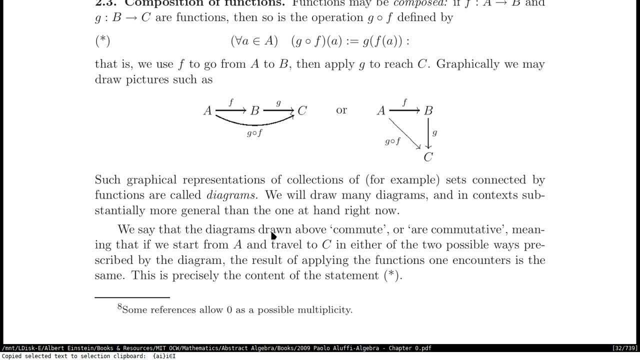 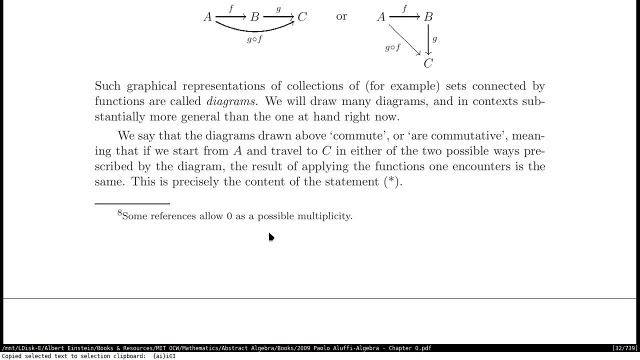 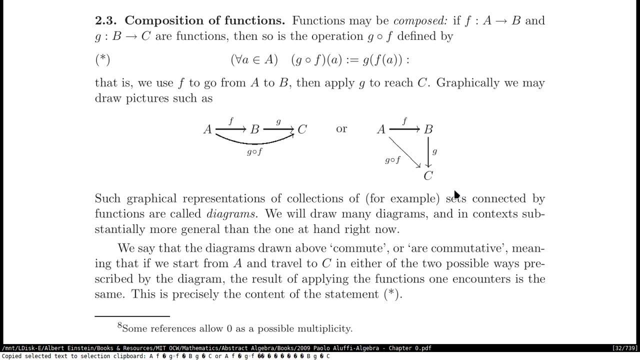 yeah, so the composition is one of the most basic and almost always used things in functions and maps, and these diagrams are what we're going to meet on thursday. we're going to use a lot of them for category theory, but this is how you represent the, the mappings of the functions. yeah, 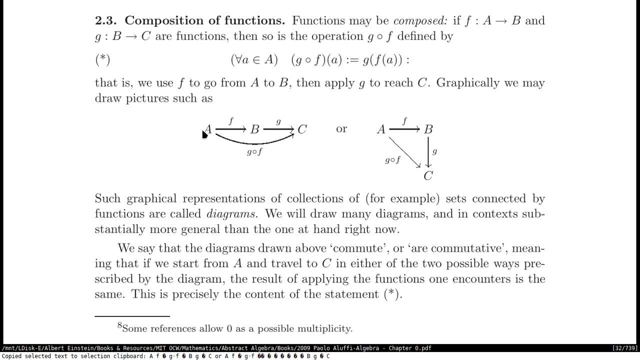 so, um, so like. these diagrams are actually, uh, what you would call of like, um, a commutative, or the commute. so what it means for it to commute is that if you take um, like the composition of these two functions, you're going to get this one right. 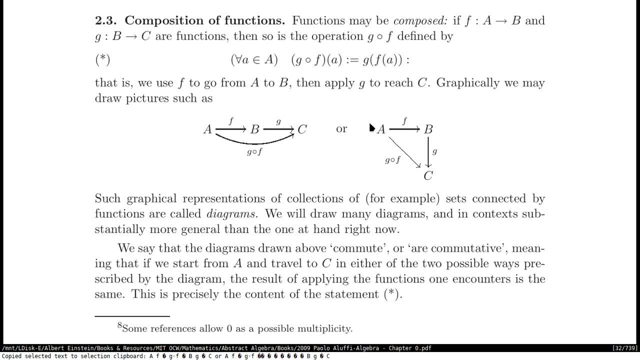 so f circ g, sorry, g circ f- is going to give you this function and then, if you like, do it in any other way, going to get the other function if you take the composition of the other two. so that's what it means to commute: you can like travel around following each. 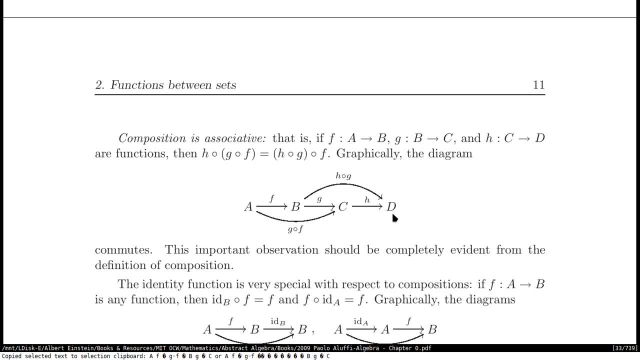 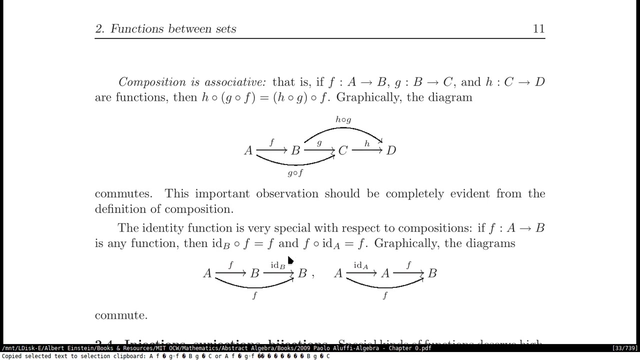 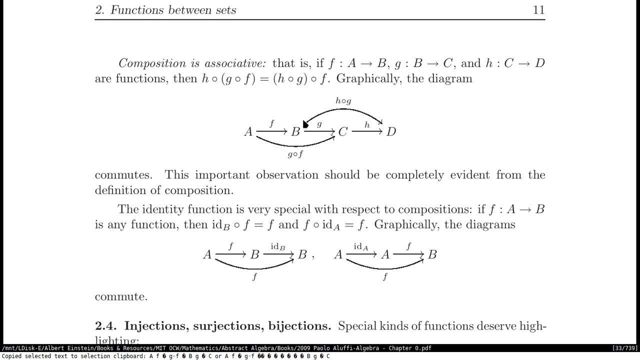 function as it is defined. and yeah, one of the properties of composition operator operation is that it is associated. so H serve G, serve F in parentheses is equal to H serve G, parentheses, then serve F. you can move around the parentheses and the composition still stays intact. and this is pretty much straightforward from what 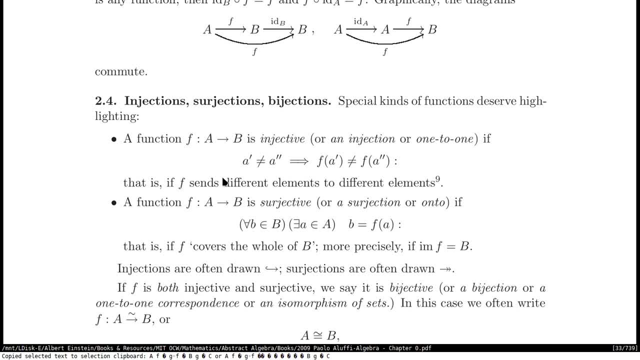 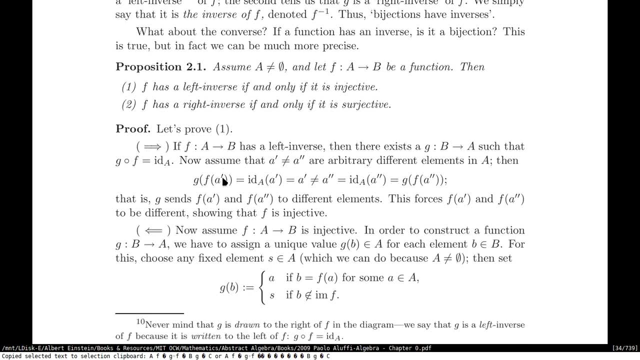 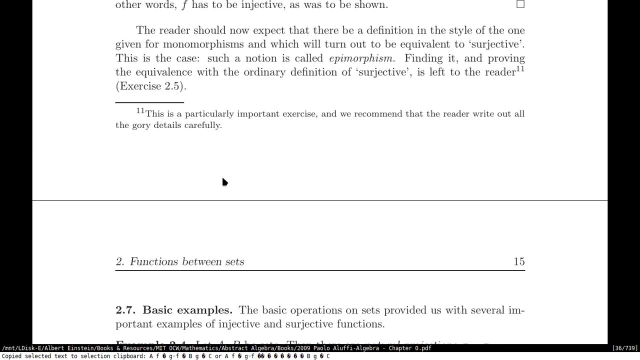 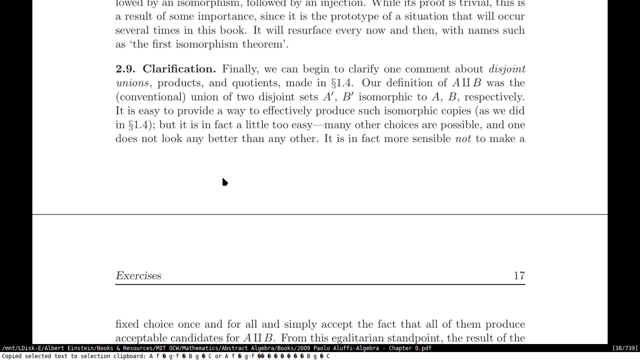 is defined, as you the composition. so yeah, that's, that's about the basic stuff. we're going to see the injectivity and subjectivity, and then we have some interesting results. not interesting, I mean, you've seen this before. but yeah and yeah, let's see you. 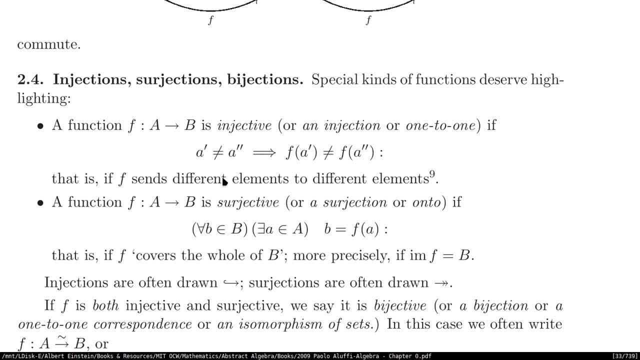 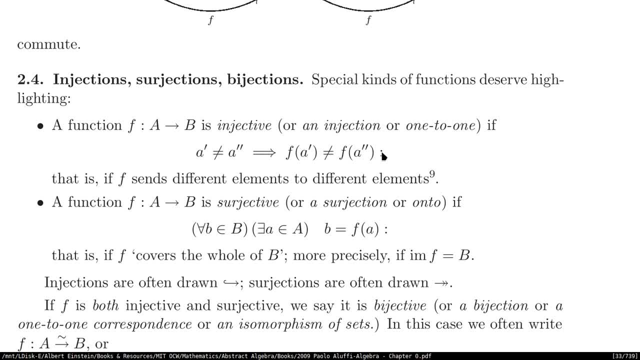 so the image of a prime can never be equal to any image of any other element under F. so F of a prime is always: um, uh, you can never be equal to the image of any other element unequal to f of a prime. so, yeah, it sends different elements to different elements. 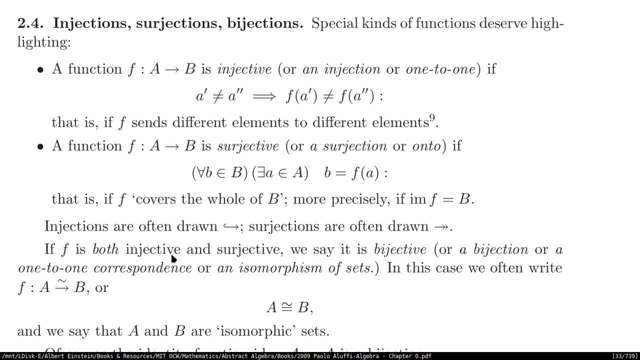 so that's injective. then what's subjective is that it sends one element at least to another element in the codomain, but it can send to more than one element, right. so for all b. in b there exists a, such that b is equal to f of a. 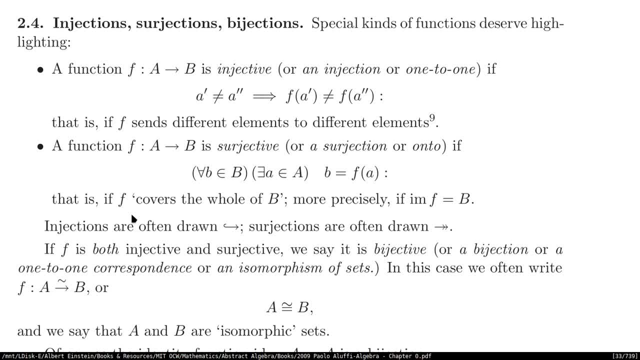 so f- quote, unquote covers the whole of b, but yeah, more like, like the image of the function is the codomain itself, right? so each of the element in b is always mapped. sorry, yeah, mapped by something in a right? so for every element in b you can find: 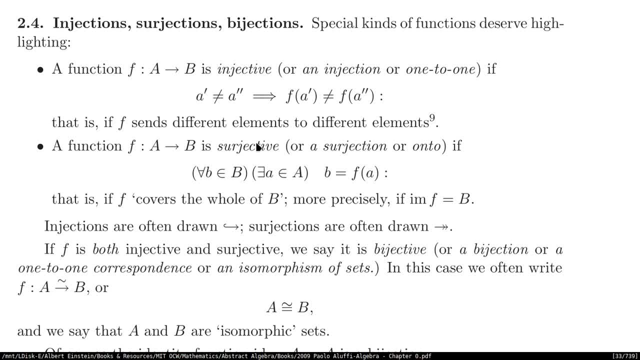 another, something in a such that is mapped to b, right? so, yeah, b is always covered, or more like these: like no element of b is missed, okay so, and when you have, like, both of these properties, you get but a be objectivity. so that's everything to be. 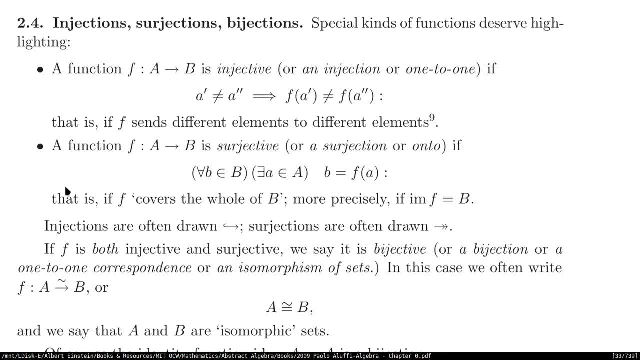 moved around. you can see they're� connected, you know. so in general sentence: you Чер galaxy, so distribute that. it's in here. Download ā you and paid money Jeżeli n through. so fierasti kind of correspondence you want between two sets, so every element is mapped to. 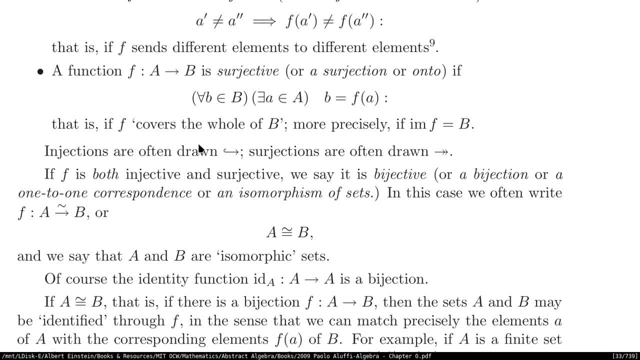 something and then mapped to precisely one thing. and yeah, and when you can have this projectivity between two sets, you can write them like this, and that makes them isomorphic, and we're going to have isomorphism and different things as we go along the course. the next one that we're going to meet is going to be the 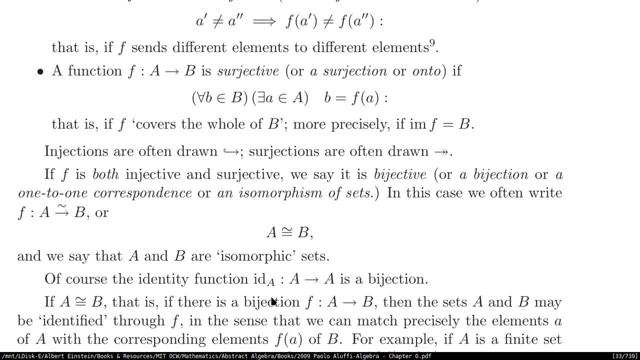 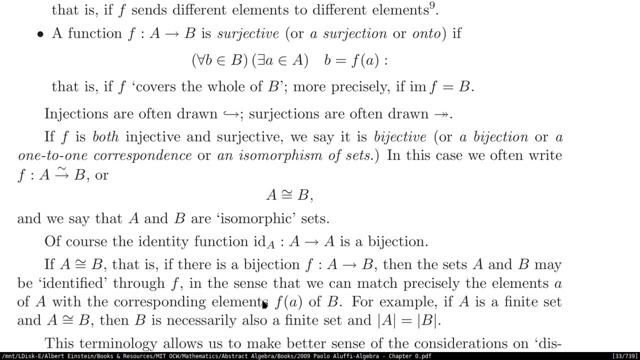 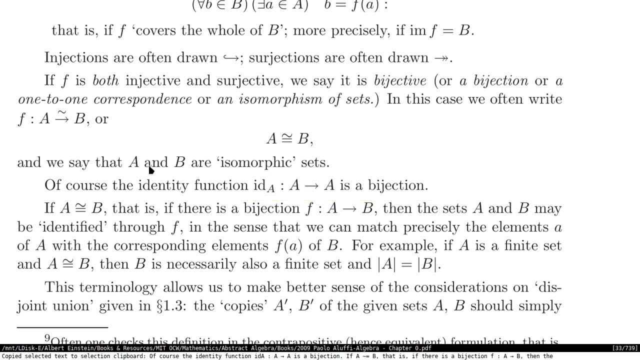 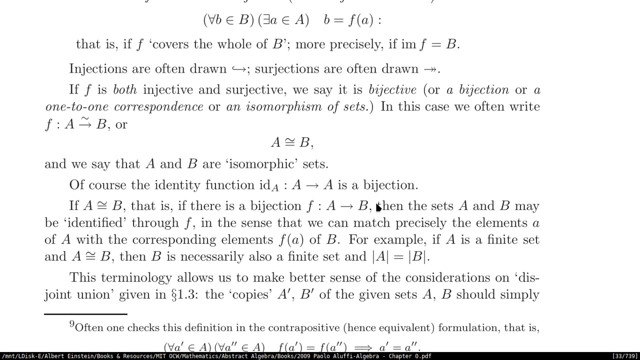 group isomorphism, but isomorphisms are always bijective, no matter what objects they're dealing with. and yeah, quite obviously the identity function is the bijection, because you're mapping the same thing to same thing, so you know, it's always something injector, and so 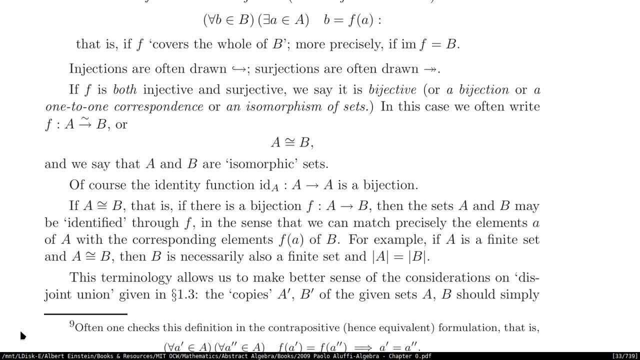 okay, so if A is isomorphic to B, so that means you have a bijection from A to B, then the sets A and B can be quote-unquote identified to F. right, so so F allows you to like identify each element of a with some element of B, and you can. 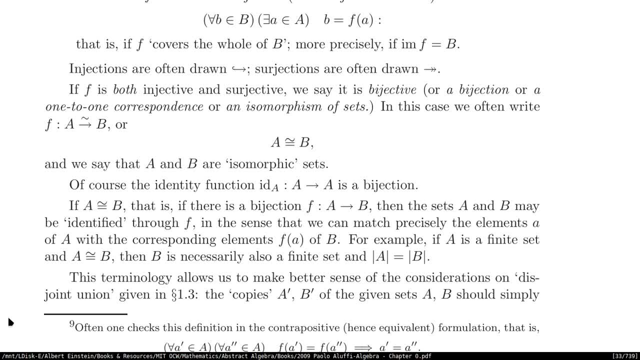 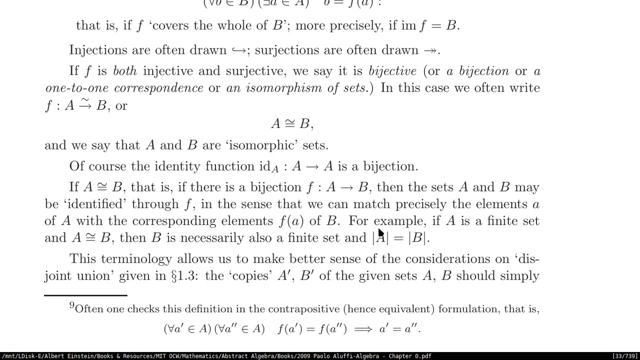 do that for every elements, each of these elements, elements, and then what you have is like a unique way of identifying every element with this function, right? so these sets are now identified, or they identical, under this specific function, right? so yeah, in the sense that we can match precisely elements of a of a with the corresponding 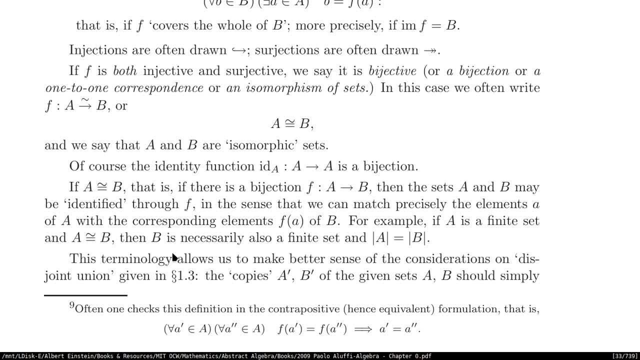 elements f of a of B. yeah, yeah. so this, this is like a corollary- that if A is a finite set and A is isomorphic to some set, B, then B also has to be finite, because you know you have an isomorphism, so like, like there has, there can be finite. 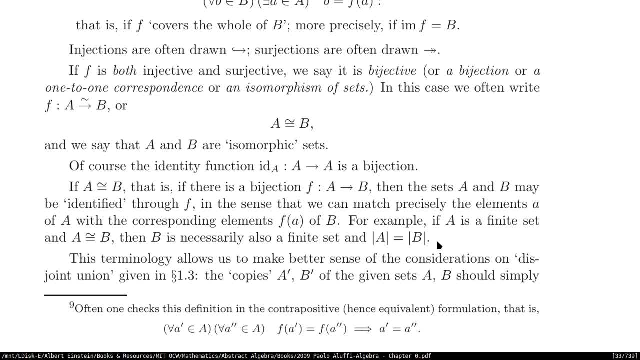 many, finitely many correspondences from the elements of a in the Norwegian Spell elements of B, and so that means B has to have finite many elements, and also that the cardinality of A is equal to cardinality of B, because each of the elements need to be mapped to a specific thing. 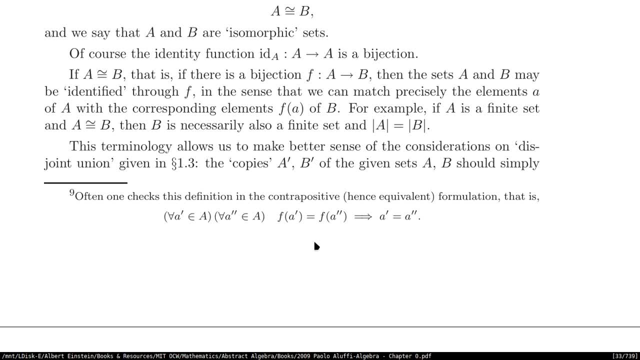 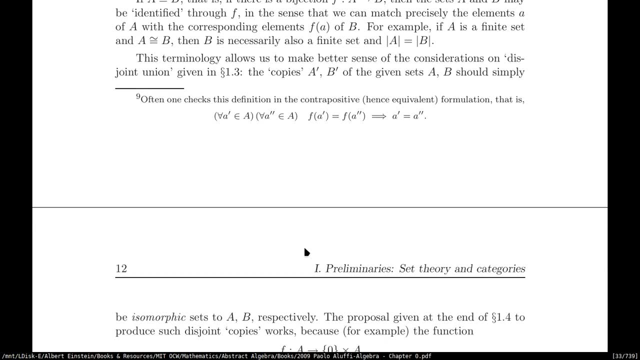 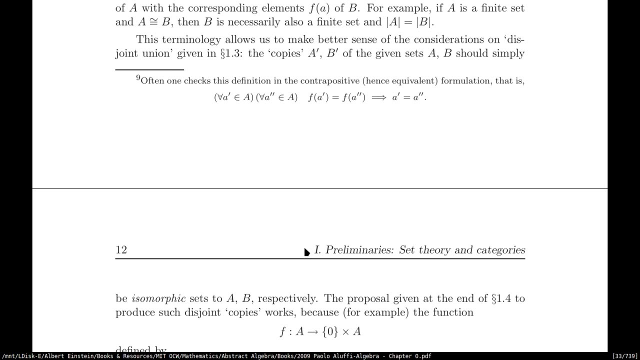 Okay, yeah, okay, you know what, Once we go through this, we might have some time to discuss about. the Wellke-Wiley equation is an interesting thing, yeah, so I don't want to discard it, just that we can. we should just cover the important thing that we need to in. 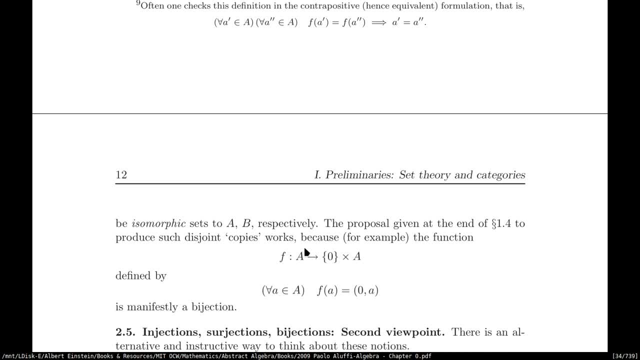 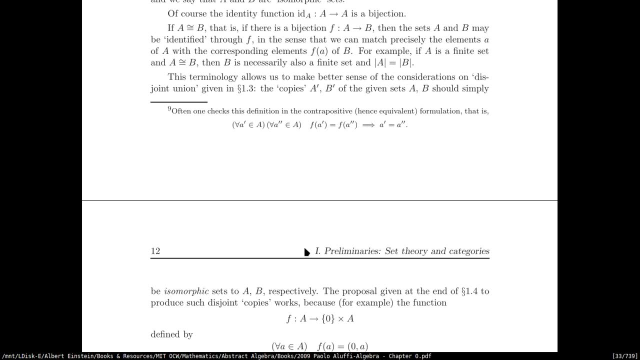 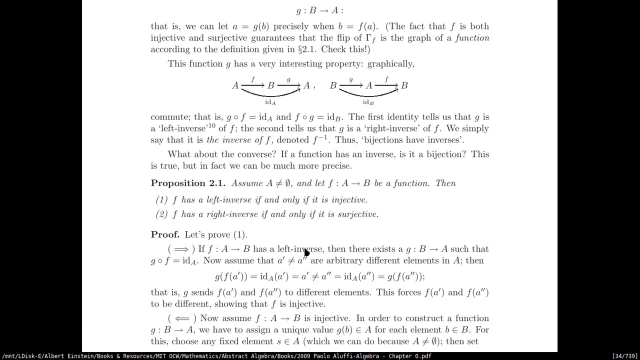 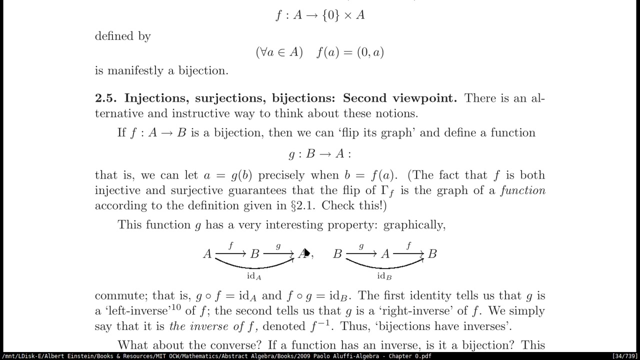 the lecture. okay, so that was about the bigacivity and the, the classification of functions, but we have like a second viewpoint here as well. It's kind of the same thing, but it's in terms of the graph, as we saw before, yeah, and it's kind of interesting. so let's see. So if 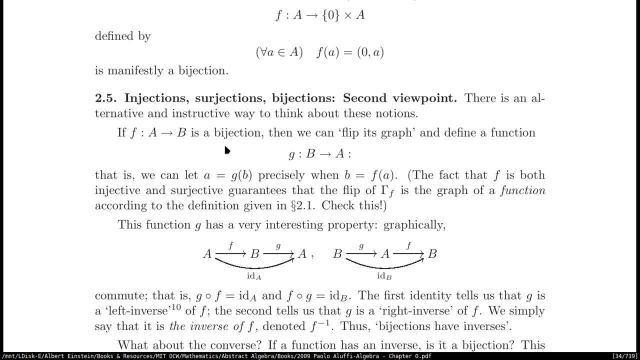 ff is actually a bijection, then we can flip its graph. so flip its graph in the sense that you can like make the codomain its domain and you can like define a function from there. So you have g defined from b to a, that is, and we can let a. 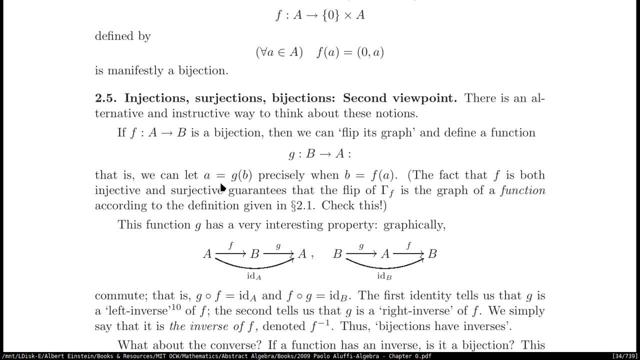 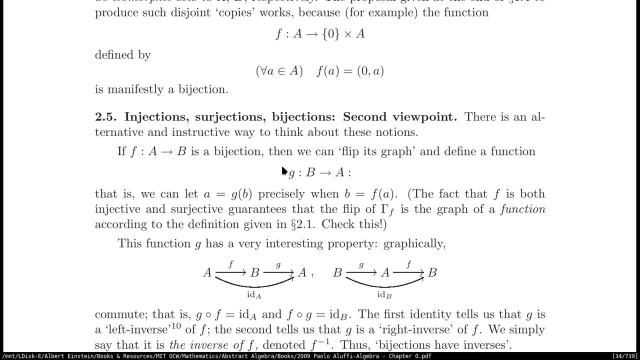 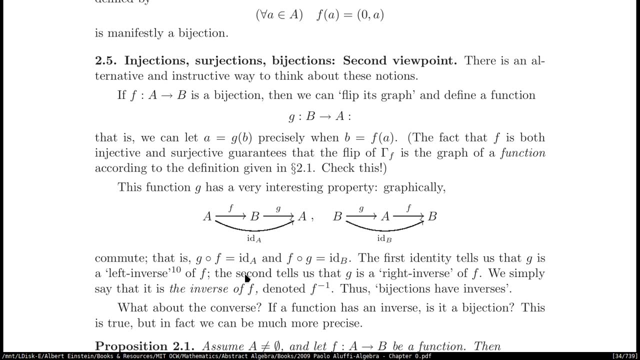 to be g when b is equal to f of x. yeah, so this is like you know, you try to like define a function in the opposite direction and like so that, when you compose it with the original function, you get the identity on each of the sets. 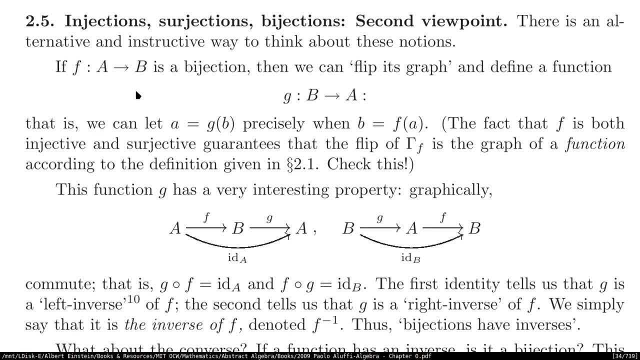 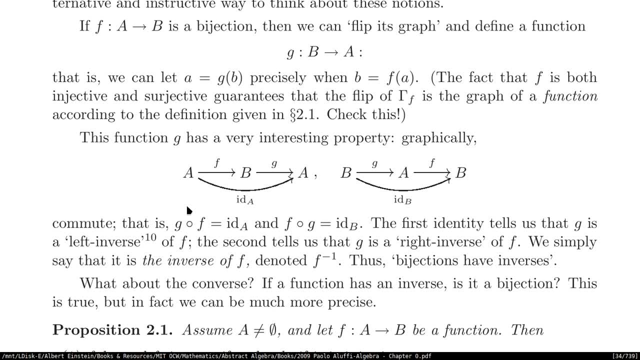 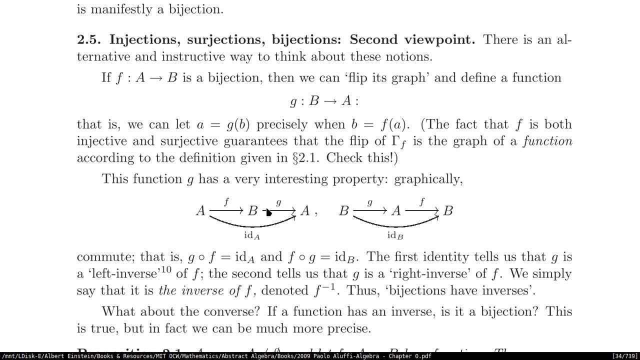 So this is very interesting. So let's see, You have f going from a to b, You have g going from b to a. So if you have a g composition, f right. so g composition, f means g comes first. you do sorry, f comes first, you do f first. 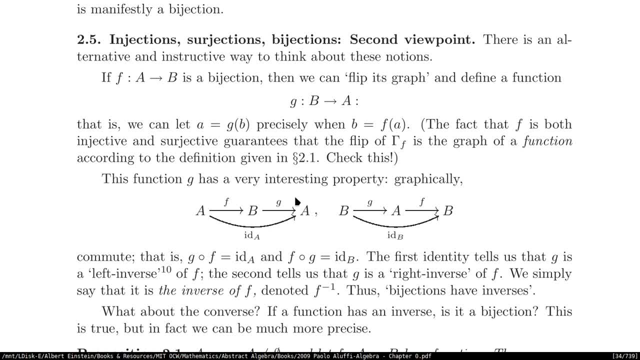 you go from a to b and then you use g to go from b to a right. so when you have g composition f but you end up is at a. so essentially eventually, as f is a bijection um and so is g um, you eventually end up with an identity map, right? 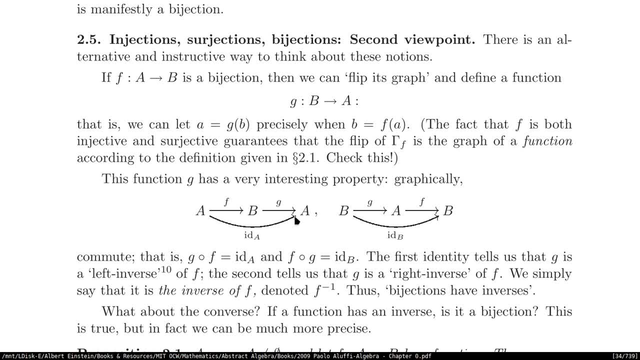 The composition of these two maps gives you the identity function that maps the same element in A to the same element in A right, And if you change the order of this composition you end up with something similar, right. Then here, you first do G, then you do F. 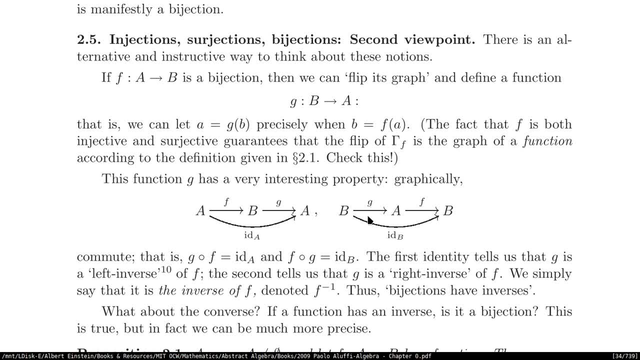 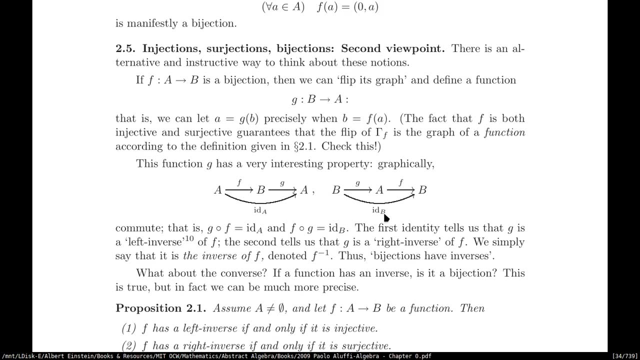 So this is F, composition G, And what this leads to is that you have an identity map over B, right? So yeah, Hello, Killer Whale, Thanks for joining. Would you mind if you can meet your mic, please? Yeah, thanks. 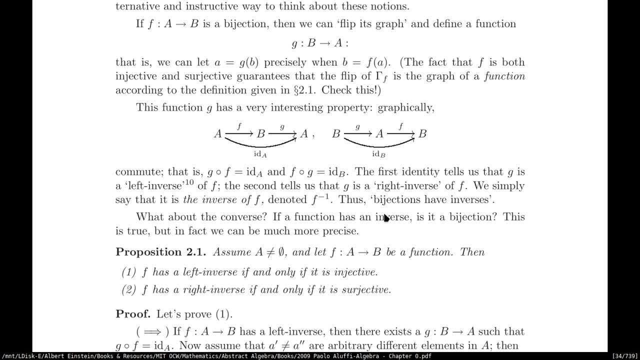 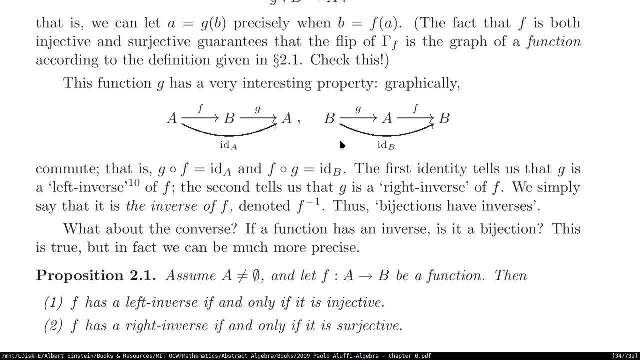 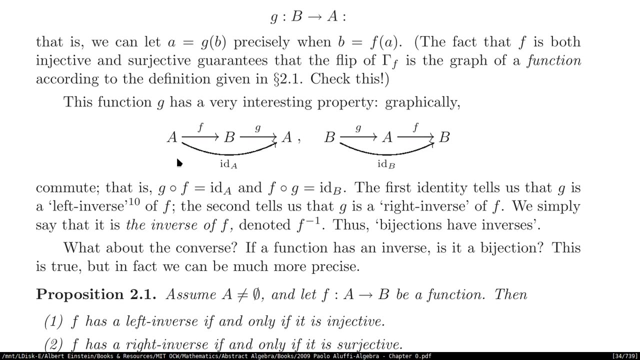 Okay, so, Yeah. so this leads to two interesting things. One is that you can get the identity of these, These two sets, using the composition in two different ways, right? So the first identity, the identity of A, tells that G is the left inverse of F. 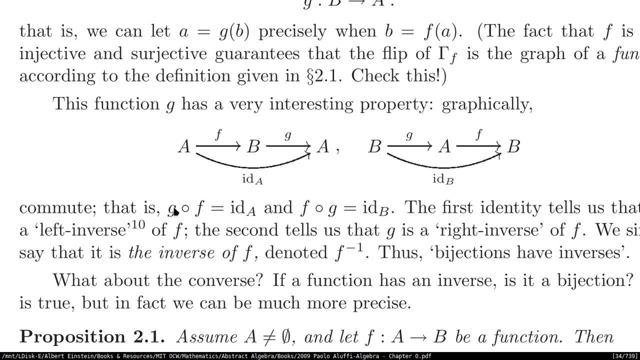 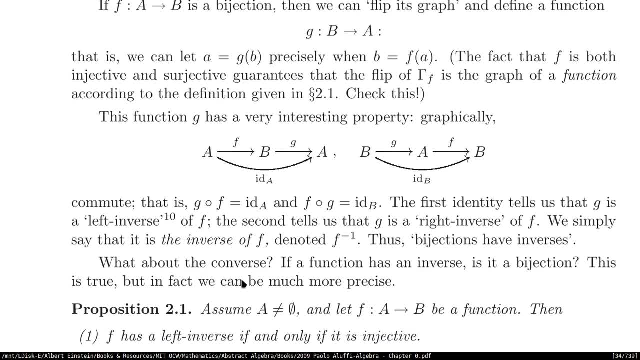 So the left inverse. what it means is that when you can write G on the left side of F and then take the composition, you get the identity right, And the second tells us that G is the right inverse of F. So like, do you even use the composition? 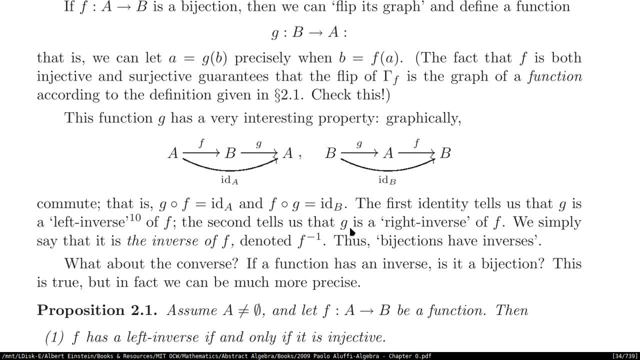 You can write G on the right side, you get the identity too, and what this means is that, like, G is the inverse of F. If it's also right inverse and it's also left inverse, then it's actually the inverse of F, written as F to the minus 1.. 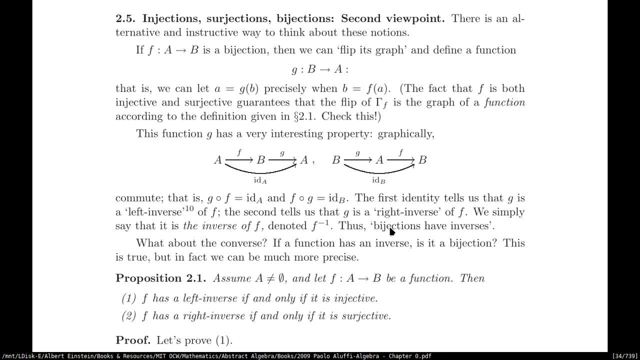 And thus we can say that bijections always have inverses. This is not really like a strict proof, but you can do something with it and then you can prove it, that every time you have a bijection, you're always going to get the identity in these two ways, and then they're going to have inverses. 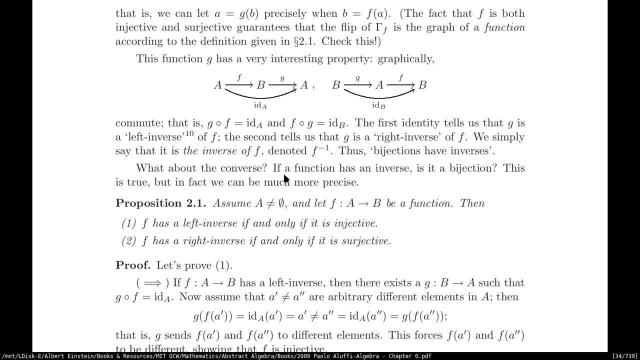 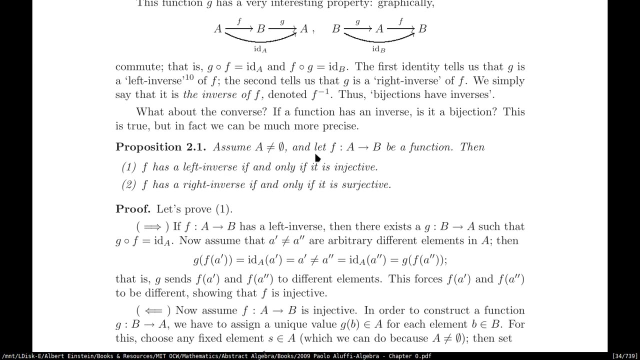 Okay, so what about the converse? If you like, if you have, If a function has an inverse, then does that mean? Does that mean it's a bijection? Not really, And this is how it is. So assume that A is not the null side of A and F goes from A to B as a function. 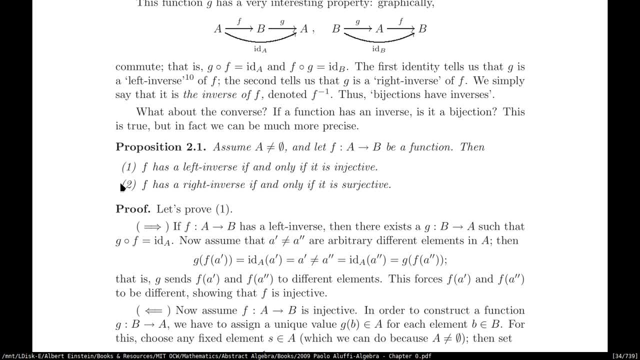 So then you have two propositions right. The first one is that F has a left inverse if, and only if, it is injective. If F is injective, then it has a left inverse, And if it is, If it has an inverse, then it has an inverse. 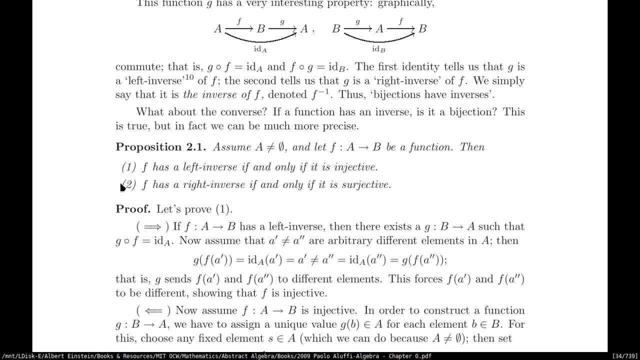 If it has a left inverse, then it is injective. If, and only if, is like a two-sided equivalence, The same for right inverse, except for subjectivity. So if you have a subjectivity, then you have the right inverse. 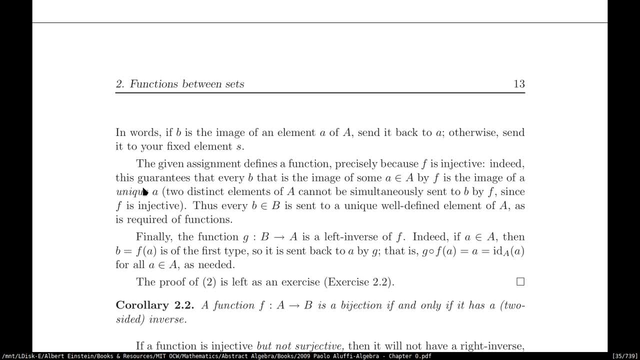 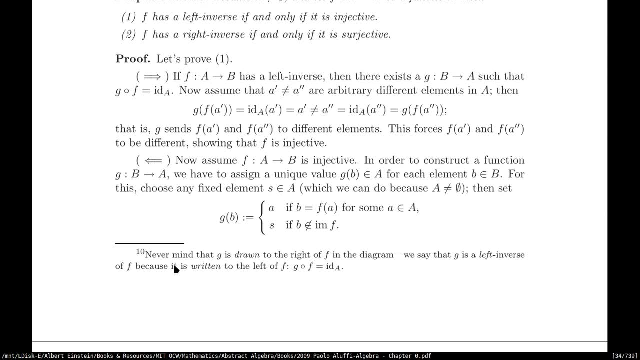 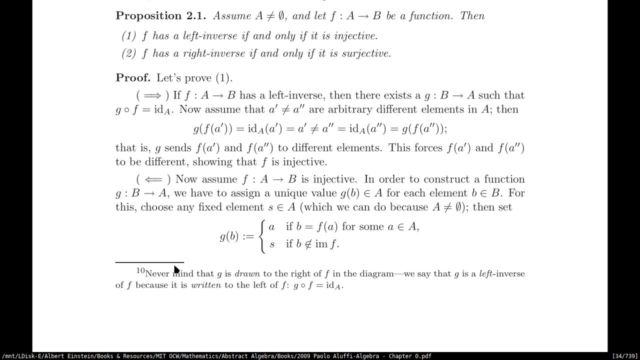 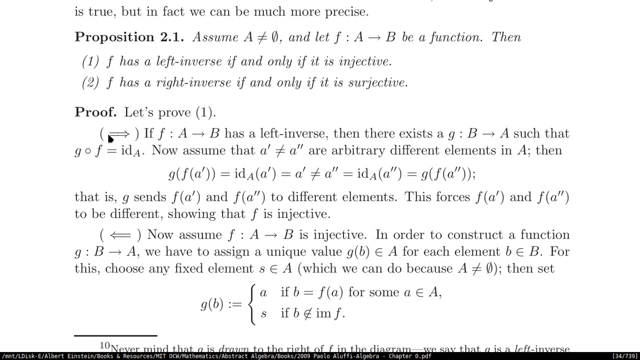 So now he goes on to prove these two things. Essentially he does the first one and I believe he does it quite Regulously. But yeah, let's go through. you know pretty quickly. So again, like every if, and only if statement, you have to prove both directions. 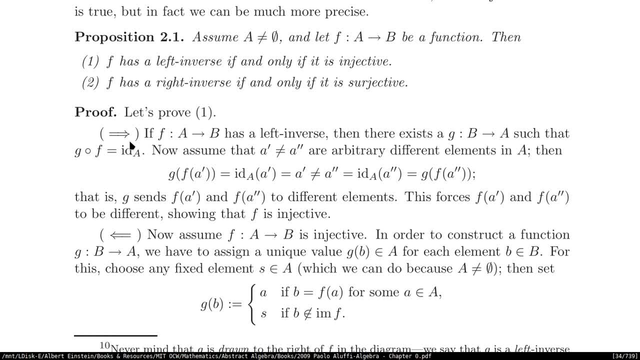 So the first direction, the implication in the, you know, from having a left inverse to being injective. So if F has a left inverse, then Right. So then there exists a G from B to A. It's such that G gives you the identity on A. 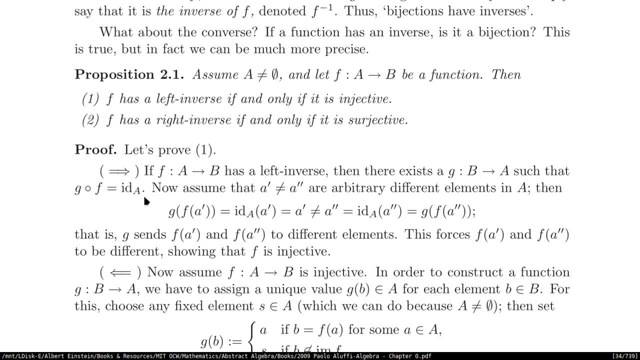 Right, And that's what we just defined here. Now assume that you know like A' and A'' are two like distinct elements in A Right. So what you do is you apply this G to these two elements and you're going to see that. 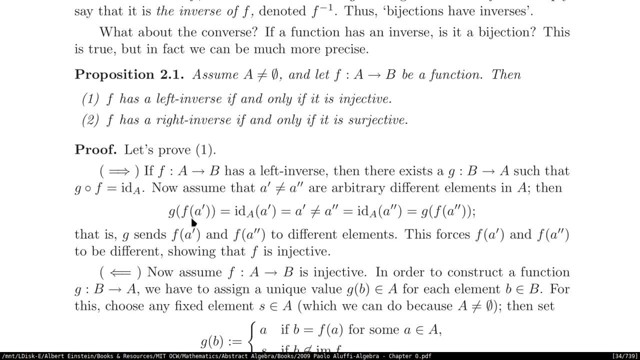 like G, of F, of A' gives you the identity of A', which is A' itself and the same for A'''. So the point is that, like when you apply the function on two different elements, you always get two different images. 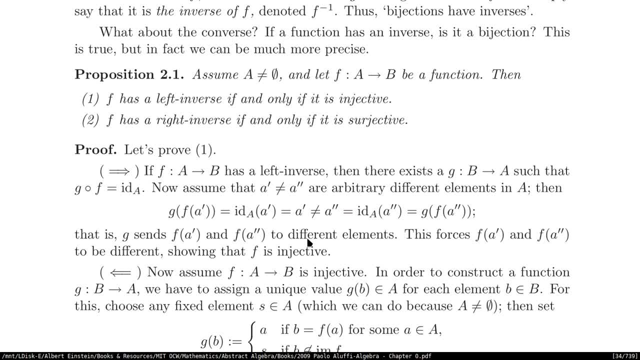 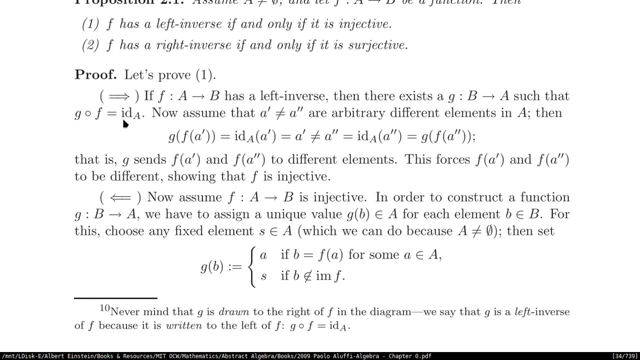 Right- And that's the definition of injectivity- that different elements get mapped to different elements in the image Right. So that makes it That's like halfway through the proof. Now the other direction is when F is in. 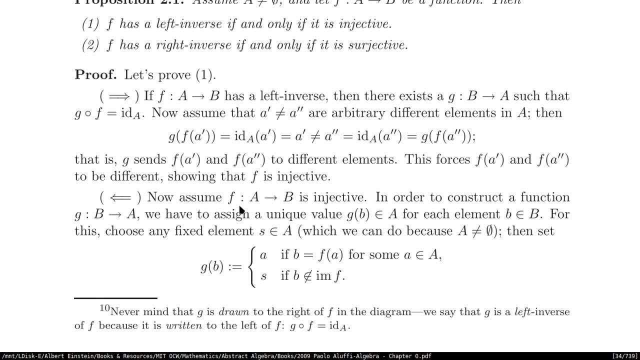 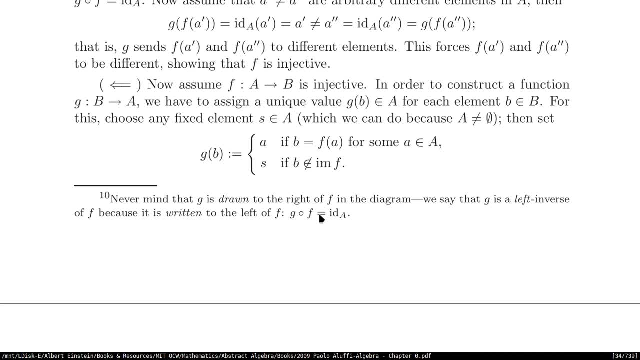 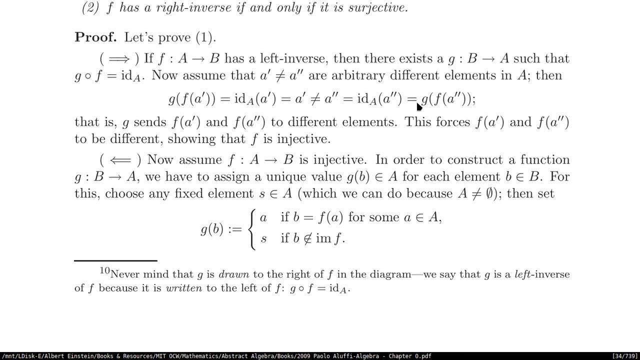 We assume that F is injective, then we have to show that it has a left inverse. Now this is kind of a bit lengthy, but let's see. So yeah, All right. So we have to first construct a function. 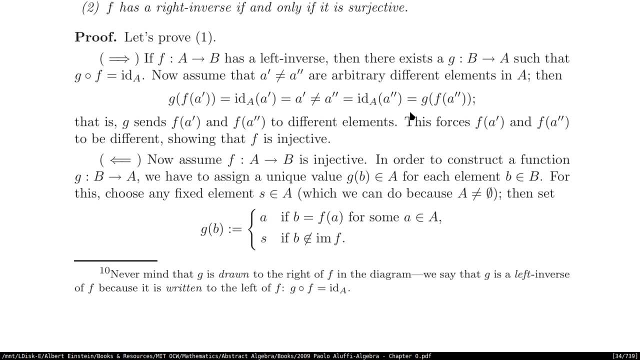 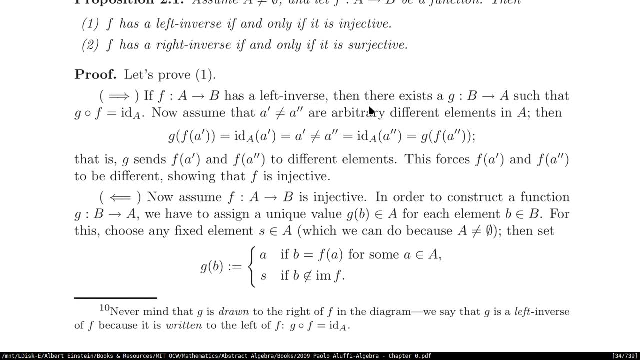 Right, And then show that when we compose it with F on the right side- Sorry, on the left side- we get the identity. Okay, So right. So again, by definition, a function must have a unique G of B, the image for each element. 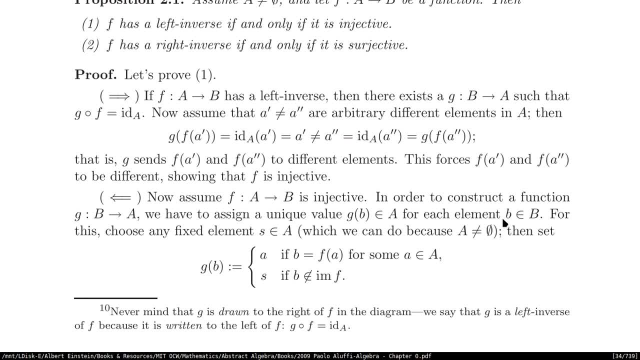 Right For this. choose any fixed element as Yep. Okay, Then set G of B to be A if B is equal to F of A. Right? So if G of B is like you- define it as a function, as a piecewise function, it gives you A when B is the image of F of A. 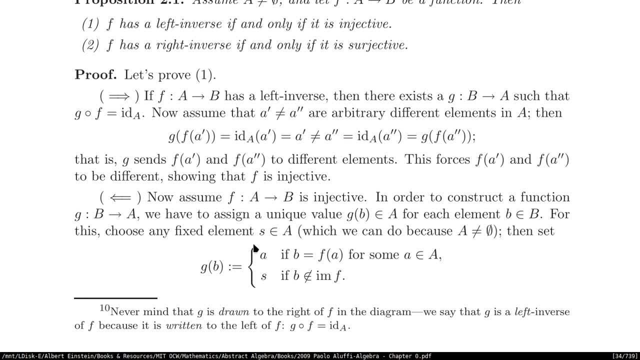 Right. So if G of B is like you define it as a function, as a piecewise function, it gives you A when B is the image of F, of A Right For some element of the set A. Or it gives you S if B is not at all in the image of F. 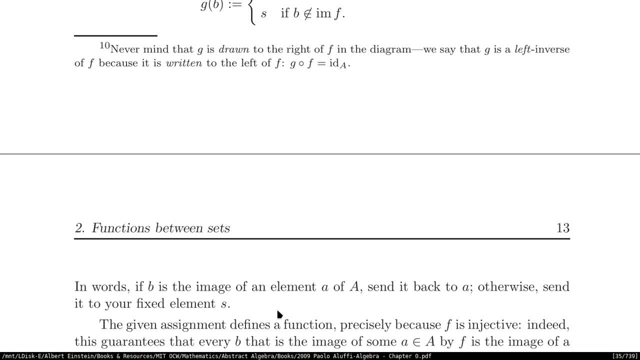 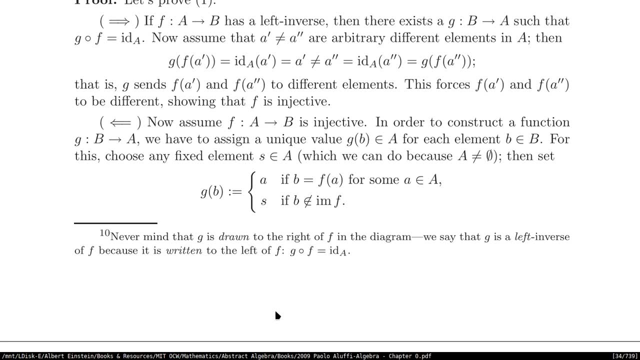 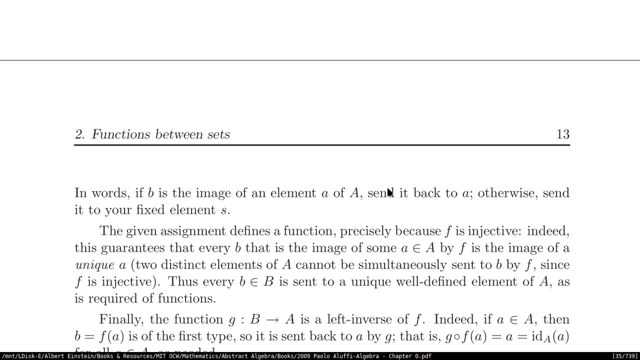 Right Now, what we are going to show is that, like it is indeed the first case, Let's see So. in other words, if B is the image of an element of A, send it back to A. Yeah, 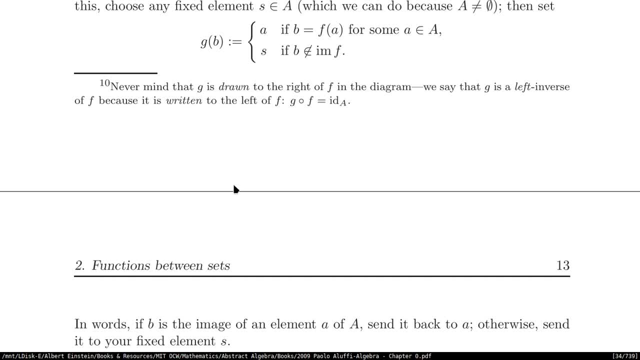 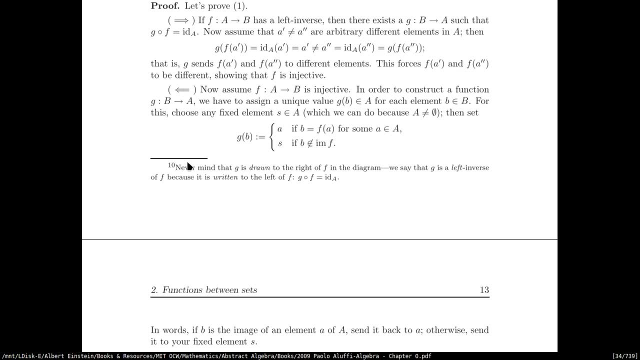 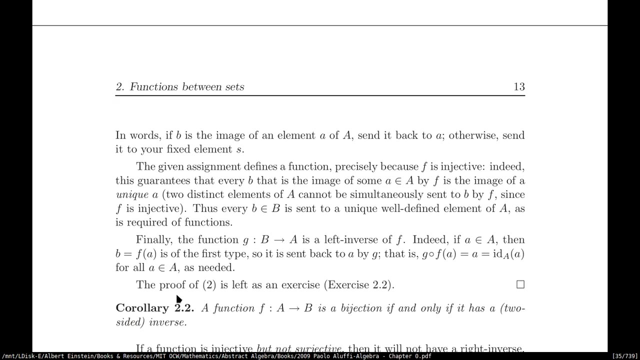 Otherwise, send it to your fixed element. S Yeah, It gives you A if you have some image. If you don't, then you just go back to the fixed element that you picked. Right, Okay, So So this is actually a definable. 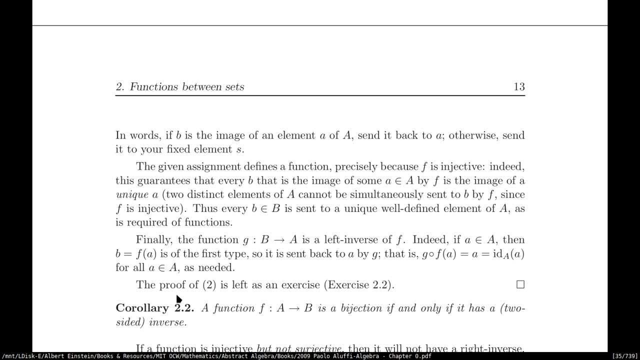 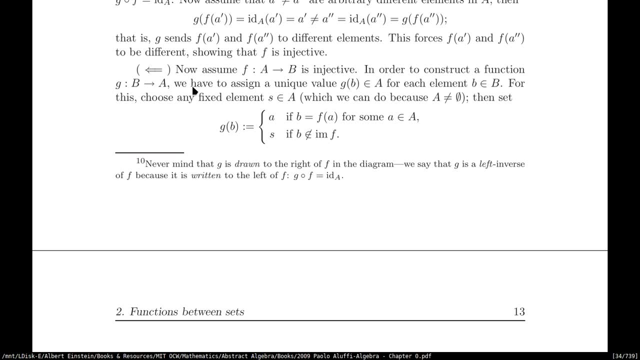 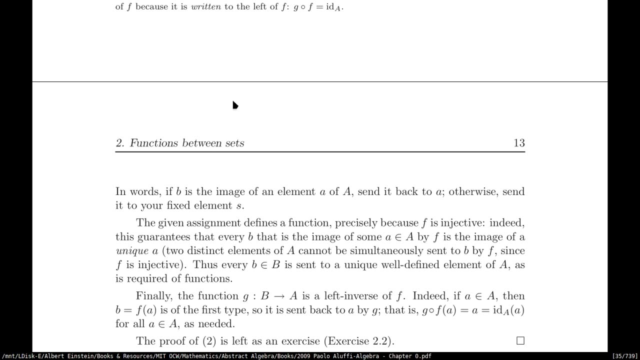 A defined function, Right Um And F. Um Is Um Injective, Right F is injective, So we can like actually have um, like different elements separately mapped to different things. So this guarantees that every B that is the image of some, A by F is the image of a unique. 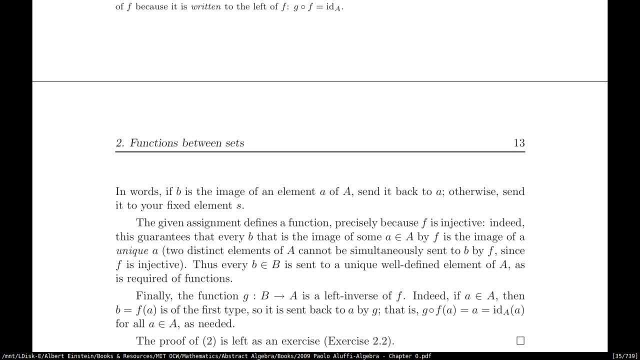 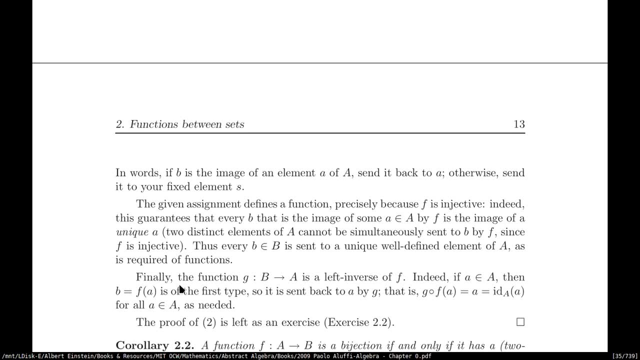 A. Right, So like you have unique elements mapped to unique elements, Okay, Mm-hmm. So So what this says is that, um, every B is sent to a unique, well-defined element of A, as is required of functions because of injectivity of F and because, you know, G is actually. 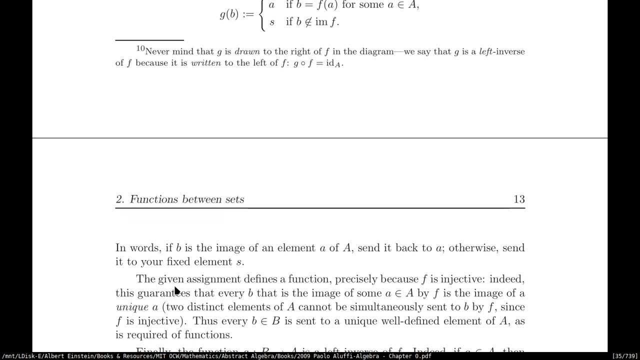 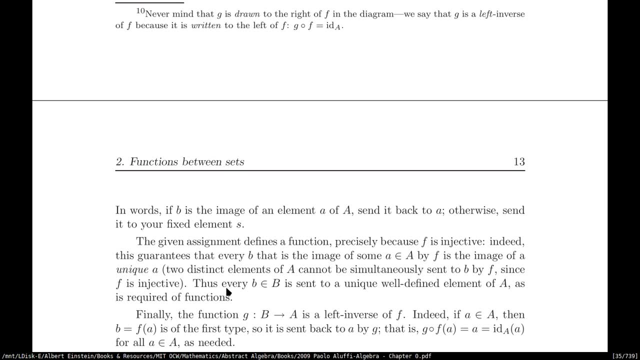 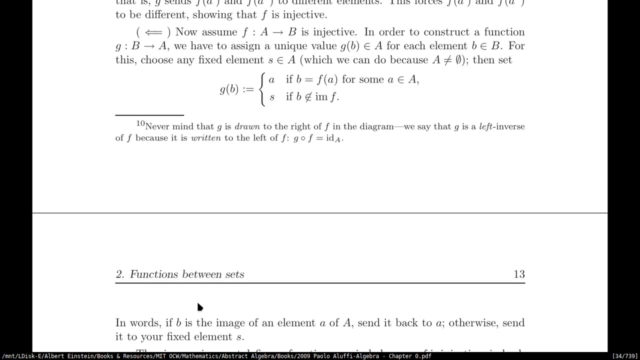 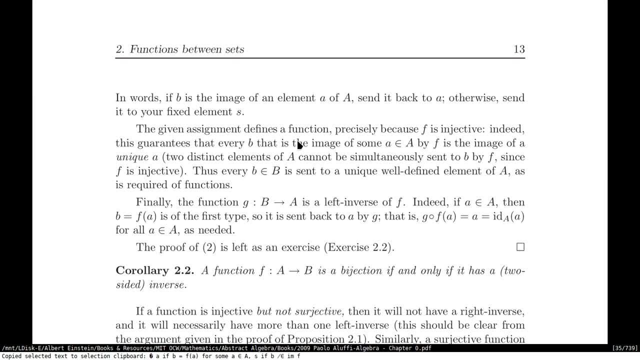 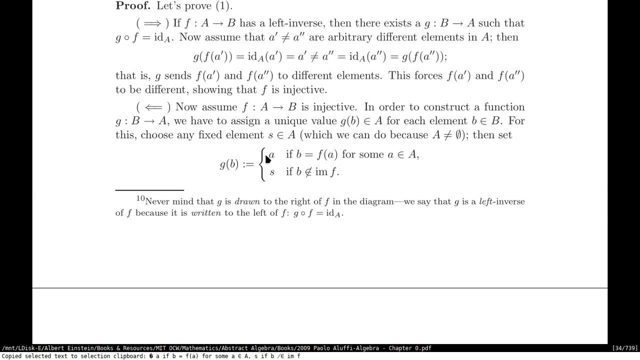 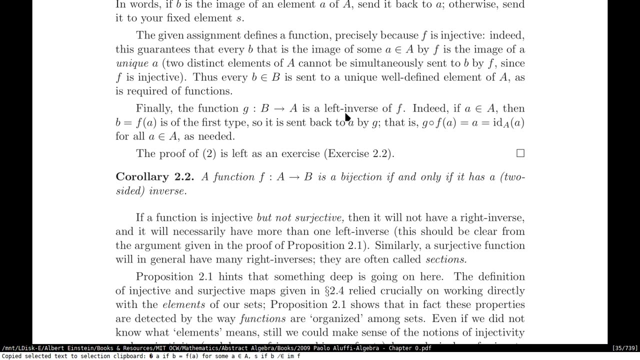 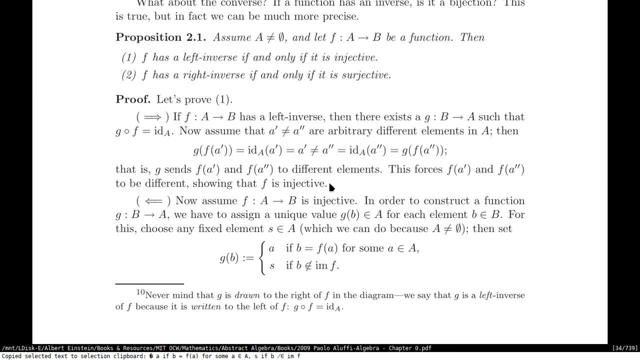 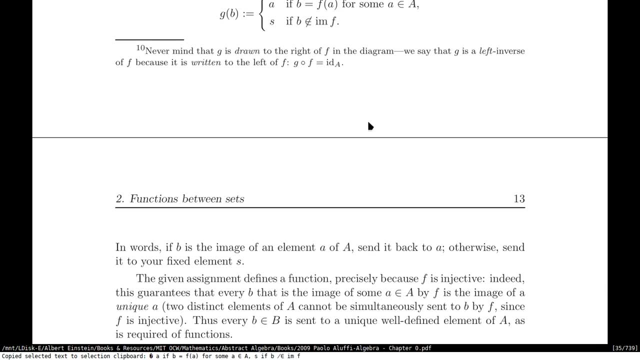 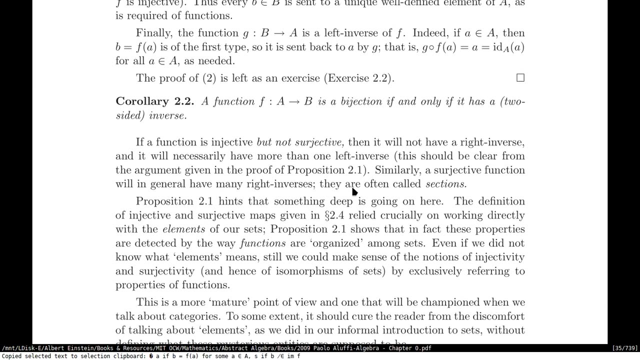 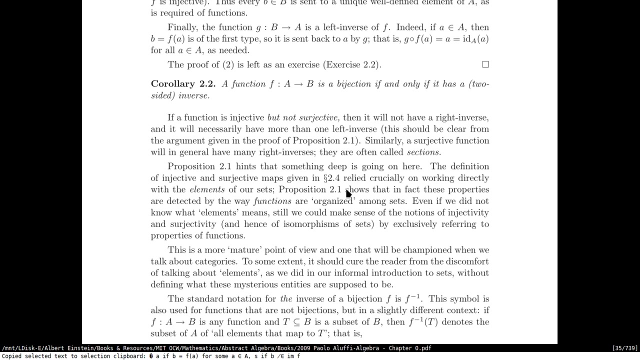 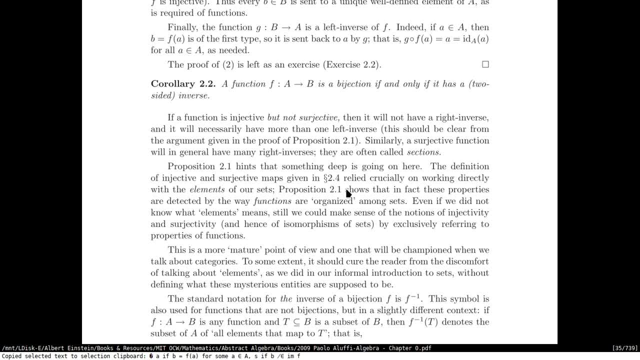 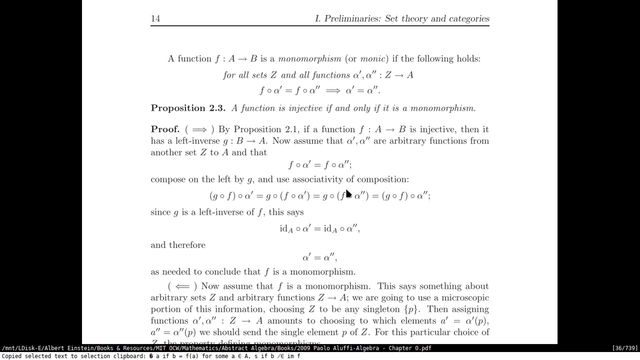 and only if it has a two-sided inverse. so you have a two-sided inverse in the sense that, like if F and F, if G is an inverse of F, then F is also an inverse of G. so that's two-sided inverses and we're going to see more of that, but we 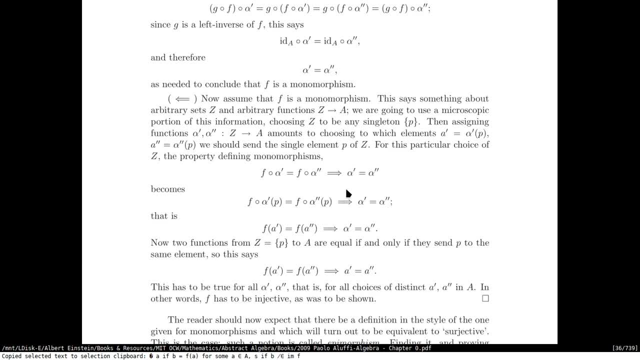 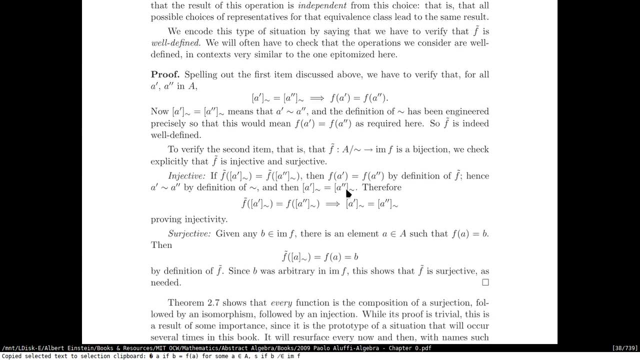 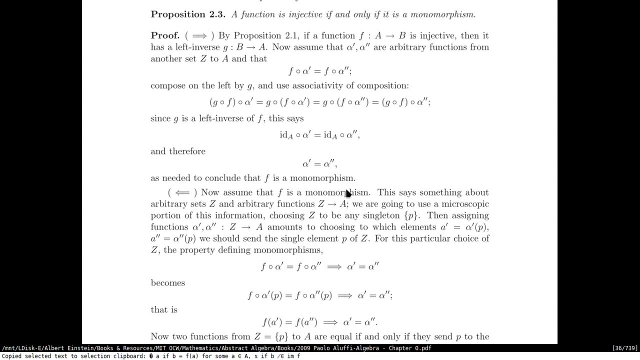 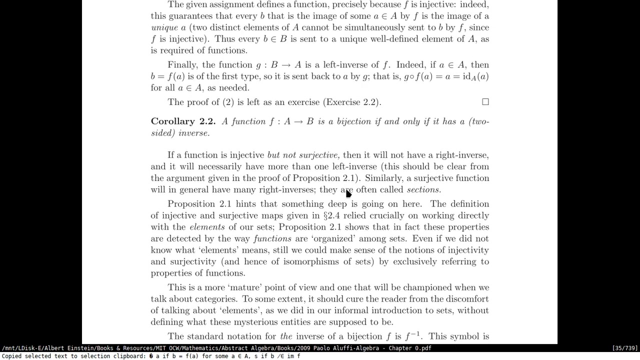 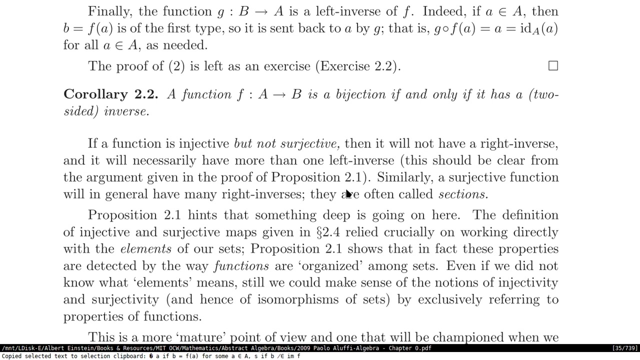 have this proposition, which is like pretty long. I don't think we'll be able to cover that, but yeah, okay, so let's see about this color. so okay, so, let's see about this color. so okay, so, let's see about this color. so, if a function is injective but not, 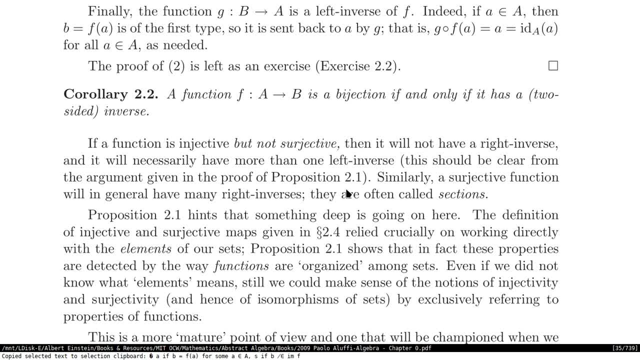 if a function is injective but not, if a function is injective but not subjective, and then it will not have our subjective, and then it will not have our subjective, and then it will not have our right. inverse right, so it's just right. inverse right, so it's just. 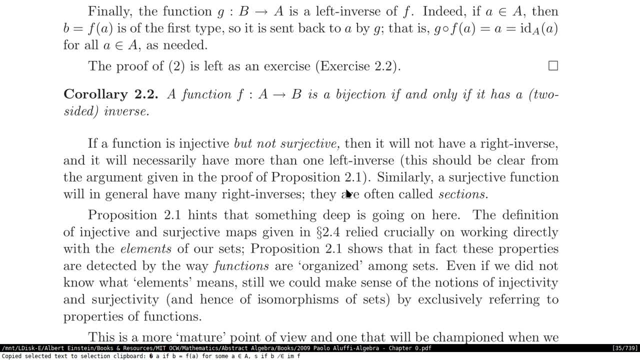 right inverse. right, so it's just injective. then it has a left inverse, but injective, then it has a left inverse, but injective, then it has a left inverse. but this says nothing about the right inverse. this says nothing about the right inverse. this says nothing about the right inverse. it will never have a right. 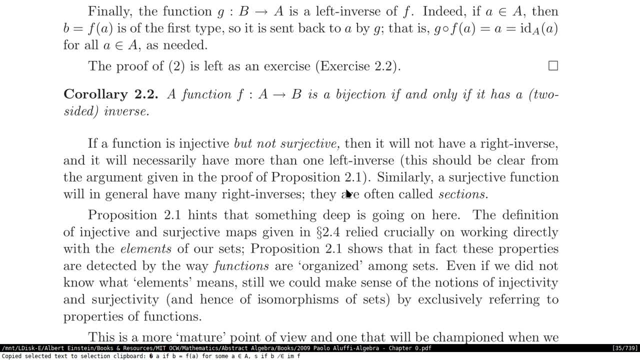 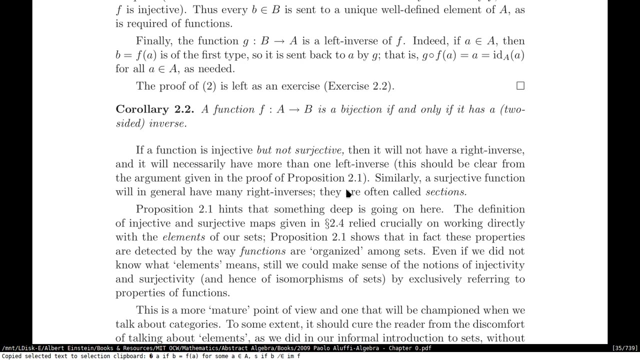 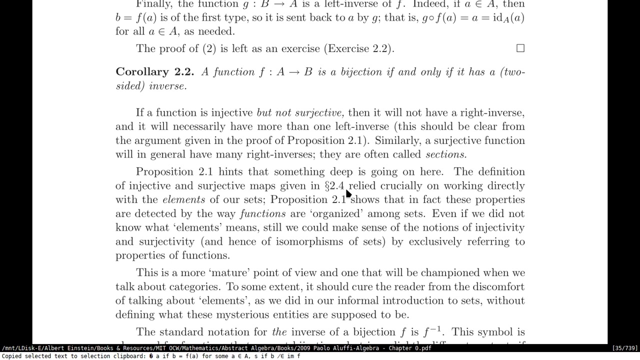 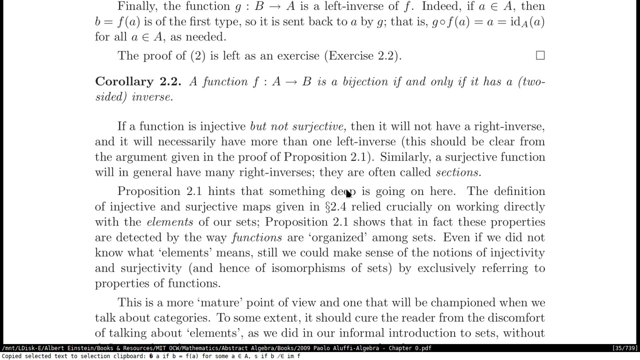 it will never have a right, it will never have a right. inverse actually, mm-hmm. similarly a subjective function will. similarly a subjective function will, similarly a subjective function will have have, have, have that have sorry sections at the right, that have sorry sections at the right, that have sorry sections at the right. inverses of subjective functions. yeah. 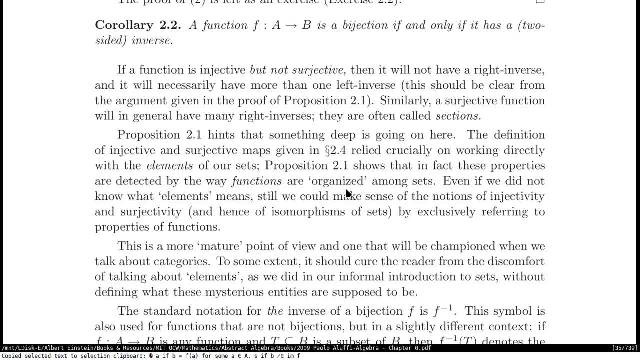 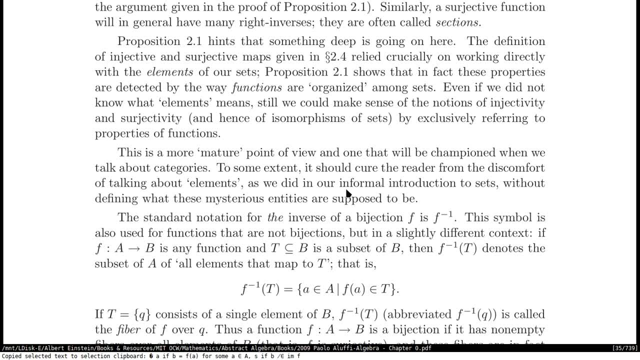 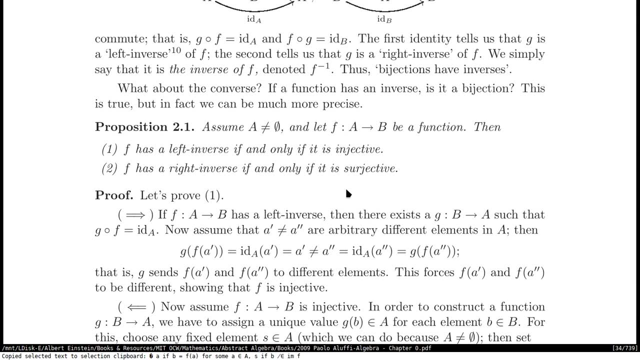 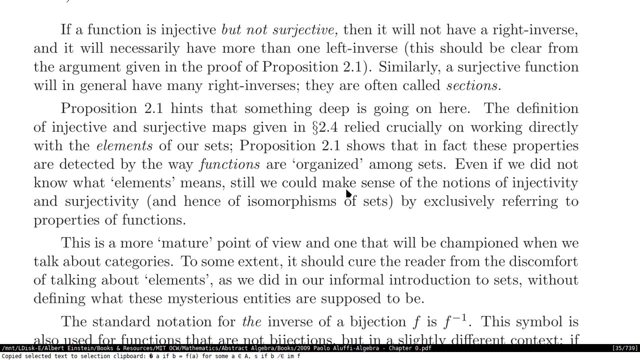 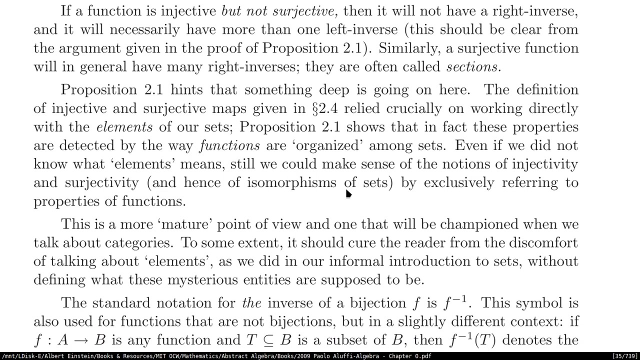 inverses of subjective functions. yeah, inverses of subjective functions. yeah, okay, okay, okay, right, so yeah. so this and this, right, so yeah, so this and this, right, so yeah. so this and this proposition that we just saw, which you, proposition that we just saw, which you. 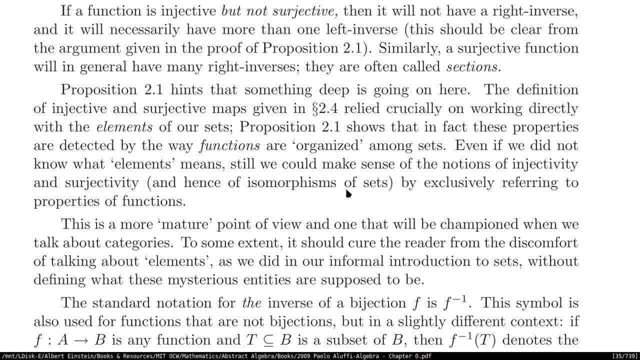 proposition that we just saw, which you know said about like left inverses with. know said about like left inverses with. know said about like left inverses with injectivity and right inverses with injectivity and right inverses with injectivity and right inverses with subjectivity, what that allows that you 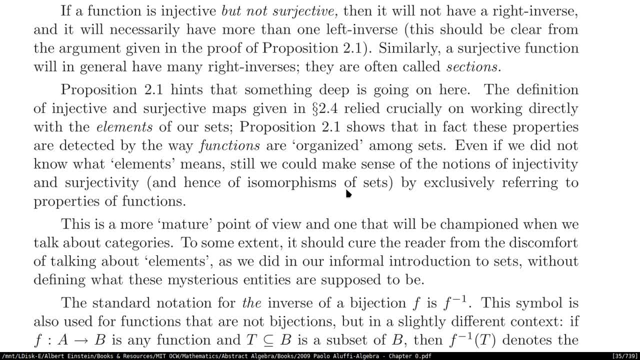 subjectivity, what that allows that you subjectivity, what that allows that you know it. it allows us to know it. it allows us to know it. it allows us to like, like, even if we don't know what's like, like, even if we don't know what's. 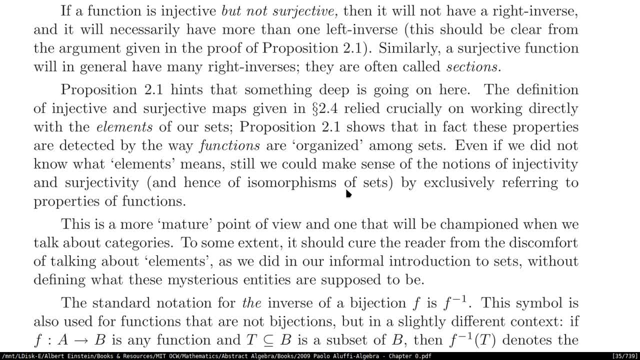 like, like, even if we don't know what's happening- at like in the elementary, happening at like in the elementary, happening at like in the elementary level. like knowing what element is mapped level, like knowing what element is mapped level, like knowing what element is mapped to which element. we can know about the. 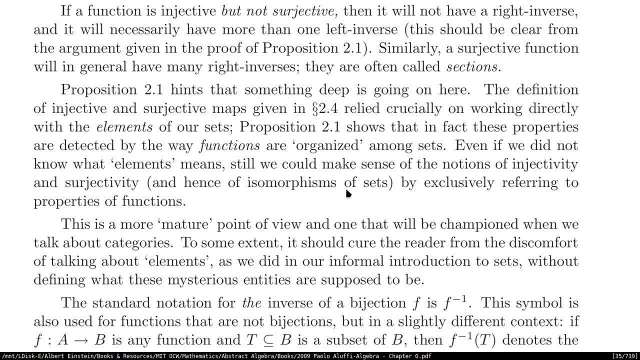 to which element we can know about the? to which element we can know about the properties of the those elements? right properties of the those elements, right properties of the those elements. right, so, yeah, that's what he says, even if we so yeah, that's what he says, even if we. 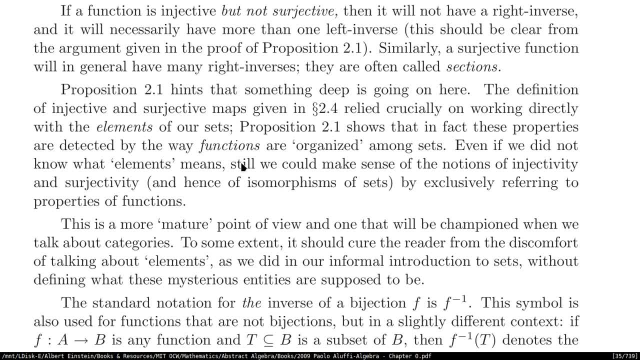 so, yeah, that's what he says. even if we did not know what elements means, still did not know what elements means, still did not know what elements means, still we could make sense of the notions of, we could make sense of the notions of, we could make sense of the notions of injectivity. right, those are that, that's. 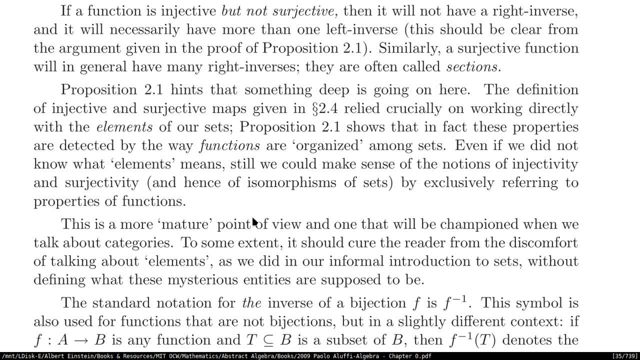 injectivity right. those are that that's injectivity right. those are that. that's the property prop. that's the property of the property prop. that's the property of the property prop. that's the property of the sense right by exclusively referring the sense right. by exclusively referring. 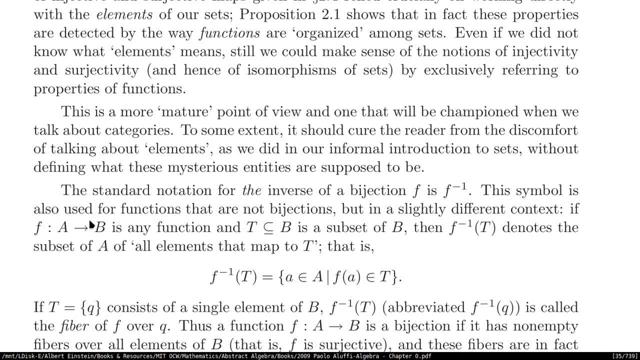 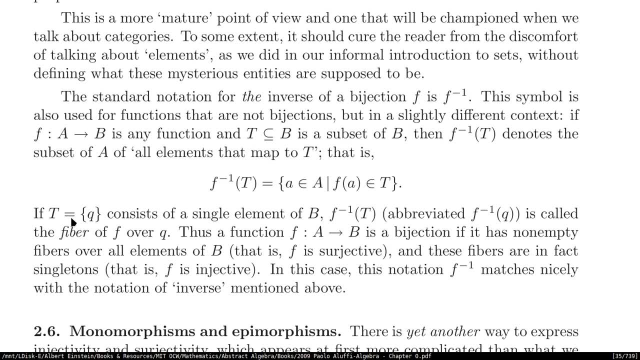 the sense right, by exclusively referring to the properties of the functions, so to the properties of the functions, so to the properties of the functions. so, yeah, and this is going to be something. yeah, and this is going to be something. yeah, and this is going to be something that we'll see in categories. 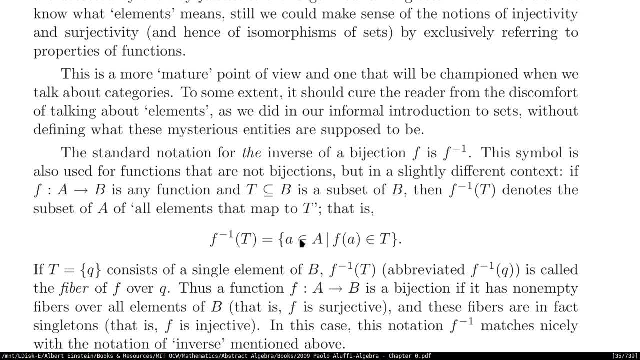 yeah, so this here is can be a bit. yeah, so this here is can be a bit. yeah, so this here is can be a bit confusing. so the inverse of a bijection confusing. so the inverse of a bijection confusing. so the inverse of a bijection is F to the minus 1. right, but we have 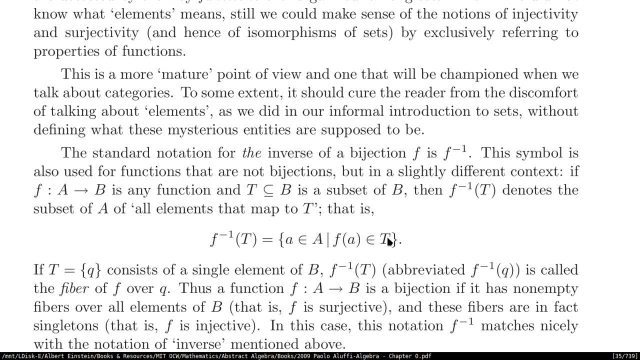 is F to the minus 1 right, but we have is F to the minus 1 right, but we have something else which looks similar, but something else which looks similar, but something else which looks similar, but it's not the same thing. so if F is a, 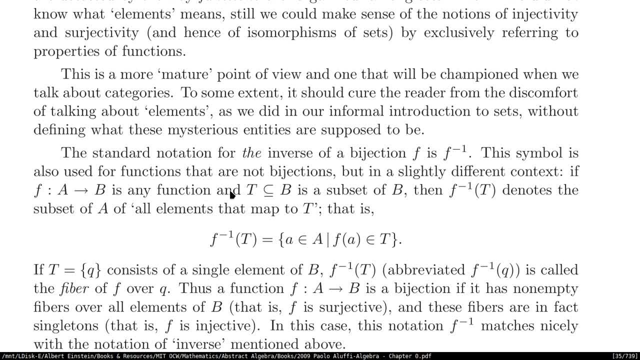 it's not the same thing. so if F is a, it's not the same thing. so if F is a function, any function doesn't have to be function. any function doesn't have to be function. any function doesn't have to be objective and you have a subset of B. 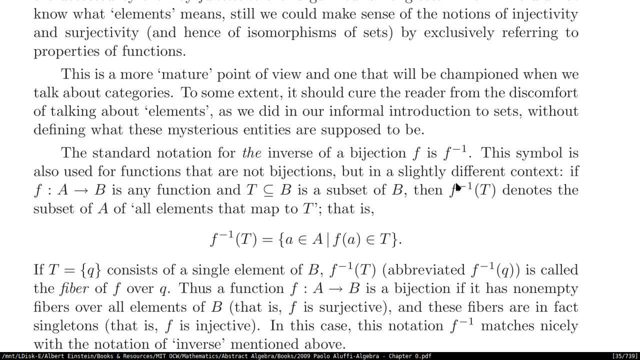 objective and you have a subset of B objective and you have a subset of B. that is T then F to the minus 1 of T. that is T then F to the minus 1 of T. that is T then F to the minus 1 of T. this is read as the pre-image of T. 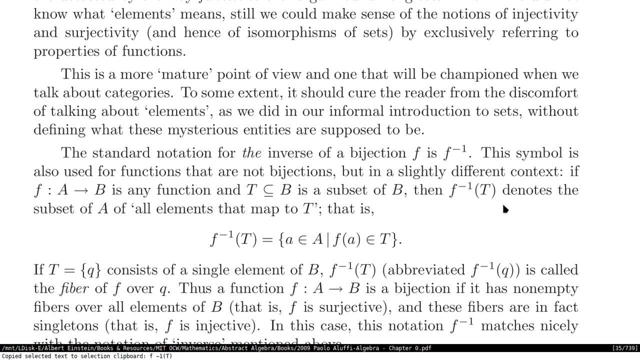 this is read as the pre-image of T. this is read as the pre-image of T under F right, and that denotes all the under F right and that denotes all the under F right. and that denotes all the elements from a sorry, all the elements. elements from a sorry: all the elements. 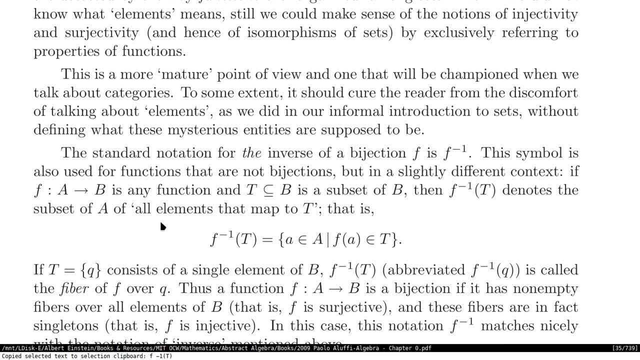 elements from a- sorry, all the elements, yeah- of a that are mapped to T- that's yeah- of a that are mapped to T- that's yeah- of a that are mapped to T. that's the pre image, and, apart from being the pre image and apart from being 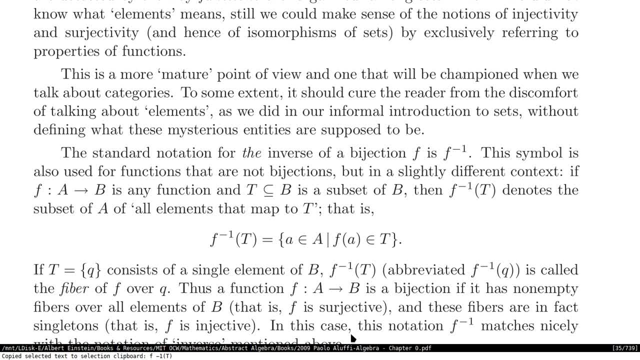 the pre image and apart from being called pre pre image, called pre pre image, called pre pre image, like, if you're like considering, like, like, if you're like considering, like, like, if you're like considering like pre images of like specific points, then pre images of like specific points, then 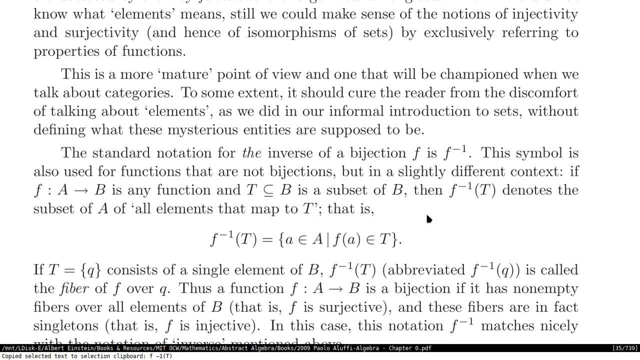 pre images of like specific points. then those are called academic fibers. this, those are called academic fibers. this, those are called academic fibers. this again comes up in algebra topology and again comes up in algebra topology and again comes up in algebra topology and differential geometry. and we're not. 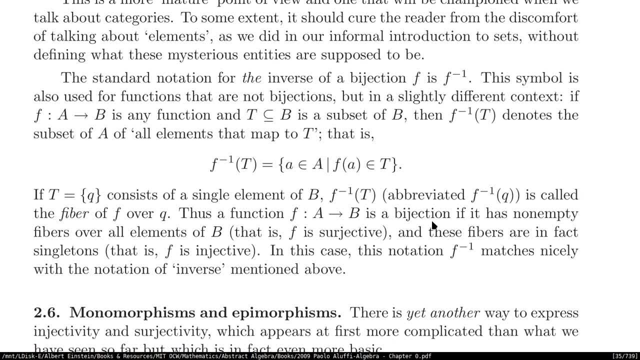 differential geometry and we're not differential geometry and we're not going to. we're going to use it at some going to. we're going to use it at some going to. we're going to use it at some point when we do we do something. point when we do, we do something. 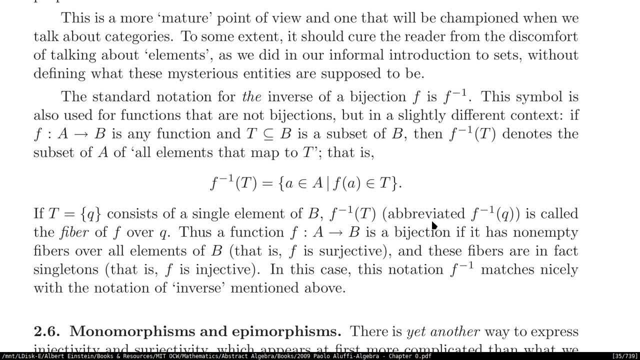 point when we do we do something related to that. but yeah, so these are related to that. but yeah, so these are related to that. but yeah, so these are. like this: is this has nothing to do with. like this is this has nothing to do with. like this is: this has nothing to do with bijectivity or inverses, right, so these? 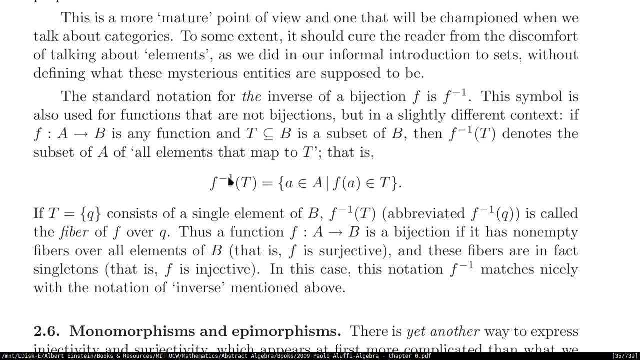 bijectivity or inverses, right so these bijectivity or inverses, right, so these are sets F to the minus 1 of T is a set. are sets F to the minus 1 of T is a set. are sets F to the minus 1 of T is a set which contains the elements that are: 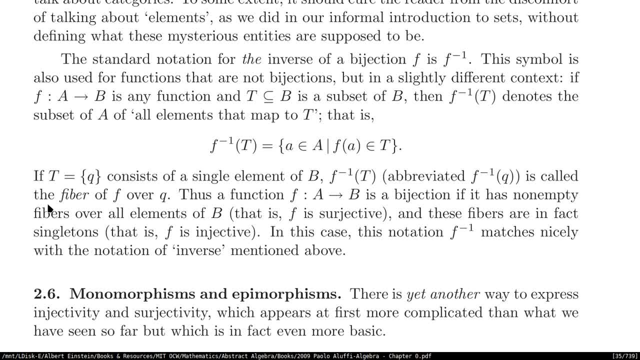 which contains the elements that are. which contains the elements that are mapped to T. the same way if T is just mapped to T, the same way if T is just mapped to T, the same way if T is just singleton containing a single element: singleton containing a single element. 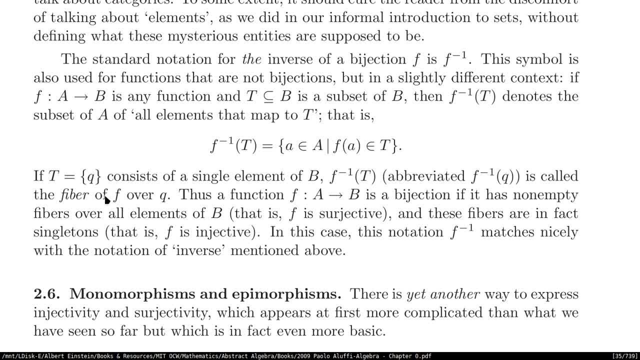 singleton containing a single element, then the pre-image is going to be the, then the pre-image is going to be the, then the pre-image is going to be the fiber of F over Q, fiber of F over Q, fiber of F over Q, mm-hmm, right, so yeah, if you think about. 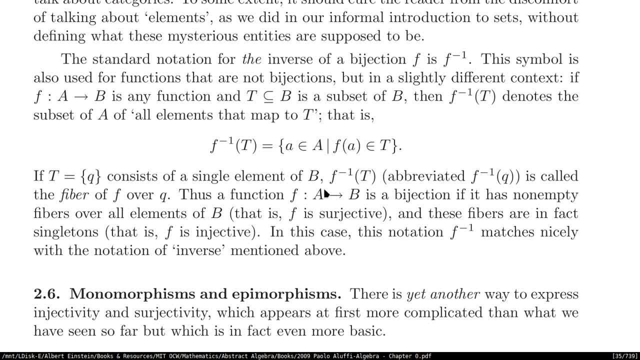 mm-hmm- right, so yeah. if you think about mm-hmm- right, so yeah. if you think about this, if like for F to be a bijection, this, if like for F to be a bijection, this, if like for F to be a bijection like the fibers of all the elements of 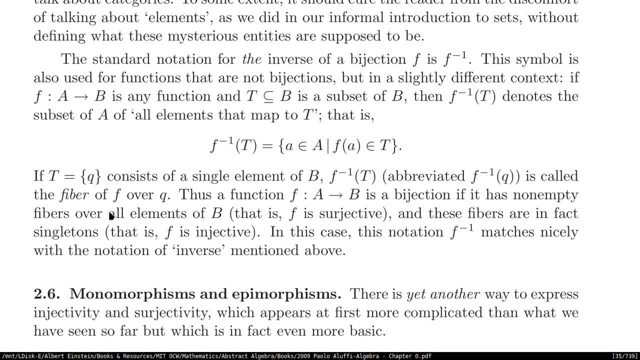 like the fibers of all the elements of, like the fibers of all the elements of B. so if you look at like the pre images B, so if you look at like the pre images B, so if you look at like the pre images of all the elements of B, 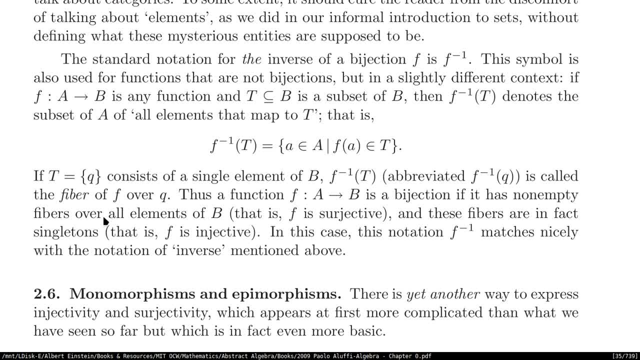 of all the elements of B, of all the elements of B, they are always going to have something in. they are always going to have something in. they are always going to have something in them, right? so something in them that them right, so something in them that them right, so something in them. that means, like something of B is mapped to. 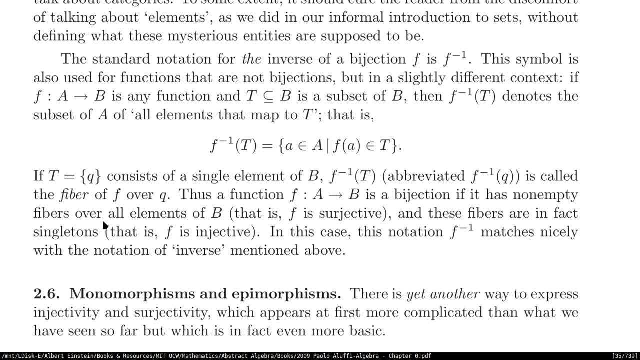 means like something of B is mapped to, means like something of B is mapped to something of a, which is, by definition, something of a, which is, by definition, something of a, which is, by definition, subjectivity and the as its objective it. subjectivity and the as its objective it. 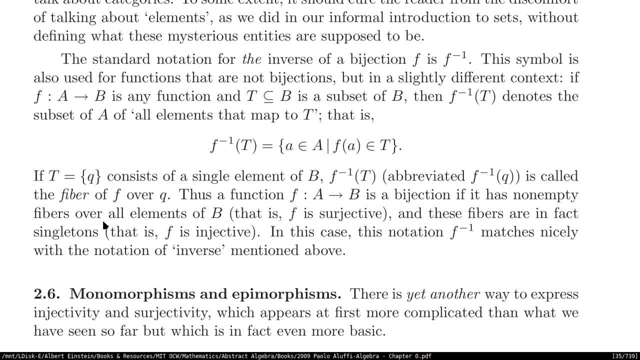 subjectivity and the as its objective. it means that the fibers are actually, means that the fibers are actually, means that the fibers are actually singletons. so like so. the fiber of F singletons, so like so. the fiber of F singletons, so like so the fiber of F over any element of B is actually a. 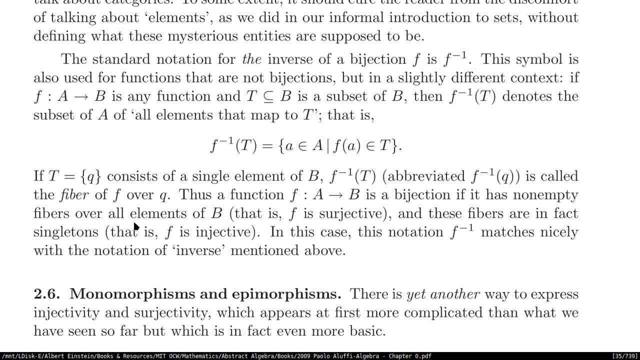 over. any element of B is actually a over. any element of B is actually a singleton, a single element. so that's singleton, a single element. so that's singleton, a single element. so that's injectively that every single element is, injectively that every single element is. 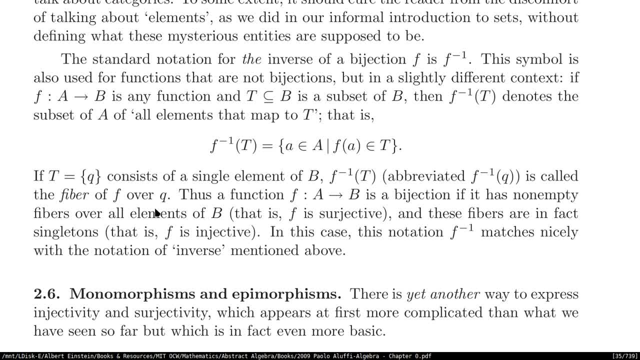 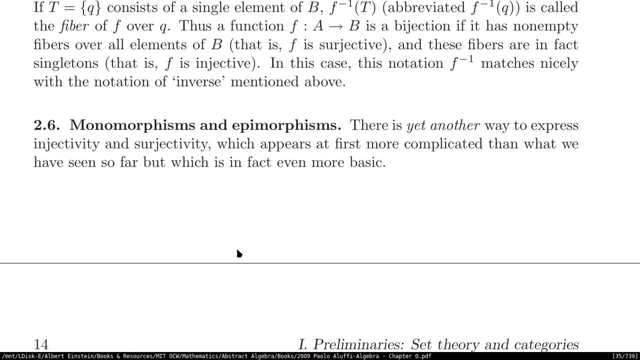 injectively that every single element is mapped to some other single elements, mapped to some other single elements, mapped to some other single elements. this will be one-to-one connection, okay, this will be one-to-one connection, okay, this will be one-to-one connection, okay. and then we have some other. 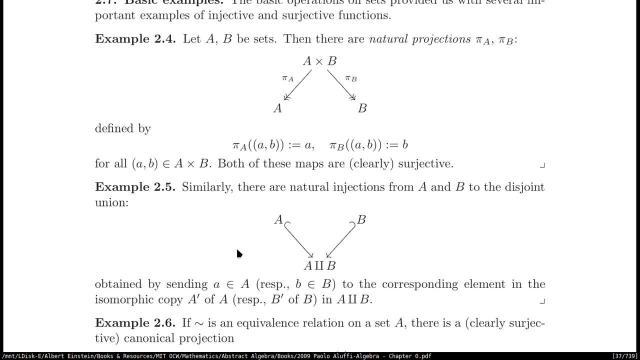 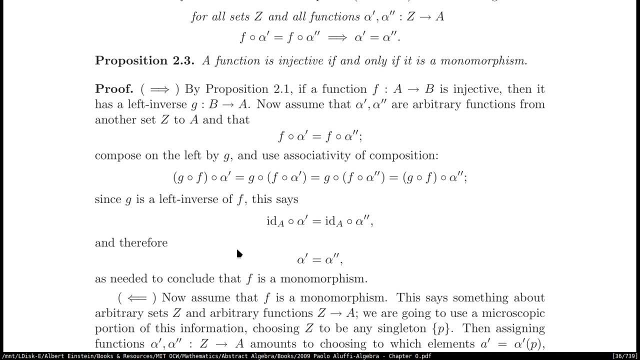 and then we have some other, and then we have some other definitions, and we'll be done for definitions and we'll be done for definitions and we'll be done for today, today, today, I'm let me get some water if you have. I'm let me get some water if you have. 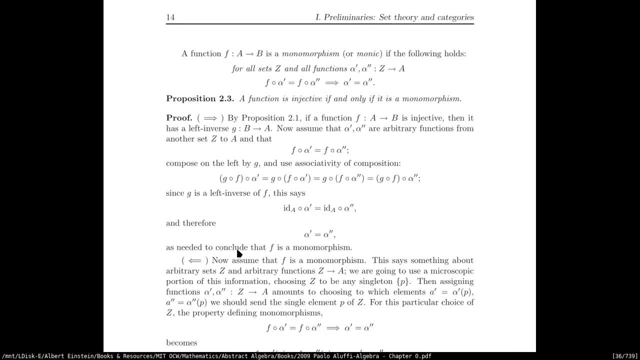 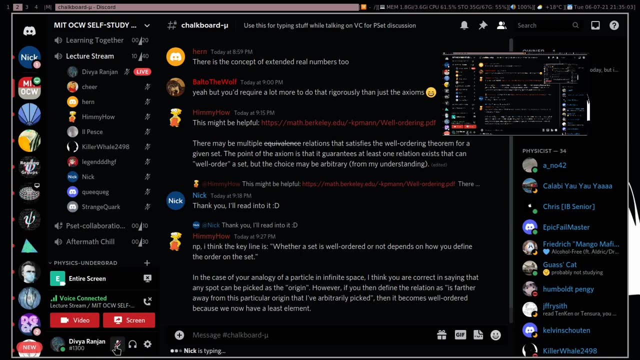 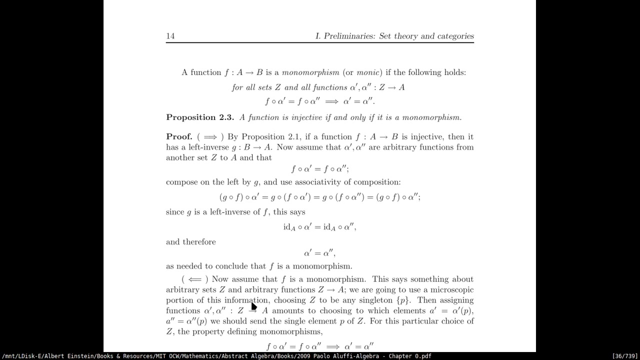 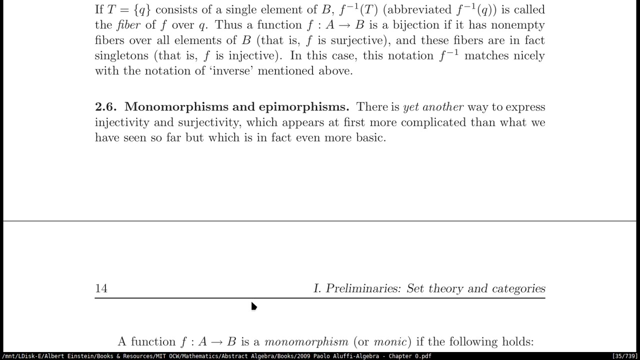 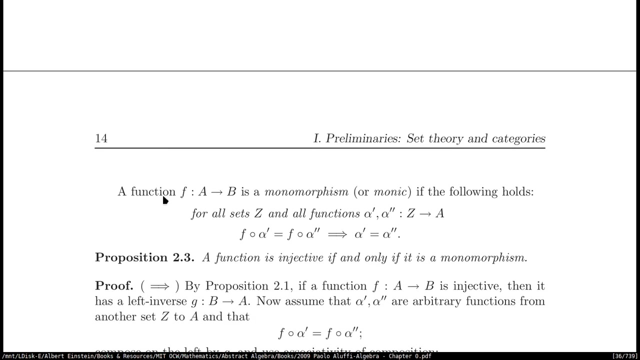 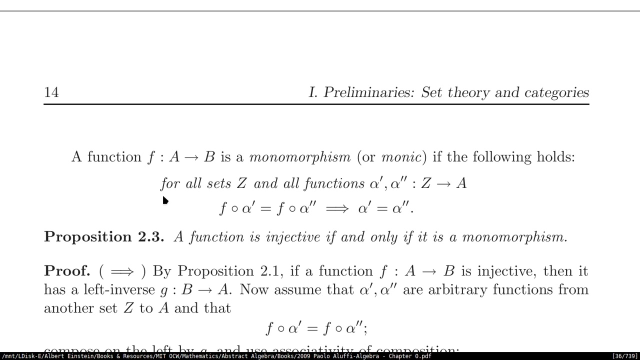 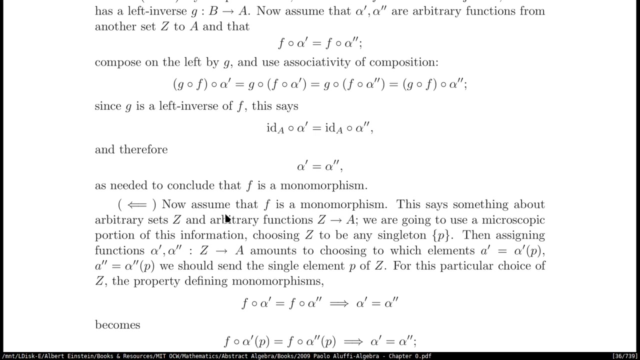 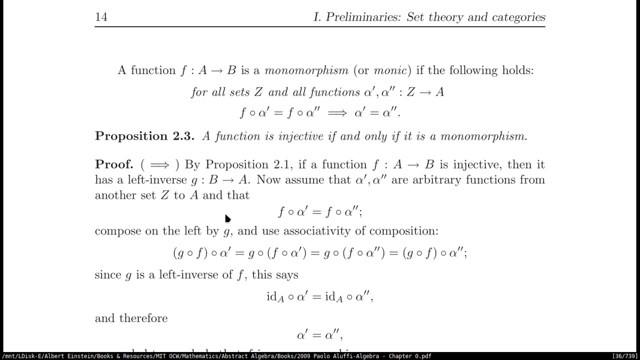 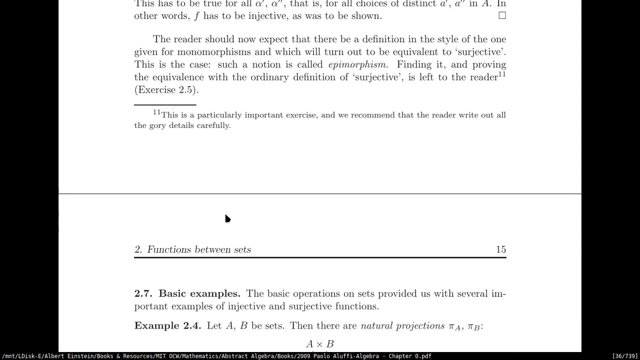 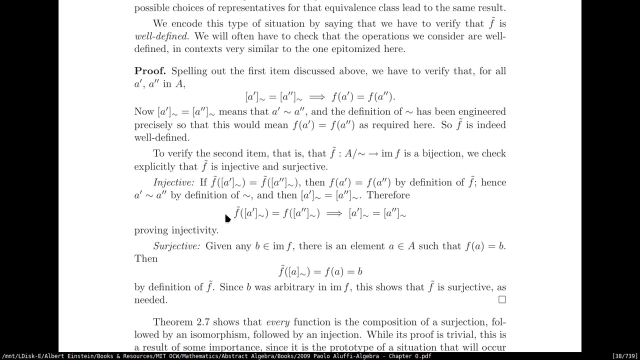 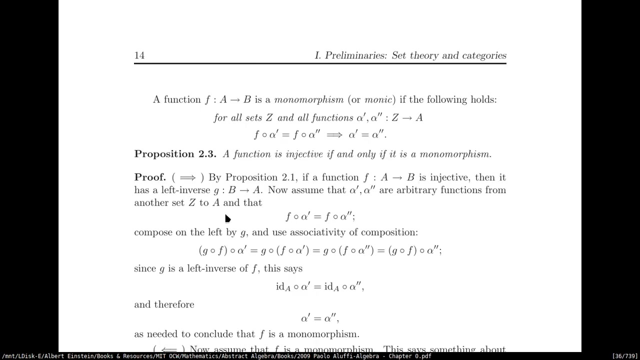 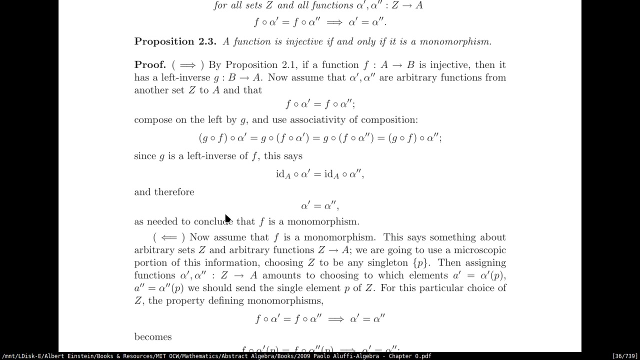 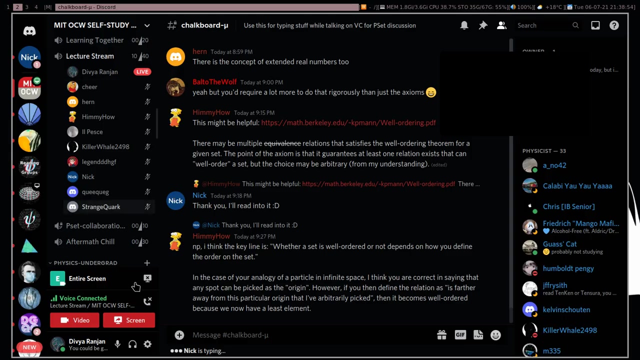 I'm let me get some water. if you have any questions you can ask. yeah, I'll grab any questions you can ask. yeah, I'll grab any questions you can ask. yeah, I'll grab that, that, that, yeah. so I just asked like if we should. yeah, so I just asked like if we should. 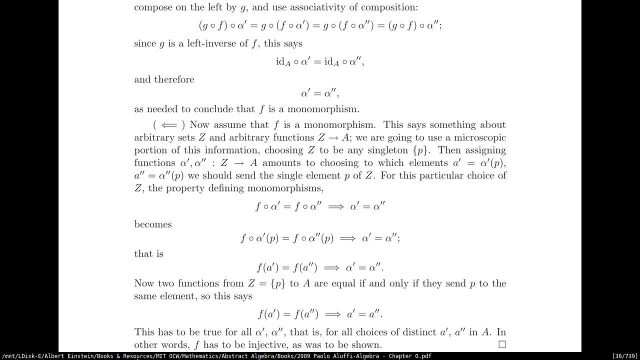 yeah, so I just asked like if we should, if anyone actually wants me to go to, and if anyone actually wants me to go to, and if anyone actually wants me to go to and explain this proof about injectivity, and explain this proof about injectivity. and explain this proof about injectivity and monomorphism, or does it look good to you? 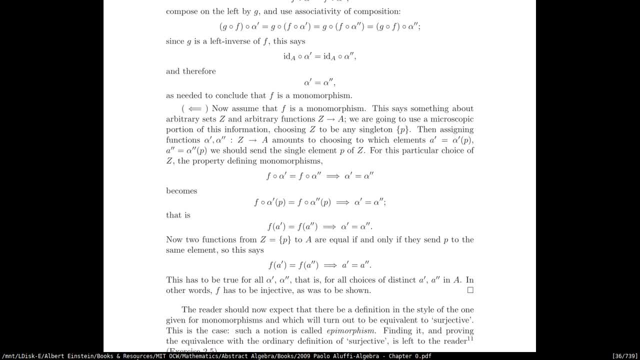 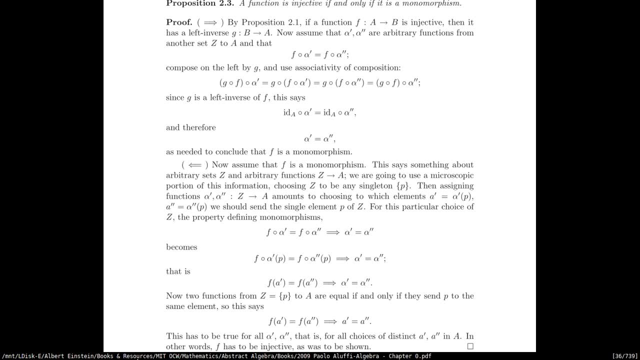 monomorphism, or does it look good to you, monomorphism? or does it look good to you so that we can skip? so that we can skip, so that we can skip. yeah, if anyone actually wants me to go. yeah, if anyone actually wants me to go. 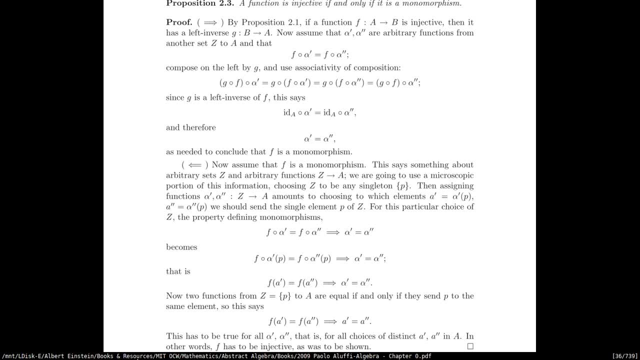 yeah, if anyone actually wants me to go to it, I will go to it. but if everyone's to it, I will go to it. but if everyone's to it, I will go to it. but if everyone's fine, then that's fine. fine, then that's fine. 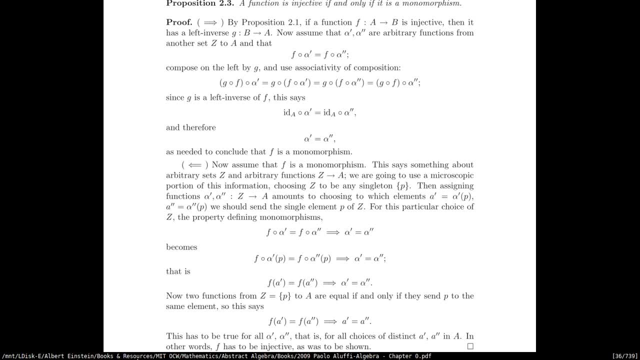 fine, then that's fine, okay, yeah. so the idea is again: you have. okay, yeah, so the idea is again: you have. okay, yeah. so the idea is again: you have to like, like you know, prove the two-sided to like, like you know, prove the two-sided to like, like you know, prove the two-sided thing. and essentially, you have to use the. 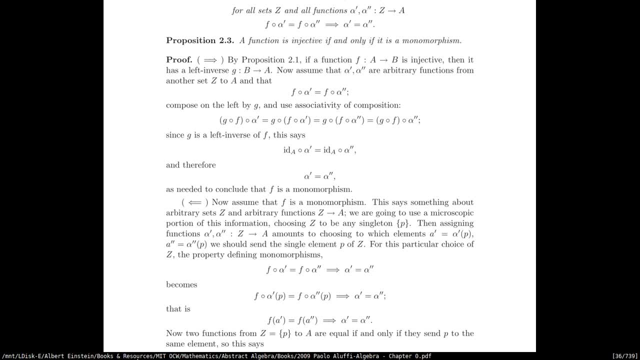 thing and essentially you have to use the thing and essentially you have to use the fact that it's injective means it has a fact that it's injective means it has a fact that it's injective means it has a left, inverse right, but like for the 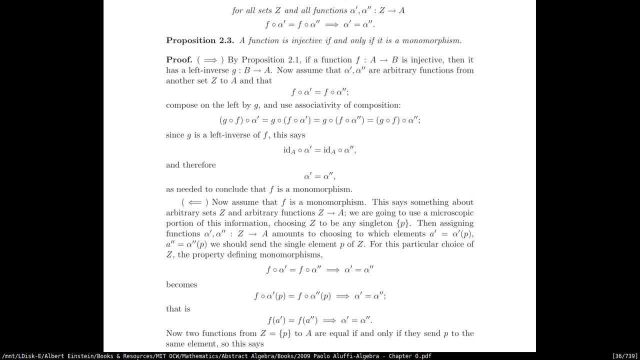 left inverse right, but like for the left inverse right, but like for the forward direction. you can use that to say forward direction. you can use that to say forward direction. you can use that to say that like those two, that like those two, that like those two things, alpha prime and alpha double. 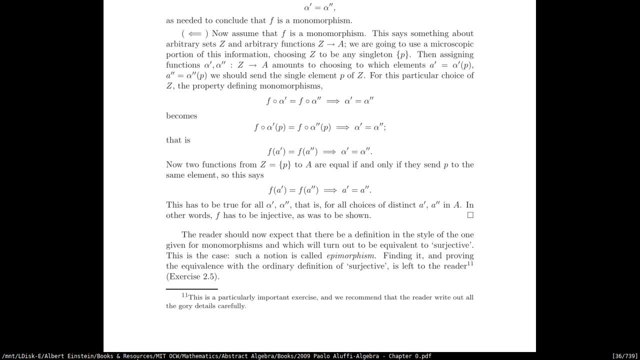 things: alpha prime and alpha double things, alpha prime and alpha double primary cool and then for the other primary cool and then for the other primary cool and then for the other direction that's kind of complicated, but direction that's kind of complicated, but direction that's kind of complicated. but you can use that as it's a monomorphism. 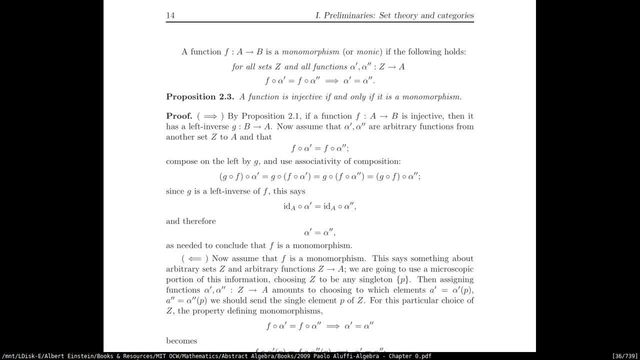 you can use that as it's a monomorphism. you can use that as it's a monomorphism. that's alpha prime and alpha double. that's alpha prime and alpha double. that's alpha prime and alpha double- primary equal. from there, you can prove primary equal. from there, you can prove. 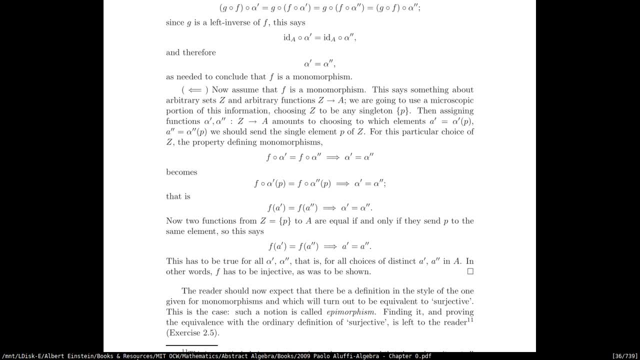 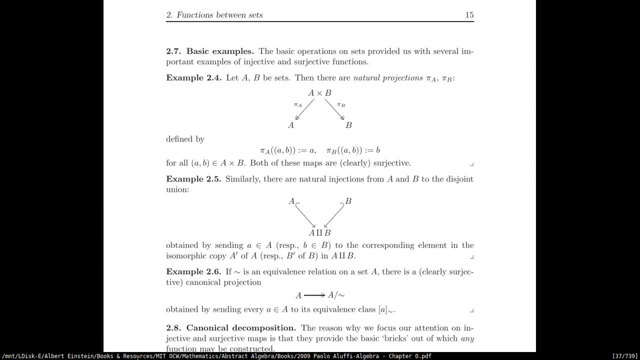 primary equal. from there you can prove injectivity. yeah, it will take a while injectivity- yeah, it will take a while injectivity- yeah, it will take a while. but yeah, it can be a good exercise to, but yeah, it can be a good exercise to, but yeah, it can be a good exercise to get you. so yeah, we have some basic. 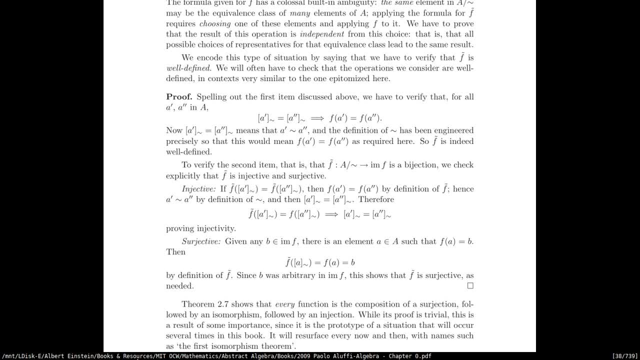 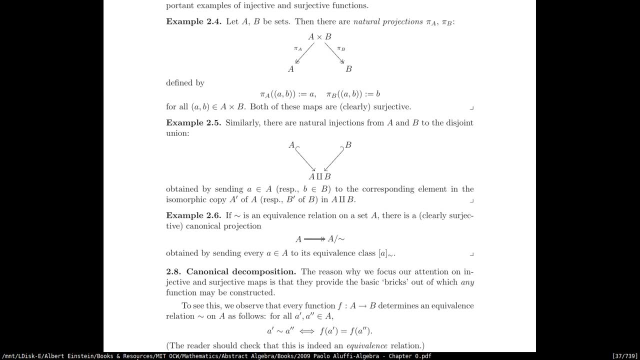 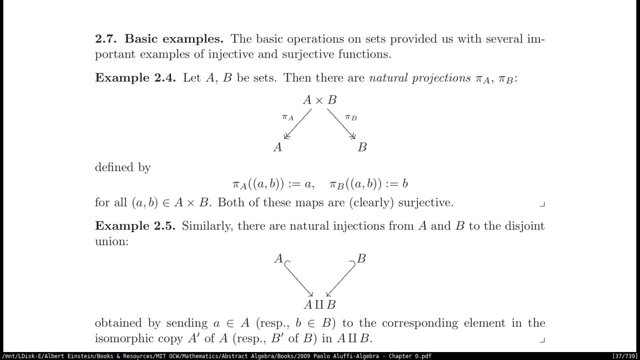 get you. so, yeah, we have some basic get you. so, yeah, we have some basic examples and yeah, and another proof examples and yeah, and another proof examples and yeah, and another proof which is sharp okay, so yeah, so there which is sharp okay, so yeah, so there which is sharp okay, so yeah. so there are some basic examples of injective and 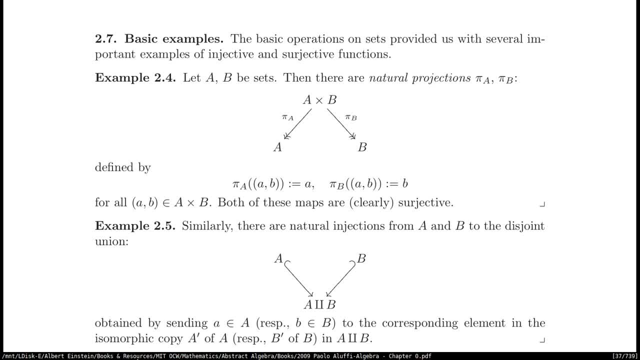 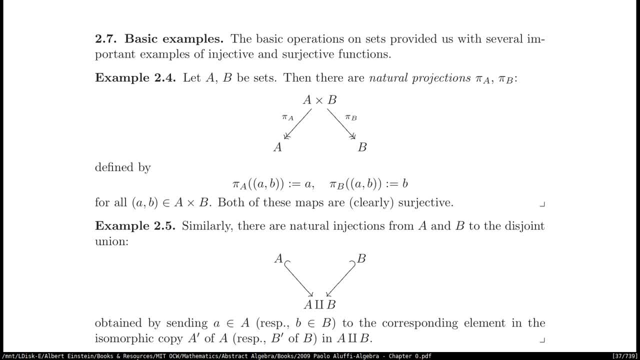 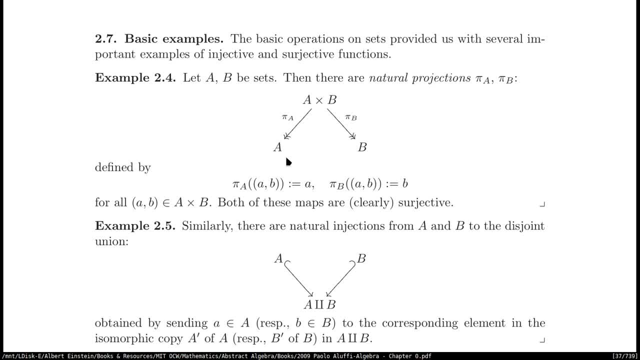 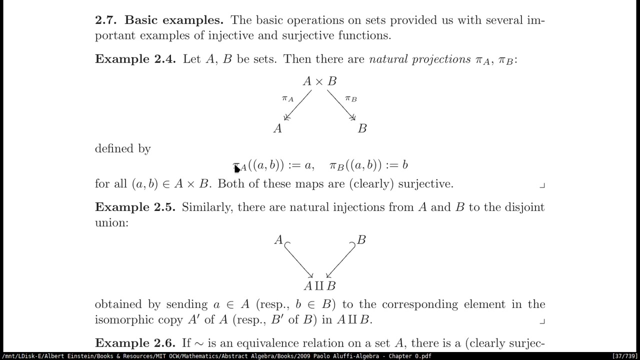 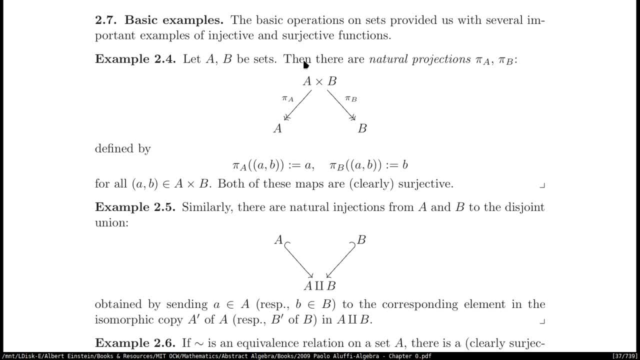 get A, you pull A out of it, and when you do it for every other pair, you just pull out the A's, you get the set A same for B. so these maps are subjective, as you can clearly see, because every element of A is pulled out with some ordered pair of. 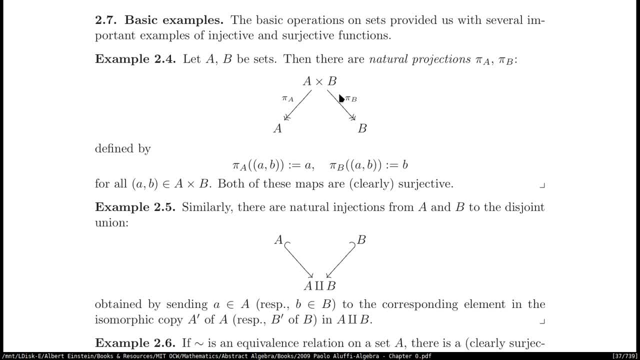 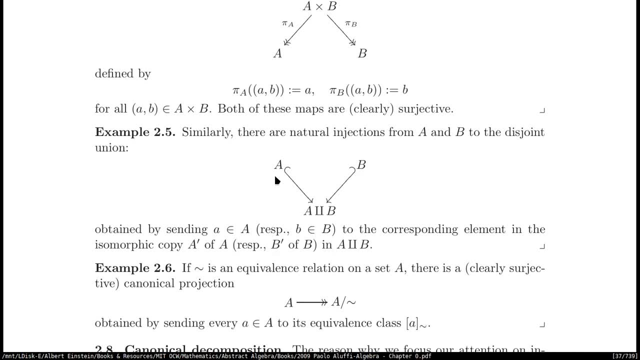 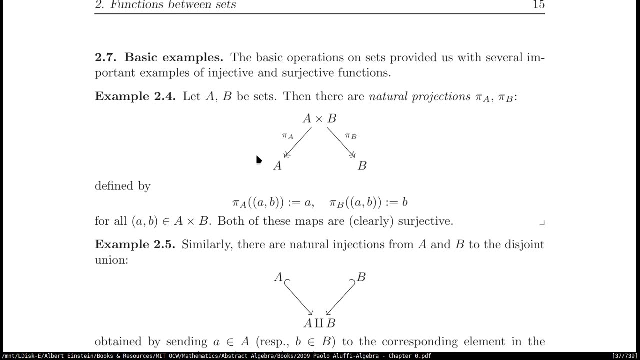 A cross B, so you always have something from the image in the domain. okay, so so naturally, from projections you can actually have injections to the. but, like, some of the calculations work well, but there are layers that are driven by the would like to make a first WOW json, not counting, being that little hesitant of. 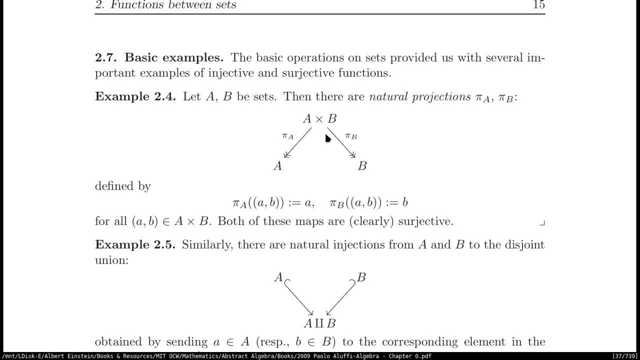 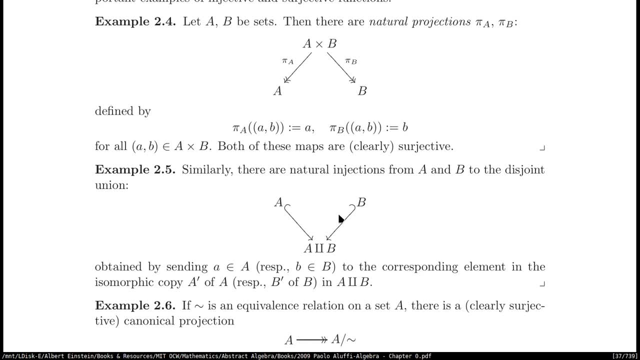 Instead of having the Cartesian product, we have the disjoint union, this time right. So what you have is like you have two different sets, A and B. Then you can inject A into the disjoint union of A union B. So what you do is you take the elements A of A cap set A to the corresponding element in the isomorphic copy, A prime of A in A disjoint union B. 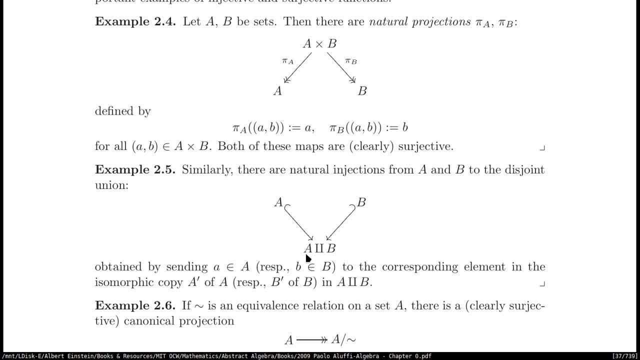 Yeah right. So again in the disjoint union, you have a set which is isomorphic to A. It's not exactly A, but it's isomorphic to A. It's unidirectional, So essentially that every element of it is the same. 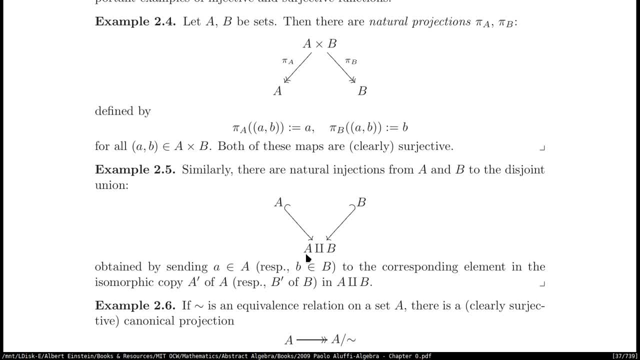 Sorry, it can be identified using a bijection And you can send these elements to there and you do the same for B and that gives you a way of injection And yeah, So, yeah, that lets us do a lot of things actually. 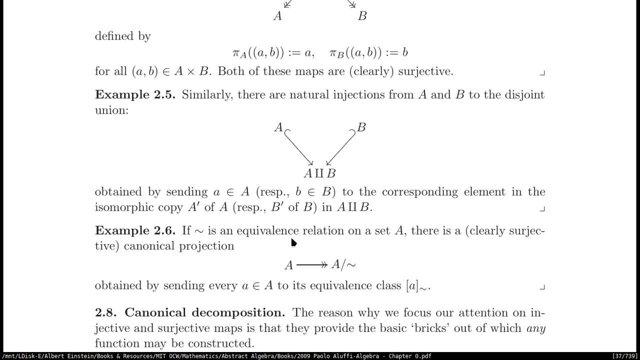 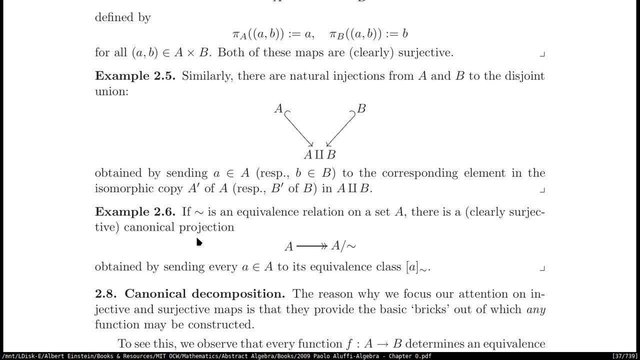 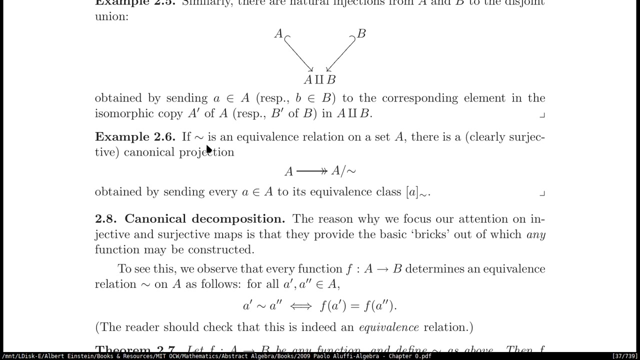 Because if you think about it in topological terms, this is basically what you call the immersion, inclusion and stuff like that. But yeah, So okay. so let's see what we have. We have another example. So if tilde is an equivalent summation of a set, then yeah, so you can have a projection. 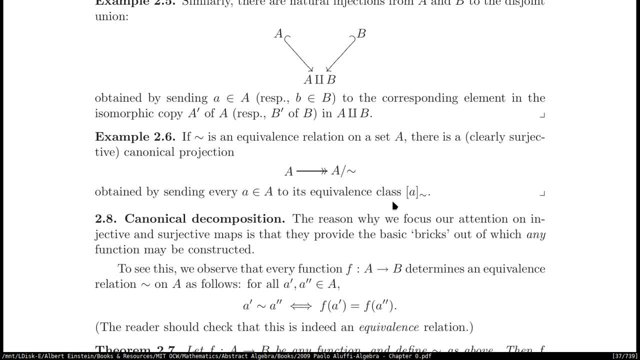 From the original set to its quotient set, right. So what it does is it takes elements of A and it maps it onto the Kugel's classes of each of those elements And that gives you a subjective map. and does you know function. subjective function. 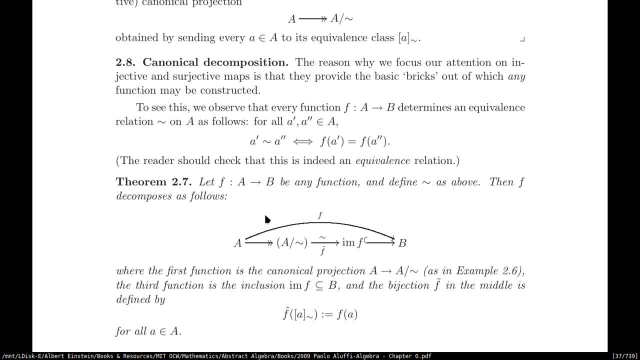 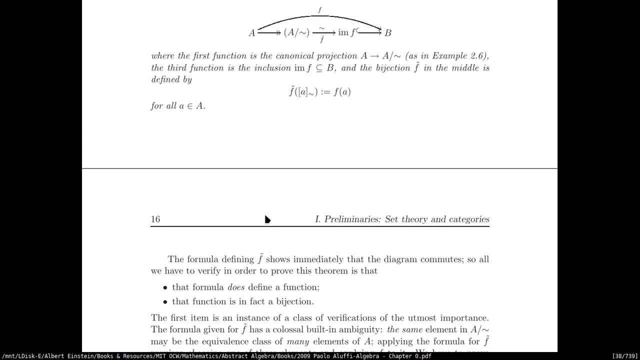 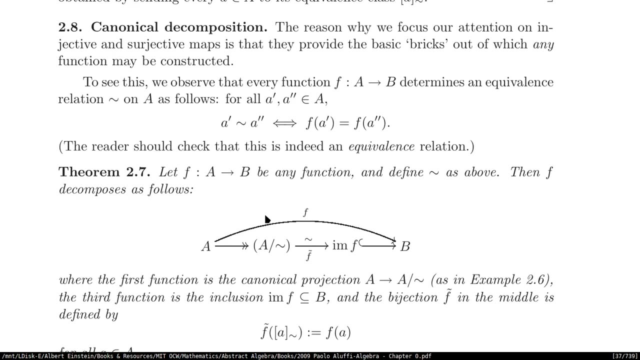 Okay, So I think this is the last section. Yep, So we have something related to the canonical decomposition. This is also interesting. We'll see How long is this lecture. It was supposed to be around 1.5 to 2 hours. 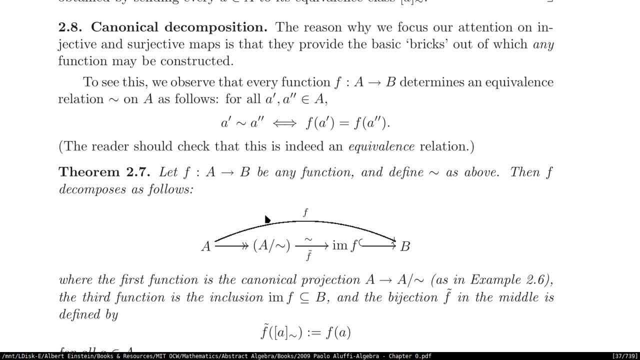 Yeah, Let's see. So what we see, what we observe, is that every function f from A to B actually determines and lets us have an equivalence relation on A. Okay, So what we see is that every function f from A to B actually determines and lets us have an equivalence relation on A. 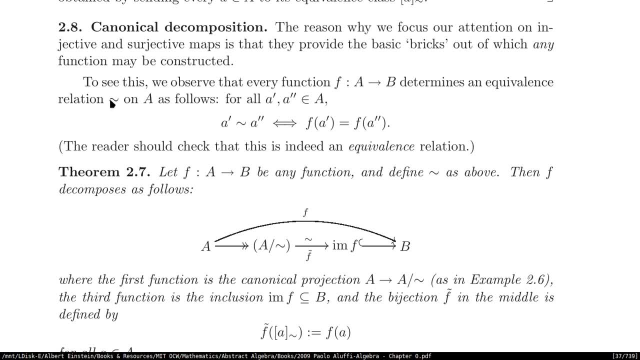 For all. Let's see- Okay, Let's see- distinct elements of the set A. so how you do this is that if you have a function, A prime, tilde, A double prime is like: sorry A tilde is identified. sorry, A prime is identified with A double prime. 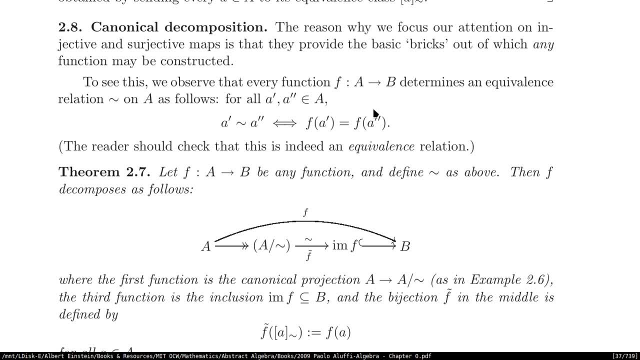 if, and only if, f of A prime is equal to f of A double prime. So essentially, if your image of two distinct elements is the same, then those two elements can be identified using some equivalence relation. so this function allows you to identify the images of elements. 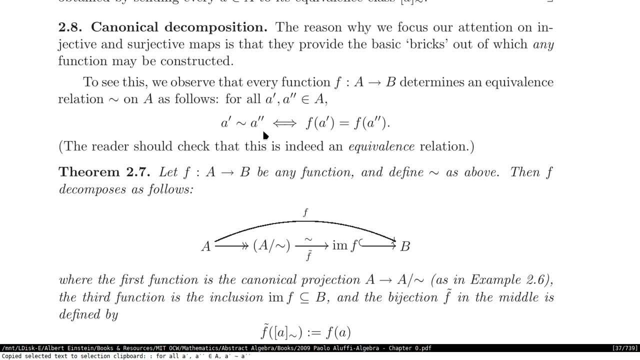 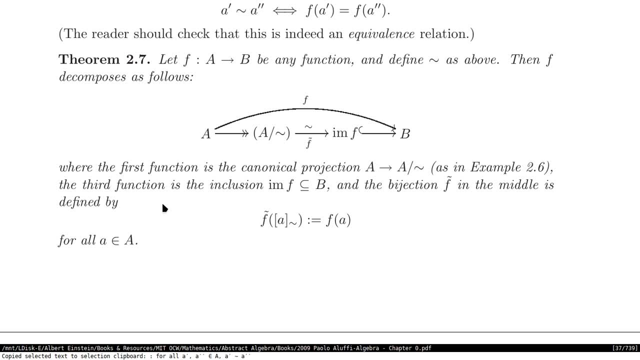 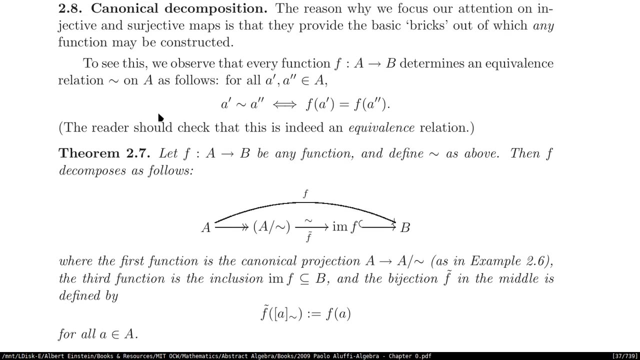 and you can have an equivalence relation with that. So what we can do is we can actually have some interesting things using this right. so f is any function and you define the equivalence relation as we defined here, then we can decompose f into in this manner. So what you do is you have 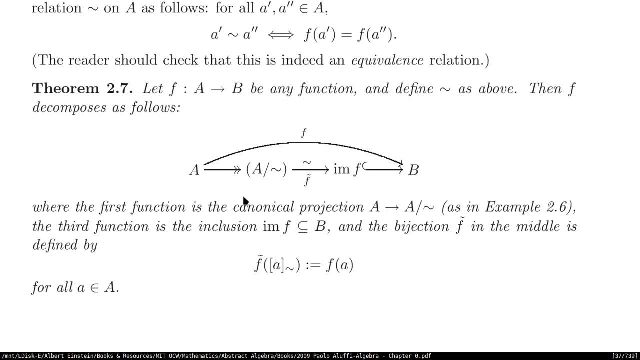 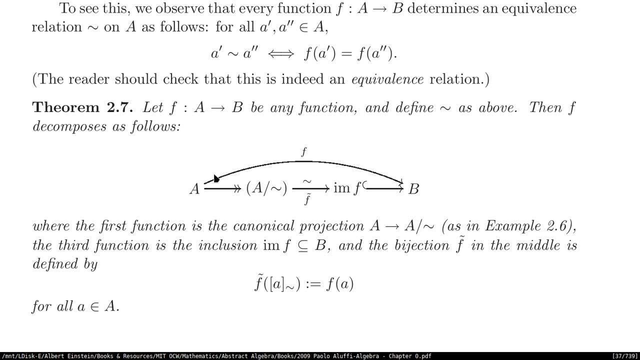 f goes from A to B. but what you do is you first have A to A slash tilde, that is, the quotient set of A, and then you have this f tilde which goes from A slash tilde to the image of A, and then you have an injection inclusion into B. 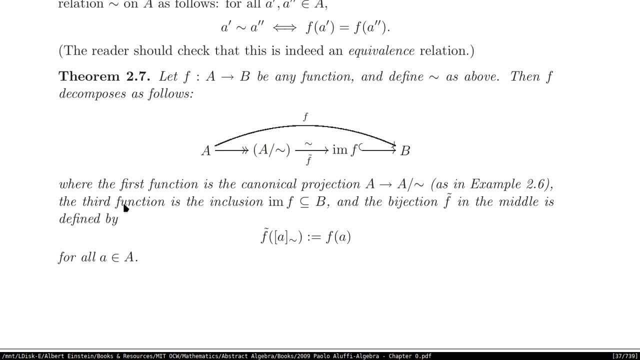 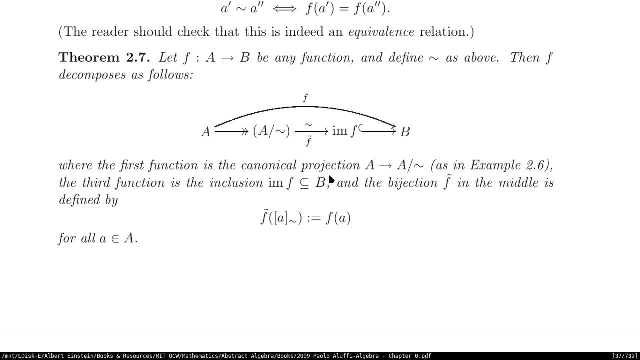 so we'll see that, but this is just the diagram, so yeah, so in detail, the first function is the canonical projection that we just saw before. It maps every element of A to its equivalence class right, and the third function is the inclusion right. so what it does is it includes the image of f. 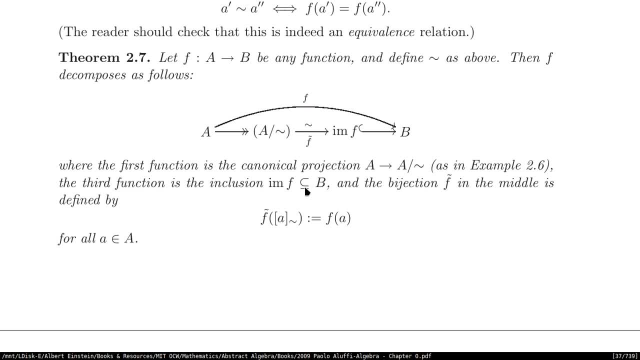 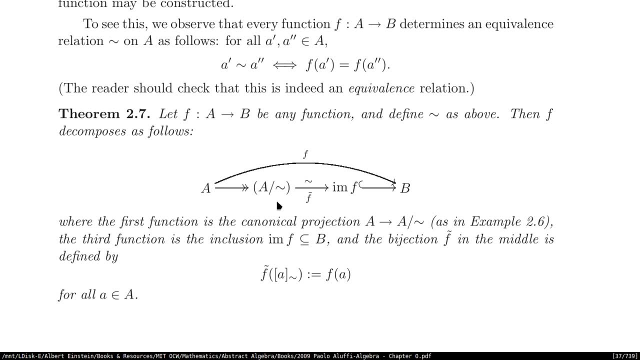 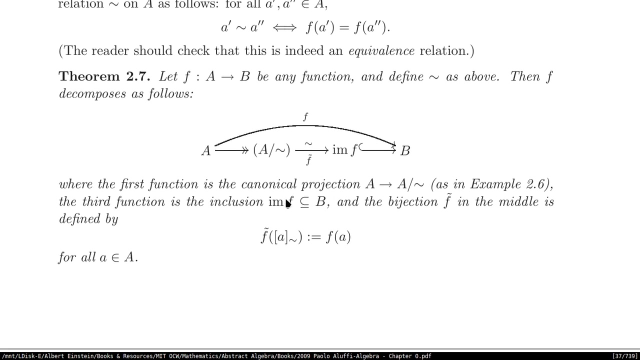 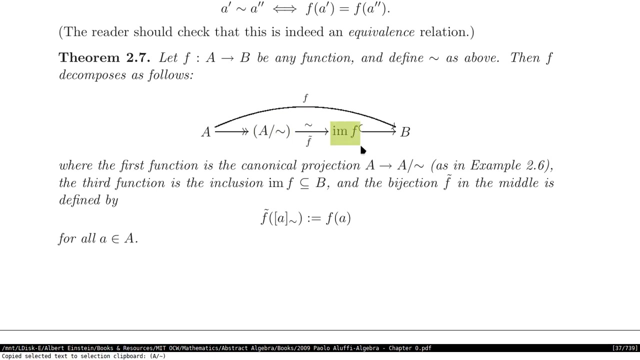 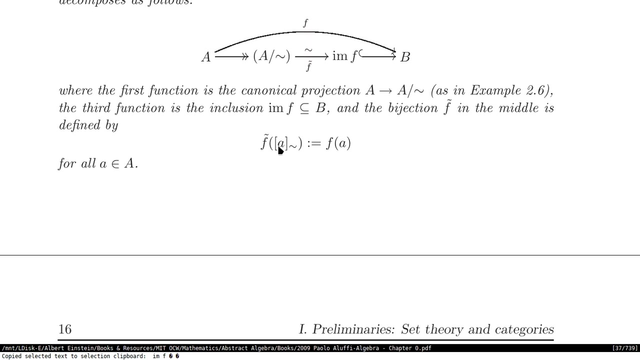 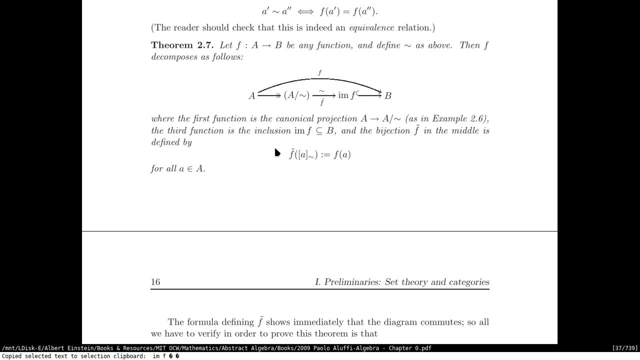 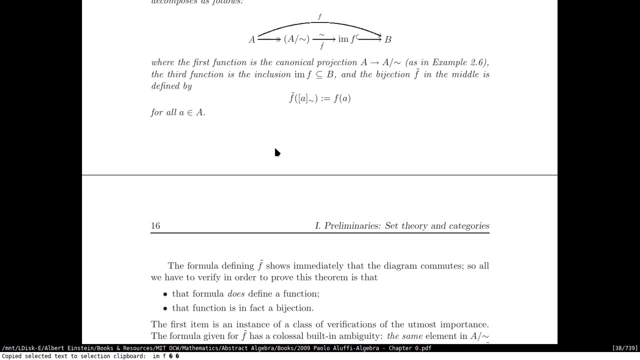 that is f of A within B right, and how it does that. well, inclusion is just a way of like it's a subjective map that um, um through the right, yeah, so this is how you can like decompose f into its, into like kind of like sub functions, like 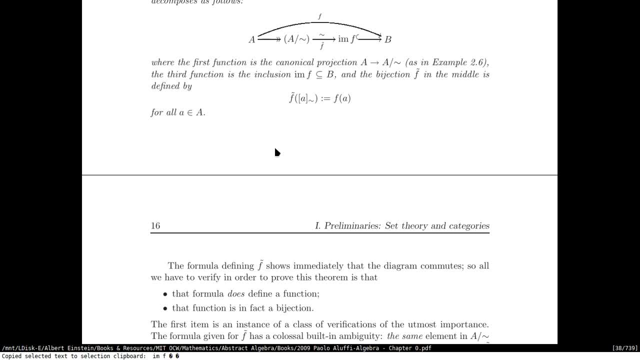 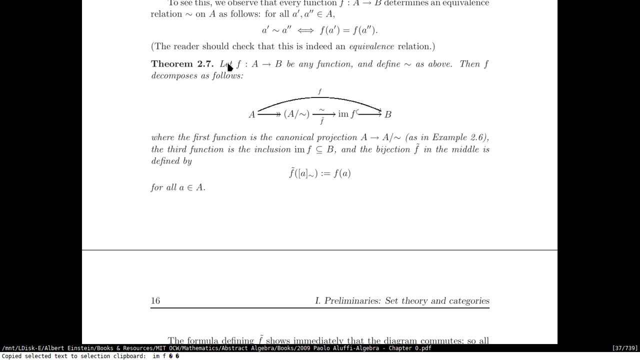 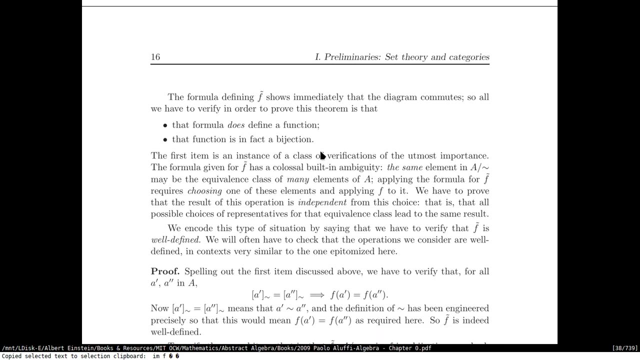 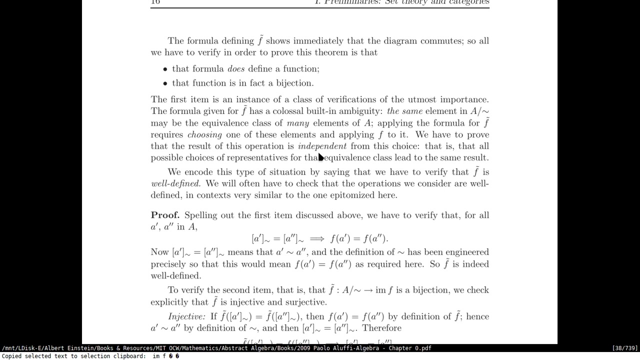 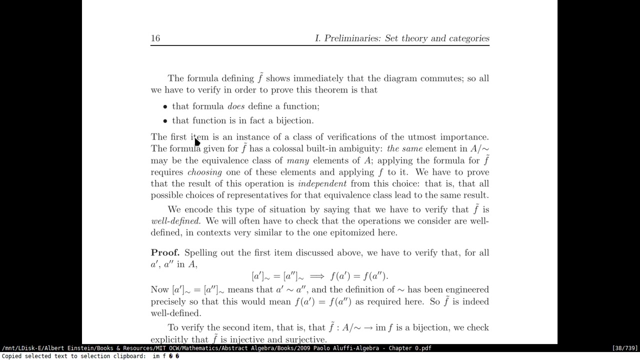 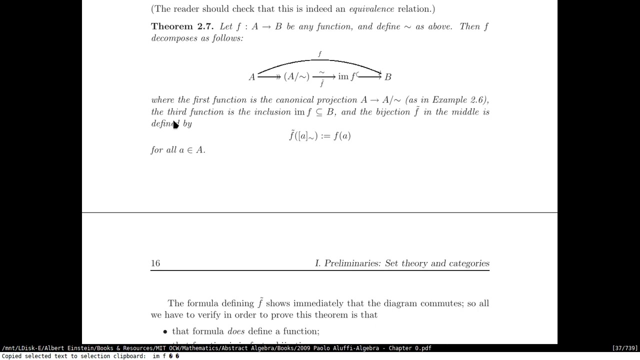 essentially composition of these functions. so we have to show that, like this diagram, commute to the and like F can actually be decomposed. So that's the theorem. Okay. so what we have to verify is that is like if we can define actually this F tilde as a bijection, then 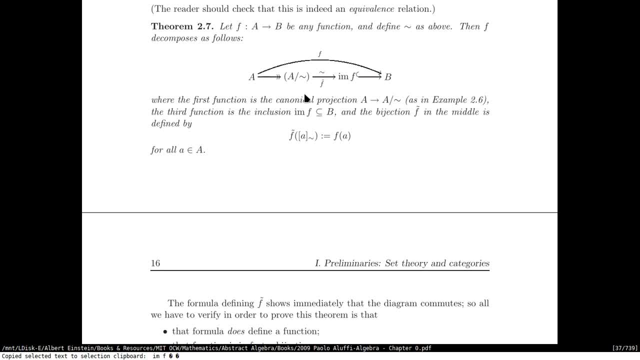 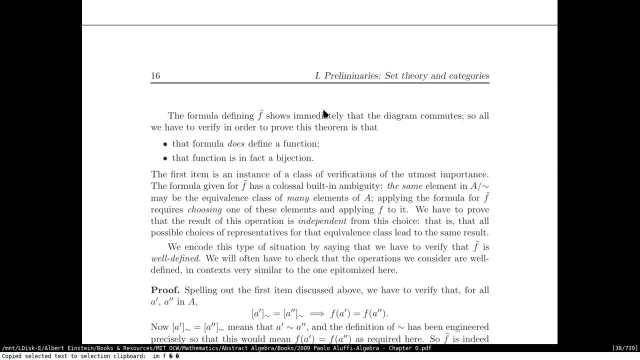 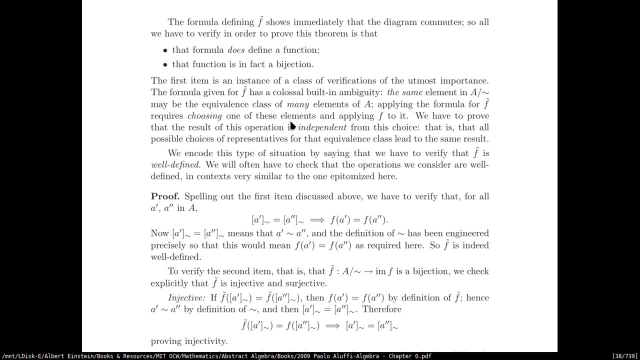 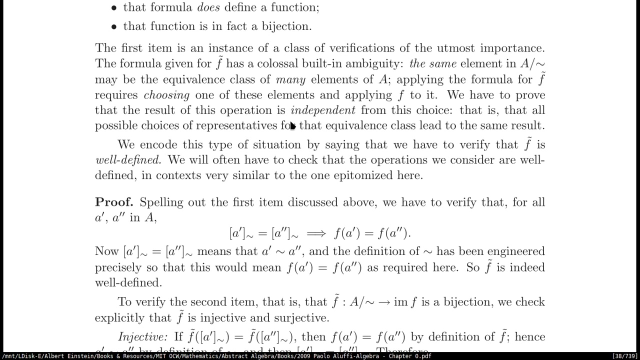 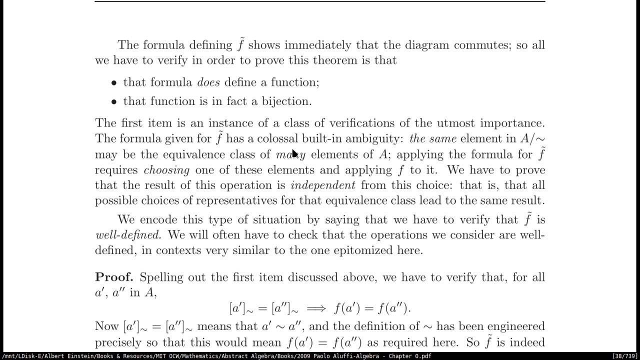 this path is connected and we need the commutativity of the diagram as we want it to have. So, yeah, so that's, that's the key part of this proof, and we'll actually go through this because it looks important. Any questions? Okay, yeah, 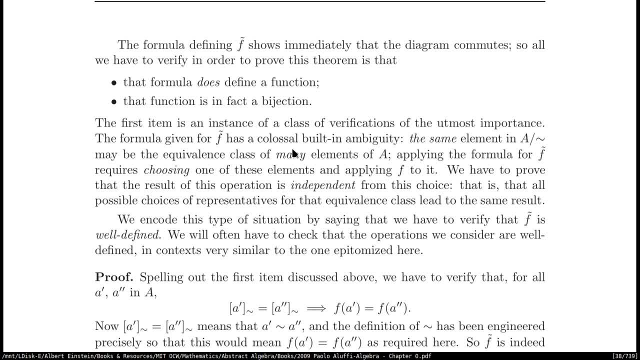 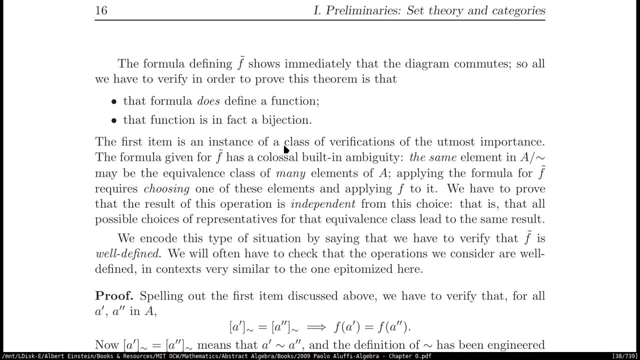 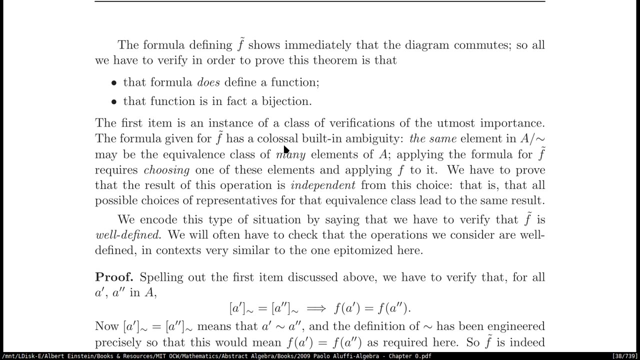 Good to see that you guys are having an actual serious discussion about the axiom of choice. Okay, I have something to say about this, but we'll see. Okay, so let's see how we can do this. So the first item is an instant of a class of verifications of the utmost importance. 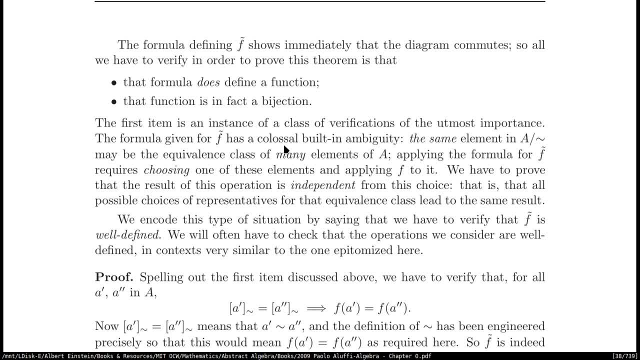 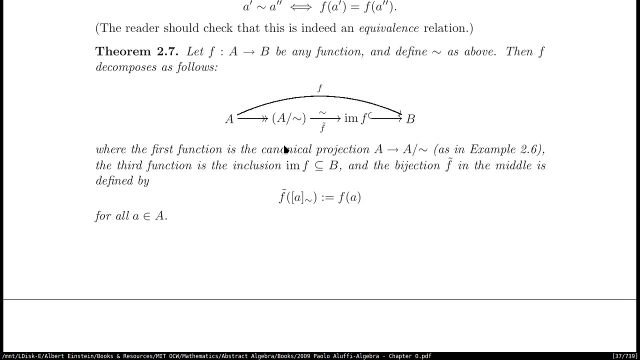 So the first item is an instant of a class of verifications of the utmost importance. Hmm, fine, let's do this. Huhu, huhu, right. So if you think about this, F-tilde, F-tilde takes you from the. 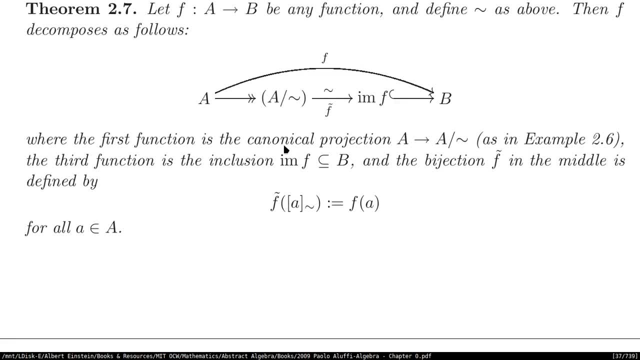 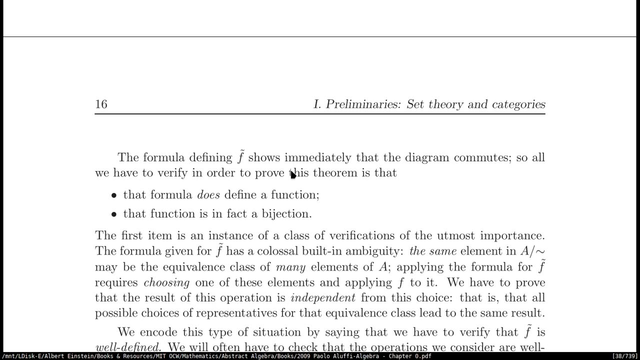 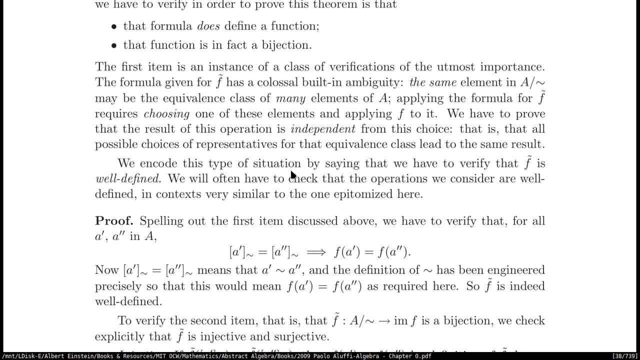 equivalence classes of the elements. Now, equivalence classes of each element is like a set of myekk. fr字 is a very big L set containing the other elements which are preserved under the fluence nation. but what this F? tilde does is that it chooses. it chooses what. 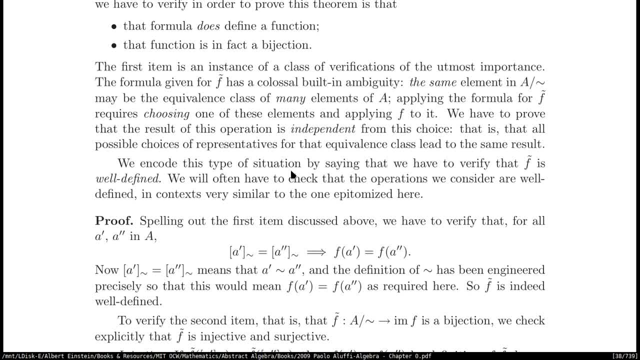 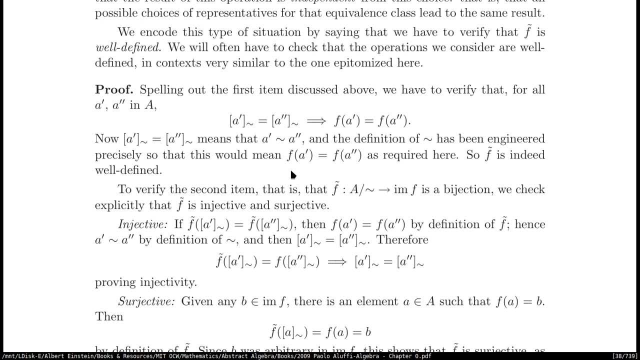 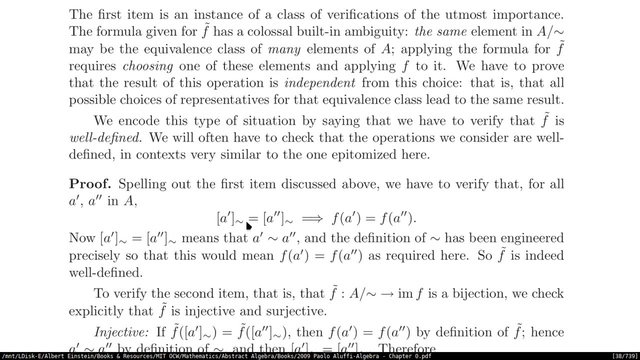 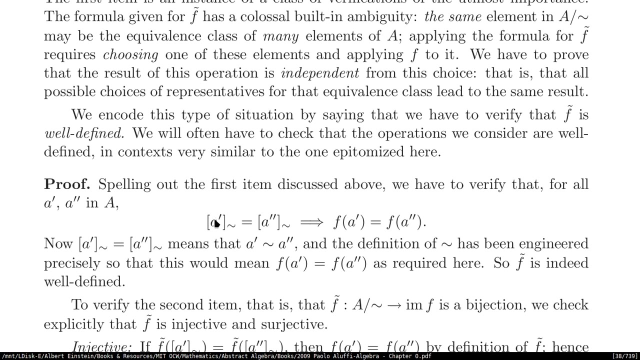 each of these elements and then then gives you the images F of a that you need. so what we have to verify is that: so if you have two distinct elements, a prime and a double prime, and if the equivalence classes of these two elements are equal, then that implies the images of both of them are equal of them. 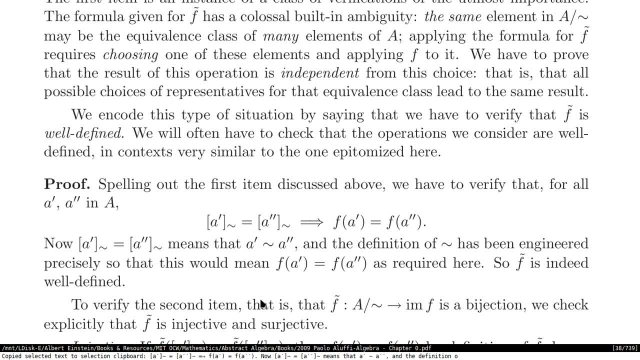 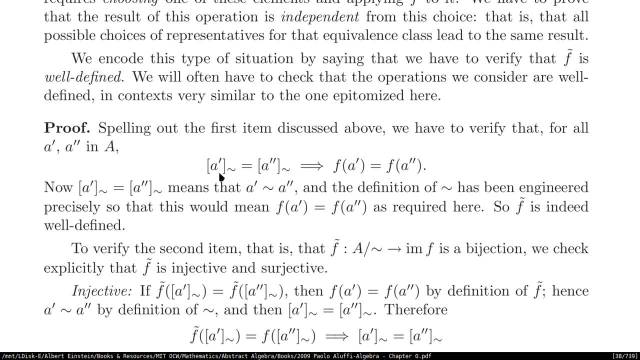 right so. so now let's see: so if, if you have the equivalence, classes of two elements are equal. so what this means is that you can have an equivalence relation between these two distinct elements. right so now. now they're no longer distinct. so a tilde, so a prime, is equivalent to a double prime, and 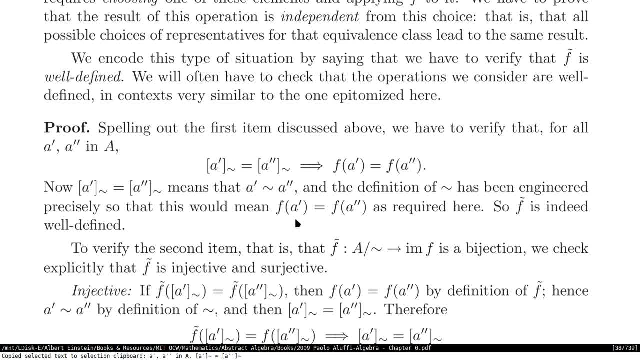 so so like by definition of the equivalence relation, what this means is that F of a prime is equal to F of a double prime. it's because a prime and a double prime are equal under this equivalence relation, so like their images are also going to be the same right, so F tilde is actually well defined. now for the second. 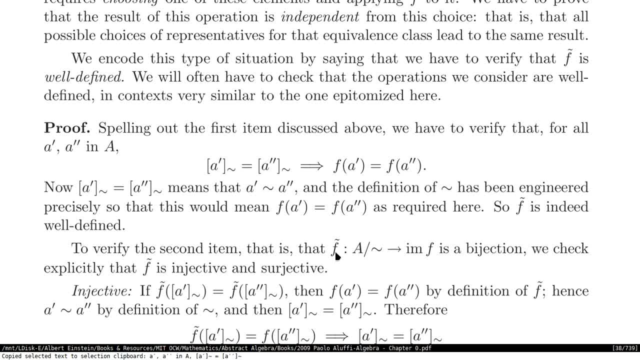 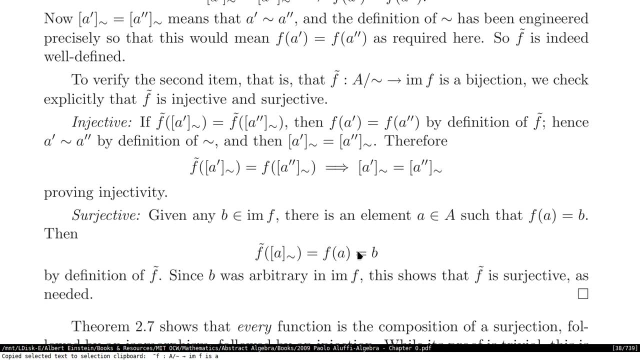 item of the second step, you have to show that, like this is actually a bijection, so we have to show that it is injective and refracted, right. so for injectivity, what you do is you have to apply F tilde on equivalence of two distinct elements, right? and you say that if the images of those underlying近 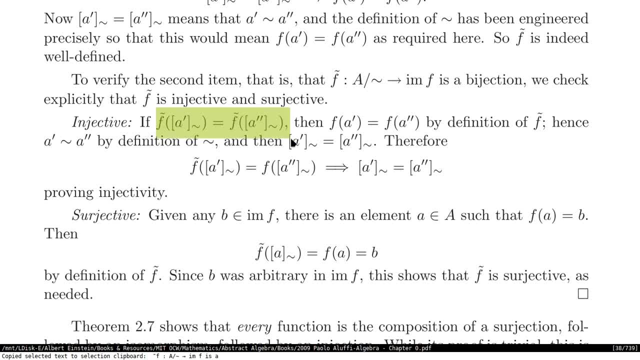 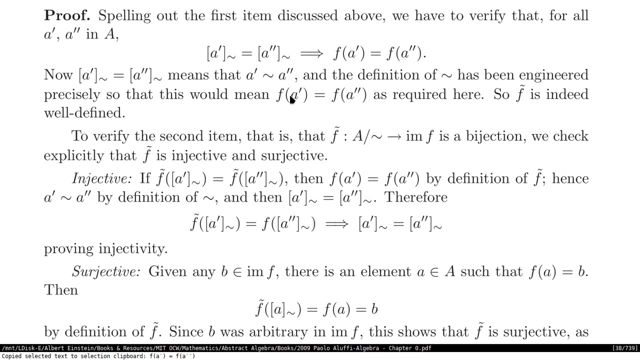 elements that have two distinct weight movements figures will be the留言 properties of those elements which we holding. the say that if the images of under f-tilde are equal, then the images under f of those elements are equal. okay, so um right, because um, we just showed that um like if um by definition of f-tilde, if you have two, 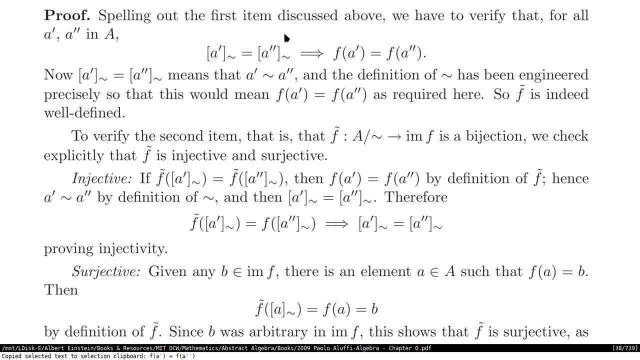 distinct elements: a prime and a double prime, um, their images are going to be the same, um, so, um, um, a. a prime is equivalent to a double prime by definition of. i tell that again, so again, yeah, so this is essentially just, you know, walking uh backwards, right, um, if we apply f tilde on the equivalence classes, 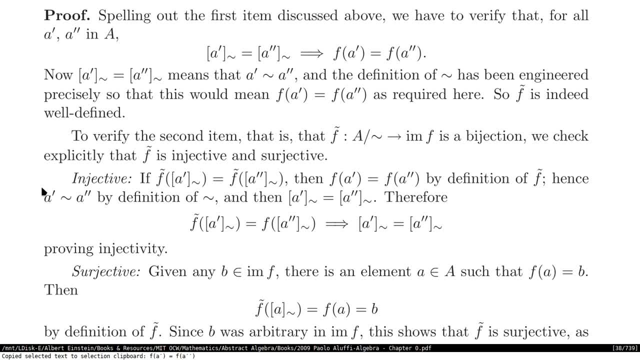 we know that they, um, um. we know that the elements themselves, a prime and a double prime, are equivalent under the equivalence relation. um, so um. so what we showed is that, uh, the equivalence classes are equal. what this means is that it is injected right and um, this one is again. you just follow the definition. 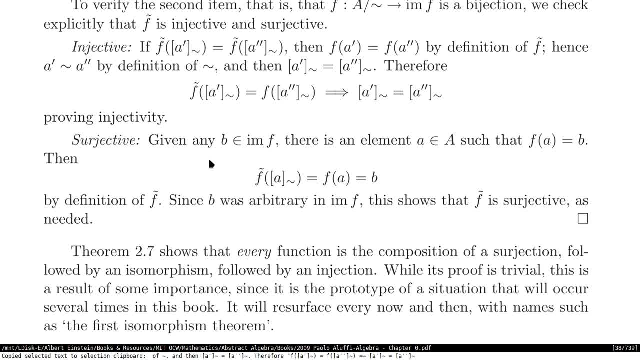 so if you take b? uh as like any image of f? uh, then there is an element a such that f of a is b right, and that's because it's an image um. so if you have, like some um equivalence class of a and you apply f tilde on it, um, you get f of a um, but f of a is just b, as we assumed um. 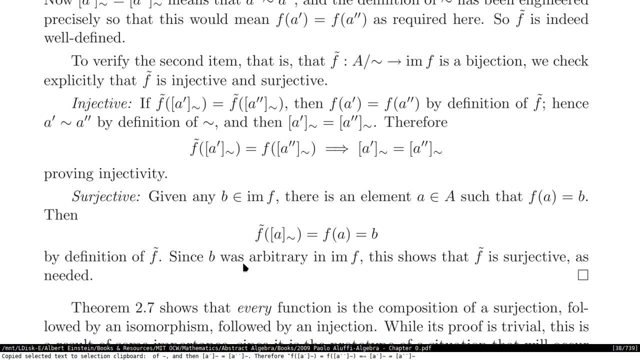 so this is from the definition of f, tilde, um. but again, as we just picked any random b in um the image, uh, it shows that, like, we can do this for any other random um element in the in the image and thus, uh, you know, it's subjective. so this is actually. 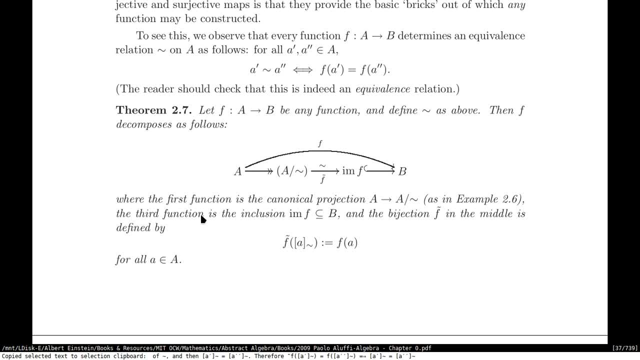 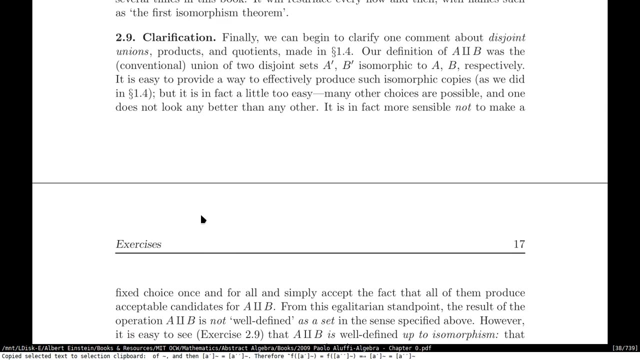 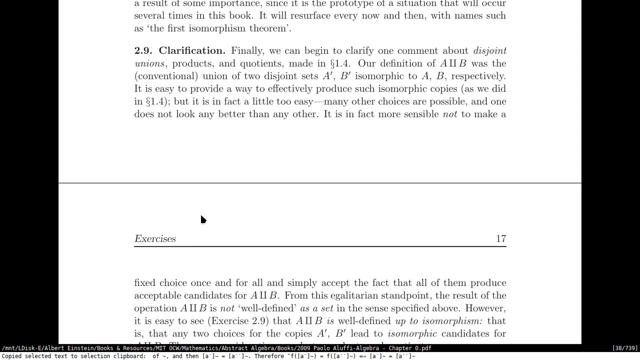 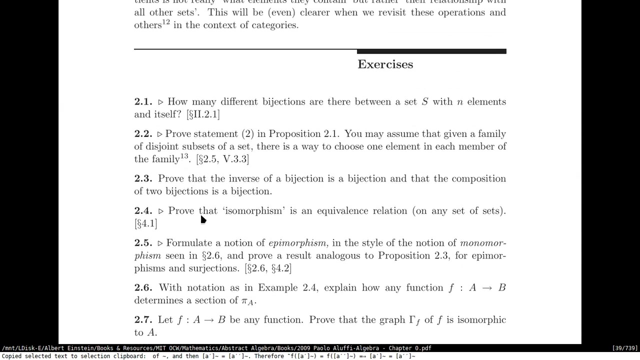 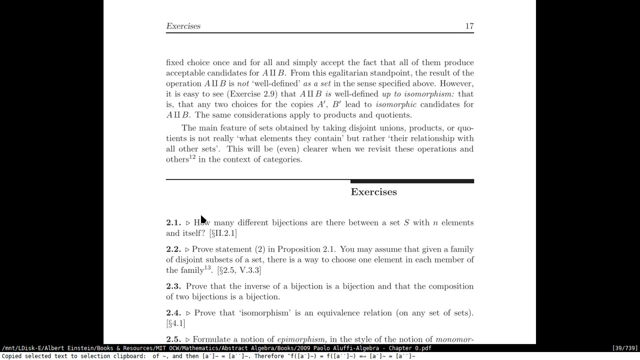 a very important thing- and the decomposition of any function using the true installations. um and yeah, so that uh supports the final state that we just looked at. okay, so yeah, we're pretty much now we're done and, uh, we have um exercises. i would recommend you doing um most of the exercises, if you can. 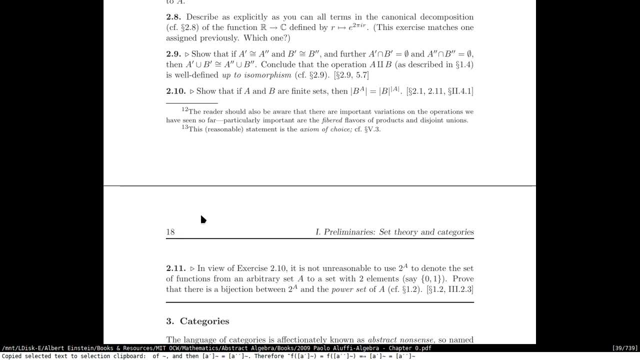 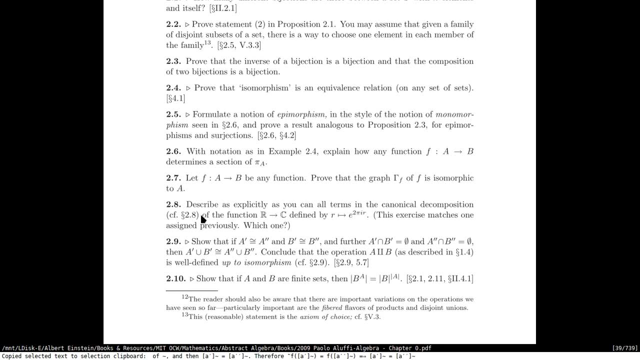 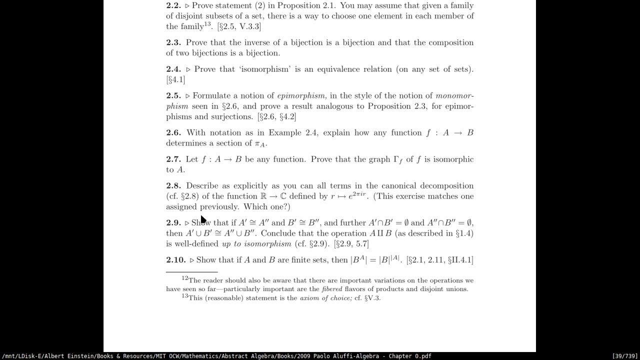 um, um, um, the ones that are like have some symbol triangle in it. they're kind of um, they look good. you can like. i don't think the author says anything about it, this is just what i've seen. but um, but yeah, do the problems? um, the problem sets are pretty much going to be from here, so they can be a. 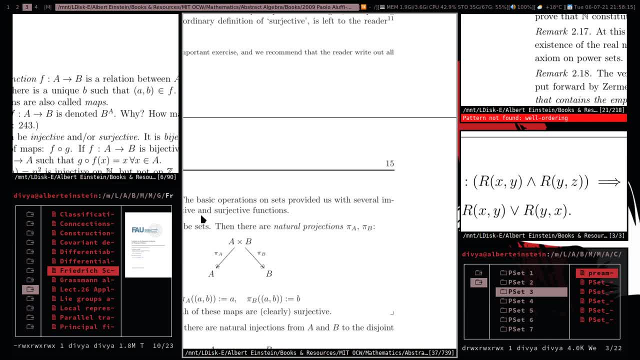 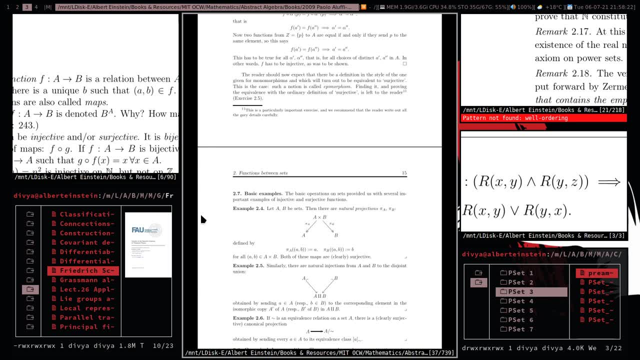 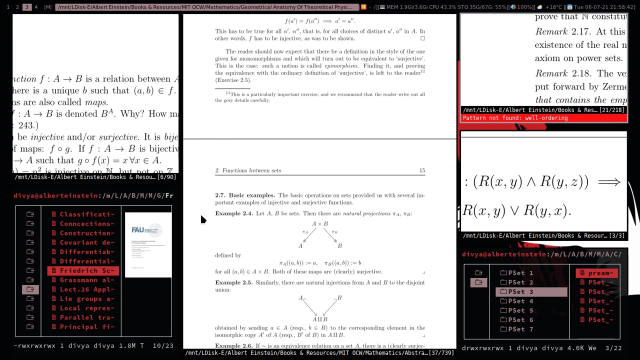 pal. so so, yeah, any questions or anything you want to say about before we leave. i wanted to say thank you, this has been very useful. ah, that's not hard to know. um, yeah, if you, if you have any kind of suggestions, uh, do you like? uh, feel free to suggest any kind of like. 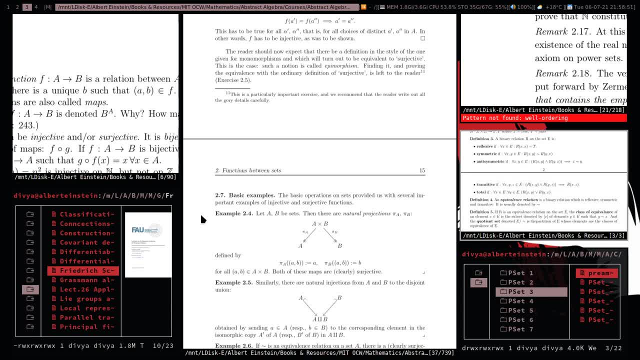 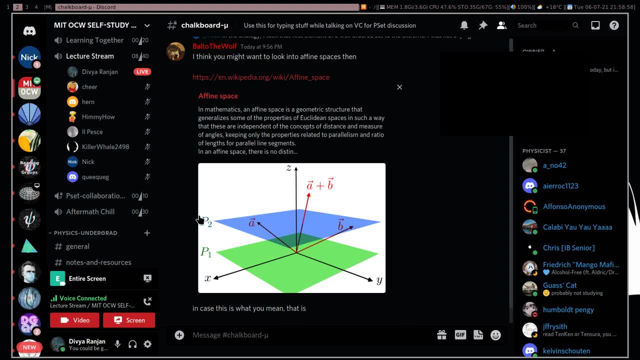 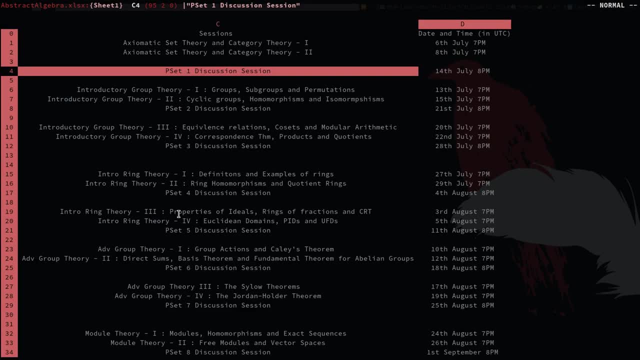 suggestion material or anything. i mean, the material can be changed because the schedule has been apparently like that. but um, yeah, um, okay then. so yeah, let me take a look at the schedule again. um, the pset discussion will be on 14th july. uh, the pset will be. 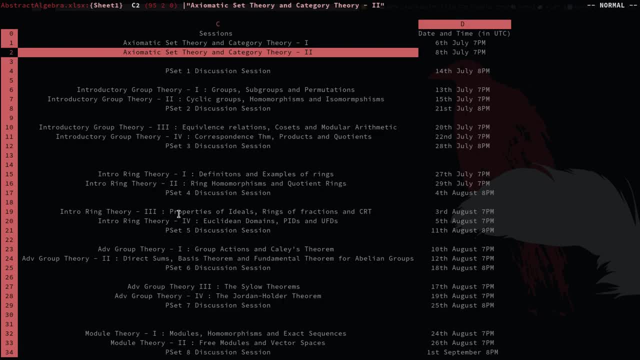 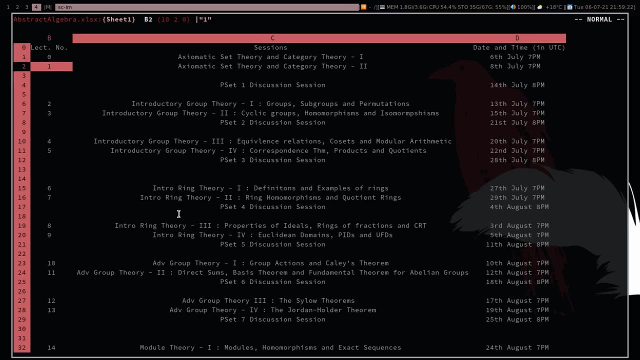 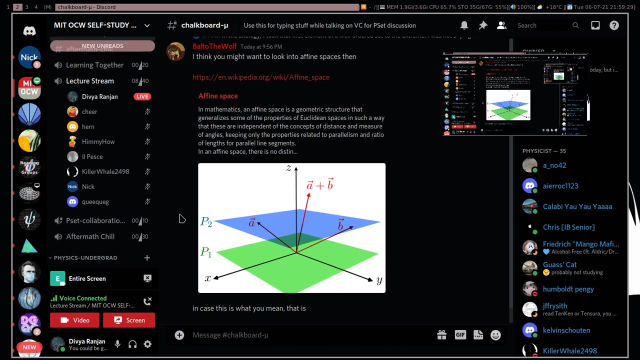 released on 8th july, that is a that is thursday, and you'll have around six days to solve it. yeah, yeah, and about the uh axiom of choice, as you guys were discussing um, i would say the axiom is that, uh, if you have an original origin um, then you're 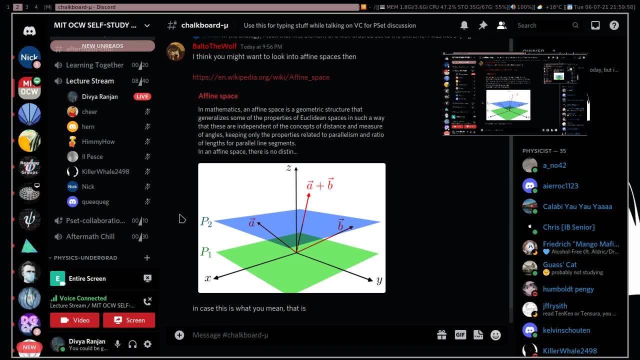 you're, you're in a finite system. i'm not sure if that's um your original origin, but i'm not sure. yeah, yeah, as nick pointed out, uh, the aristotle's way of thinking was that, yeah, if you have an origin, then you, you are um in the finite system, but i'm not sure. 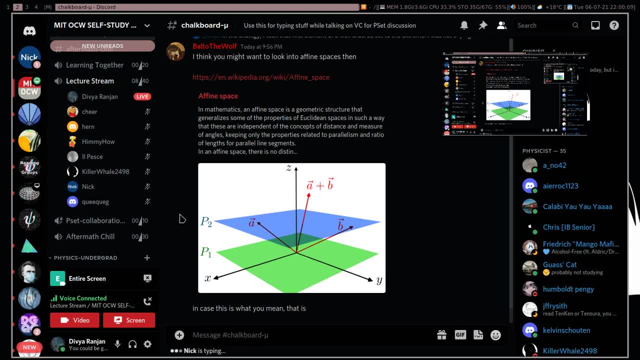 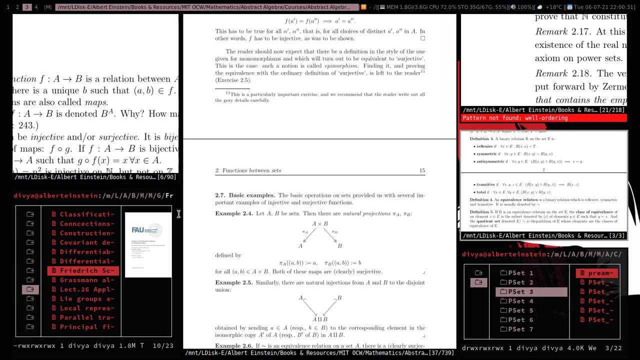 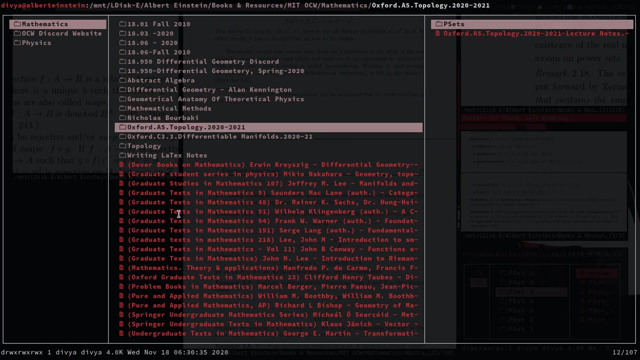 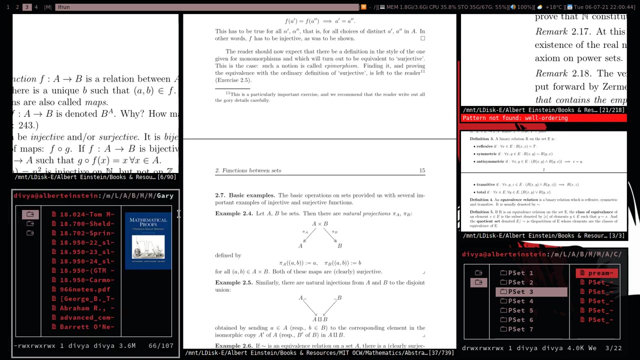 um, that's what the axioms are intending to say. Okay, so yeah, practice sunset theory or if, like I think, I have this book, which was this Transition to Advanced Mathematics- yeah, so this is a book on proofwriting actually. 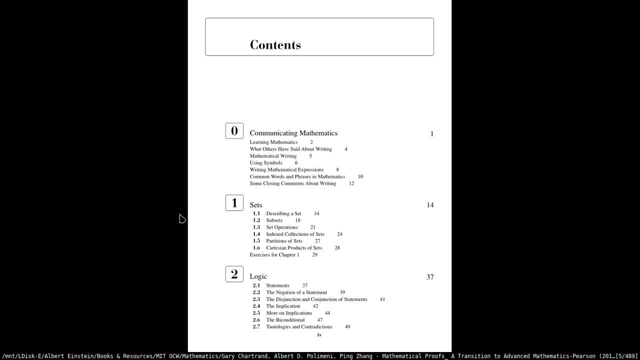 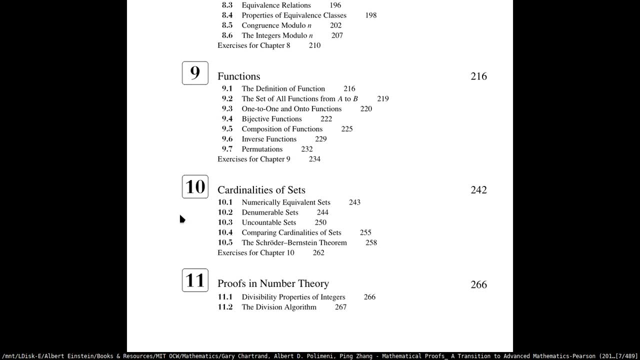 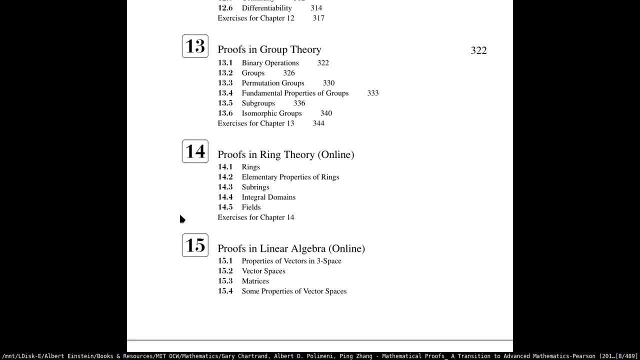 it is. it is pretty good. it has like proofs and like of different kinds, so you might like- I mean, we're not doing a course on proofwriting, so but like you can like. 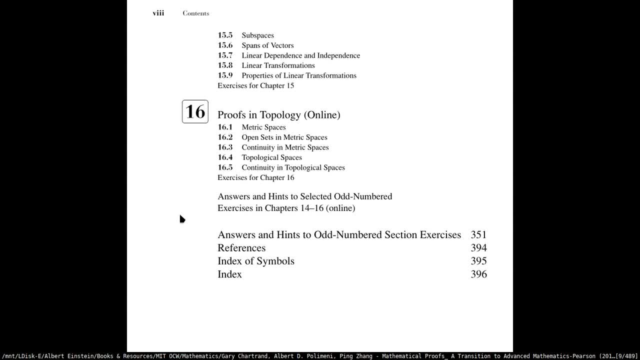 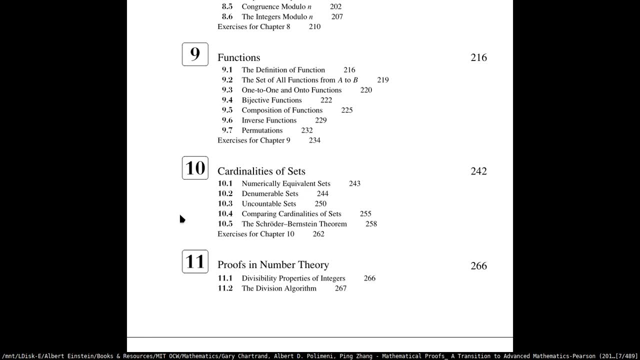 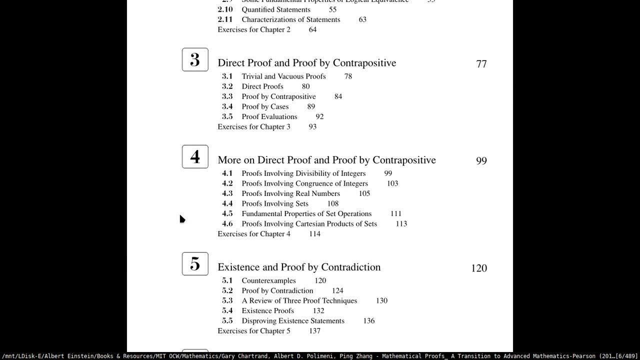 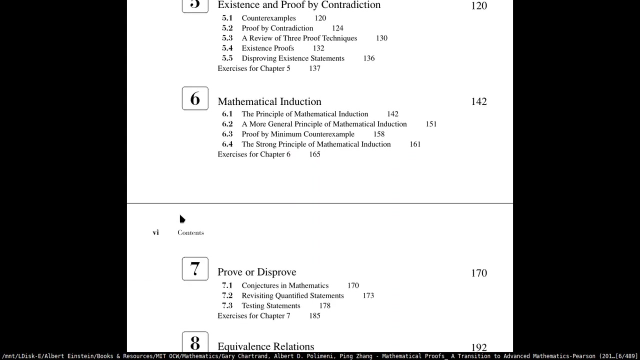 pick up certain things from certain chapters that would be helpful. For example, they have a chapter on group theory- proofs in group theory. that can be helpful, and even I think the chapter on logic would be helpful for someone who wants to know like about like how to make you know deductive statements in mathematical. 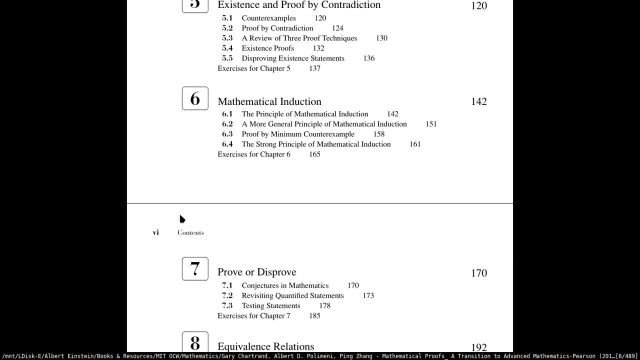 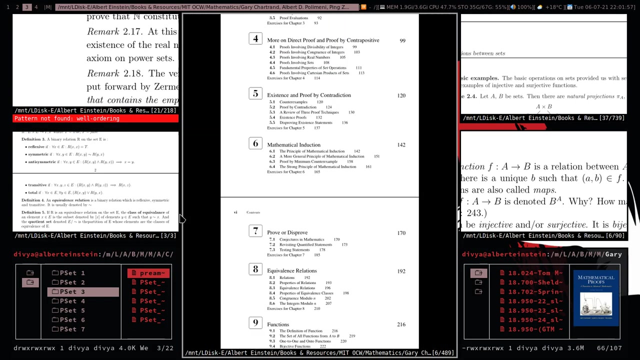 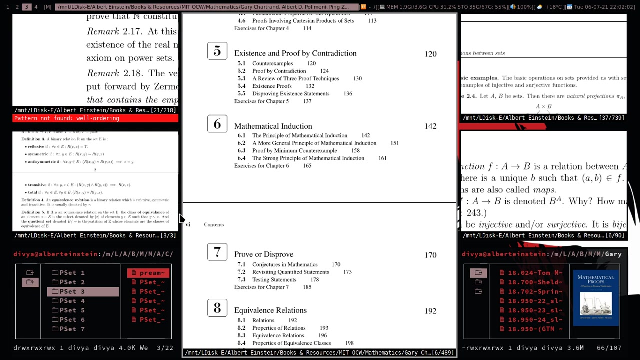 logic. so yeah, Okay then. so we'll meet on Thursday for the second lecture. we're going to cover the sections 3, 4, and 5 of Luffy. you're recommended to just skim through it and we'll go through. 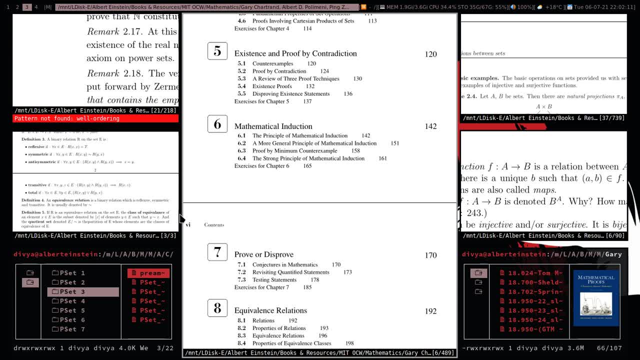 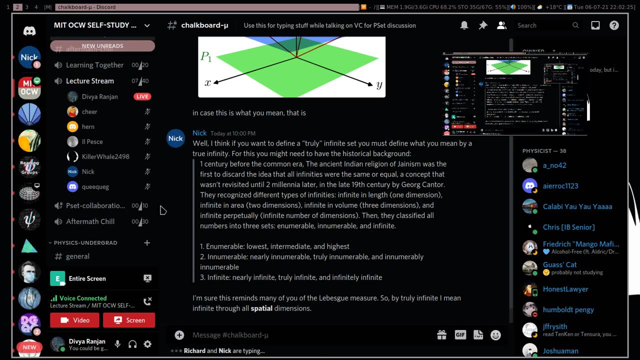 it together and, yeah, We'll meet categories. those are interesting things. so, yeah, Um, till then, um, take care and uh, see you on Thursday. Thanks for joining. Bye.